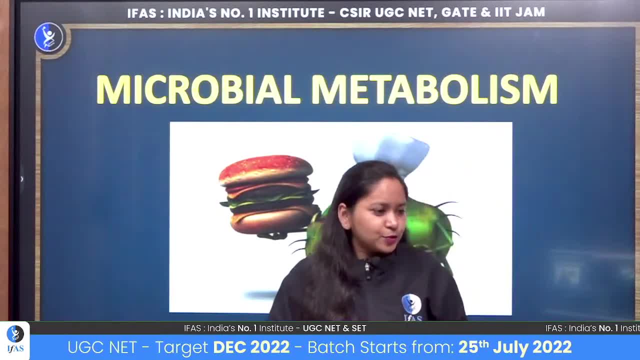 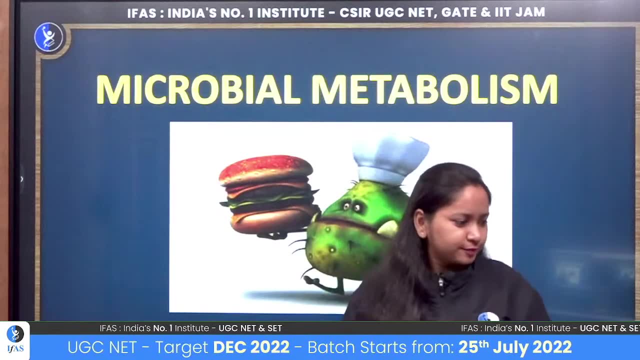 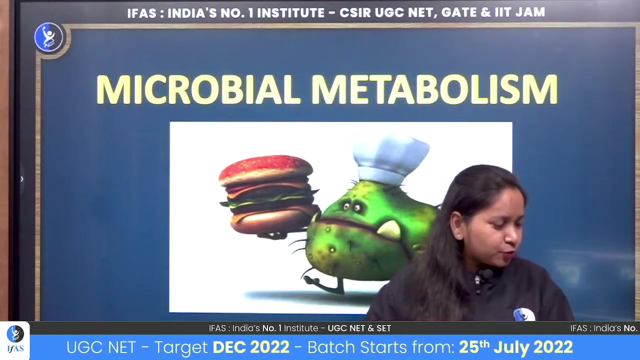 Good morning Vagdevi. So how are you all? How is your preparation? Good morning Abhinash. Best Abhinash, I think. first time you have joined live, I think, so Best, Great Good. 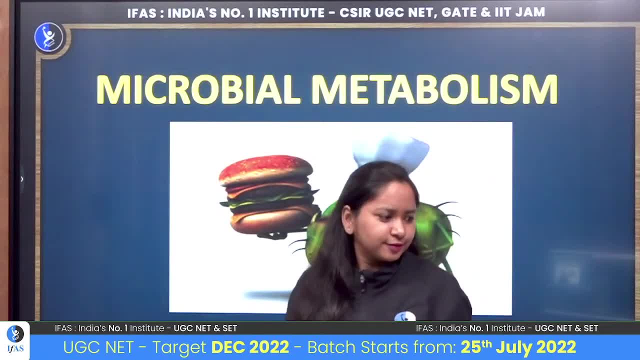 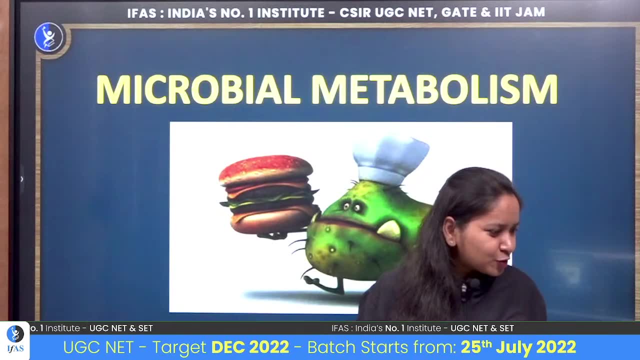 Good morning Anamika. Hello Nia, Welcome to the session. I think Nia is also new. Good morning Shubhi. Good morning Rakesh. Yes, guys, please come on, Share the session with your friends. 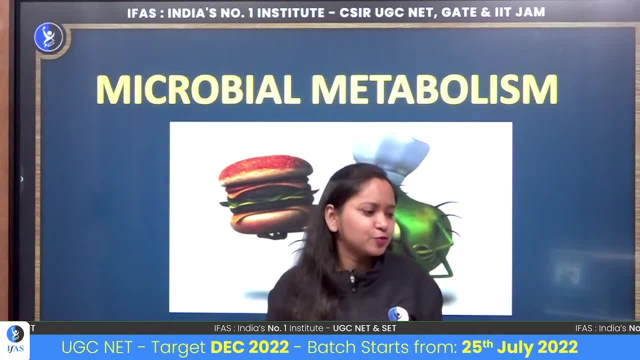 Text in your groups that the session has started. Tell everyone, Let's start the session. This is the last session of this series- microbiology series- which we started on Tuesday. We have taken five sessions. We discussed about bacteria, Then we discussed: 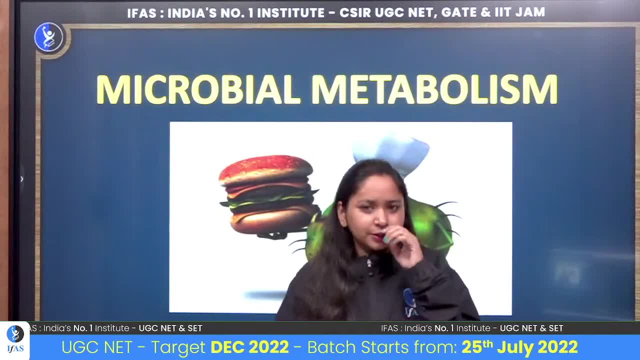 We discussed virus. We have studied bacteria virus, then we studied the genetics part as well. We also discussed the pathogenic organisms, and today we are going to discuss metabolism at the end. Good morning, Shreya. It's so nice to see you too. 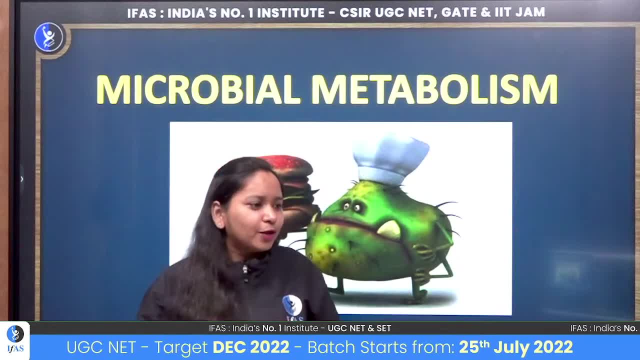 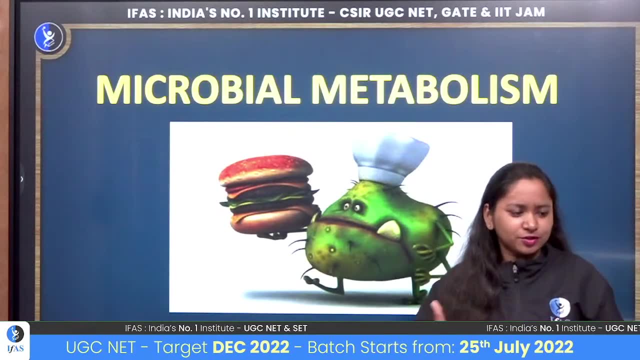 Okay. so yes, today we are going to discuss metabolism. So, as you can see in the image, what you can see is a pathogenic bacteria. a pathogen is there and he is trying. he is like balancing his food- Right. 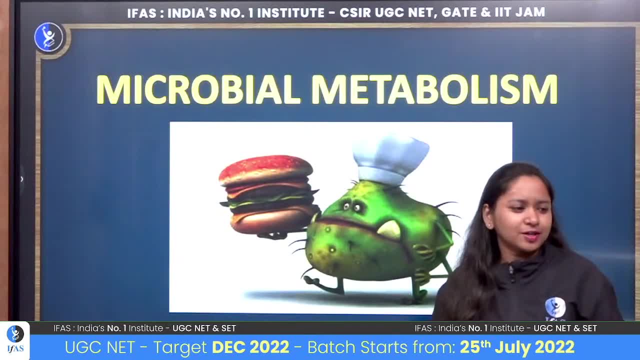 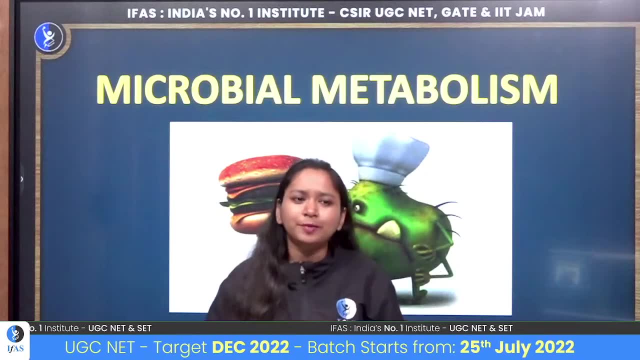 He is looking at his food, How to consume it, What to do. He is looking at everything. So we are also going to study that- how bacteria use your energy, how they metabolize things. okay, how they metabolize things, what they use, what things are present. we will discuss all of that in detail today. 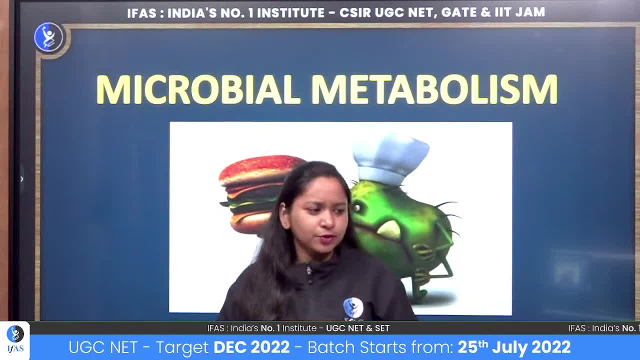 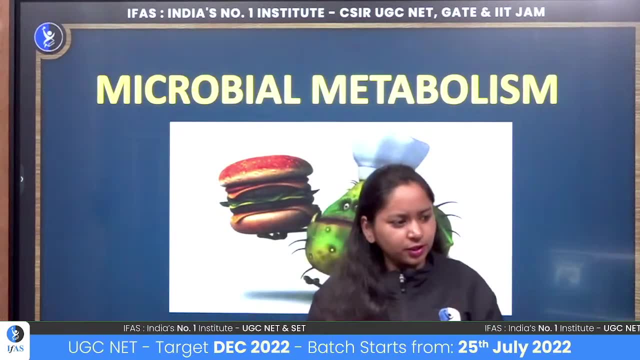 Okay, we have some questions also for you. like I have made like seven to eight questions. like yesterday's session, we will study first, we will practice some questions, then we will end the session. Okay, today's session is a little bit like. I will try to keep it for only one hour. 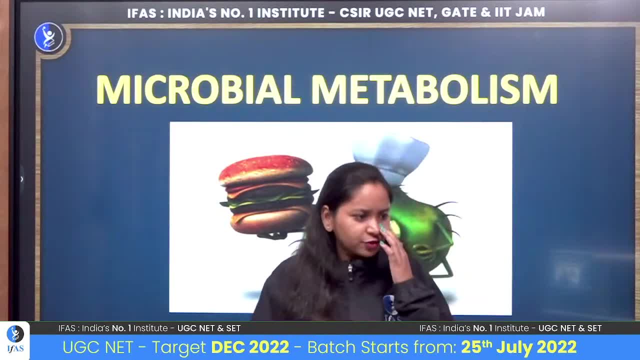 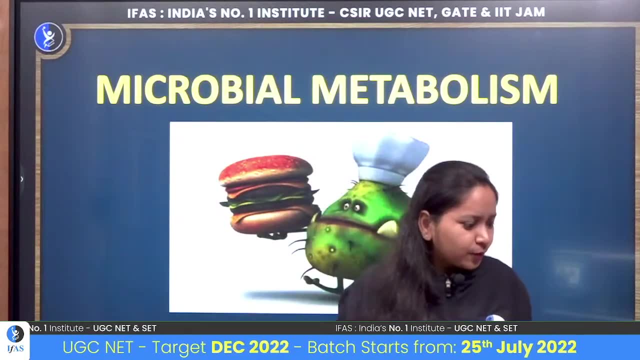 Yesterday we had extended a lot, So today's session We will try to complete it as soon as possible, because you have other sessions, so today's we will try that. Okay, so let's start the session. then come on, just text your friends, call everyone in the session. 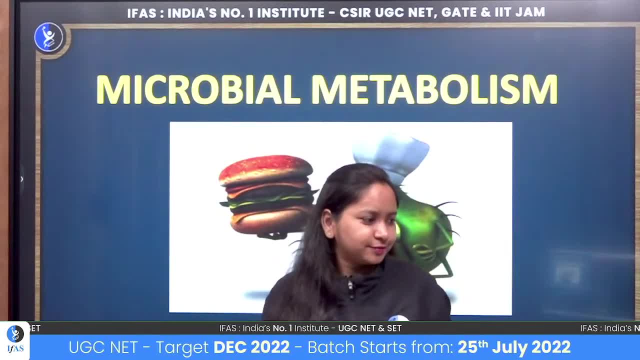 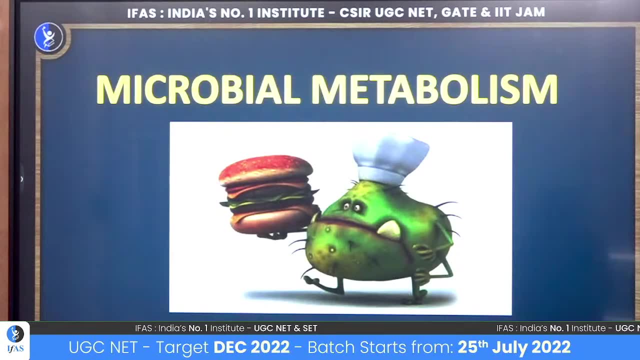 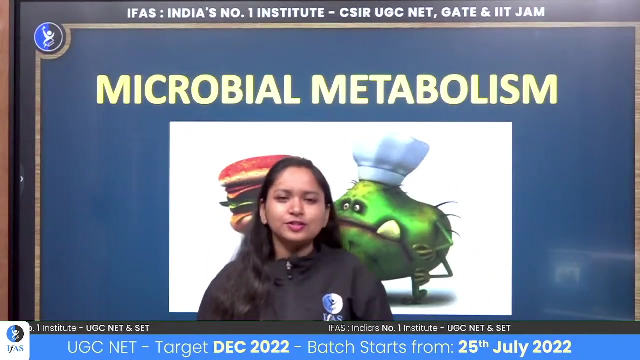 If everyone reads live, then it is very fun, right? Okay, Good morning Madhu. Welcome to the session. Welcome to the session. Yes, so let's start the session then. so yes, today we will read microbial metabolism. 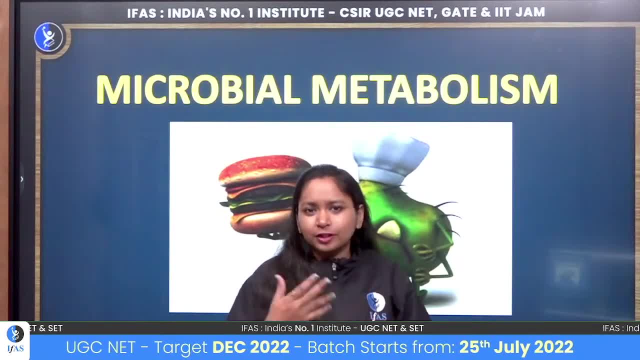 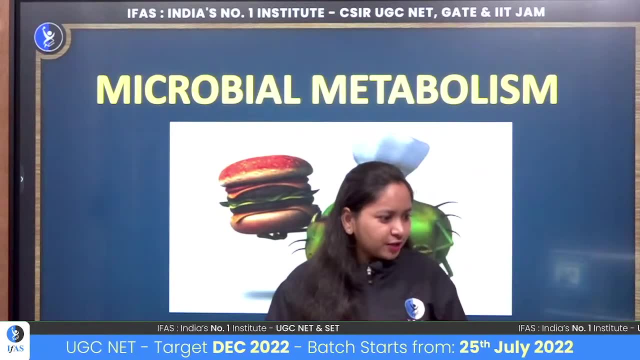 What does metabolism mean? All the metabolism pathways that are running in the body, all the metabolic pathways, Environmental meditation. I did not plan anything like that for you. good morning Manisha. If you have, If you want any sessions from our side. 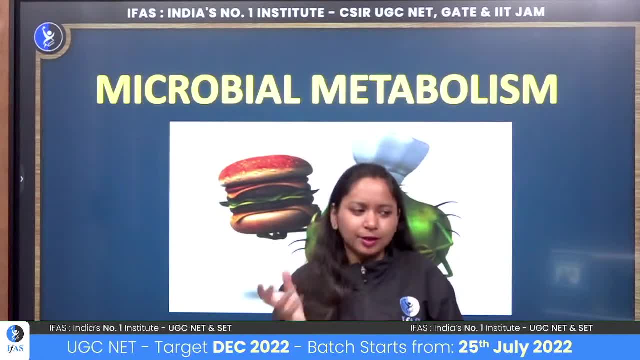 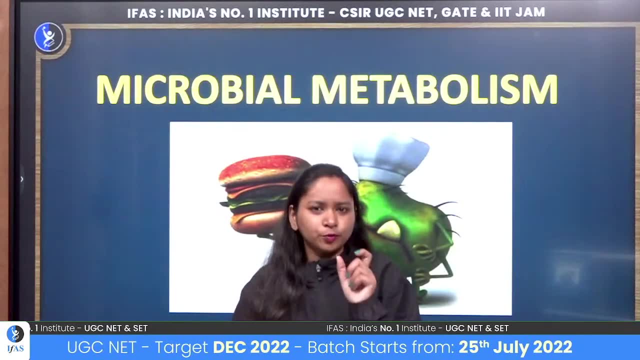 Then you can. We have a. If I mention what we have to study in the chat box, then we can plan those sessions for you. At the end of the session, in the comment box you can post your request that which paper revisions you want. 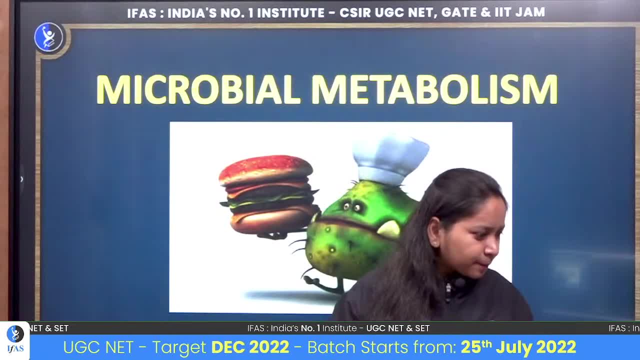 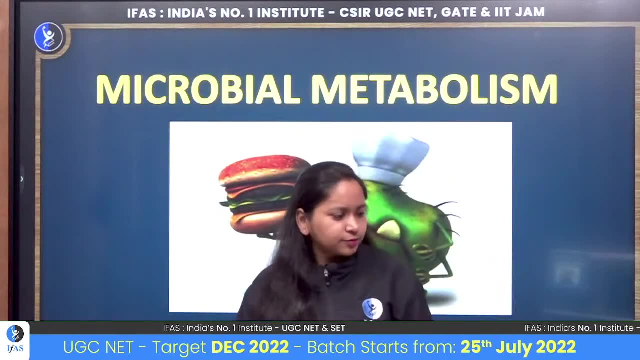 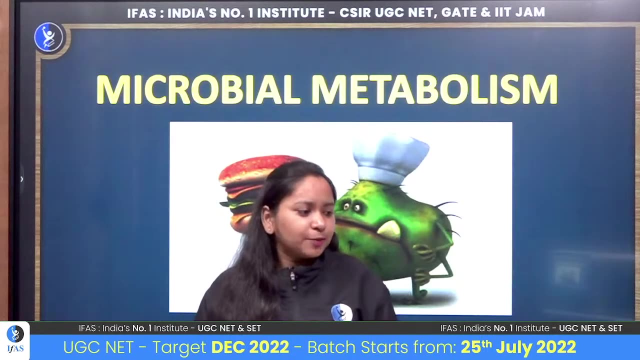 Accordingly, we can plan things for you. Good morning, Manisha. MTech Bio Process. Yes, it's good. It's good, Rakesh. So, yes, if you have any request that we have to study this topic- we want this revision- then you can post your messages there. 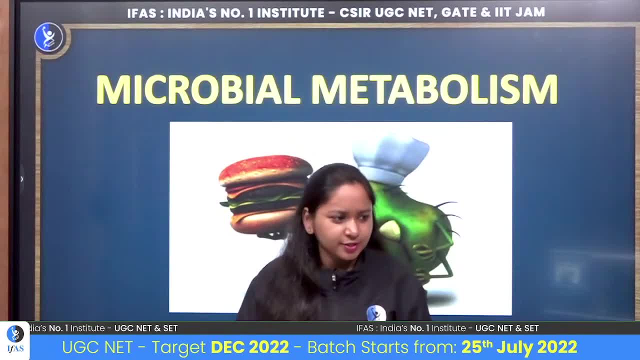 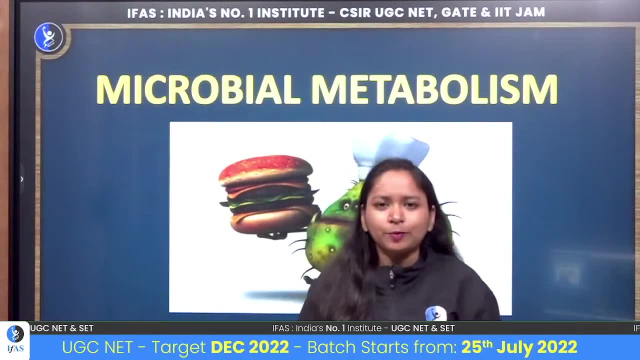 So we will see that and, accordingly, we can bring sessions for you on this particular channel. So, yes, if we talk about your metabolism, then what I tell you is that there are many metabolic pathways running in the body. We have glycolysis, TCA cycle, we have electron transport chains are present in the body. 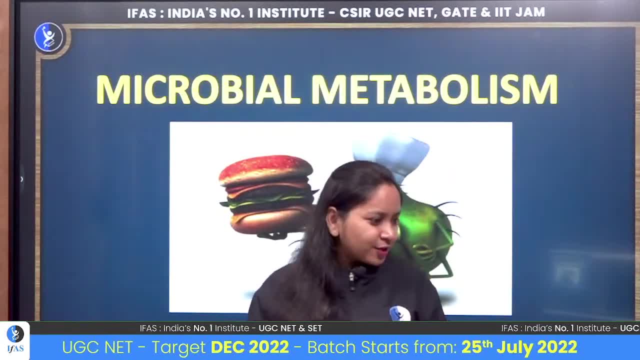 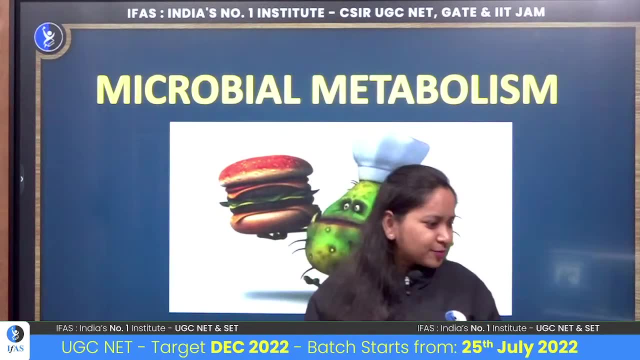 Wow, Rakesh, that's great Congratulations. Good morning, Meenal. Congratulations, Rakesh. So good to see. Here's some good news. Yes, yes, Vagdevi, correct, It is a way to produce energy from the digested material. 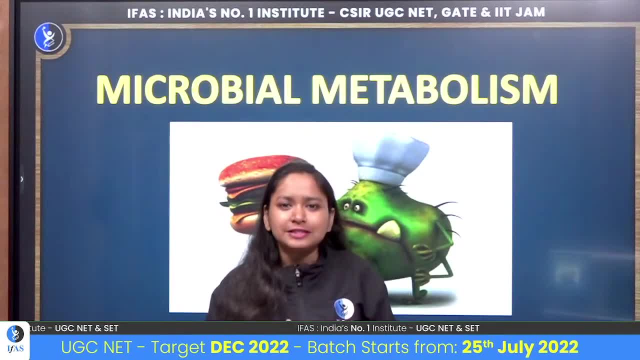 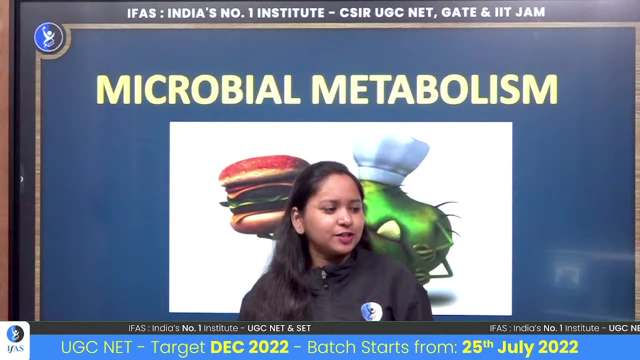 Yes. so whatever food you consume, how can we use it in the form of energy? It all happens in your metabolism, because what is our energy currency? What is the energy currency for us? What is the energy currency for us? What is our energy currency for us? 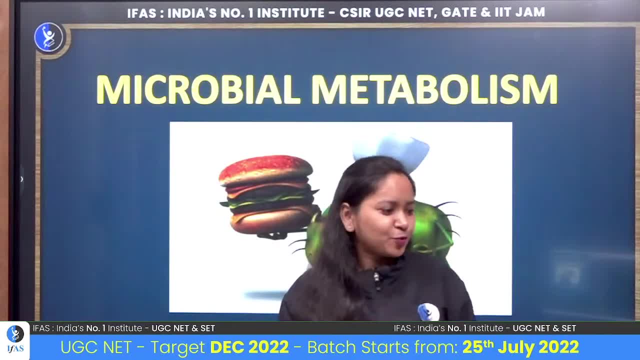 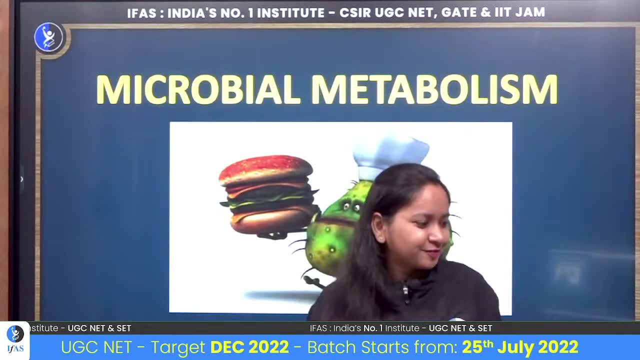 See, this is what I say. This is our small YouTube family, So involve as many as possible. There are like so many blessings and wishes for Rakesh here now. Yes, it is ATP Good Sonal Radhiksha Vagdevi, Shubhi, Rakesh Life Science: yes, yes, 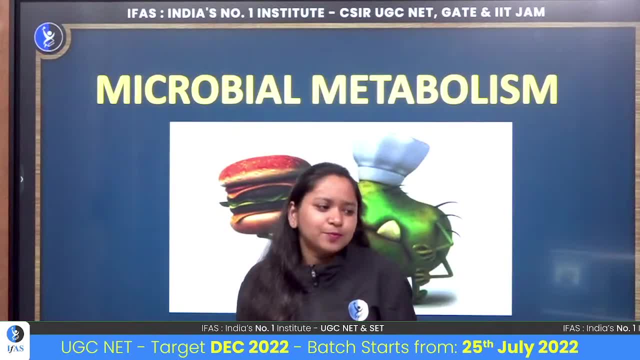 So our energy currency is ATP. If you have eaten something, if you have eaten a good idli for breakfast, then you don't use idli directly. If you have eaten something, if you have eaten a good idli for breakfast, then you don't use idli directly. 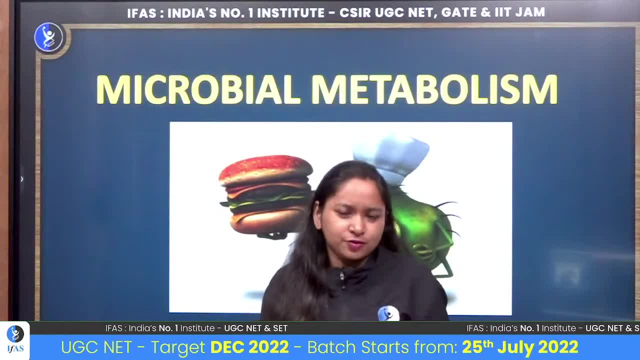 If you have eaten something, if you have eaten a good idli for breakfast, then you don't use idli directly. We basically use ATP as our energy currency. Okay, So what do we do? That idli will break our body in small pieces. 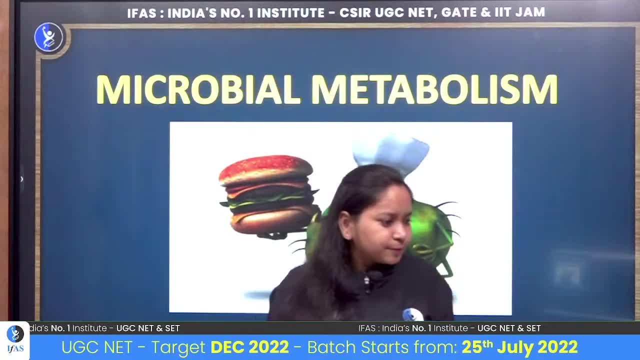 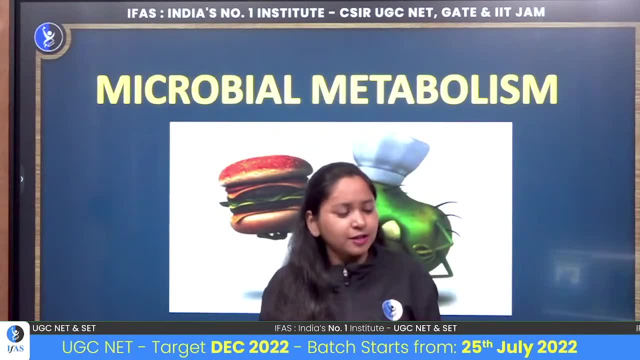 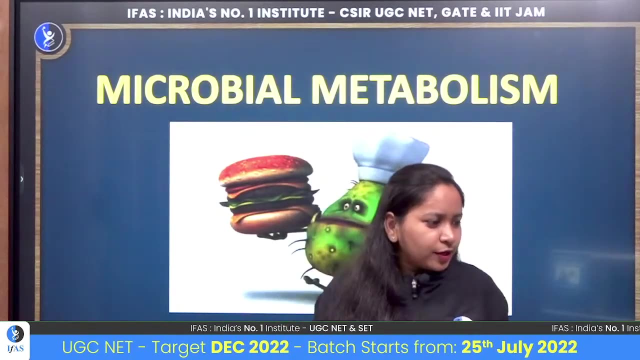 We will absorb some energy After that. why that, Anjali? Why you rejected it? If you have any good reason that if you got some better opportunity that you wanted, then it's good. Definitely it's good. It's on your choices, child. 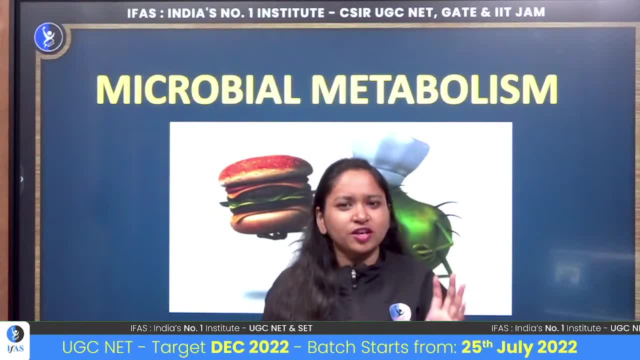 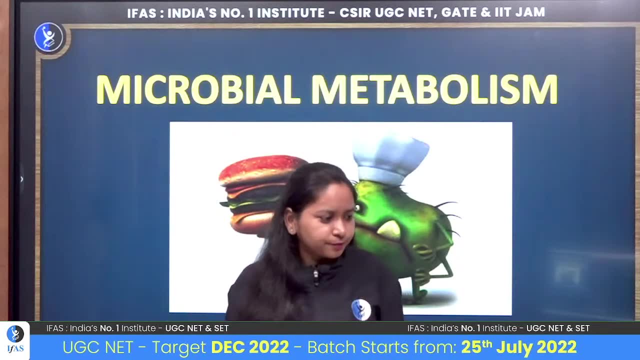 Because we, like I also like, want, like, suppose I want to do this thing, So we also reject good things for that, Like, if you are happy with your decision, it's completely fine, No issues. If you had some other plans, then it's the same decision for you. 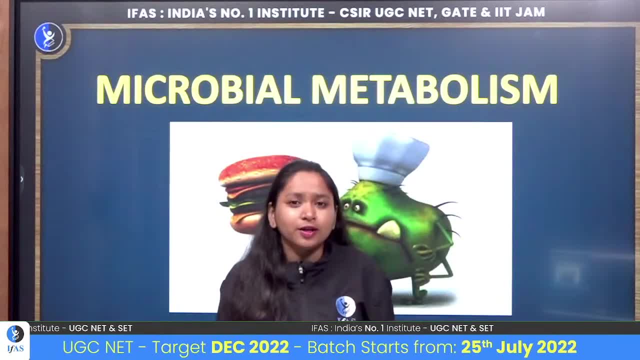 Okay, Just follow your dream, follow your passion, child. Okay, Don't just be like, okay, someone is doing it, someone is not doing it, You do whatever you want to do. All of us have some dream that we want to do this thing someday in future. 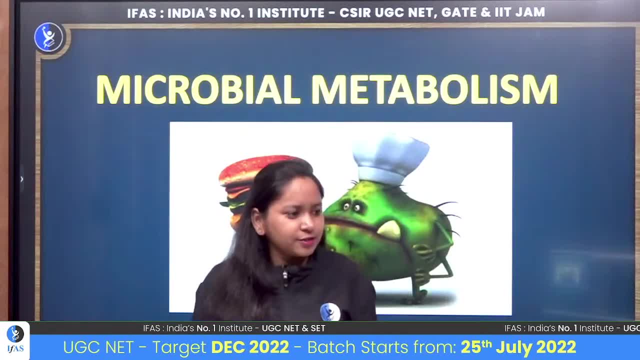 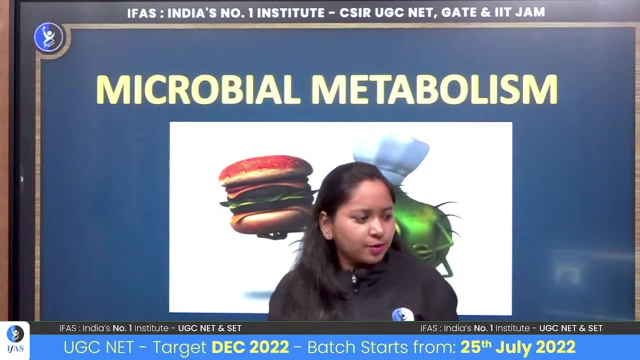 So just pursue that, Okay, And if you need any guidance, we are always there for you. You can do messages. You can write in the chat box, You can post messages on the app. We will reply to you. by the way, 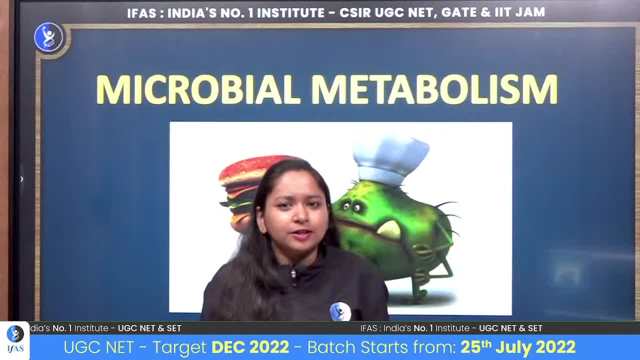 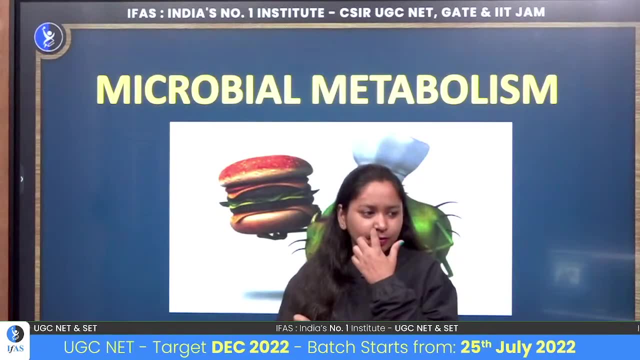 Okay. So yes, what are we going to study in Metabolism? So how will our body make ATP? How will it increase bacteria? Actually, we are not going to study. We will study how bacteria performs, So how they are preparing energy. 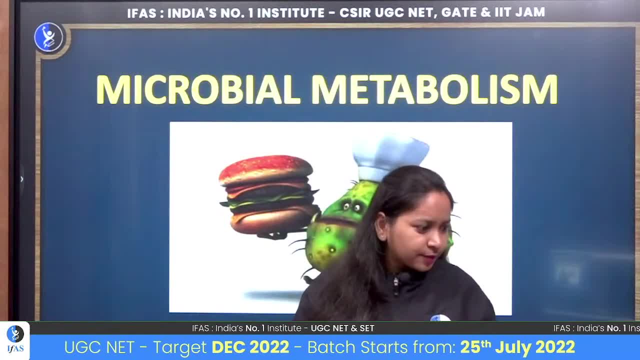 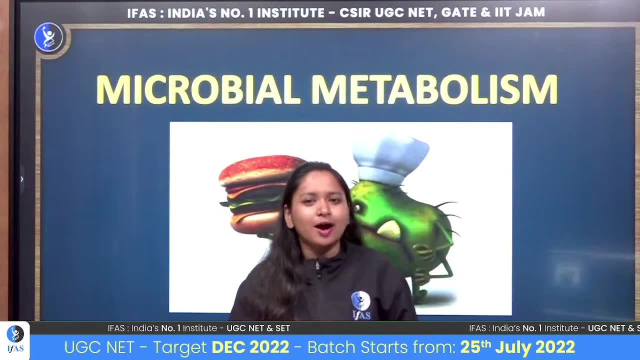 How they are utilizing ATP. We are going to discuss all that today, Good Rakesh. So that's it. If you do hard work properly, then you will all achieve your dream. We all have a dream college Right. 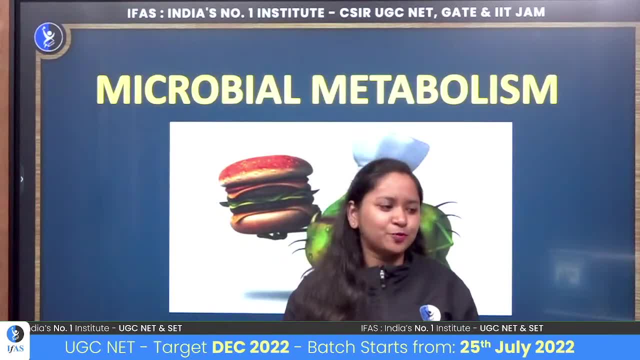 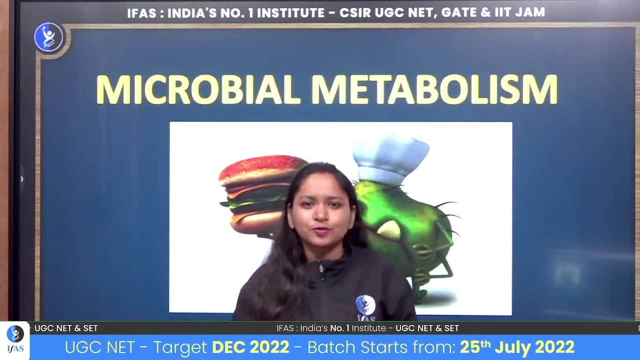 Everyone has a dream college That I have to go here. I have to take this selection, I have to study from here. So I hope all your dreams are fulfilled. I just hope you have to do hard work. You just have to prepare properly for all the exams. 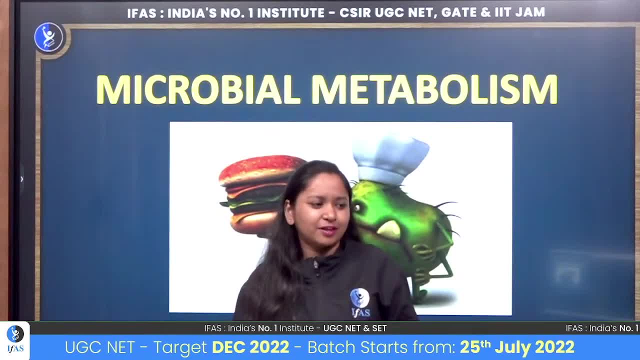 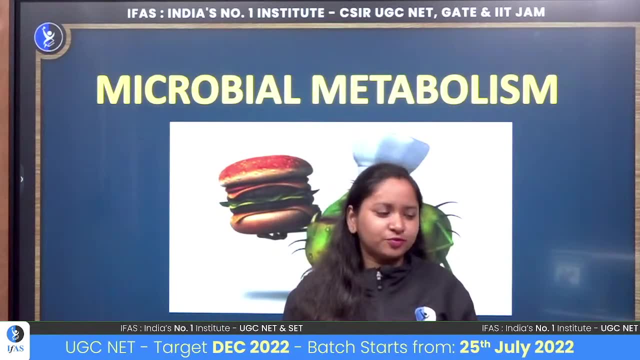 You don't have to do any work right now, That we will leave one and study. The more hard work you do now, the easier it will be for you in your future. Okay, You will get your dream college. I hope this is for everyone. 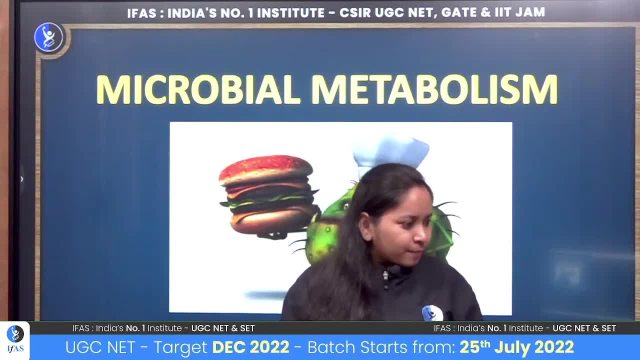 Everyone gets their dream college, Come on. So many good wishes and blessings for Rakesh. So, yes, let's start the session. We are studying Microbial Metabolism. What is Metabolism? So there are two important things. 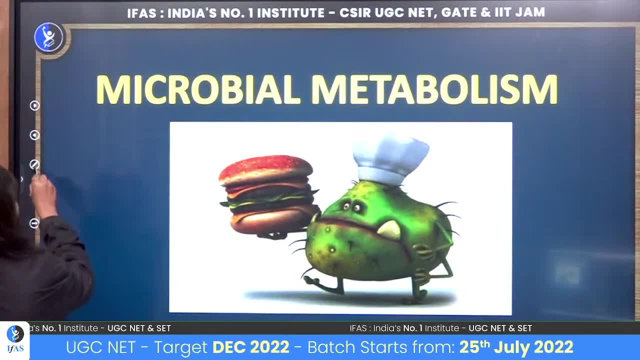 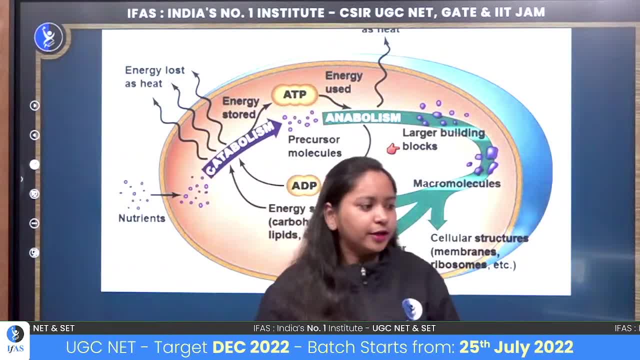 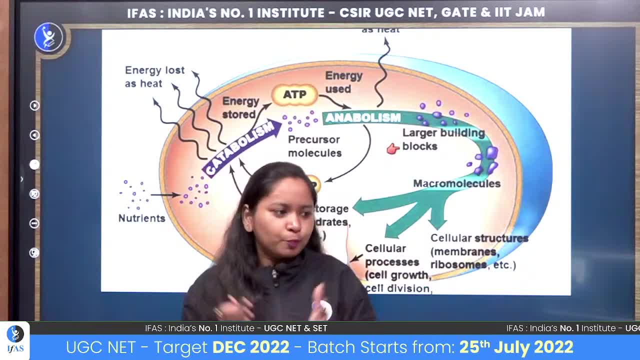 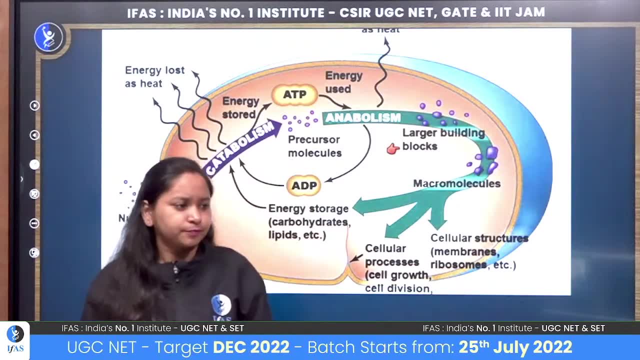 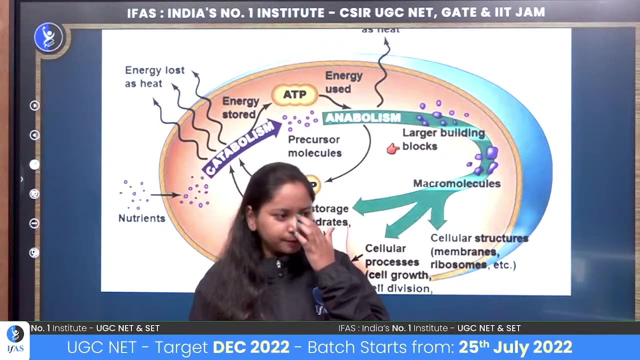 Okay, What is Metabolism? What does it mean? What does it mean Make macromolecules? What is To make macromolecules? Anabolism or Catabolism? To prepare To make energy Macromolecules. Is it anabolism or cat ablazite? 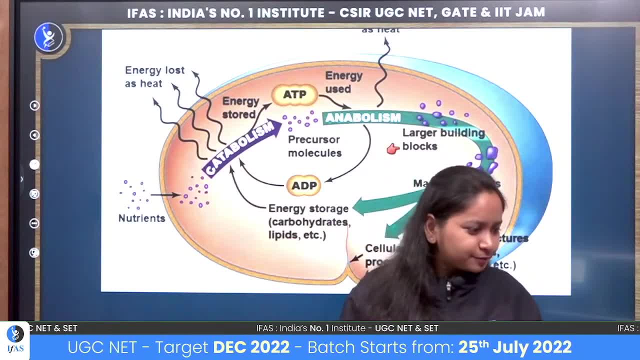 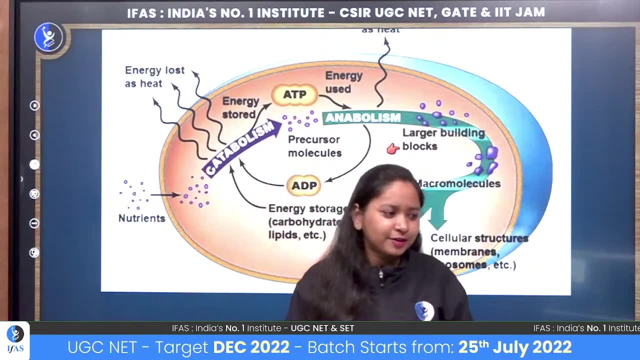 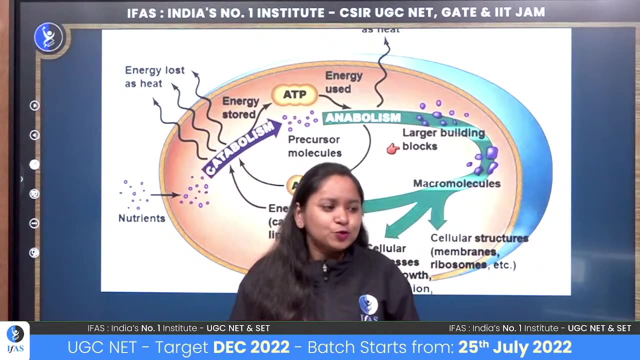 Anabolism- Paramissing Anabolism. Good Morning, Param, Adhikshaising Anabolism. Sonal Vagdevi: Yes, Yes, Shreya. Yes, Anamika, Yes, you all are right here, okay, yes, Shubhi, Rakesh, Anna. so, yes, yes, Aditi. so what does anabolism mean? so, where you are preparing something, that is anabolism, and when you break something, we call it catabolism. 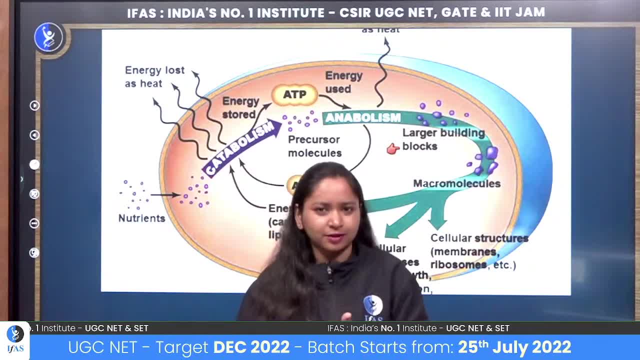 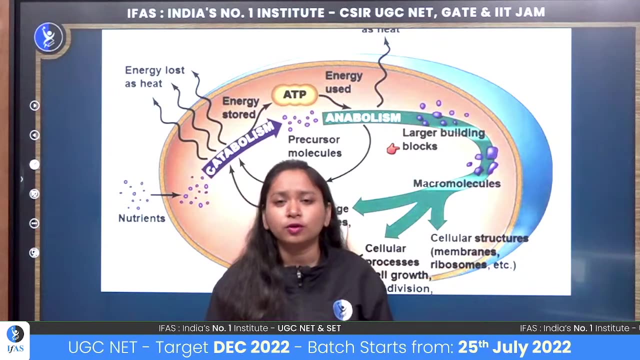 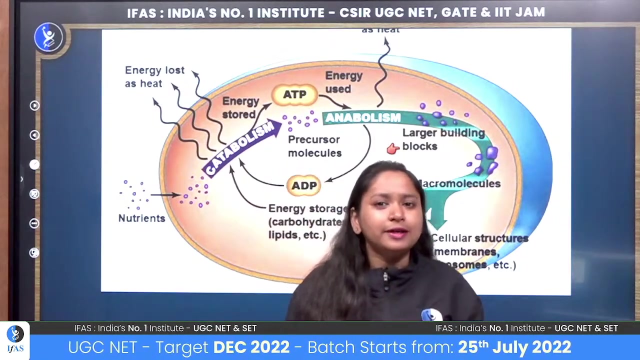 catabolism. if you remember, cata means to cut something. that is catabolism. so when your body needs energy currencies, when your body needs some energy in small forms, then our body performs catabolism. that is when you break- yes, you break- all the complex molecules. you break all the macromolecules into small pieces and you take energy from that. we call it catabolism. but yes, when you eat, when you are consuming food, at that time what will happen? a lot of glucose in your body. 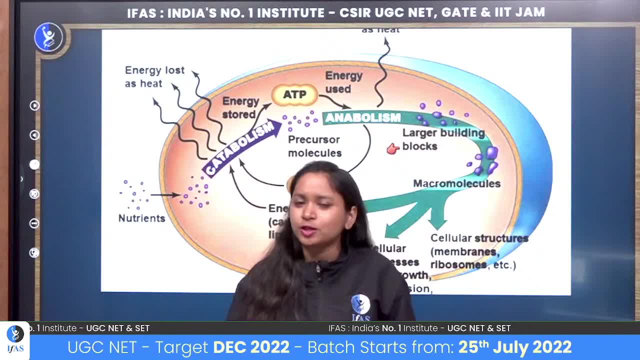 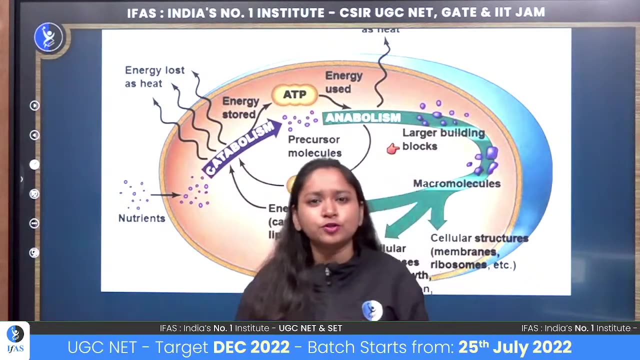 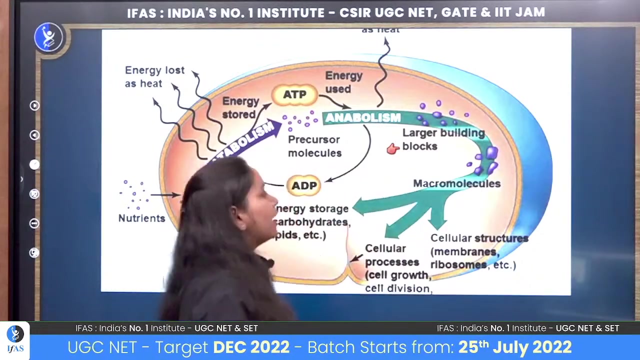 a lot of glucose will come together, a lot of energy particles will come together, a lot of biomolecules will come together. so keep it converted, keep it prepared into a large macromolecule- we call it that. then you have an anabolic pathway, okay, in which you do what in anabolic? what are you doing? you are making things, storing them. what do you do in catabolism? we break those things into smaller particles and, yes, we get energy out of it. okay, our ultimate aim is ultimate. 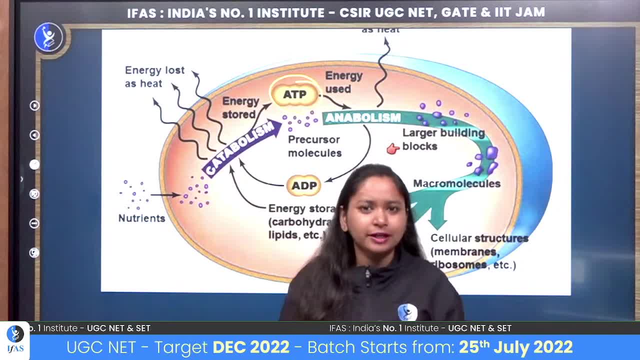 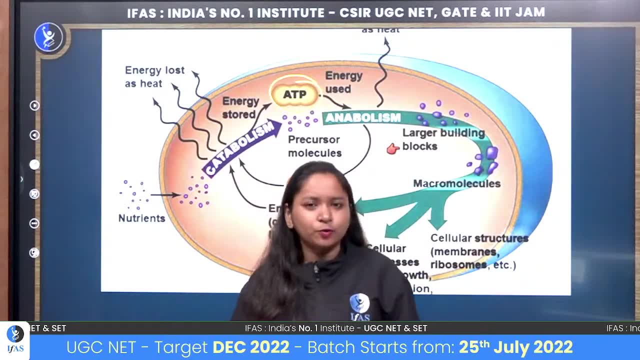 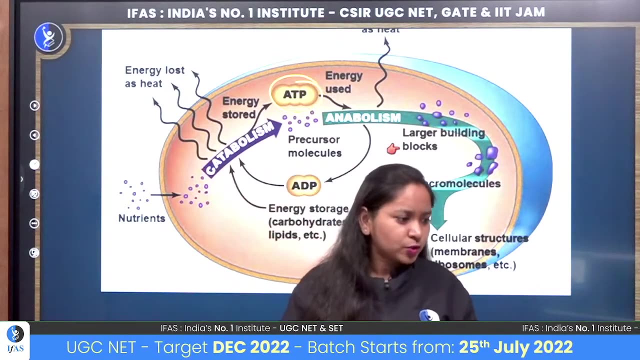 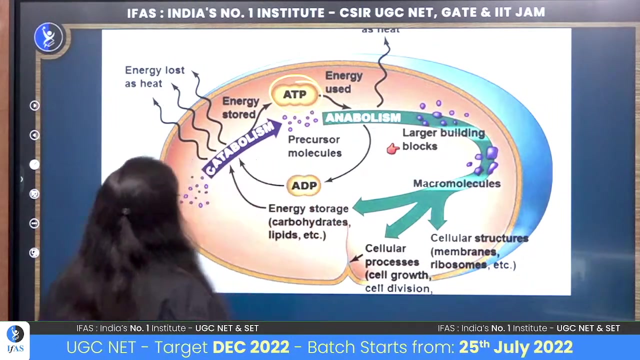 our ultimate aim is that we always use ATP. we have to make ATP, ultimately, because that is our, that is our actually currency. okay, if we also have to buy something in the shop, then what do you do? you take money, cash, money we take. we can't take any other form. so that is your anabolism. okay, most welcome. okay, so let's move to the next part. so, yes, if we talk about anabolism, then what is happening here? your large building molecules. 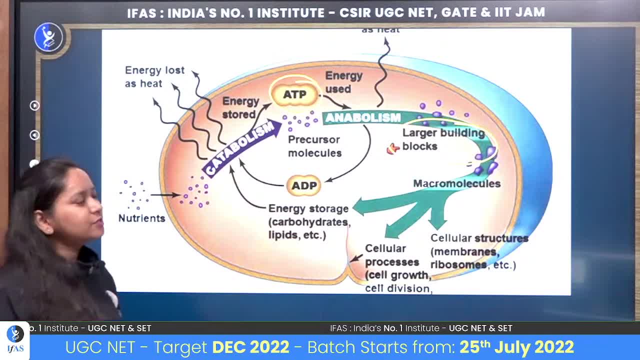 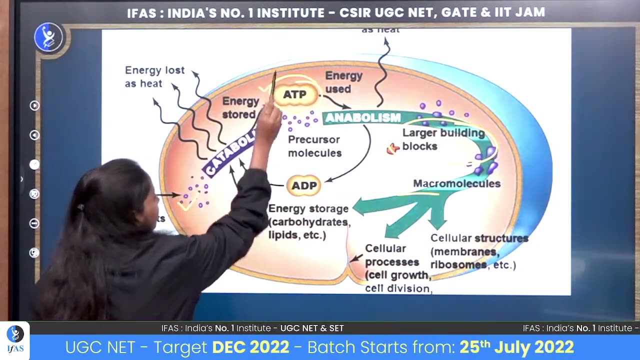 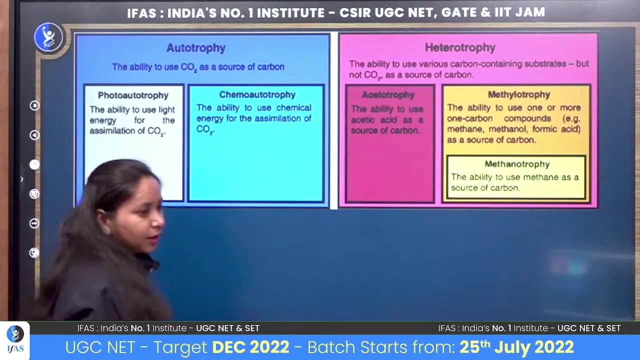 these are formed. okay, in case of this anabolism, what happens? these larger molecules, they are just formed. and if we talk about catabolism, then what happens here? here, whatever macromolecules are there, they are broken into smaller pieces and, yes, whatever energy you have in the form of ATP, we are getting that. okay, so that is anabolism and catabolism. now next part: now, if we talk about your microbes, how we classify our microbes? so, yes, 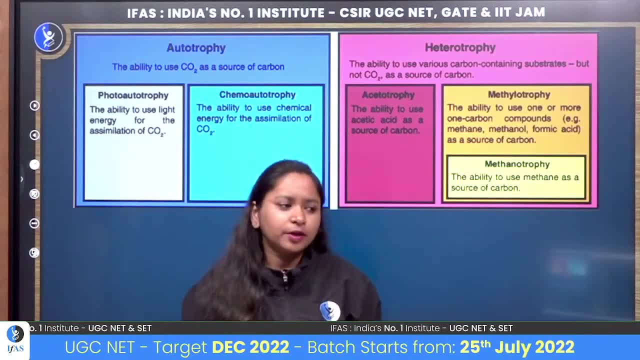 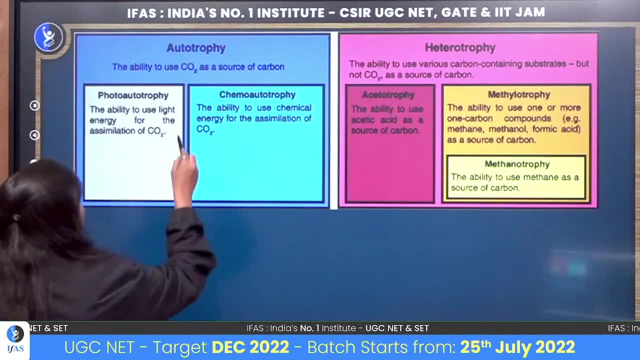 yes, now, okay, so how we classify it? so one is your, one is the mechanism of autotrophic, one is the mechanism of heterotrophic. okay, what does autotrophic mean? ability to use carbon dioxide as a source of carbon. 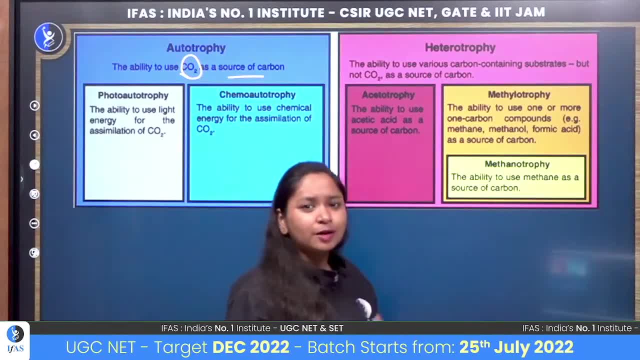 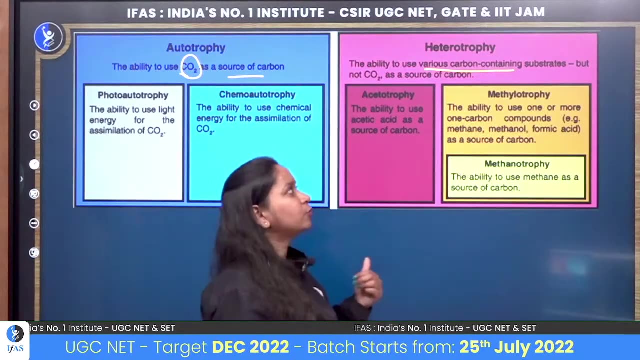 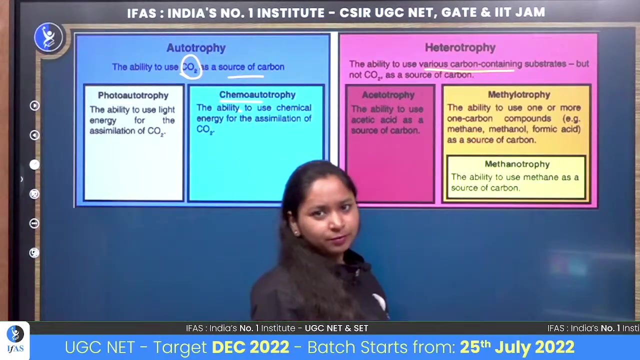 in this you get such species which use carbon dioxide as a sole source of carbon. and what happens here? here, your various carbon containing substrates are used. okay, whatever can be used those species, they are performing this heterotrophic mechanism. if we talk about autotrophic, which again comes in your photo autotrophic, and one comes in your chemo autotrophic, what will happen? photo means it is related to the photosynthesis, that is. photo means you are using light, photons are being used. so, yes, those who use your light for the energy production, we call that they are performing photoautotrophic. 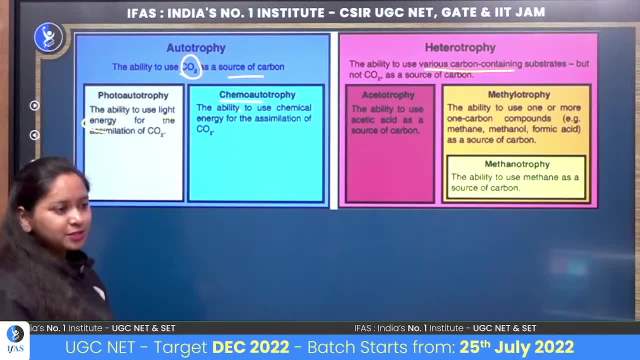 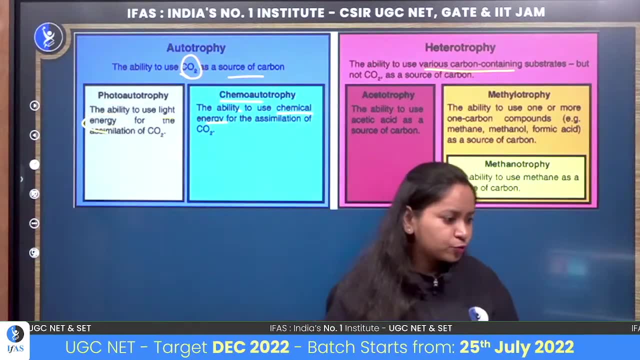 and those who use some chemical substances, which are using some chemical energy for the assimilation of CO2. they are called chemoautotrophs. yes, Riddhiksha, good, so they are called. yes, what will be the meaning of photo? 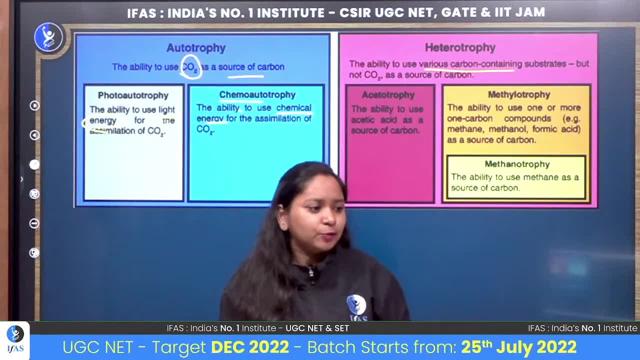 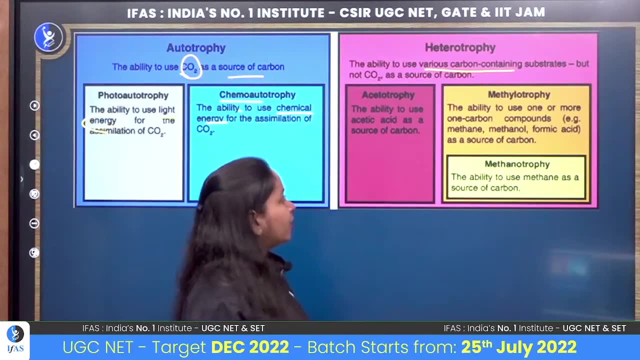 you are using photons, that is, you are using some light, and what will be the meaning of chemo? you are using some chemical substances there, so they are called autotrophs. if we talk about heterotrophs, then some more things will come here. 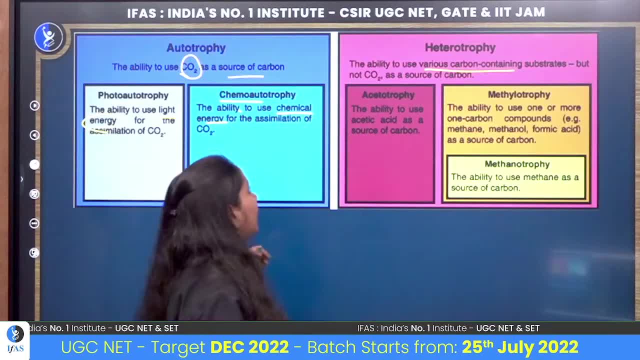 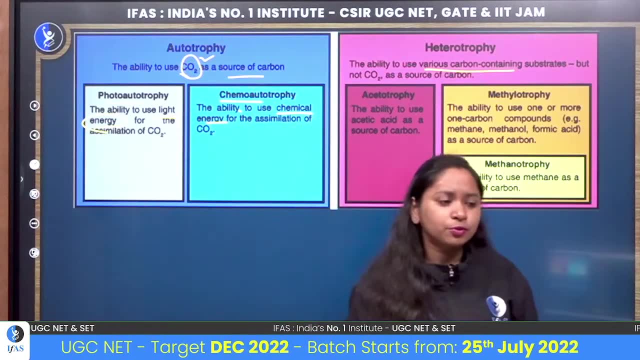 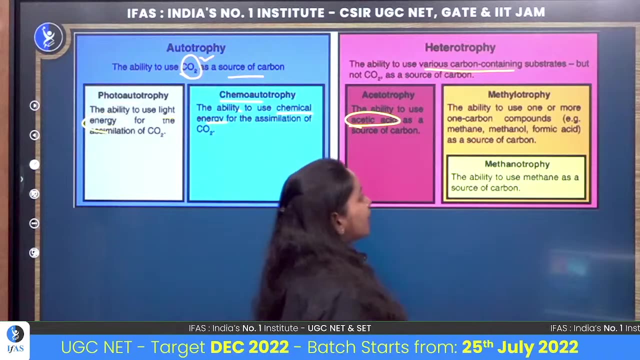 some more complex molecules will come here. what is simple here? simple carbon dioxide was being used here, but in this case we will not use CO2. we will use some more things here, like one: is your acetic acid? ok, either, the bacteria can use acetic acid. 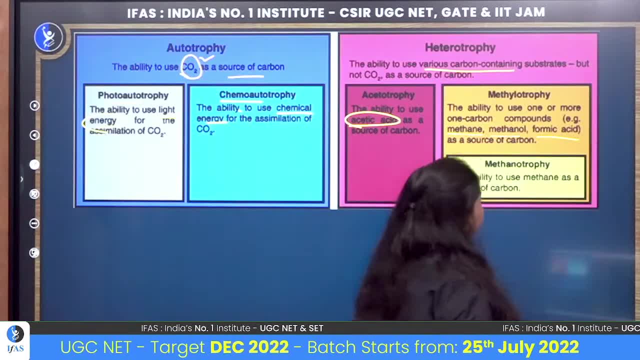 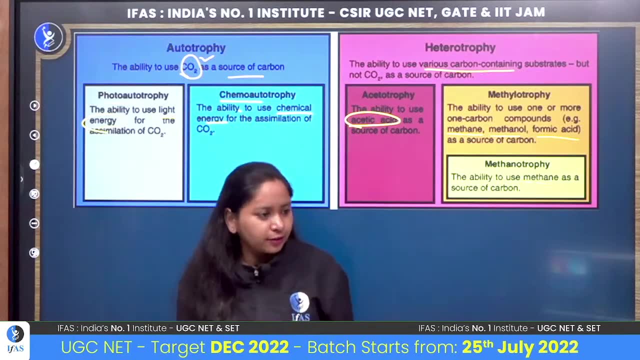 or it can use methane, methanol, formic acid. ok, so you have many such microorganisms which use some more compound of yours. ok, so you have many such microorganisms which use some more compound of yours to get the energy. they usually belong to your Archaea. 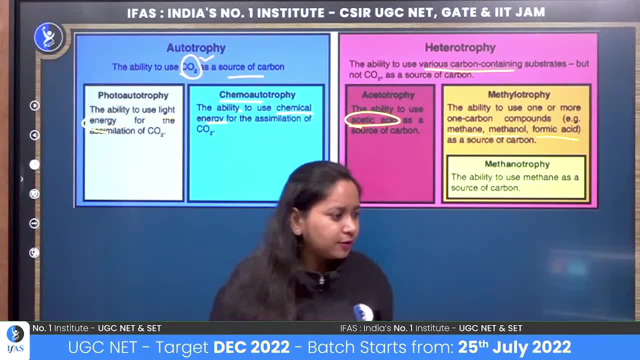 you must have heard of species. have you heard of the word Archaea? what is Archaea? what is Archaea? have you heard of Archaea species? guys, please, I can share the session as well. good morning, Samad. what is Archaea species? Archaea species. what type of bacteria comes in Archaea species? yes, Samad, they survive in the extreme conditions. ok, Archaea species means such organisms come in it. yes, thermophiles can be there, cyclophiles can be there, halophiles can be there. 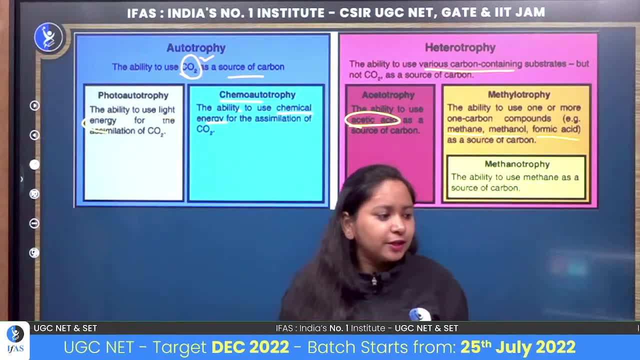 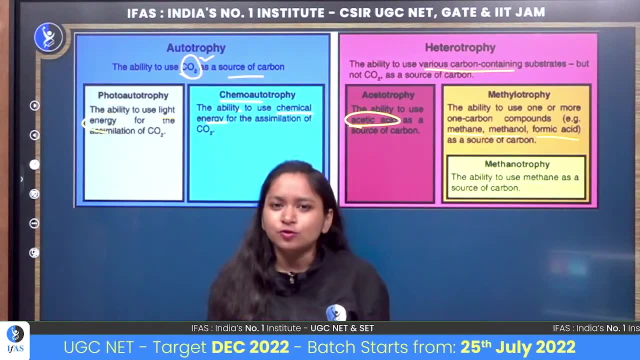 ok, so those who are there, they survive. yes, they survive in your extreme conditions. ok, your earlier 5-gram system: there was no space for Archaea. you know, in the 5-gram system which are there protista, which are there in the 5-gram system. 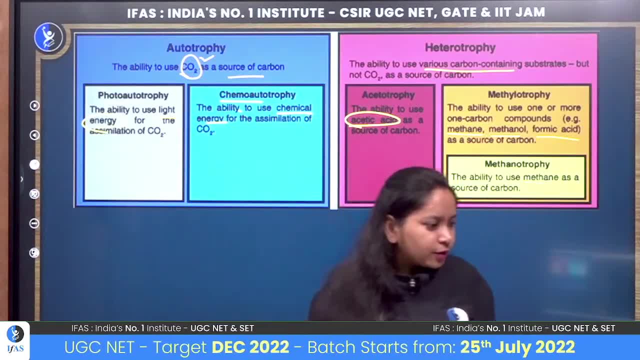 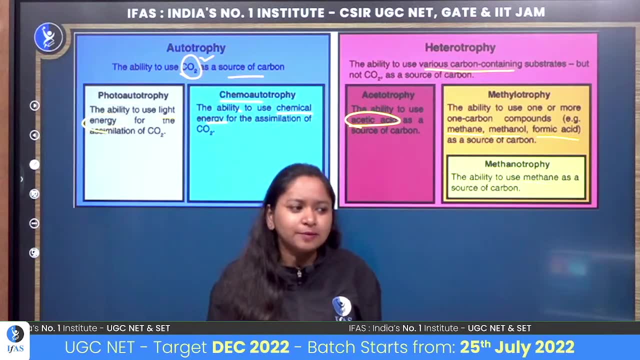 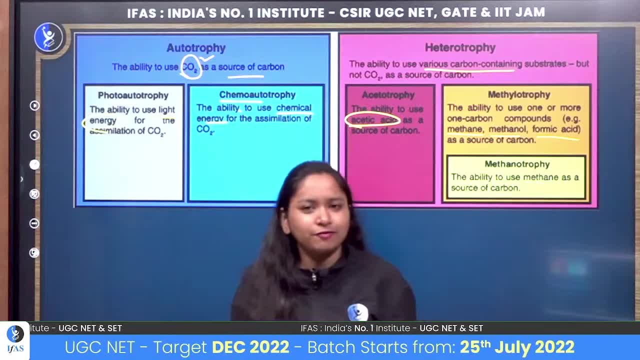 your 5-gram systems. there means: yes, monera, protista, fungi, planty and anemalia. yes, monera, protista, fungi, planty and algae. Yes, monera means. monera means protista means, but for Archaea. 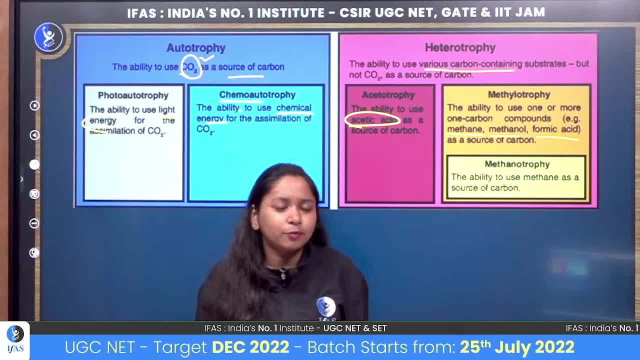 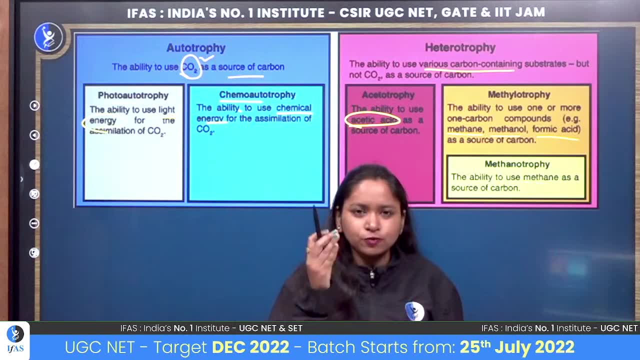 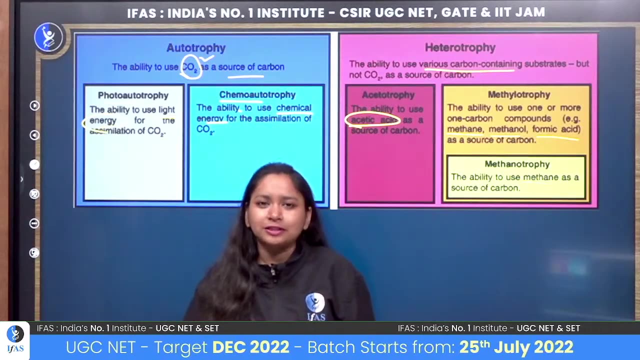 there was no space because Archaea they are very different, their organisms are are very different. they are basically prokaryote. we can say interlink between the eukaryote because to the prokaryotes, ok. so that is why after that your three domain system came in which 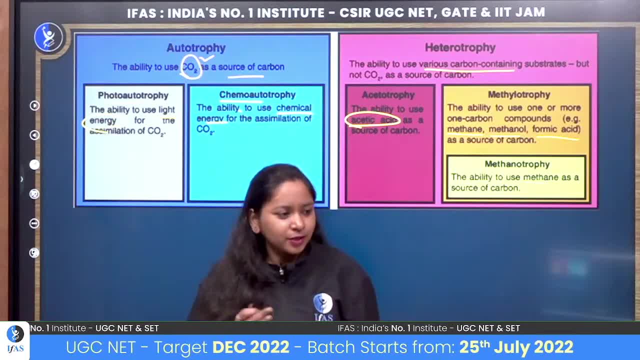 what has been done now. so all your prokaryotes have been kept in a different place, a different class of Archaea has been found, a different family has been found and all your eukaryotes come in one place where your plants and animal cells will come. ok, so in this way, your three 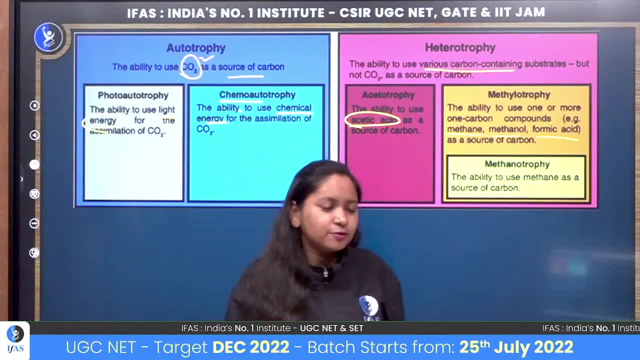 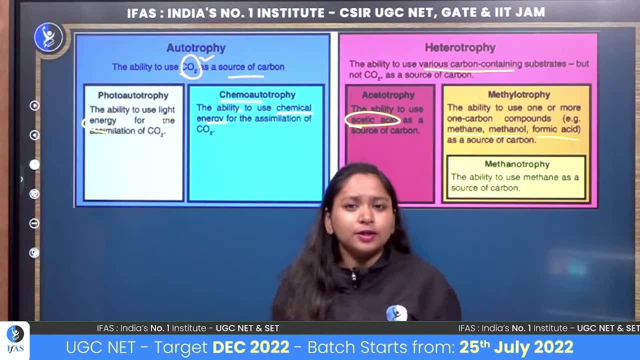 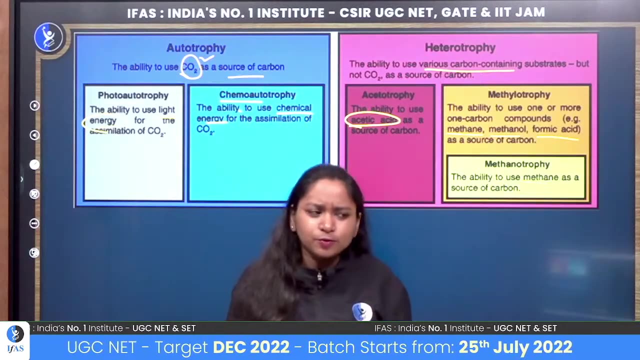 kingdom. sorry, your three domain system has come basically now in which what is happening. so in this your Archaea was also given a proper separate category. so your Archaea is a child. they use some of your extreme conditions. ok, they survive in, like extreme conditions means they can be in extreme cold where there is a lot of heat. such organisms 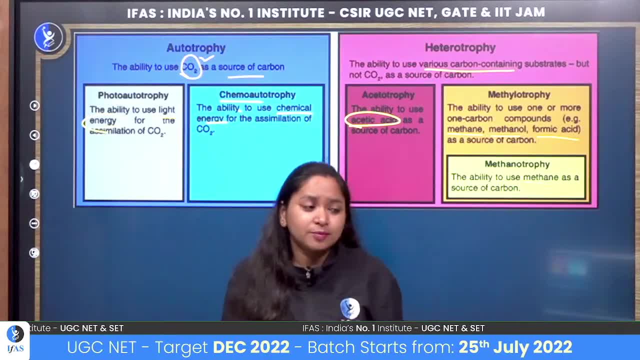 survive there, they use methane. there are a lot of summer methanotropes who know how to use methane. ok, so some of your species are like this. these are all belonging to the heterotrophic class, so they also carry some of your different pathway separately. 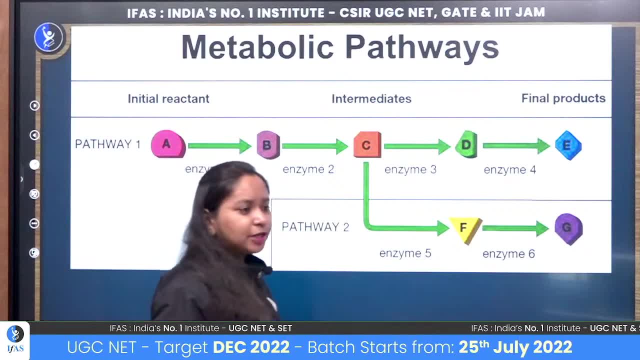 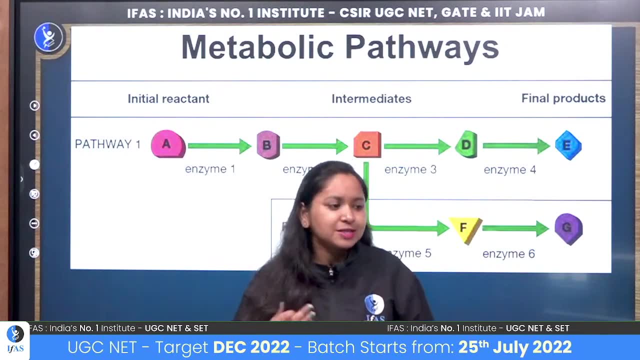 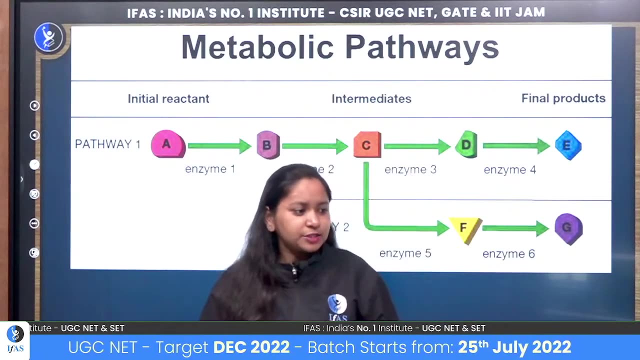 now, if we talk about metabolic pathway, so the metabolic pathway is like this: the metabolic pathway is what happens. then if we talk about your metabolic pathway, then here what will happen? here your many substrates are used. ok, here, many substrates. are there substrates to which we call your precursor molecules? ok, precursor means. 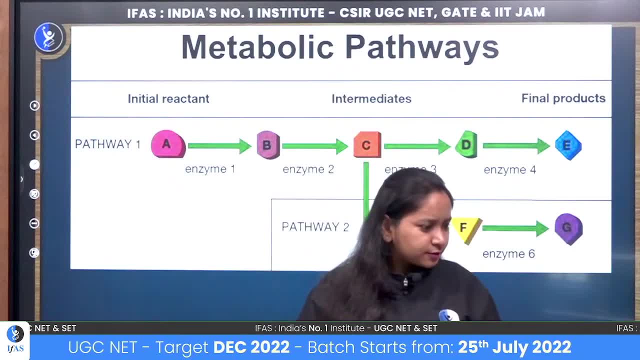 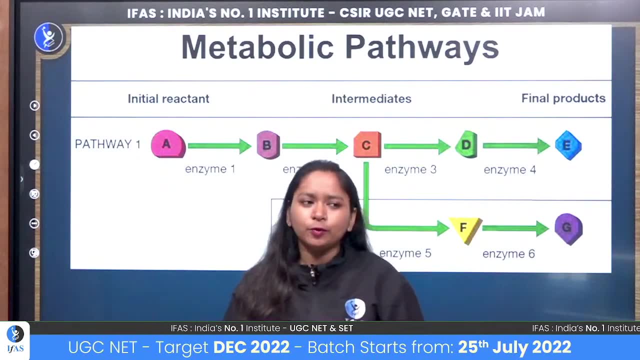 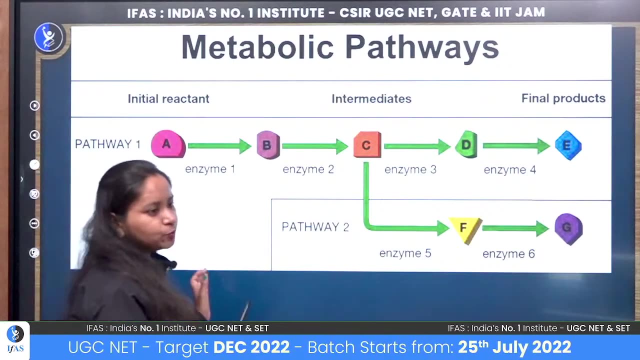 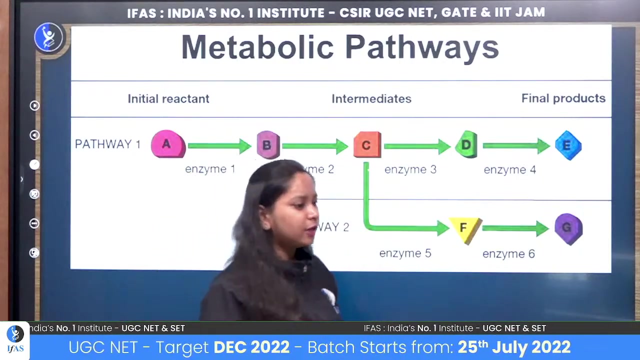 what happens? yes, ok, whatever your precursor molecule is, what happens then? they are yours, The ones who are the oceanic molecules? ok, they are called precursor molecules. ok, Metabolites are formed by using them and in the end we get a product. So today we will discuss how the metabolism bacteria performs. 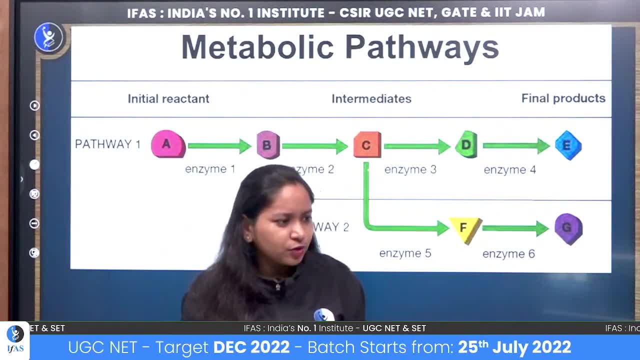 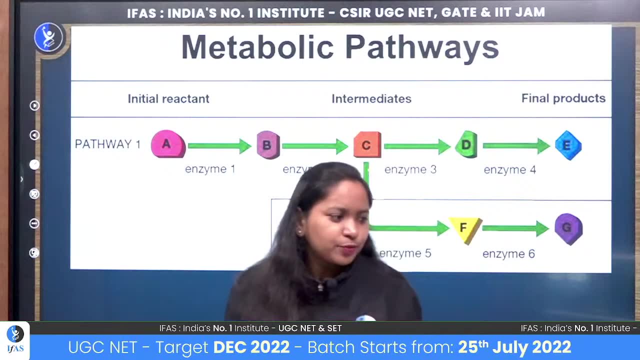 We will discuss some important pathways which are very important for you, And I will be taking only the session for like approximately one hour. Yes, precursors, which initiates the reaction. Yes, when your first metabolite is there, we also call it precursor. 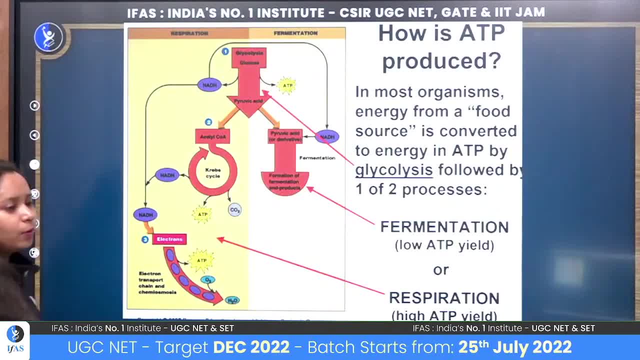 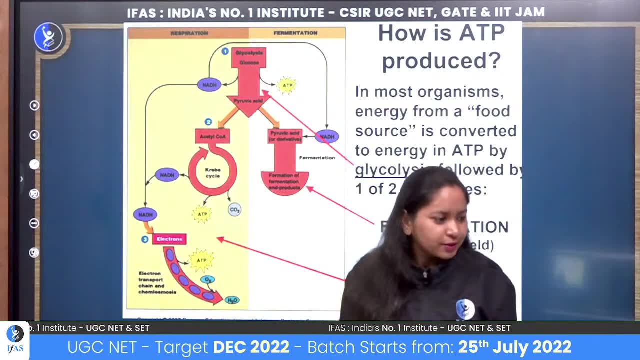 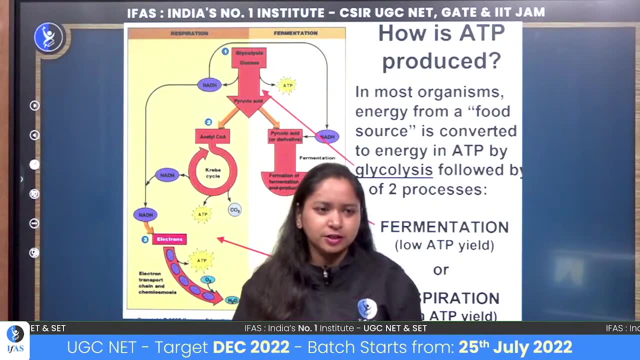 Now how exactly the ATP is produced. in case of organisms, We will talk about how exactly ATP is produced. We will discuss it as a comparison between us and the bacteria. We will like study in the form of comparison so that you remember a little bit. 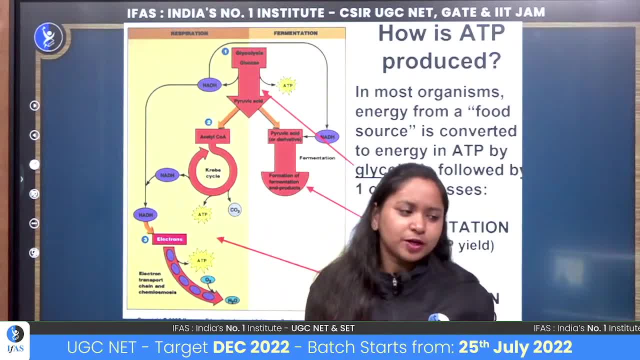 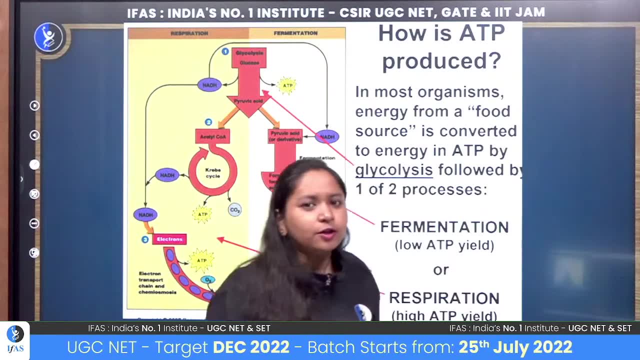 So that you can recall a little bit. Okay, we have discussed like this, So the bacteria will perform something like this. Okay, now how ATP is made in the organism. So we consume glucose. We consume glucose, we consume food in which glucose is present. 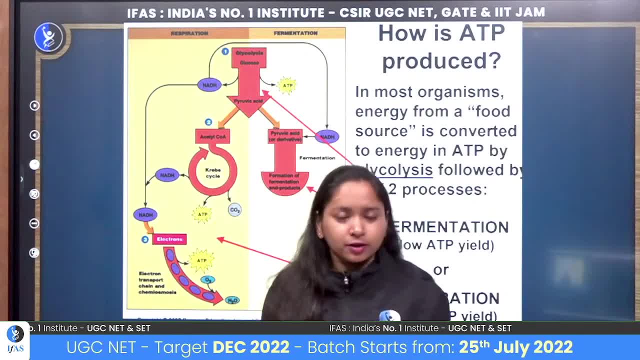 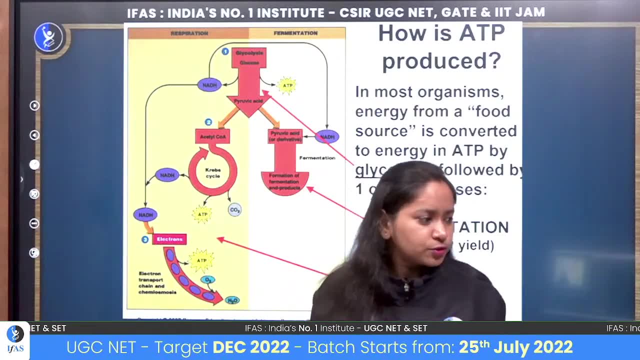 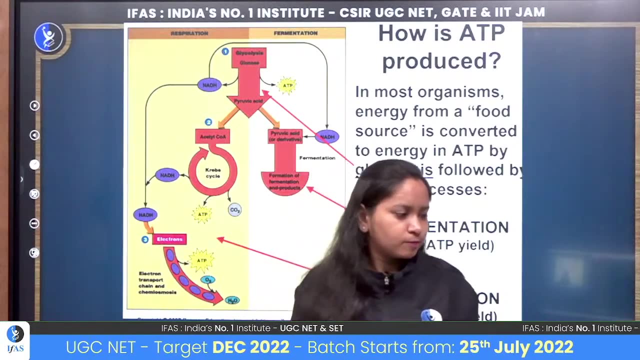 And what does the body do? The body performs a pathway to utilize that glucose. What is the pathway in which you use glucose? What is the pathway called as in which we use glucose? The pathway, yes, yes, it is glycolysis. 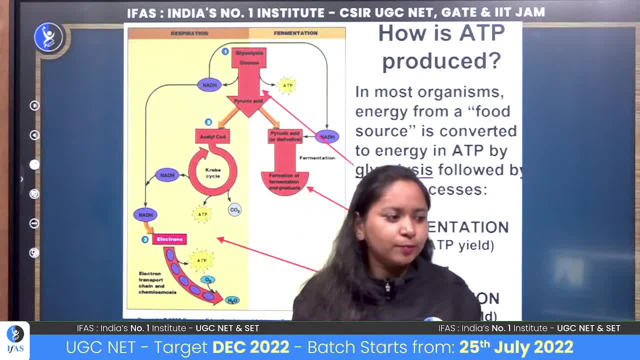 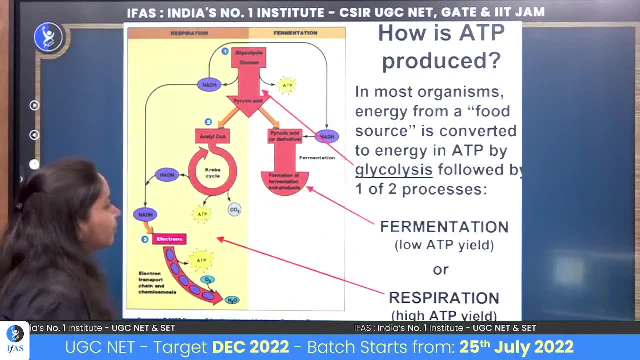 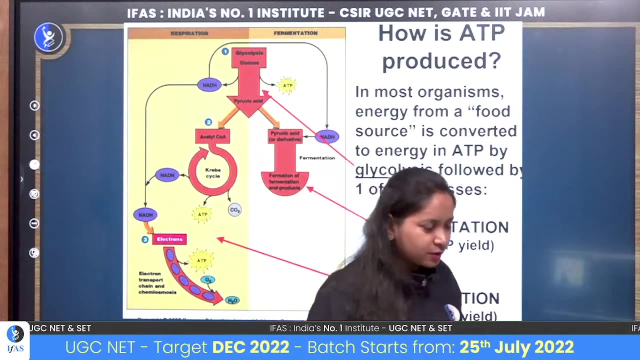 Okay, that is, we break the glucose. There is a whole pathway in which you use glucose And in the end, we are making some different products. which is your pyruvic acid? Okay, your glucose is 6 carbon. pyruvic acid is your 3 carbon product. 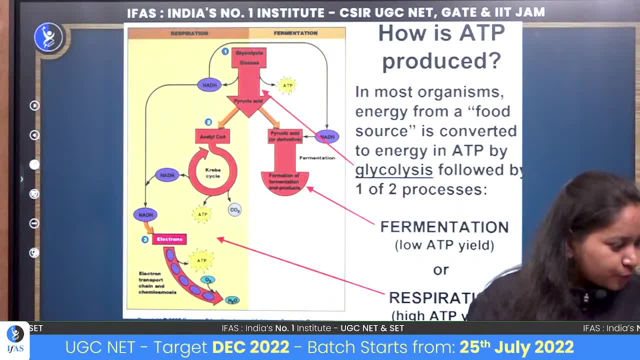 Okay, yes, Samad Vagdevi Param Shubhi Anamika Hridhiksha. Yes, you all are right here. kid. Yes, pyruvate will be made in your end. 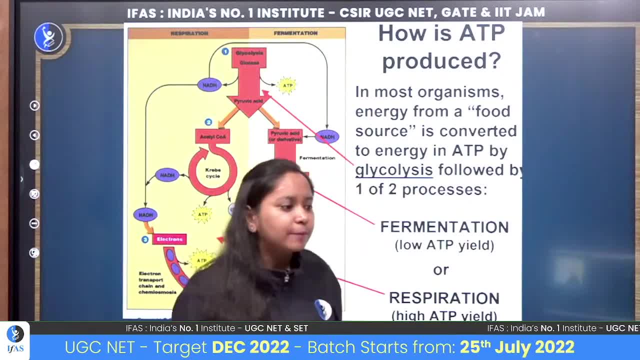 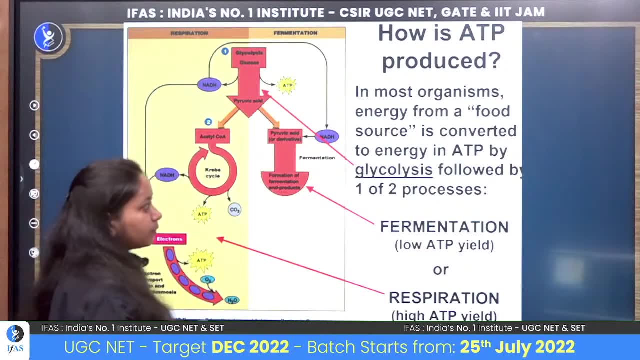 That is, glucose is converted to pyruvate. Okay, Yes, it is a 3 carbon substance. What is pyruvate? It is a 3 carbon substance. It will be a substrate. Okay, So what is happening here? 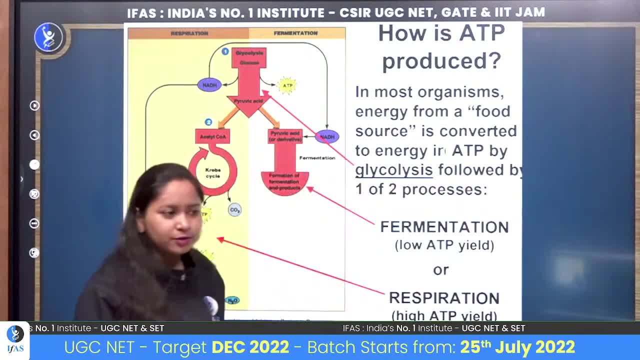 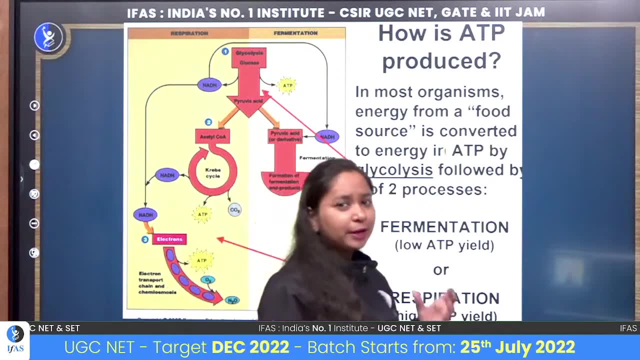 What is happening in this? Energy is generated by the process of glycolysis. What happens after glycolysis? What is pyruvate? We have to fix it At the end, When pyruvate is made. we have to fix pyruvate after that. 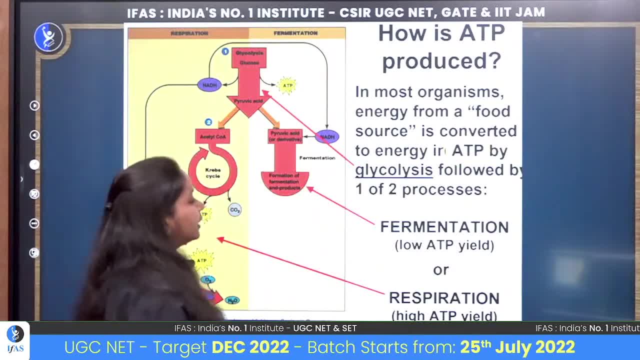 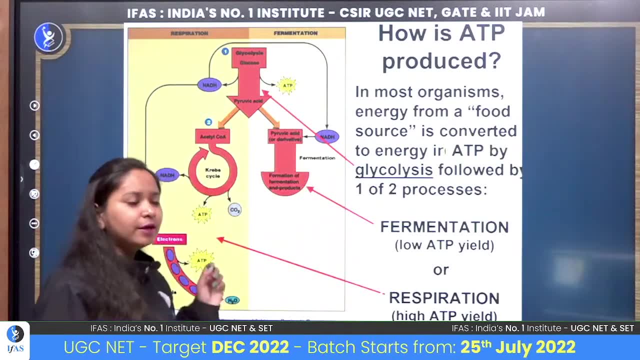 And how do we do that? So that can be done by two pathways. One is: either you can do fermentation or you can do respiration. Okay, If an organism is aerobic species, If the organism is aerobic, then it uses respiration. 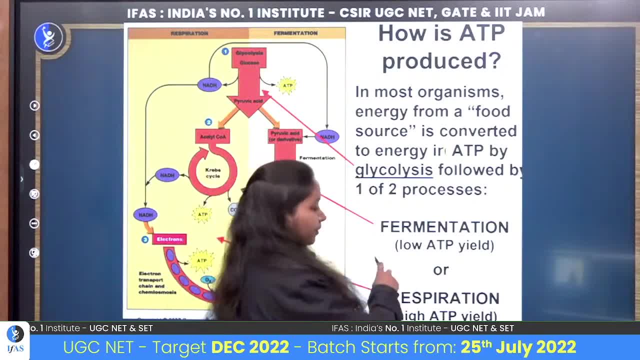 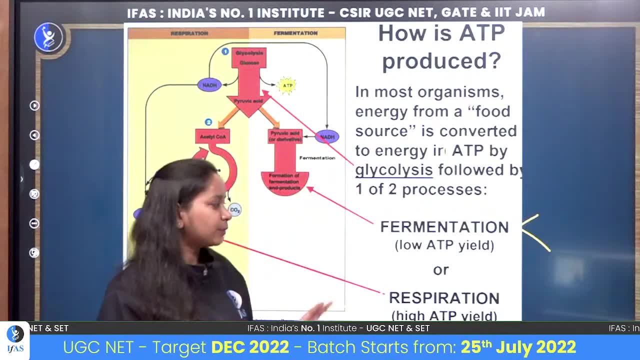 If the organism is anaerobic, then it uses your fermentation. There are two more in this We will discuss. There is lactic acid, There is acetic acid fermentation. There are two types of fermentation here, And your one is respiration. 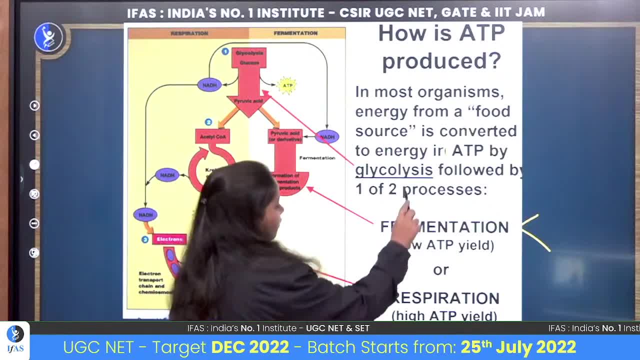 Which performs your aerobic species. Okay, Tell me, Do we make lactic acid in the body By this fermentation or by this anaerobic respiration process? Do we make lactic acid By this anaerobic respiration process? Is it possible? 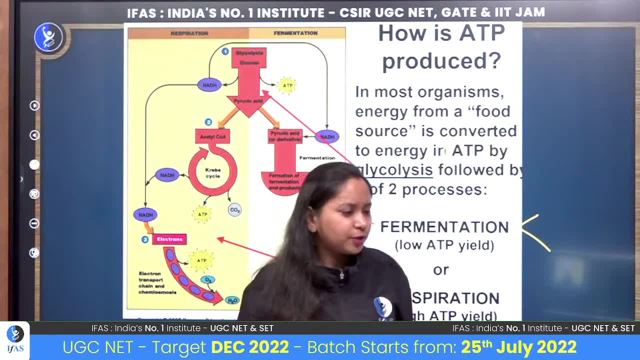 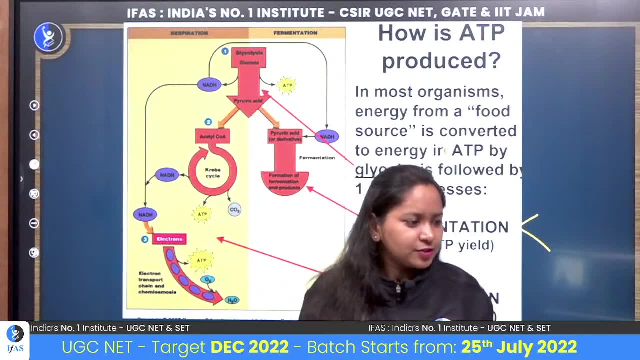 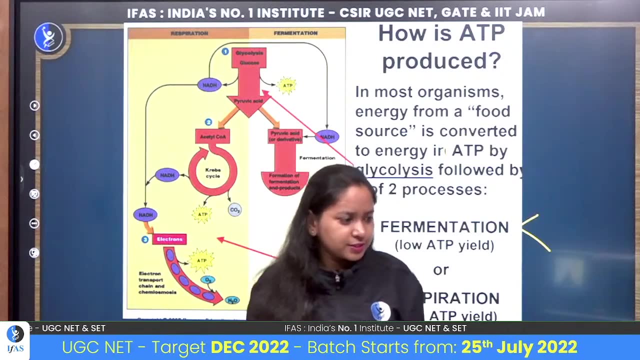 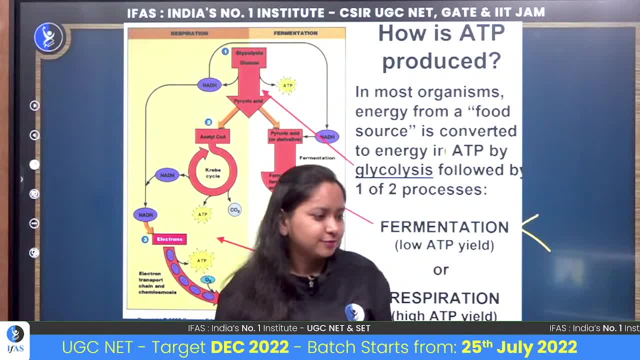 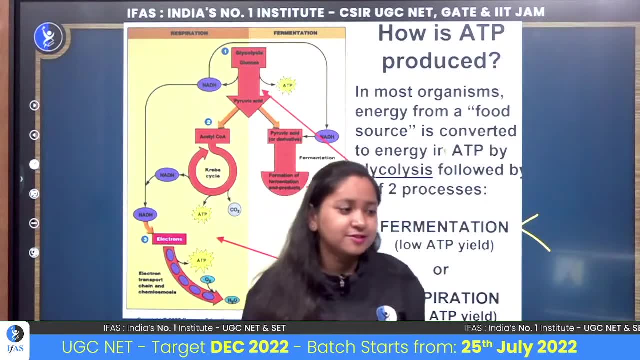 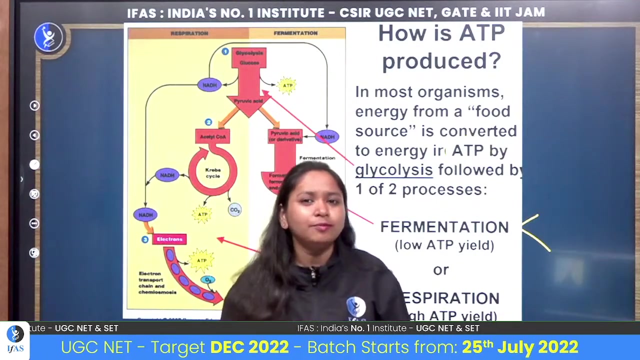 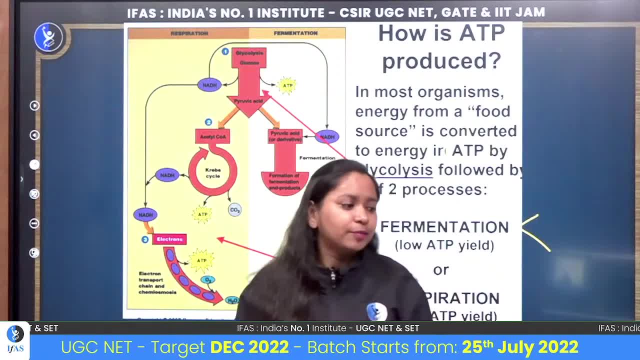 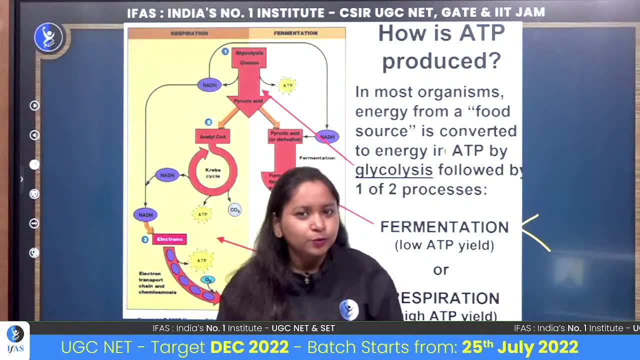 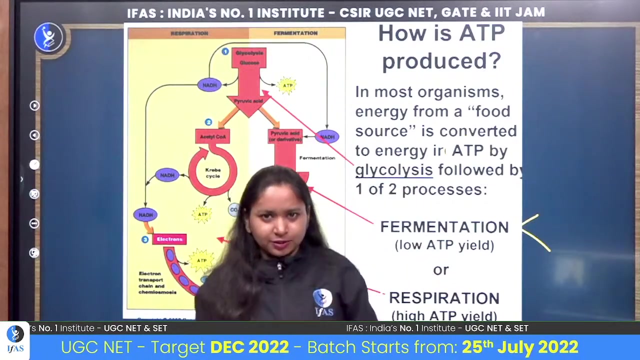 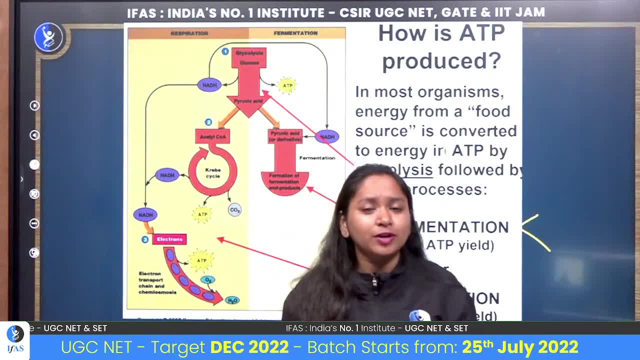 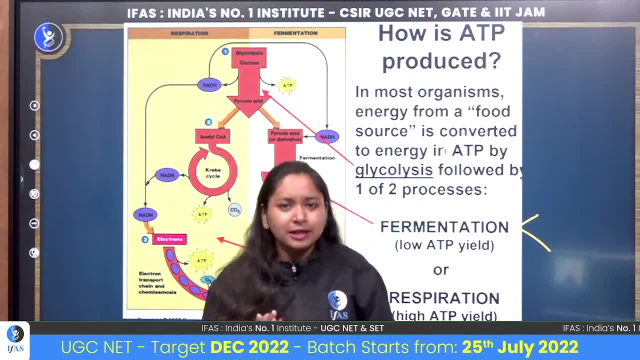 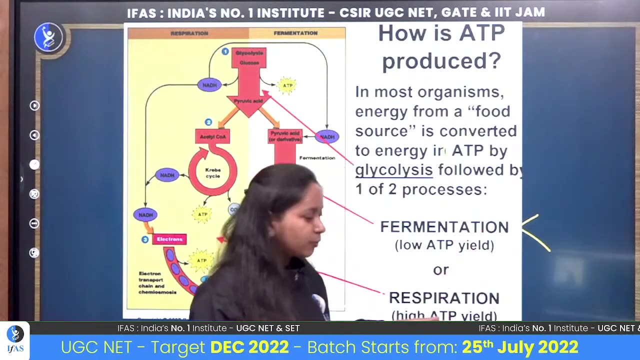 Okay, Okay, In that case, what will happen is that your body starts a different pathway. It performs anaerobic respiration, but the end product is lactic acid. We will not make ethanol, we only form lactic acid. One is alcoholic fermentation and the other is lactic acid fermentation. 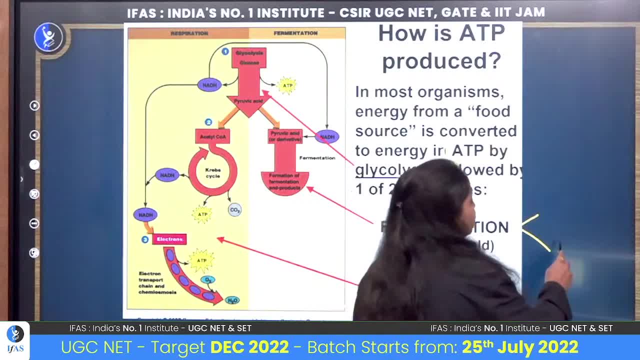 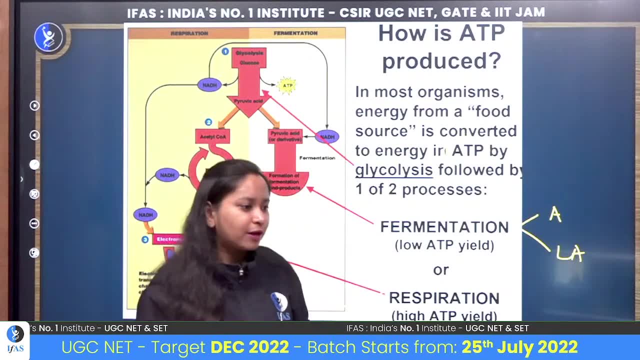 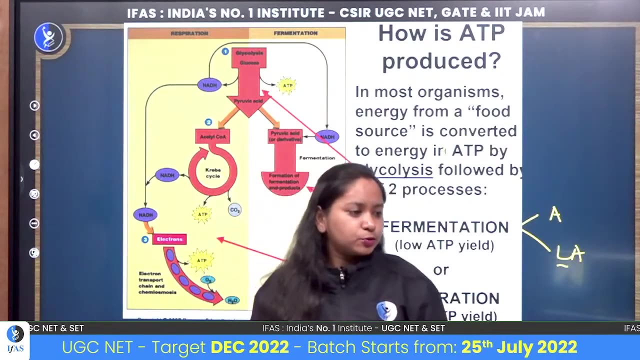 We do not do alcohol, we only do lactic acid fermentation. We do not do alcoholic fermentation, we only do bacteria fermentation. Those are used for the production of alcohol as well. We will discuss that later. We can make lactic acid, but that will now lead to the muscle cramps. 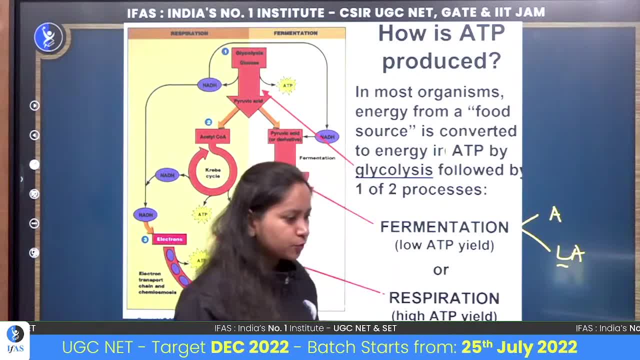 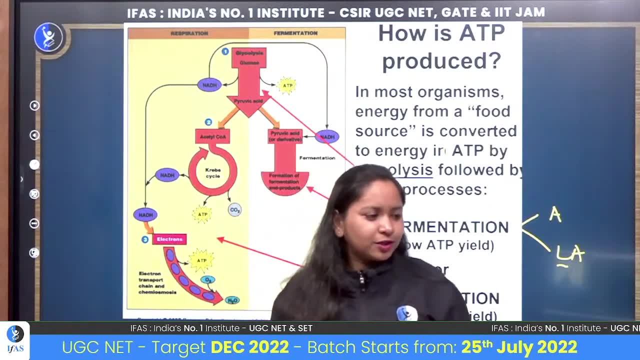 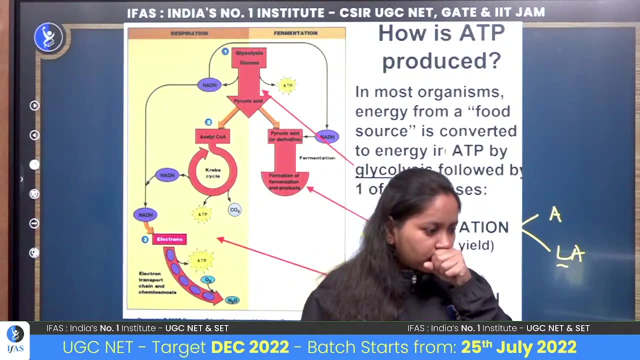 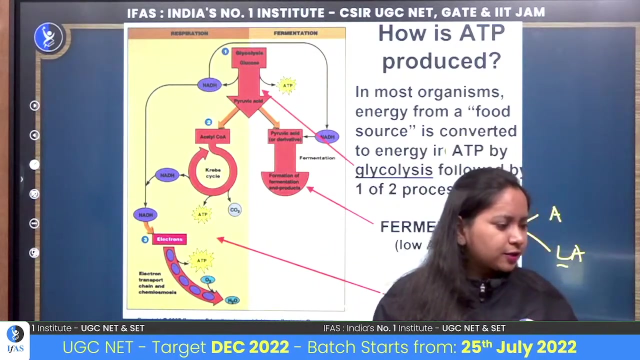 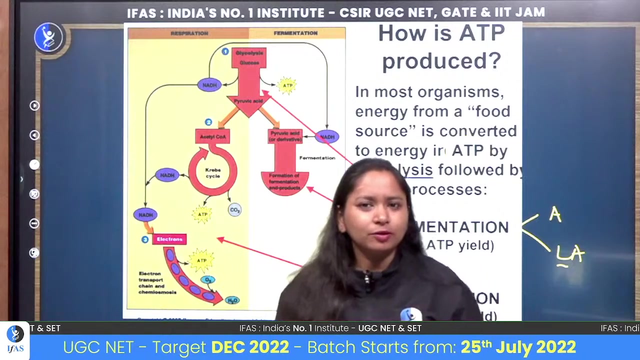 which we have a lot of pain after the exercise. If you have done something after a long time, if you are working out or if you have gone for trekking, if you have walked a lot, then it also happens. What happens in your body is that you are breathing. 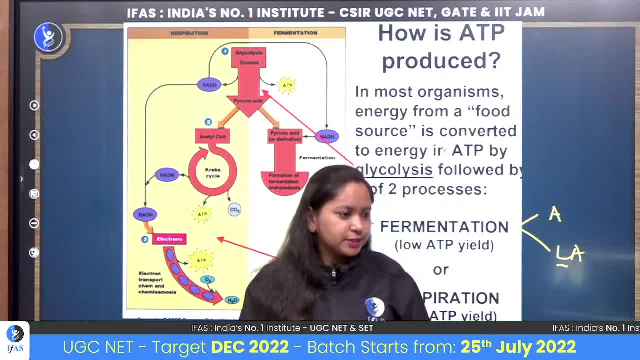 but your oxygen demand does not fulfill. You are breathing. what is happening? by breathing, Hemoglobin is also transferring oxygen to the whole body. Lactic acid- sorry, myoglobin- is also holding the oxygen in the muscles, but when it is reserved, that reserve ends. So actually they are not responsible because your demand increases so much that your body is not able to fulfill that demand. All these things start because of this. It is not like that your RBCs have decreased. your hemoglobin has decreased. no, it does not decrease. 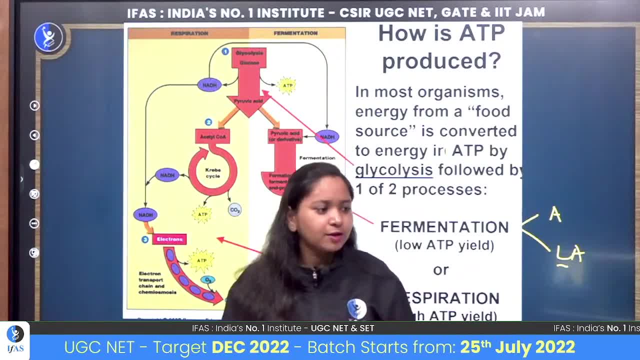 but your demand suddenly increases. Okay, so it is not like: suppose you have four rooms in your house and you live with four people at home, then four rooms are sufficient for four people. But if ten people come to your house, then what will happen now? 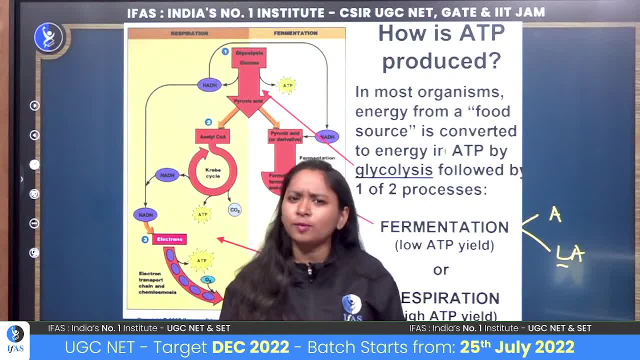 The demand has increased. right, It is not that your house is small. your house is sufficient for four people. as much as you had to live there. it was sufficient for that. But because the demand increases, suddenly, because of this our house will start looking smaller. 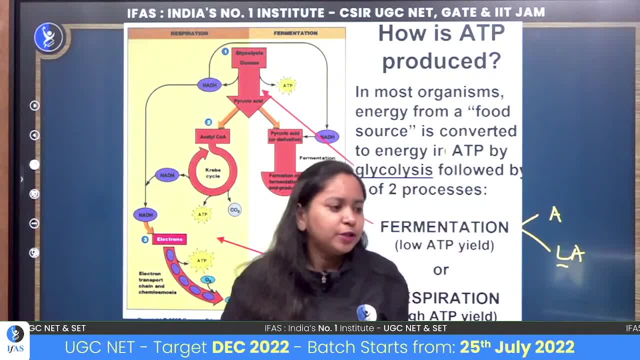 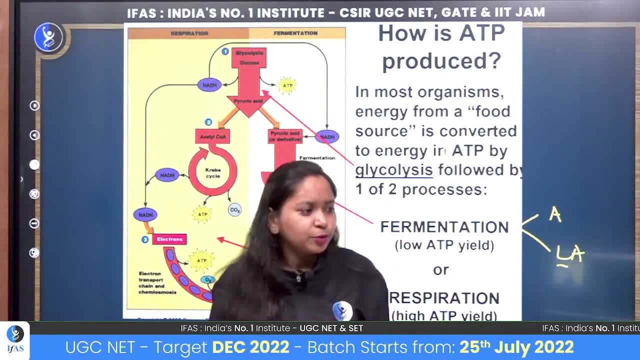 Okay. What is the difference between myoglobin and hemoglobin? Come on, tell me What is the difference between hemoglobin and myoglobin, What is hemoglobin and what is myoglobin? Guys, please share the session as well. Call all your friends. 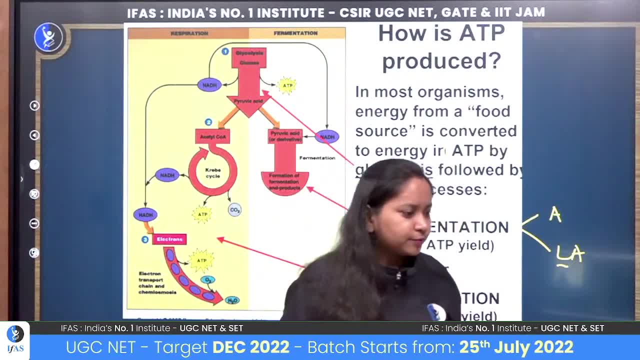 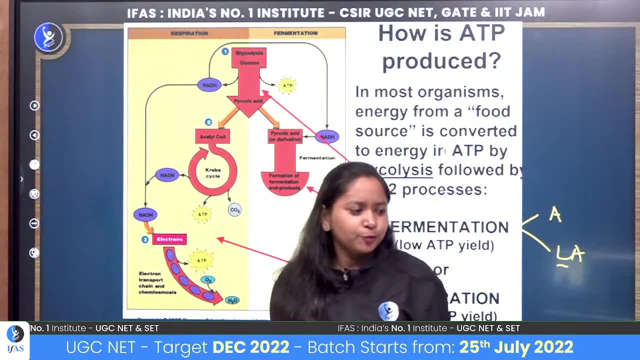 What is the difference between hemoglobin and myoglobin? Good morning Ishika. How are you? What is the difference between hemoglobin and myoglobin? Okay, What is the difference between myoglobin and myoglobin? There is a difference between polypeptide. 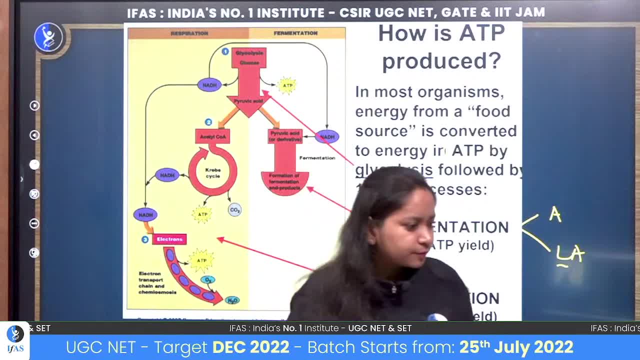 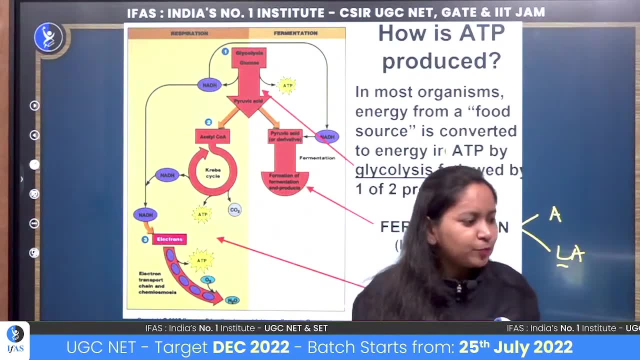 Okay, Param. How much is there in this? Okay, That's very good, Samath. Myoglobin is tertiary. Hemoglobin is quaternary, Very good. Myoglobin stores oxygen. Hemoglobin carries oxygen. Yes, I am also good, Ishika. 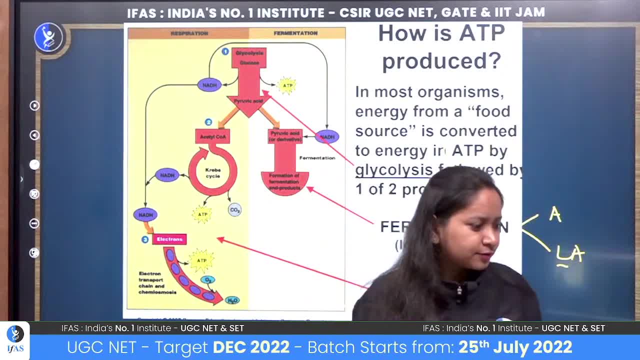 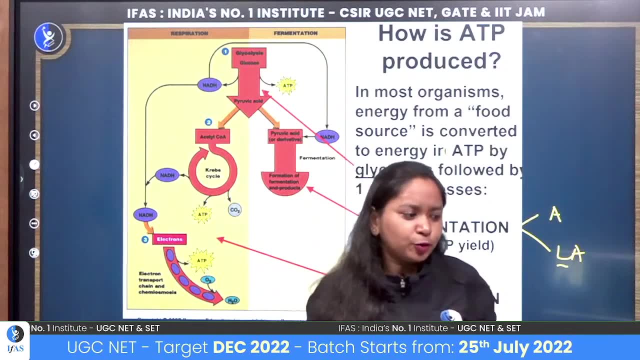 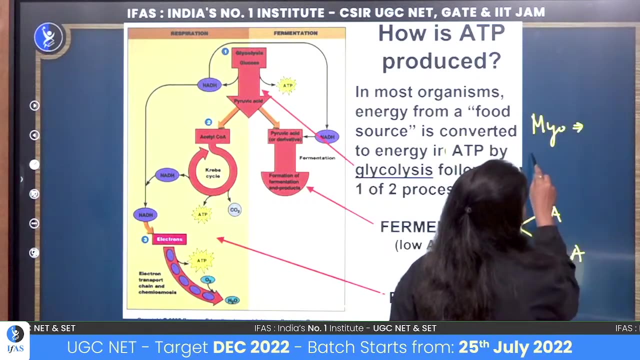 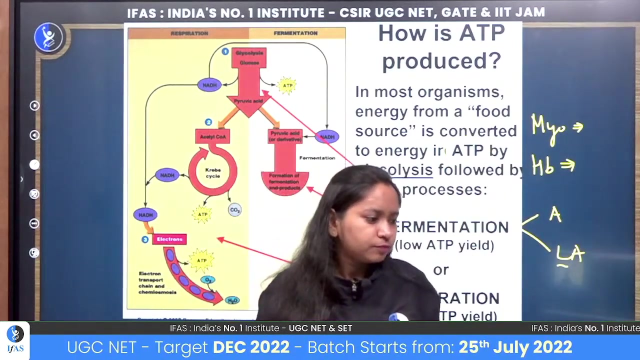 Thanks for asking. Okay, Yes, Yes, You all are right here. How much monomers are there in myoglobin? How many monomers are there in hemoglobin? How many subunits are there in myoglobin and how many subunits are there in hemoglobin? 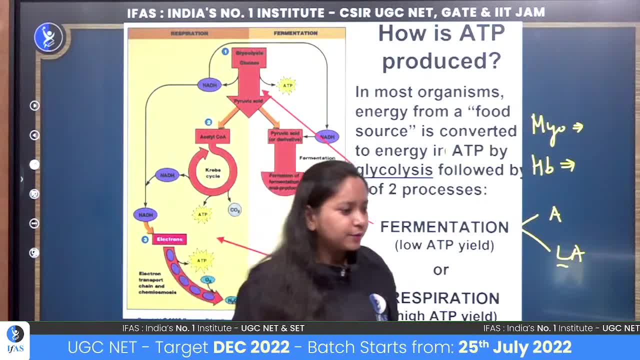 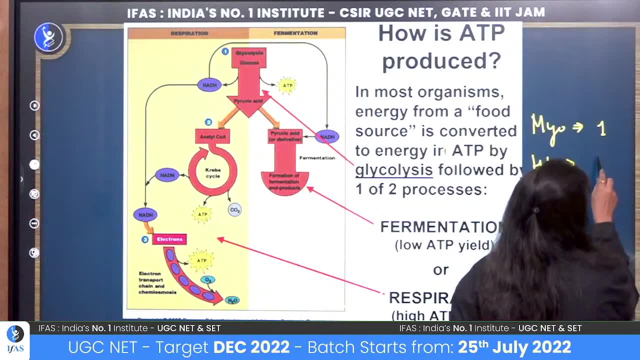 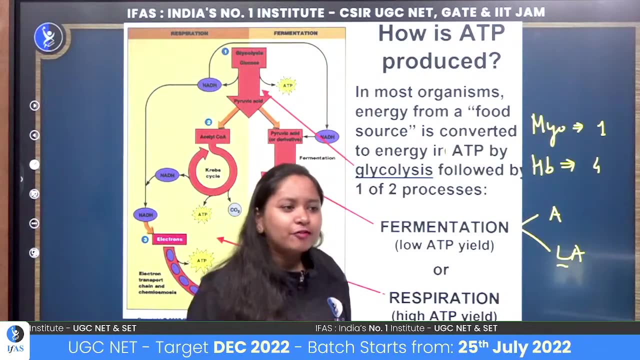 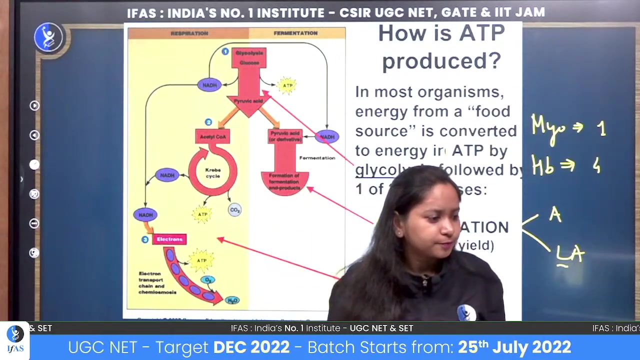 Shikha is saying that myoglobin carries one molecule of oxygen. What about hemoglobin? It carries four. Which of these have higher affinity for oxygen, Myoglobin or Hemoglobin? Yes, Hridhiksha, Myoglobin is present in muscles and they only store oxygen. 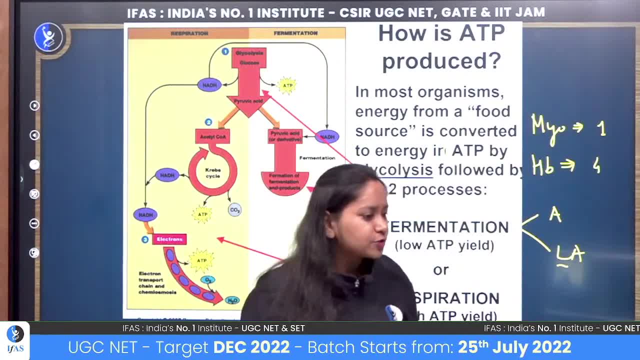 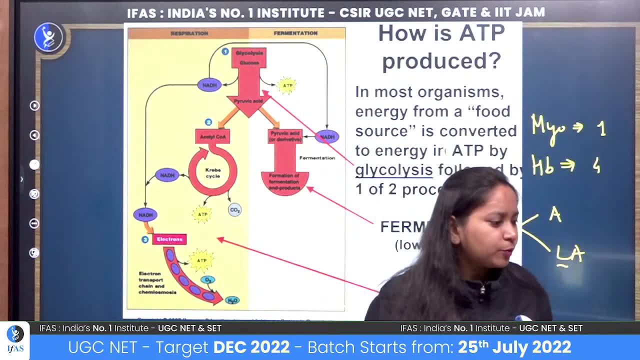 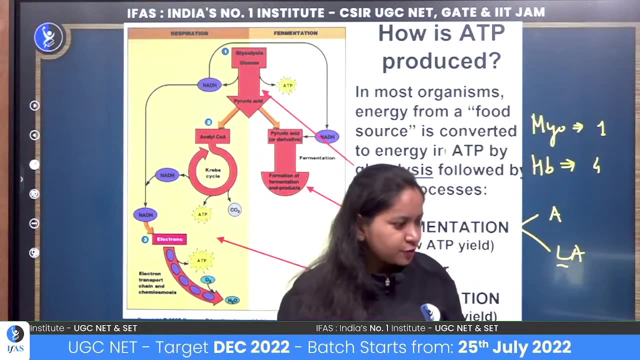 And RBCs carry oxygen to all the body parts. Myoglobin has more affinity or Hemoglobin has more affinity? Shikha is saying that Myoglobin has more affinity. Rest Param, Samad, Jhanvi, Vagdeva Namikasa. Hemoglobin has more affinity. 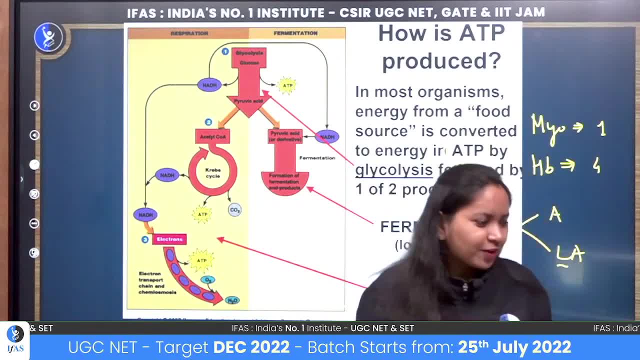 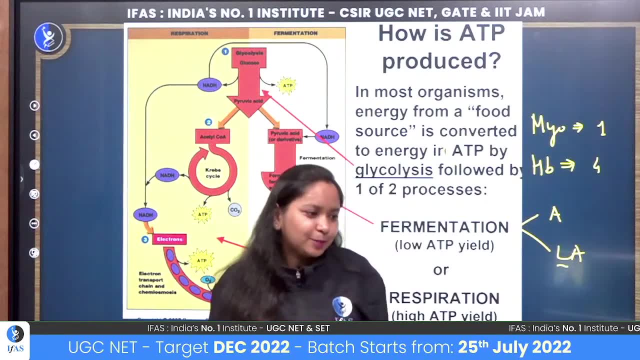 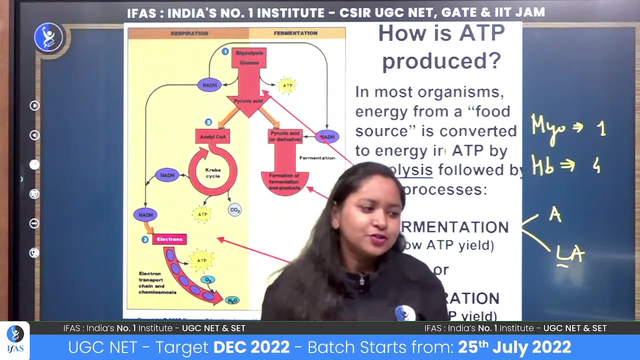 Shikha is again saying Mayo, Hridhiksha is saying Mayo. So let's see, Yes, Okay, tell me. Suppose you have one chocolate And one more And you have four chocolates, Who will give his chocolate easily? 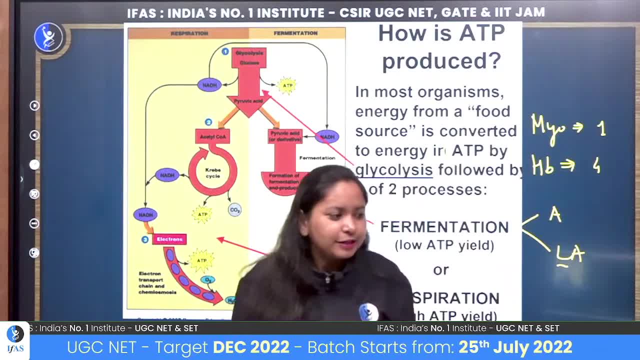 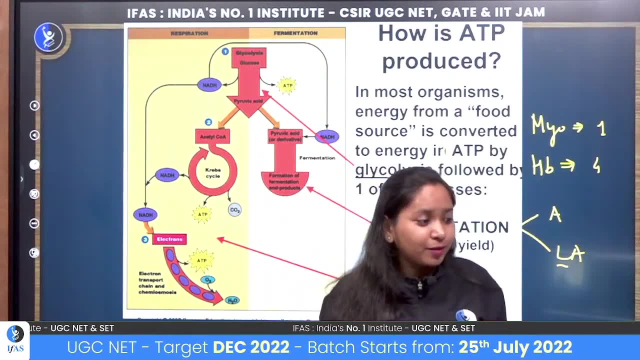 Four or one. Good morning Rishi. If you have one chocolate and one person has four chocolates, Who will give his chocolate? easily, By the way, no one will give, But still, If we make a comparison between the two, Who will have four chocolates? 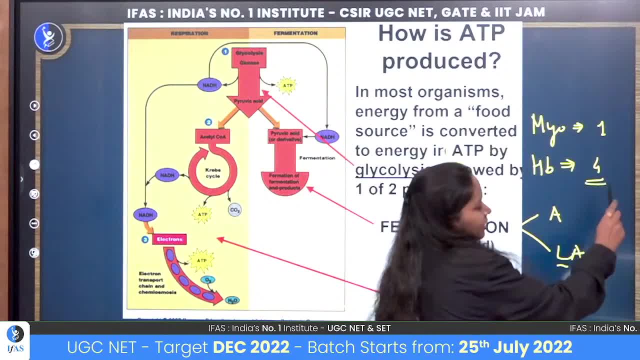 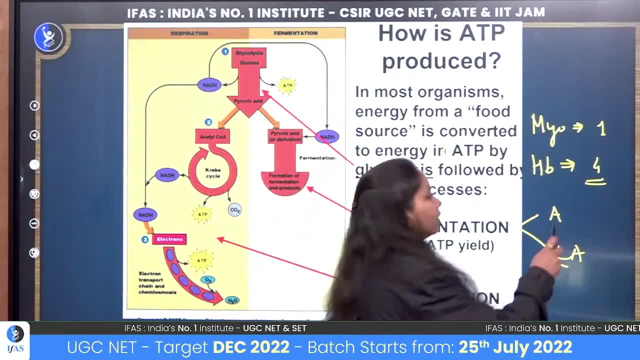 Right, Hemoglobin has four oxygen. As you always remember, It has four oxygens, Four oxygen is there. So that's why you remember Hemoglobin will give its oxygen very easily Because it has four oxygens. This is just to remember. 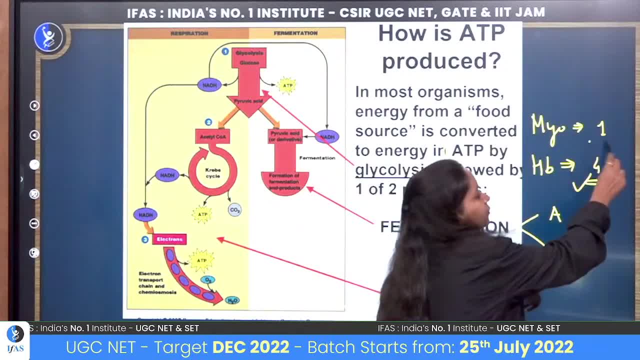 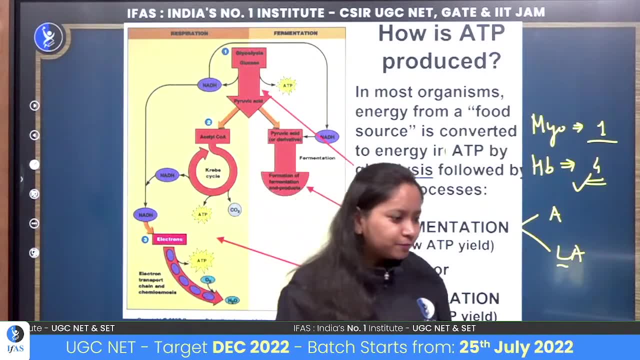 I will explain you the logic. Myoglobin has only one oxygen. It never leaves it. It holds it When the condition is very extreme. In that condition only Yes, it was a matter of giving, It was not a matter of taking. 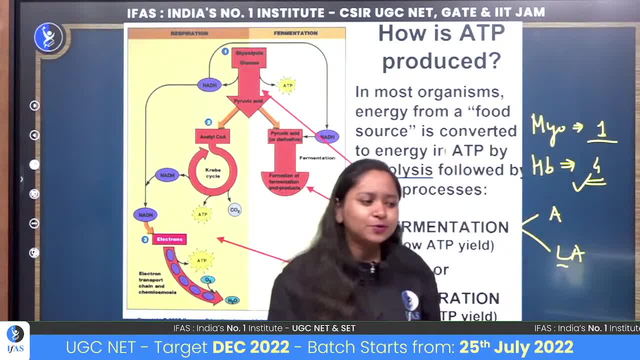 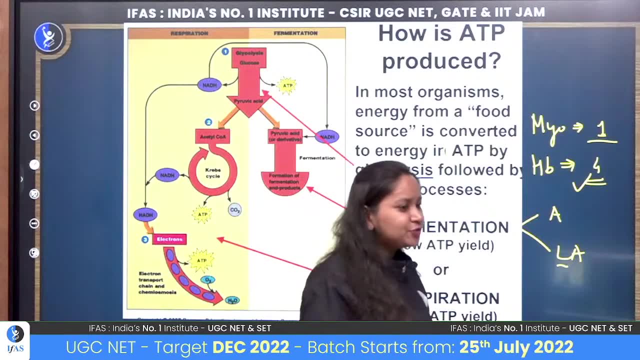 If someone has one oxygen, Then he does not easily donate it. Okay, So your myoglobins? They have a very high affinity for the oxygen. See, Imagine If the hemoglobin has a very high affinity for oxygen. Imagine: 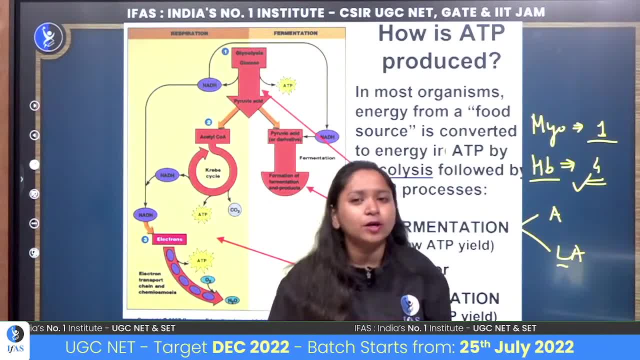 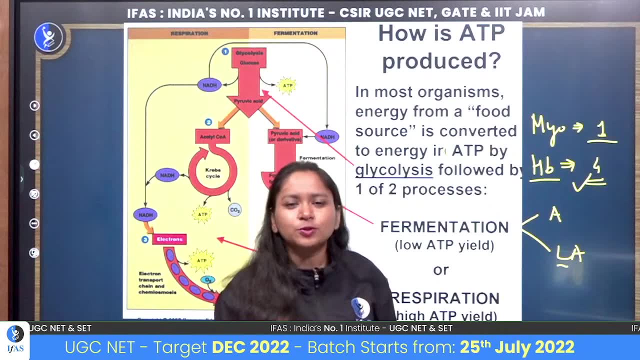 If the hemoglobin binds your oxygen very tightly, It does not release it. Then what will happen? Brother, The work of the hemoglobin is to donate oxygen. while walking, It has a normal job: To donate oxygen to each and every cell of the body. 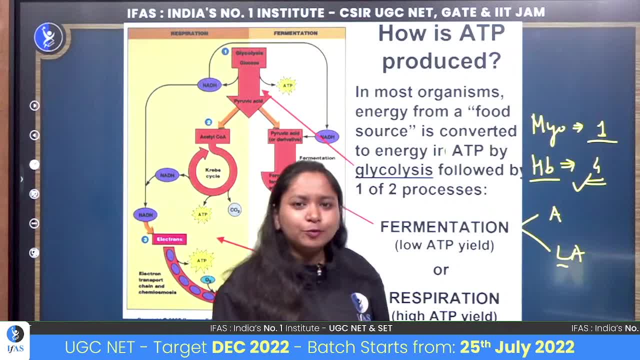 So why will it keep the affinity more? If the hemoglobin keeps a very high affinity for oxygen, Then what will it do? It will not be able to give oxygen to anyone. It will not give oxygen to any cell. It will not say that I will hold it. 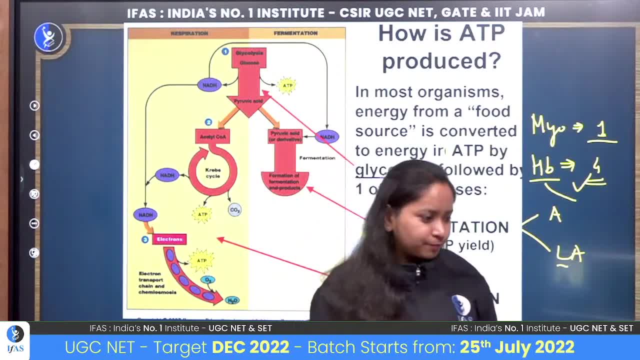 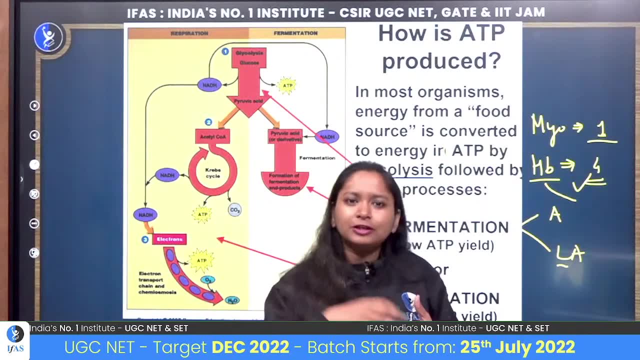 It will stay with me. It will stay with me. So its function is not happening here, Is it not? There will be a problem in transport, Yes or no? So its job is to transport oxygen, So it takes oxygen very easily. 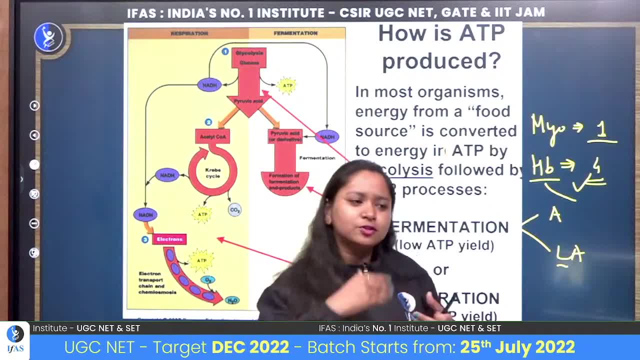 It also donates it Because its job is to take oxygen, Go and give it to someone else, Okay. So that's why Hemoglobin has less affinity for oxygen compared to myoglobin. I am talking about compared to myoglobin. 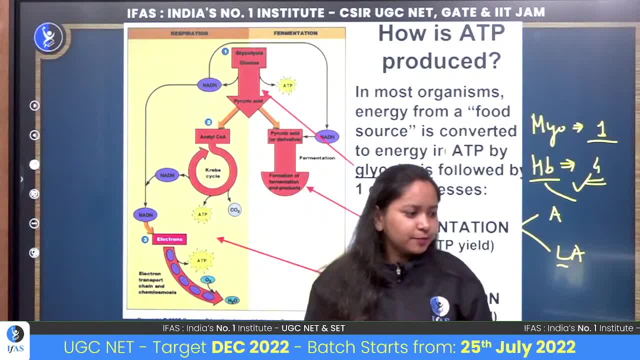 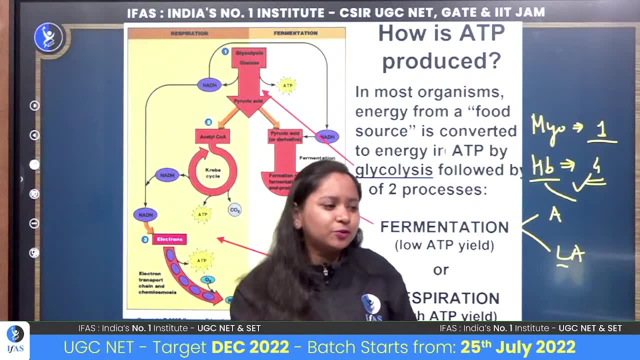 Is it clear to everyone. There were some wrong answers here. Is it clear now to everyone? Keep in mind: One chocolate, four chocolates. One will not give easily Four. Okay, Give one. I have three left, Like that you can remember it. 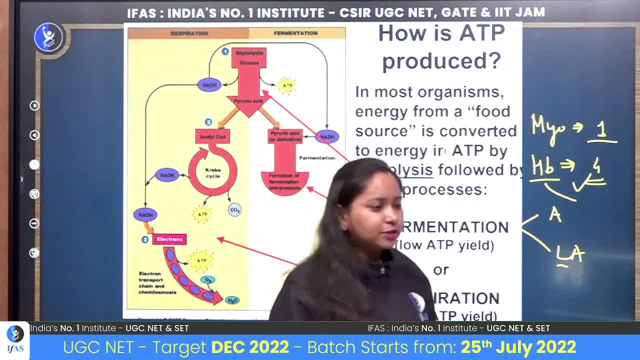 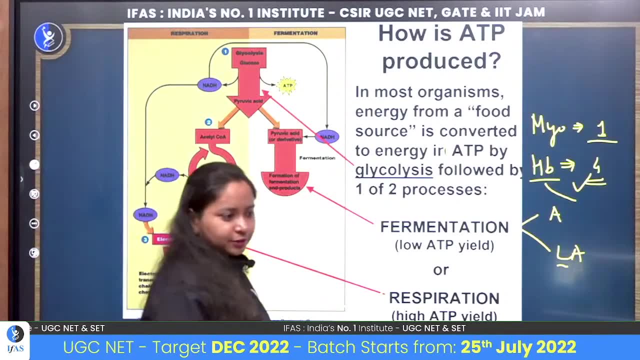 Okay, Many people get confused. This is very important. Since you brought the names, I explained this as well. Okay, Let's go. So, yes, We were talking about the fermentation. We were talking about. Good morning Arjun. 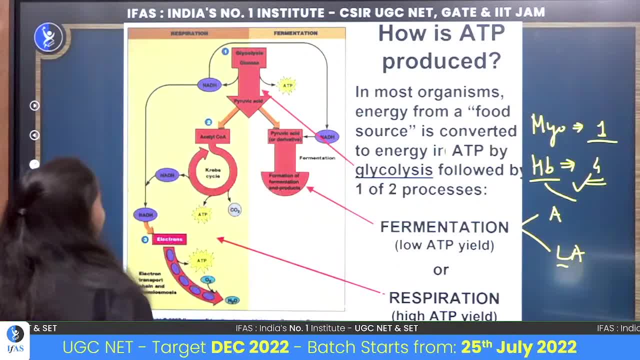 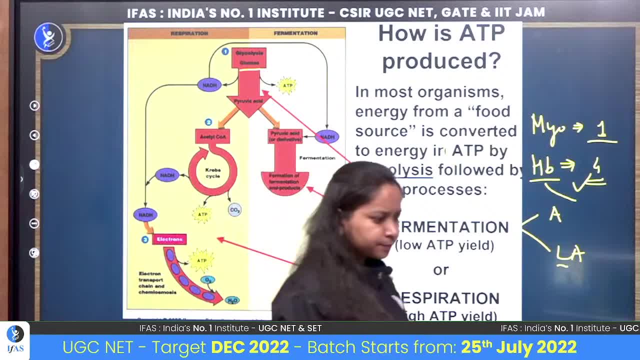 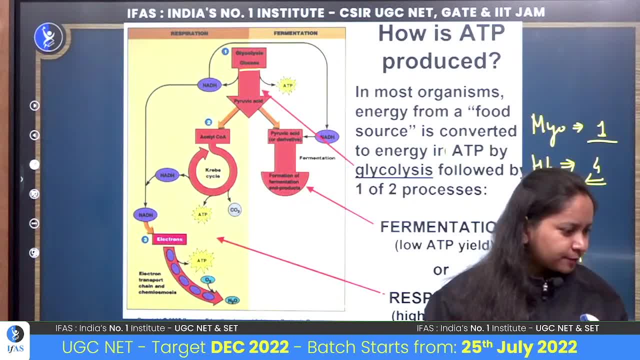 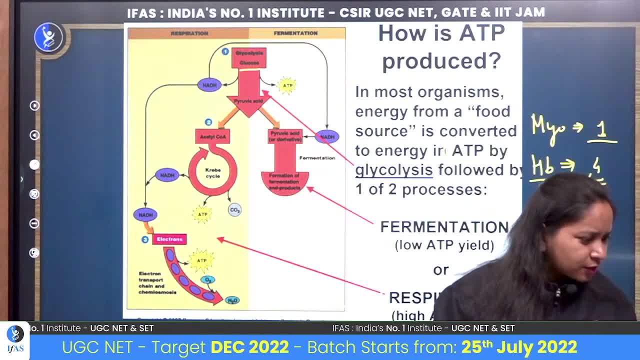 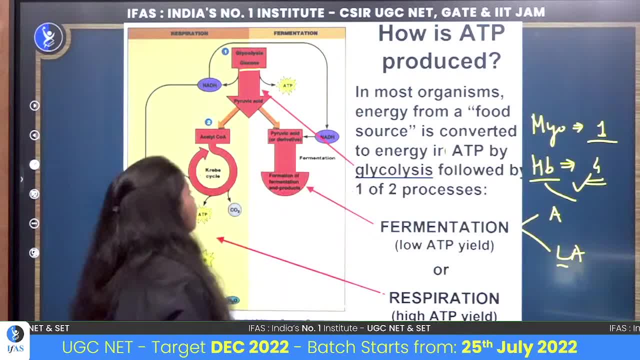 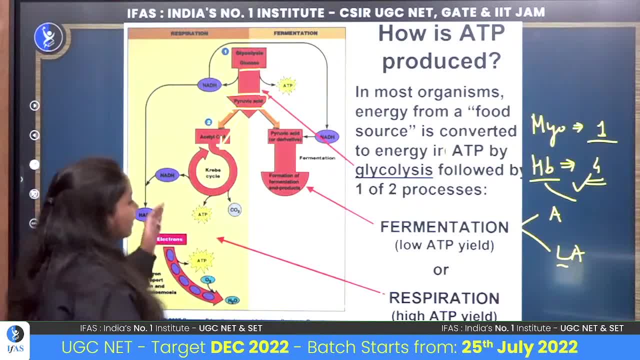 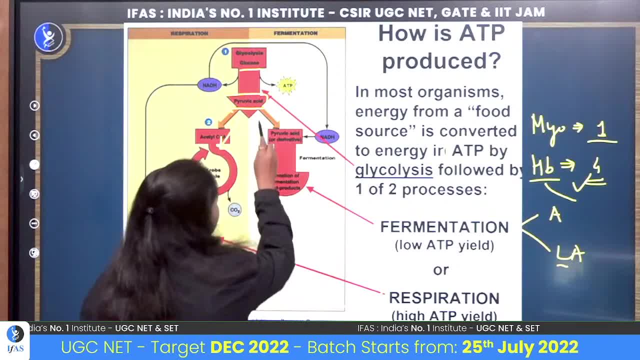 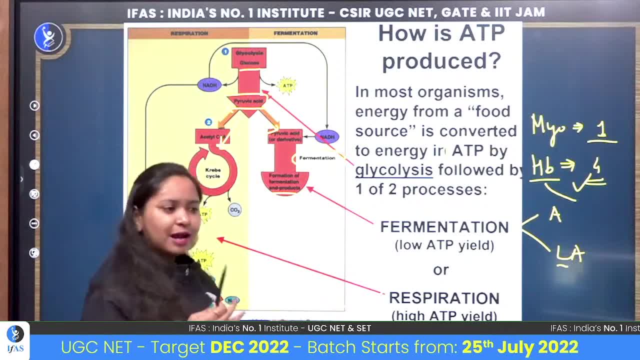 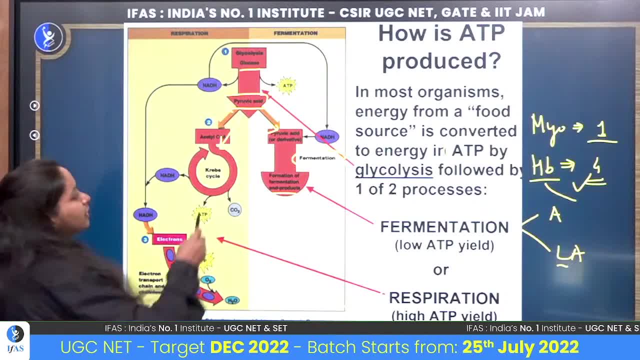 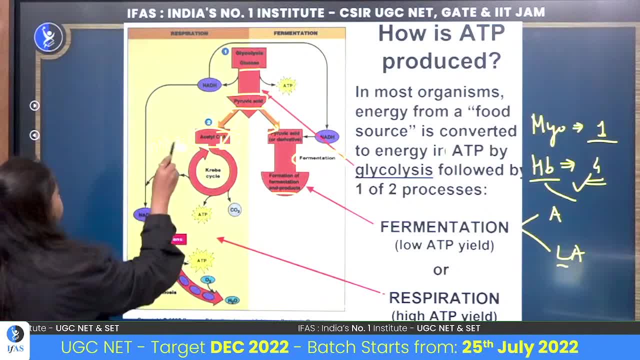 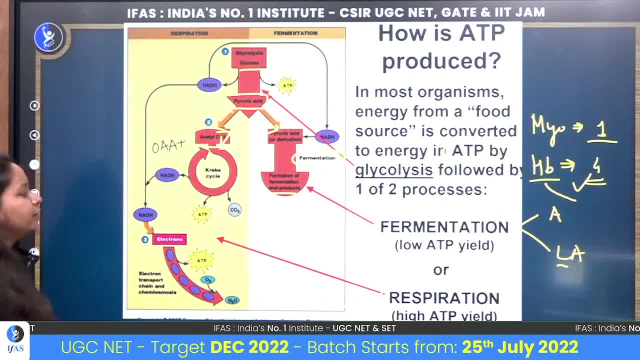 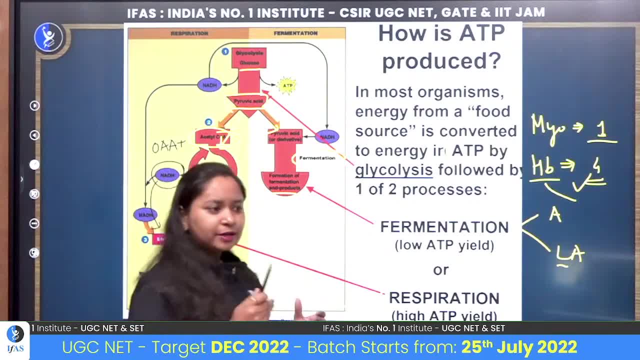 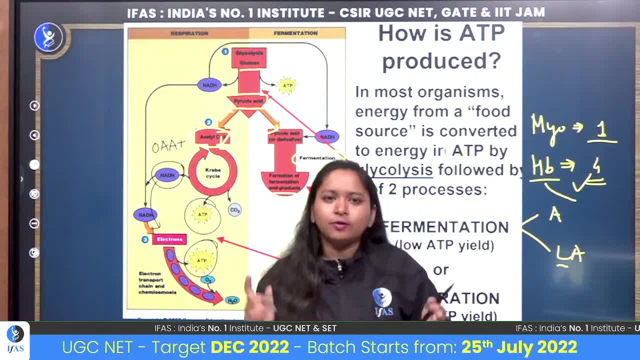 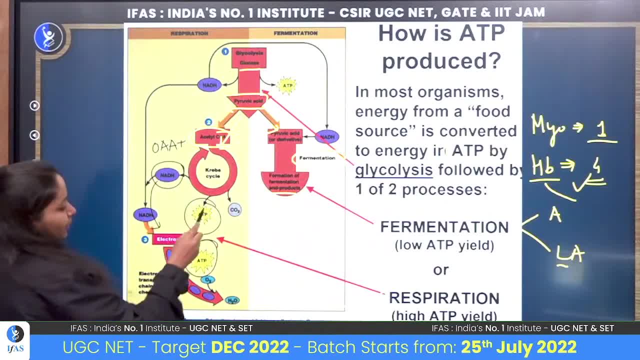 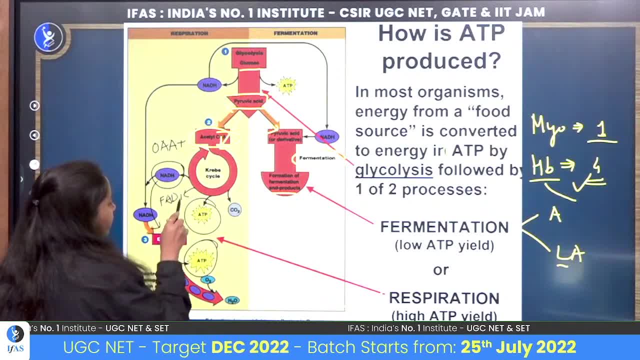 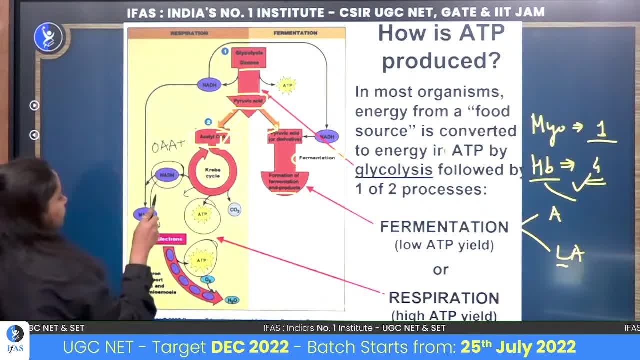 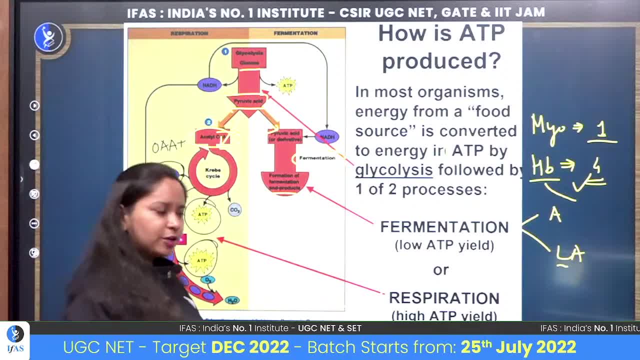 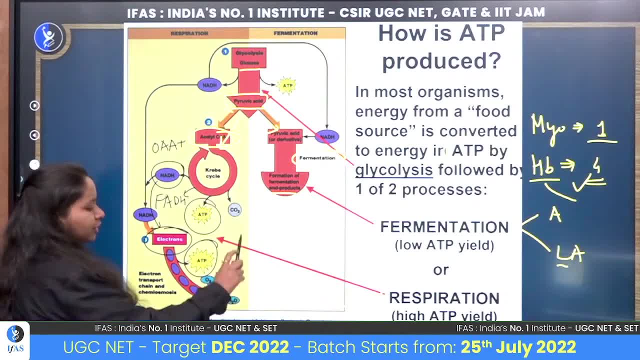 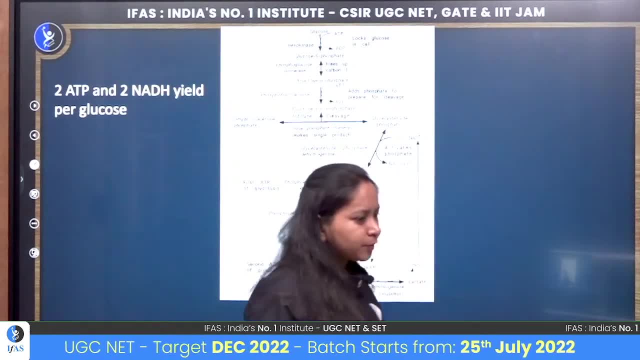 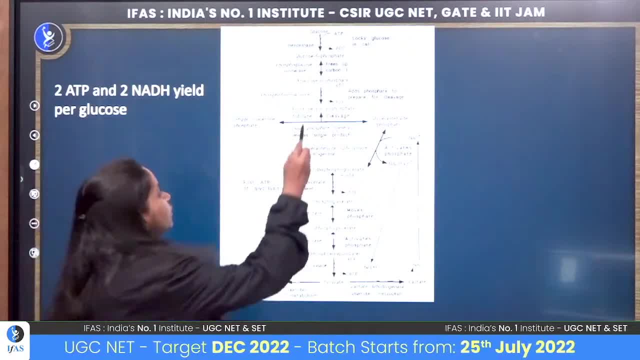 Your End Result will be: lado, saggy skin is visible and ie? Which your Glucose. it will get converted to pyruvate. it gets converted to Pyruvate. Which your Glucose- it will get converted to Pyruvate. 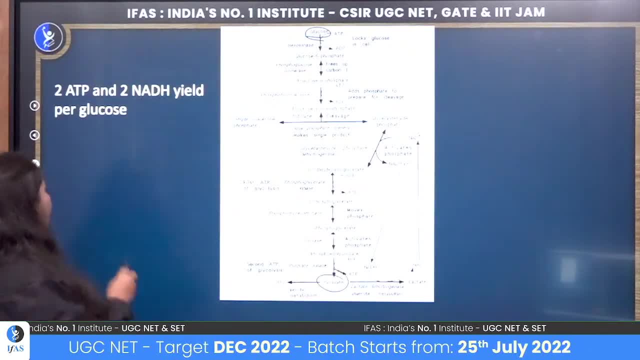 which your Glucose, it will get converted to Pyruvate. Which your Glycolysis, it will get converted to Pyruvate. If your Condition where the diagram is not clear, it's okay for this part, As the rest of the Diagrams you can understand. 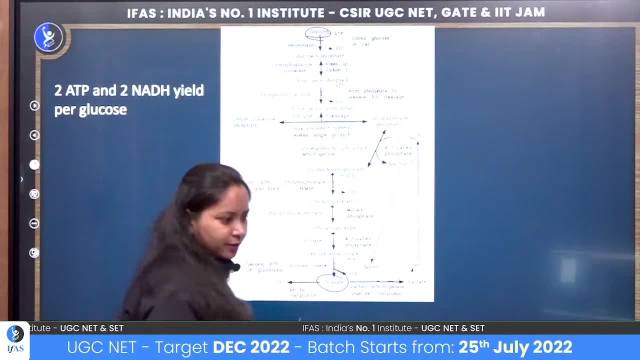 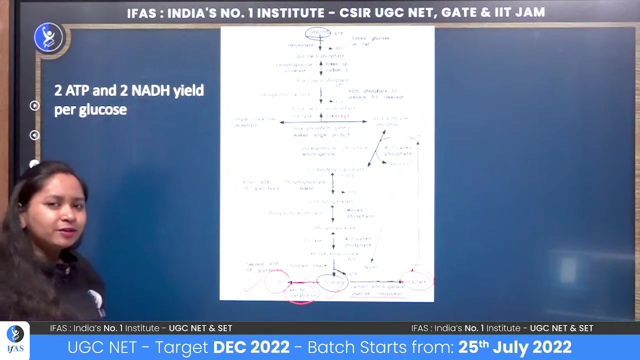 In the end of Pyruvate. if the Condition is Anaerobic, it will create Lactate or Acid. it's okay for this part. we will understand the rest of the diagrams. okay, pyruvate is formed at the end. if the condition is anaerobic, then your lactate is formed at the end, or alcohol will be formed. ethanol will be formed. if the condition is aerobic, then it is used in your aerobic respiration and in the end it is formed. then it is released in the form of carbon dioxide and whatever your end result is, whatever energy molecules we get from here, there is yield of 2 ATP and 2 NAD. 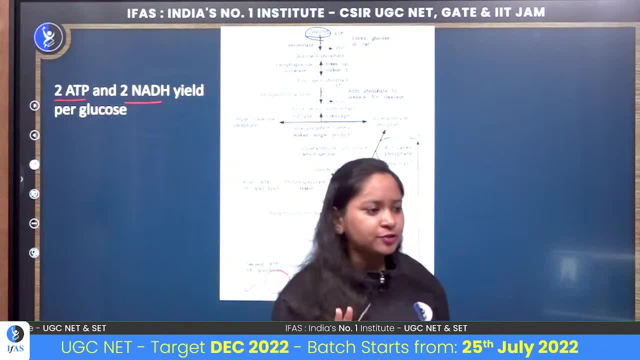 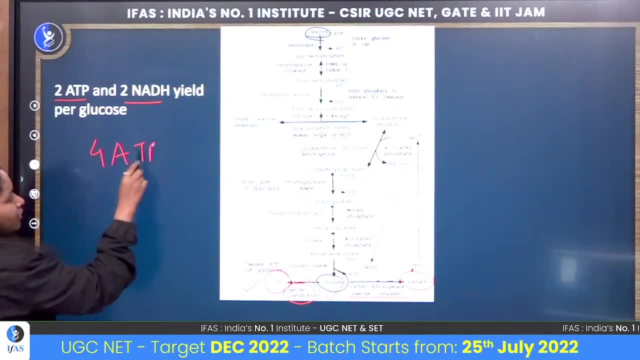 Okay, we make here 2 ATP and 2 NADH, we get yield. it happens that here 4 ATP are formed, 4 ATP are synthesized, from which what happens? then we use 2 ATP. 2 ATP are used. so that's why, if we talk about your net gain, then that is your 2 ATP. your net gain here is 2 ATP. 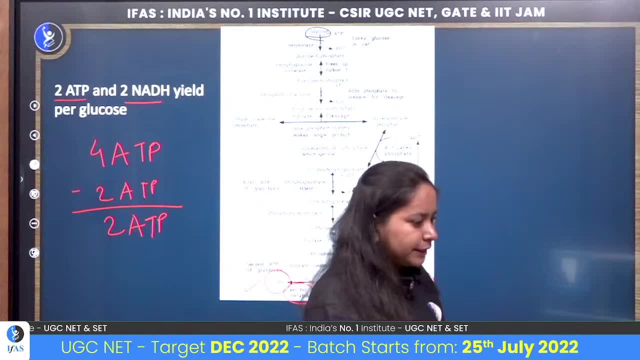 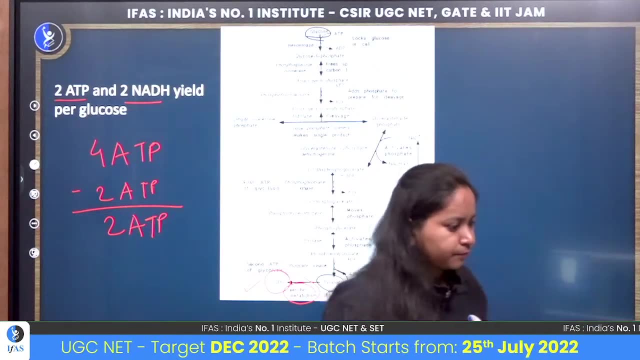 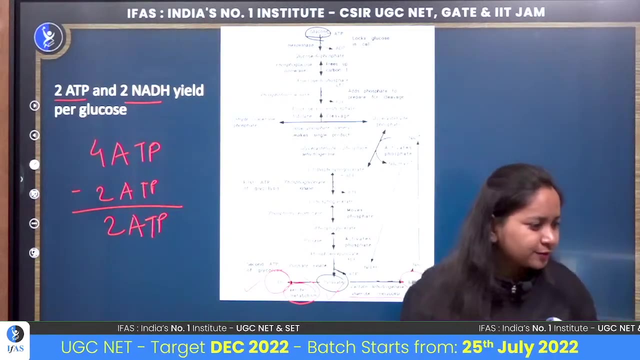 Okay, so we are talking about ED pathway enter deodorant pathway? I am not very sure about it. I will check it for you later on, but at the end of the session I will confirm it for you. okay, Hello, you are Veeru. you are okay. 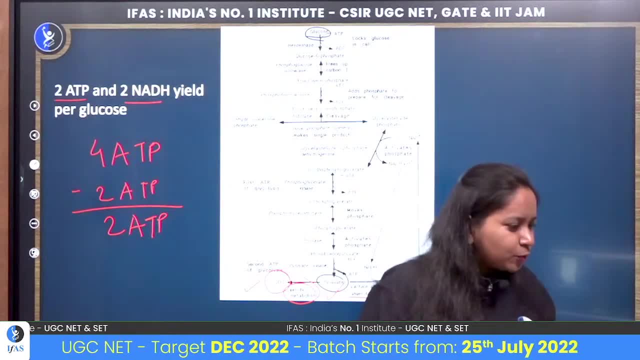 What is your QST? are you asking some question? yes, you can ask your question. I think it must have gone up. I didn't see that. can you please post it again? I didn't see your question. please post the question again. 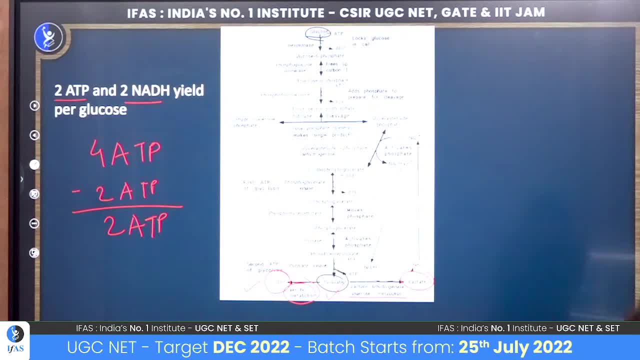 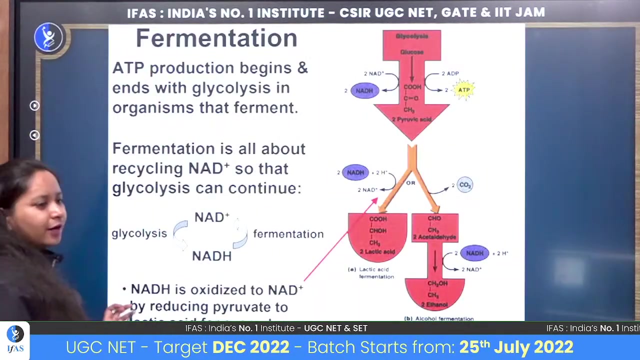 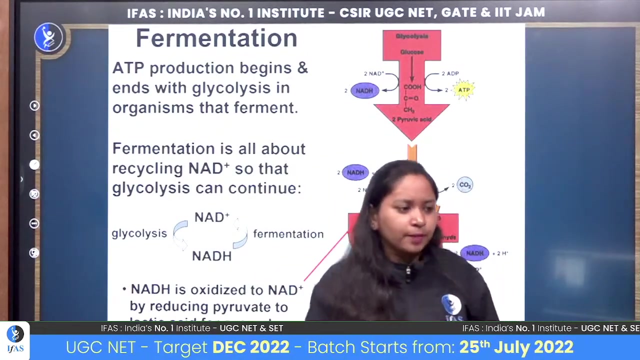 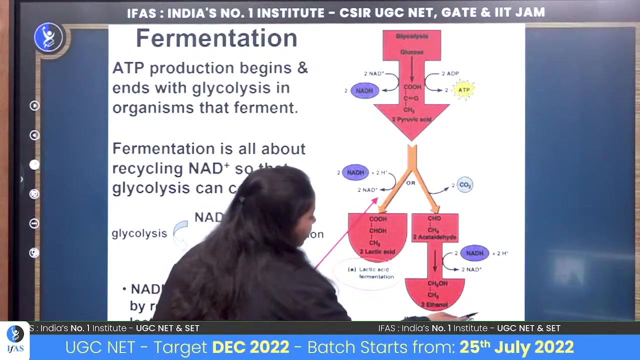 One second. I didn't see that. please post your query. okay, once again, I will answer that as well. So, yes, this is your glycolysis. after this, what happens if the organism is anaerobic? okay, if the organism is anaerobic, it will perform fermentation. what will happen in the end? so, after the end of fermentation, what happens? so it can perform lactic acid fermentation or it can perform alcoholic fermentation. okay, 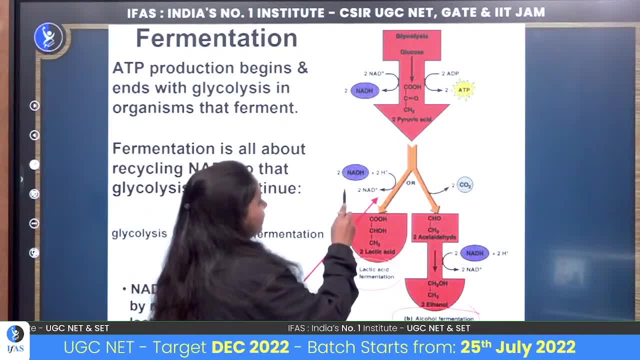 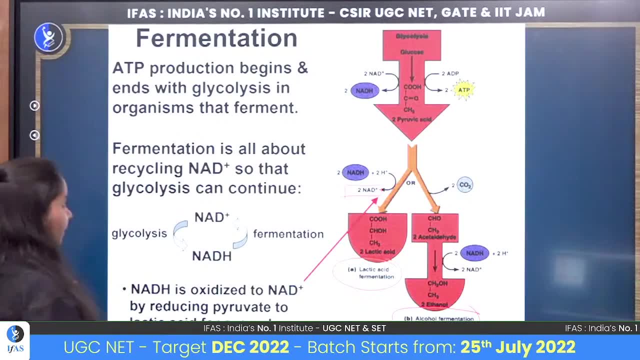 So, after lactic acid fermentation, what will happen here? only here NAD is generated. okay, here it means that whatever NAD remains here, it is only generated here. Now, when ATP production starts from your glycolysis, some ATP is created there. what happens in fermentation? your recycling of NAD++. 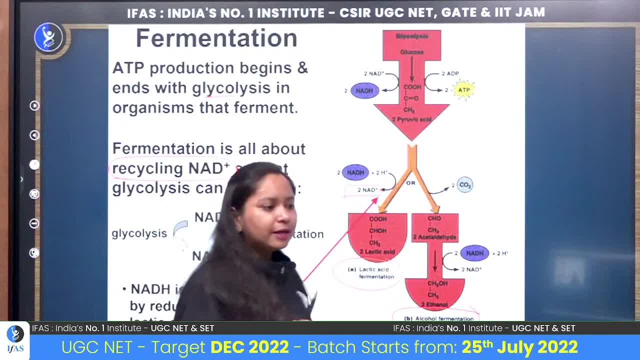 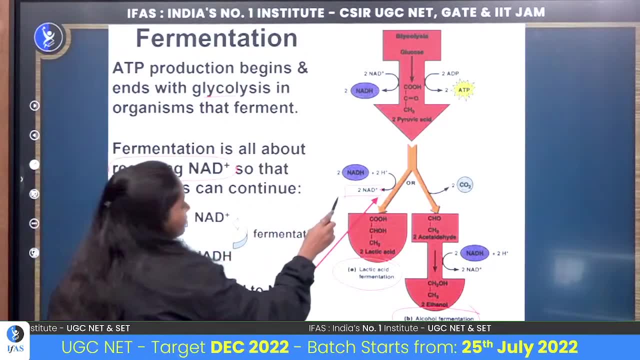 Okay, what is happening here? here, what is happening? only NAD is getting recycled, because, see, if this NAD is recycled here, If it is ready to be recycled, then it can be used again in this step and this pathway can be continued. 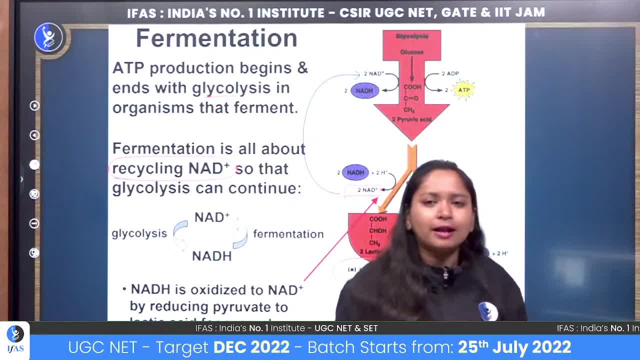 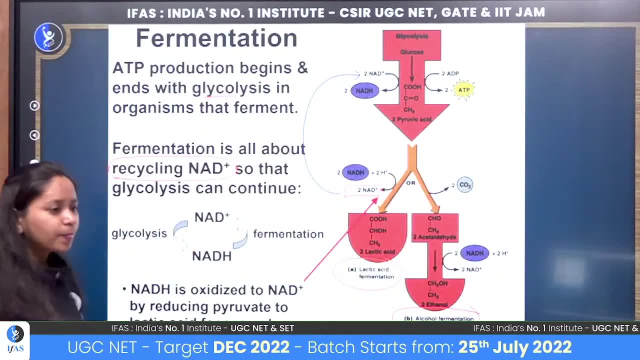 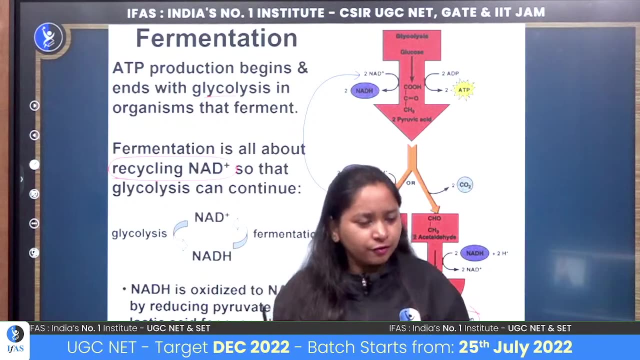 The pathway that remains is continuous and the steps above the glycolysis, the NAD, is also fulfilled by this particular step. So in fermentation we cannot make a lot of energy. There is very less production of energy in case of your fermentation. The more energy you produce, the more your aerobic respiration pathway is. 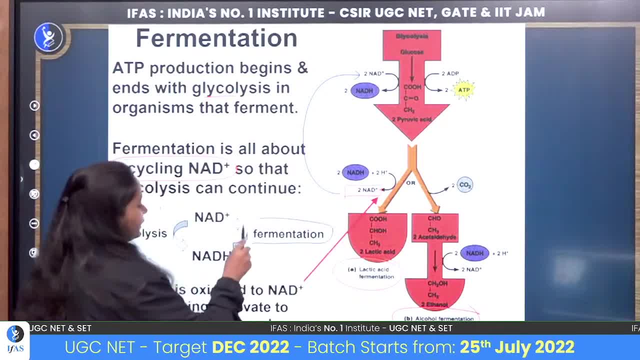 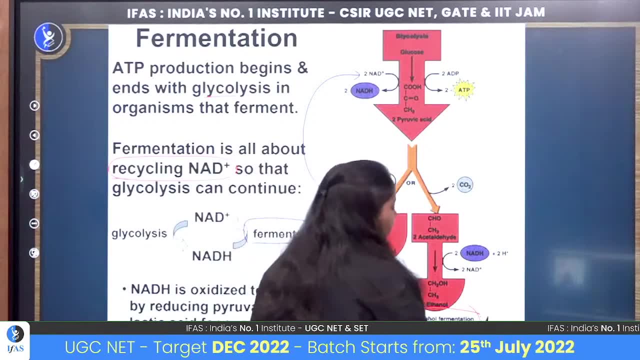 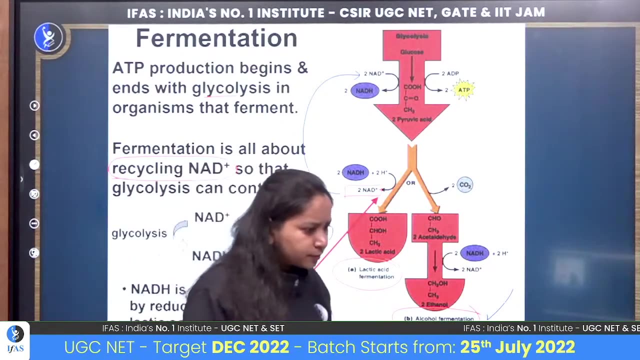 So what is happening in fermentation? here you have NAD recycling. Here NAD is getting just recycled, And another pathway that runs is your alcoholic fermentation, at the end of which you have the production of ethanol. What remains at the end is: That is your ethanol. 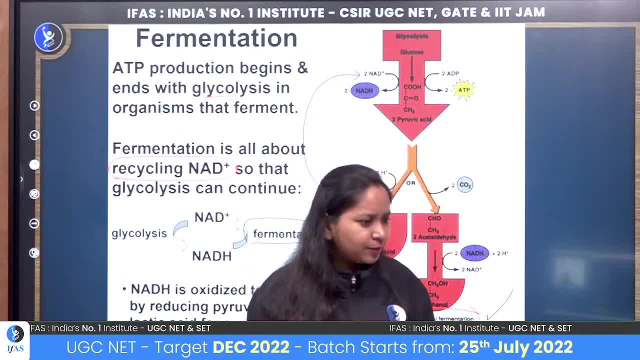 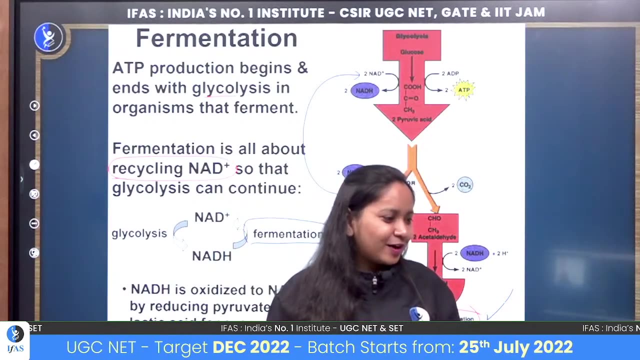 Is your question in the form of an image, You can type the message. It is not going to request. Are you seeing some request or question? Look, use short forms, but not so much that I don't understand. Okay, Are you asking if there is a request or a question? 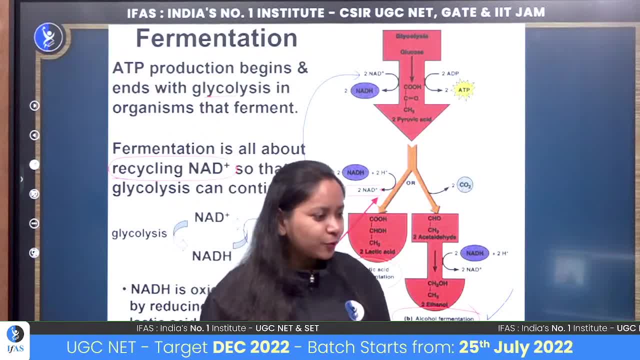 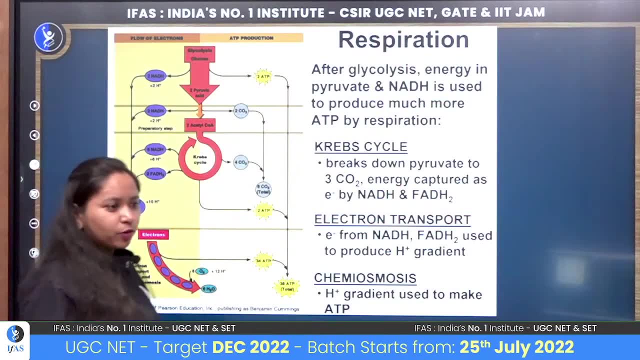 If you are writing a message in the chat box, then you can write the question here. Okay Now. Next is the respiration, which is very important for us. Someone asks questions from here. They will ask how much ATP is being formed, where ATP is being formed, how it is being formed. 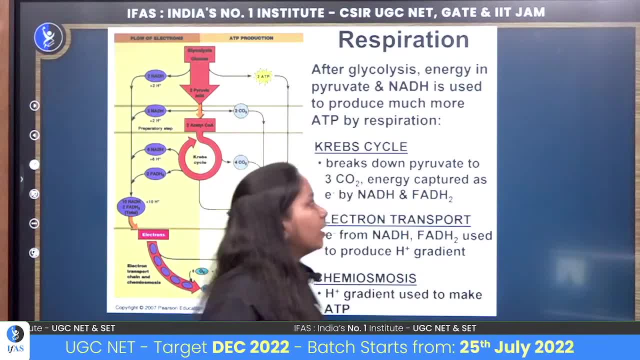 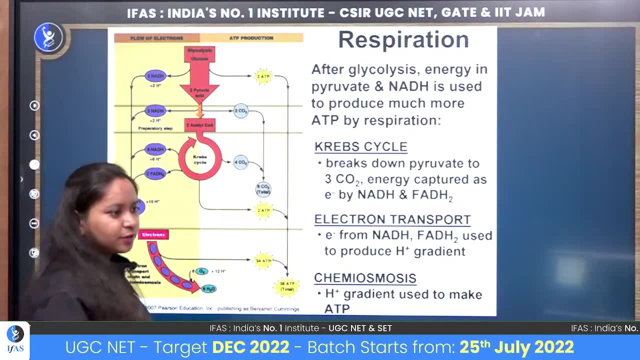 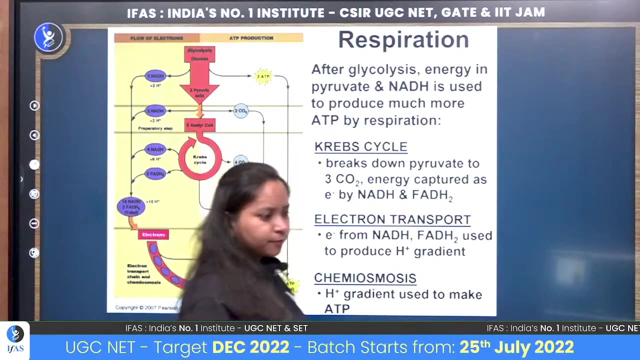 So from here you are asked the maximum questions. Now, if we talk about your respiration, then what will happen here? oxygen will come here. What is happening here? oxygen is coming here right now. Hello Gargi, Okay, it will come here. then your energy will come now. 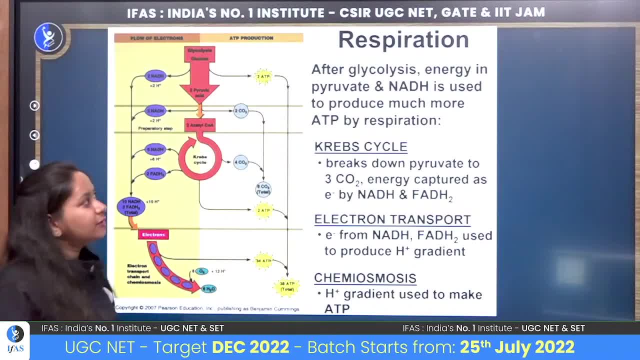 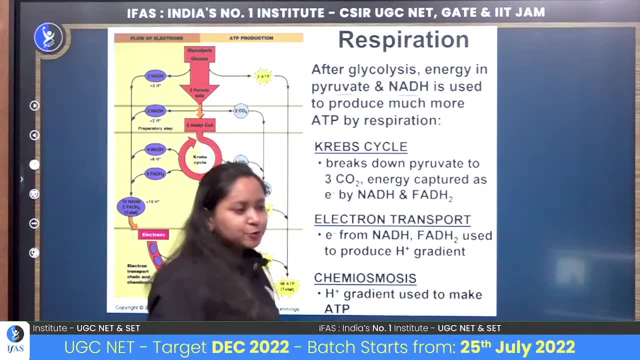 Now what is happening here When your glycolysis ends? So whatever energy you have made, whatever energy will remain in pyruvate, Whatever energy will remain in NADH, All that is used, all that is used in the production of your ATP By respiration mechanism. 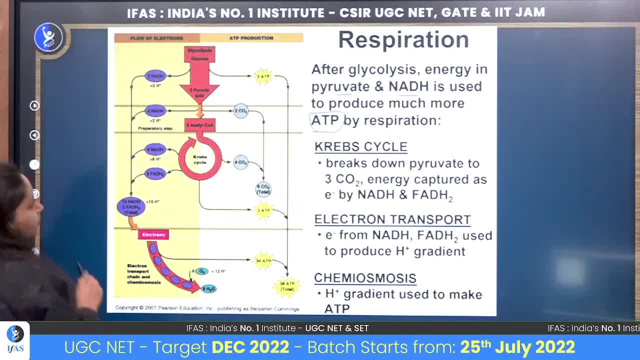 Okay, By respiration mechanism, whatever energy you have made, Whatever your energy molecules have been made, We use them now for preparing this ATP. Now what happens? Now what happens? So our pyruvate was made. we saw that pyruvate was made. 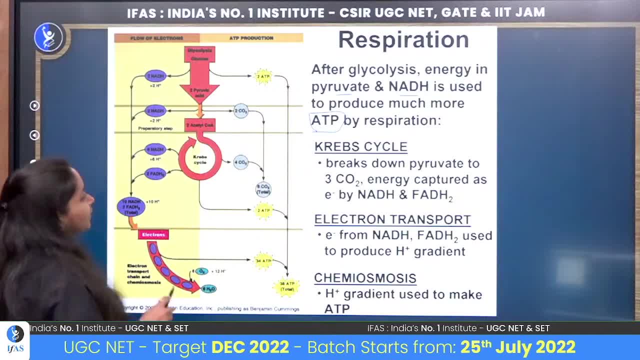 So pyruvate plus oxaloacetic acid is made together, Your TCA cycle starts Right When your pyruvic acid will remain, It will get converted to acetyl coenzyme A. I am very sorry. When this is made, your acetyl coenzyme A is formed. 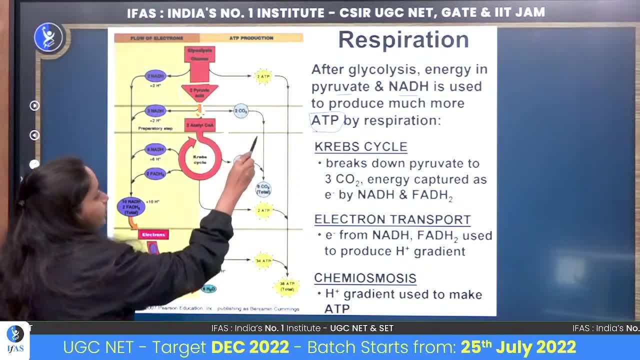 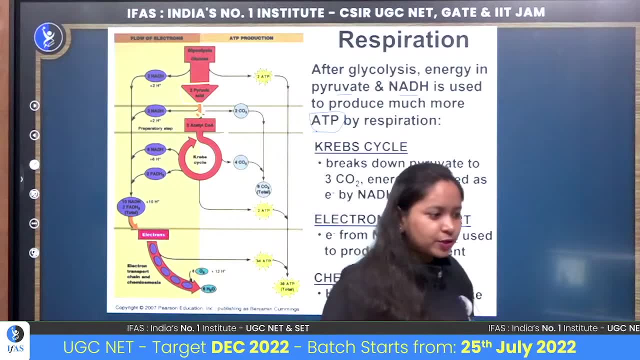 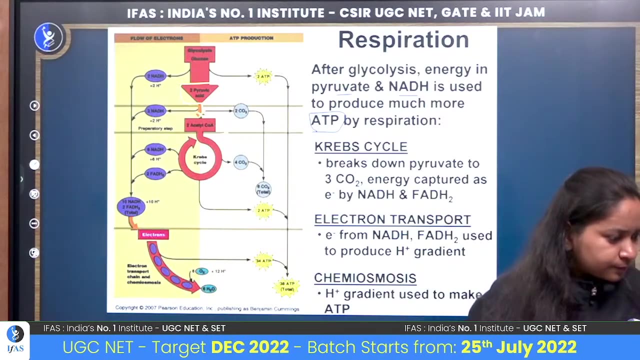 And this plus oxaloacetic acid- that remains. This enters in your TCA cycle. Okay, This acetyl coenzyme A is a two carbon compound. Okay, Pyruvic acid- that remains. That remains. This is a carbon compound. This is your two carbon compound. How is it disappearing like this? 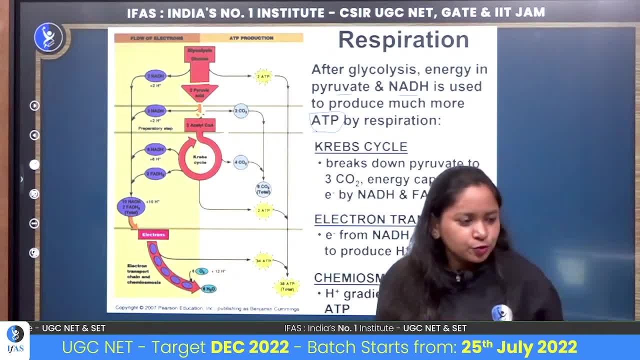 Okay, Viru. Okay, If your child has any request for some topic, Then you comment at the end of the session. So we will check it after seeing it. Okay, We will check it at the end of the session And whatever your important topics are, We can conduct some sessions from that. 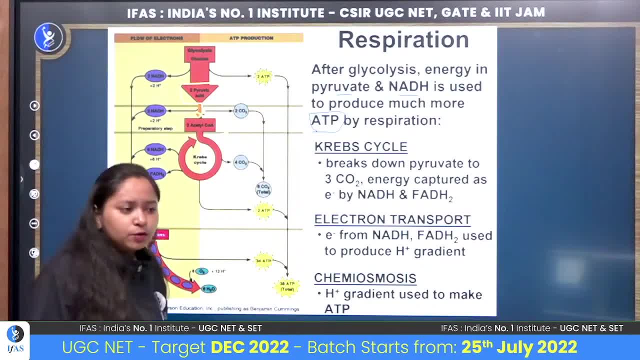 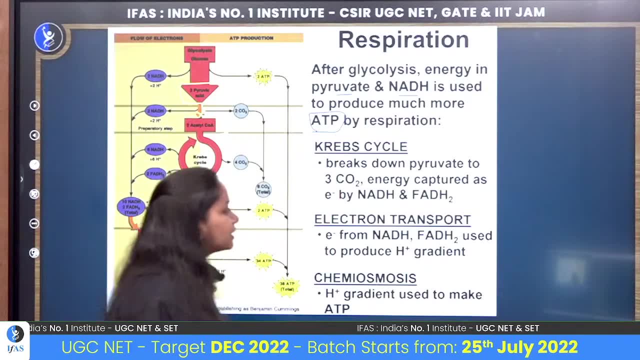 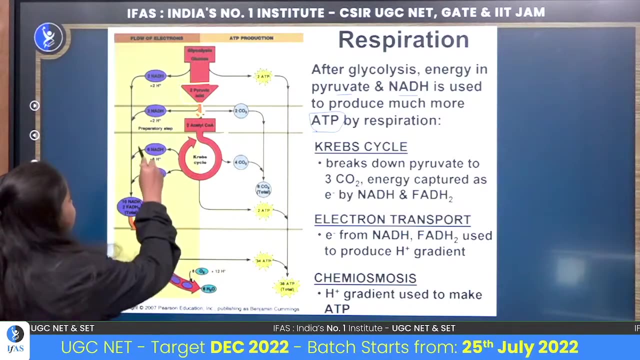 From those topics as well. Okay, After that comes your Krebs cycle, And Krebs cycle is your TCA cycle. And what happens in this cycle? So here again, some of your energy molecules are formed. How much energy is made? So here your 6 NADH is made. 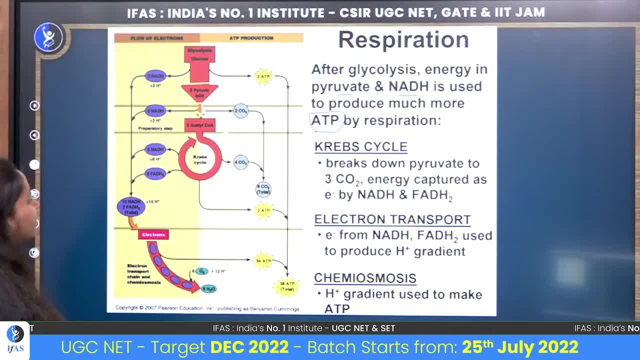 2 FADH is made. So, whatever your gain is here, In the step of glycolysis, When glycolysis was going on, What was made from here? Your 2 NADH. So NADH. In this step, again, your 2 NADH is made. 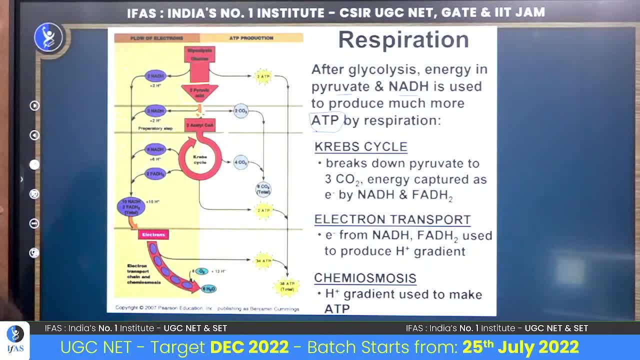 Here your 6 NADH is made Okay. So your total net gain is 10 NADH. Okay, 10 NADH is getting formed from 1 glucose, In case of your aerobic respiration. Okay, In case of your aerobic respiration. And if we talk about FADH, 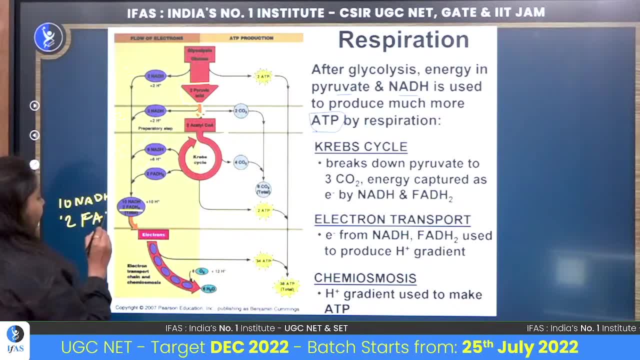 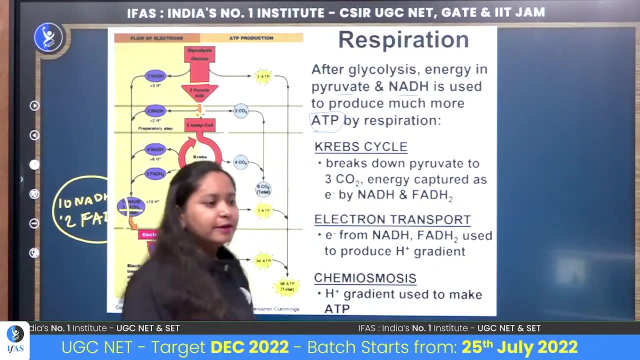 Here your 2 FADH is also formed. 2 FADH are formed And now these will enter in the electron transport chain. Okay, These will enter in your electron transport chain. In your chain, Your NADH FADH will be used. This will make your proton gradient. 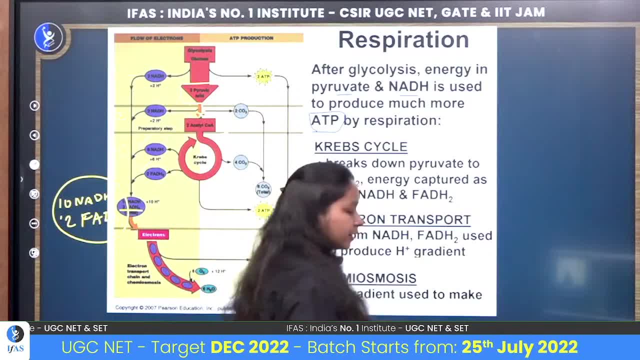 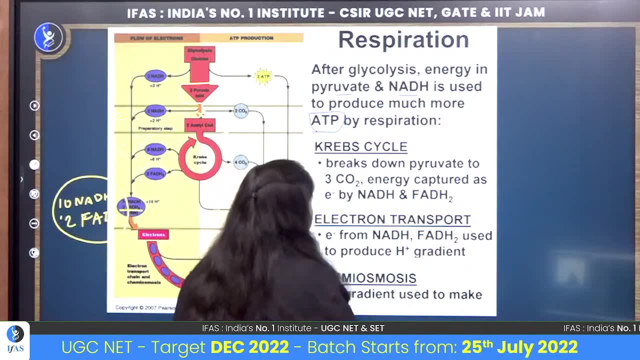 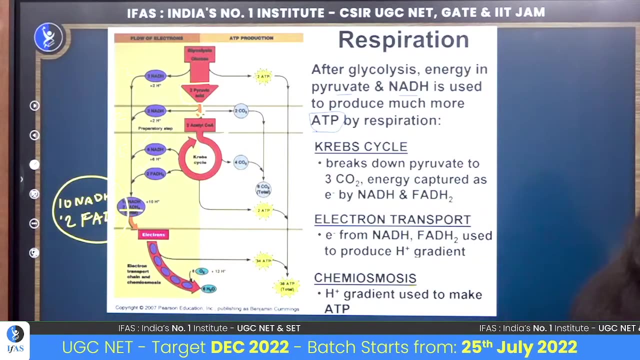 Okay, This will make your proton gradient. Now here comes a mechanism Which we call chemiosmosis. Can you tell what is chemiosmosis? There is a process called as chemiosmosis. What is chemiosmosis? It is a process called as chemiosmosis. 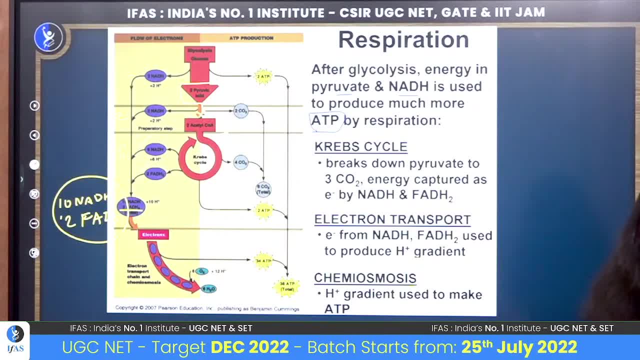 It is called as chemiosmosis. What is chemiosmosis? It is a process called as chemiosmosis. And what is chemiosmosis? It is called as chemiosmosis. It is also called as chemiosmosis. So in this case, 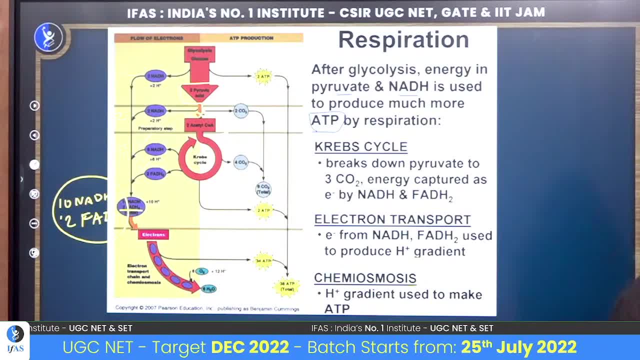 Chemiosmosis is produced by All the molecules Formed by the atom. Yes, Parham, It is also formed there. Your enzyme is pyruvate dehydrogenase. Molecules are formed there. No one is able to find out your question If someone else can see your question. 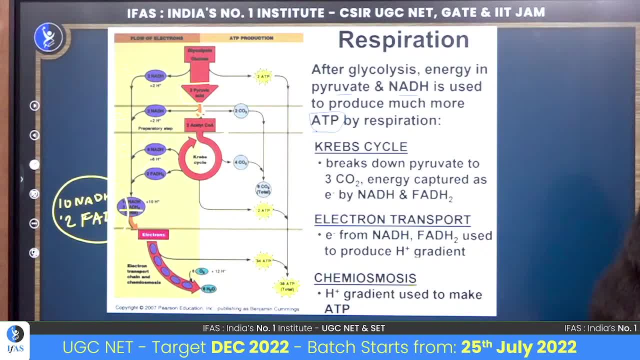 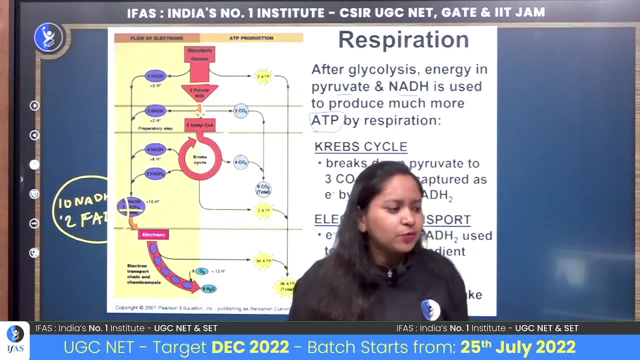 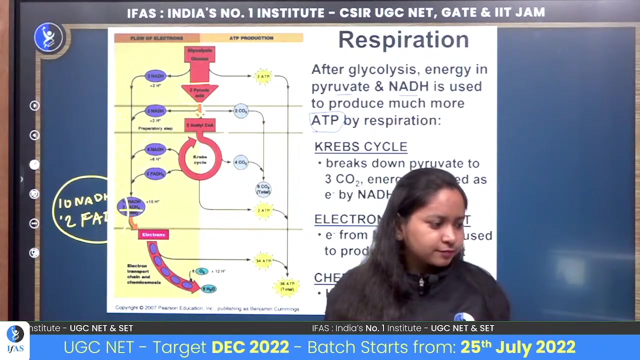 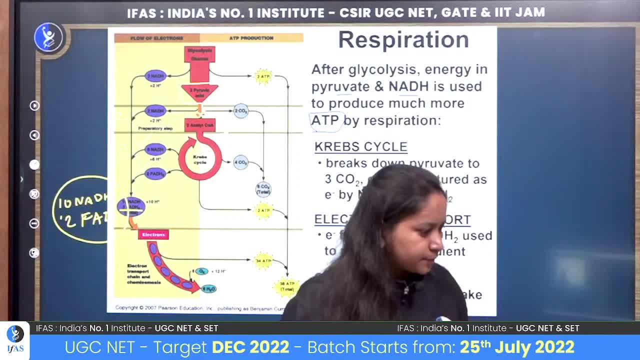 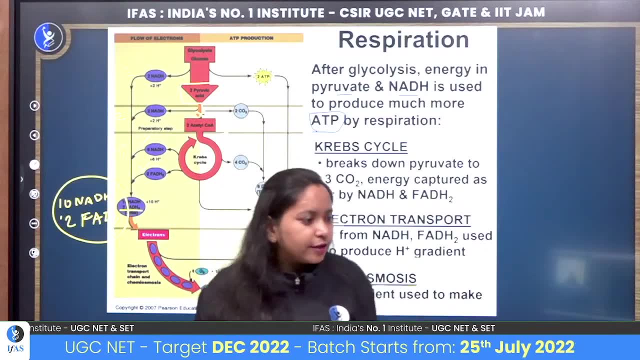 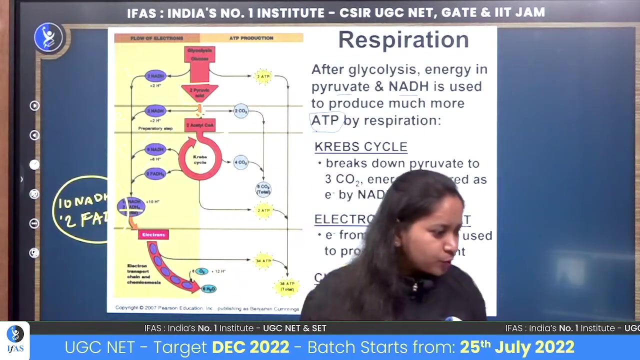 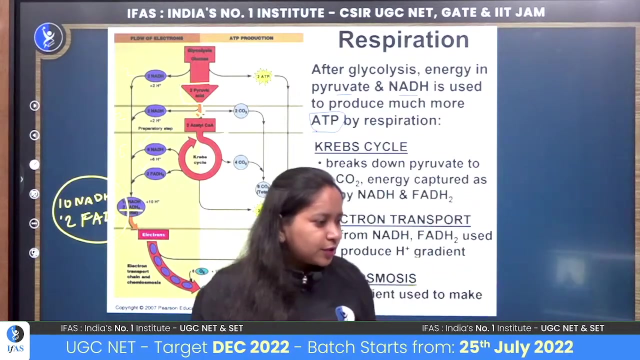 Okay, okay, okay, See, yes, okay, If we talk about osmosis. So what is osmosis called? Movement of water from its high concentration, its low concentration, through a semi-permeable membrane. This is osmosis. I think you are answering this right. Your high concentration, low concentration, okay? 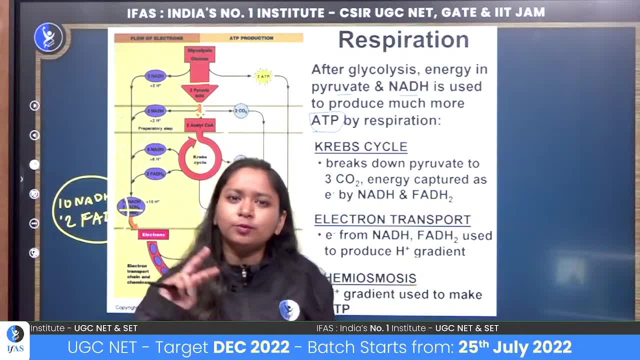 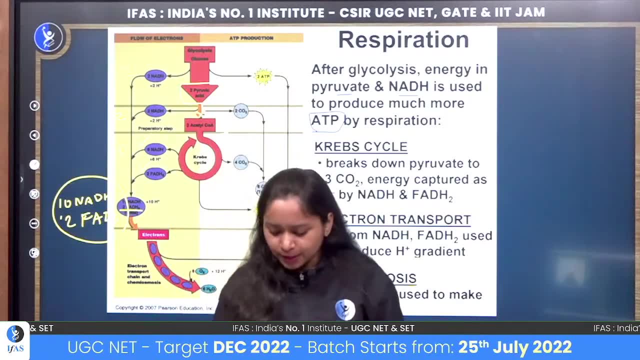 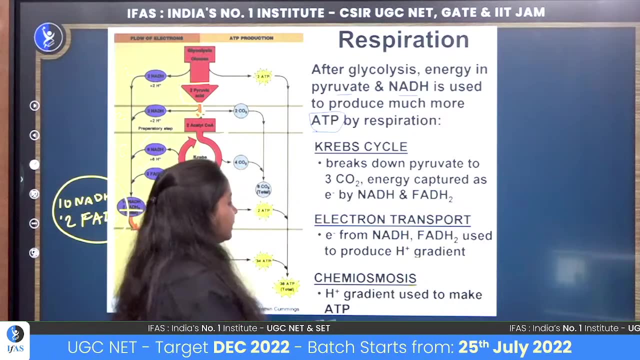 So that is osmosis, where we check the movement of water. But if we talk about your chemiosmosis, here we talk about ions. The ions that remain here move and they will prepare a concentration gradient and that gradient will be now used to make this ATP. okay, We use it to make this ATP. 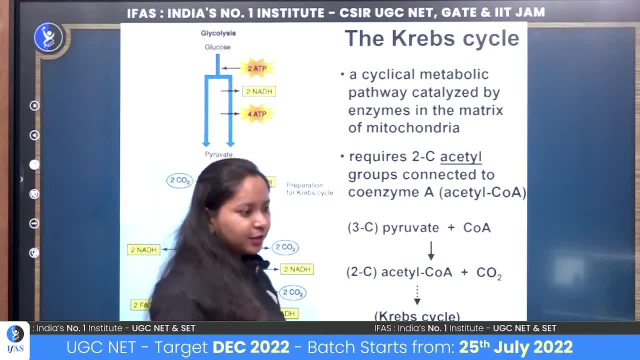 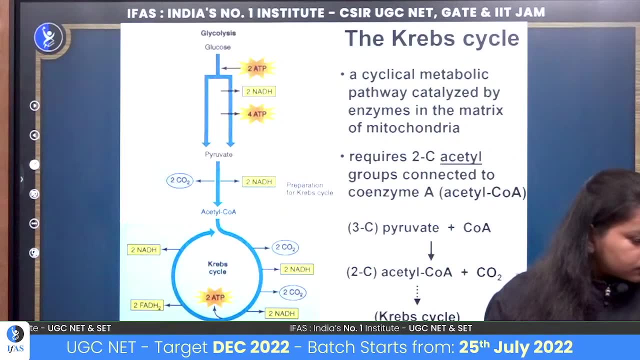 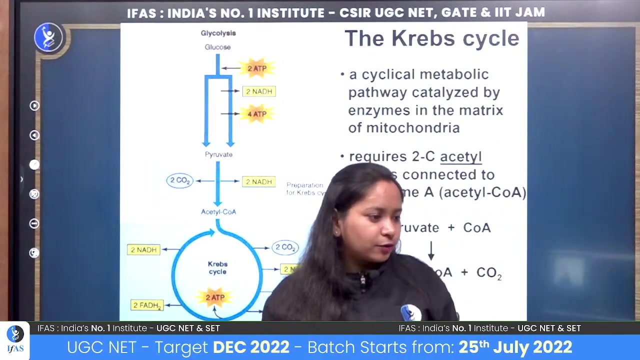 Now, if we talk about your Krebs cycle, okay, If we talk about your Krebs cycle- excessive mental work, stress, anxiety type situation- What exactly Lactic acid formation molecule? No, no, Lactic acid is made only in case of your physical workout, If you are physically working. 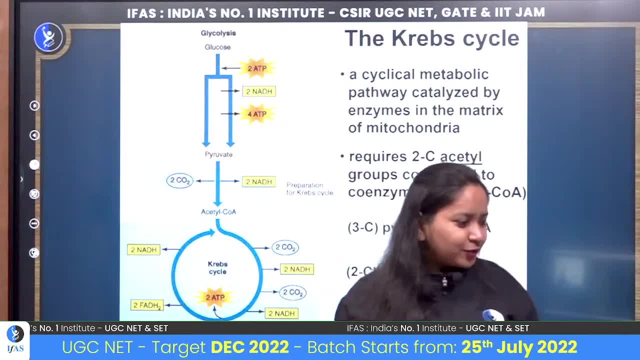 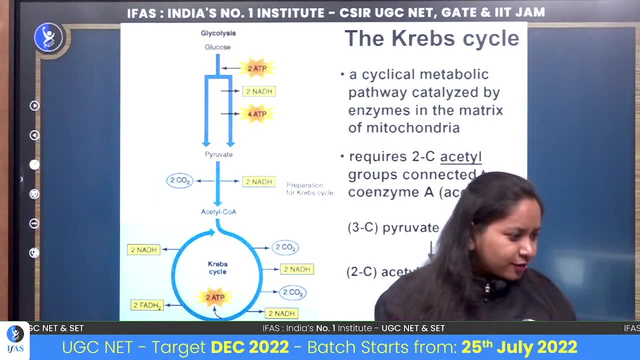 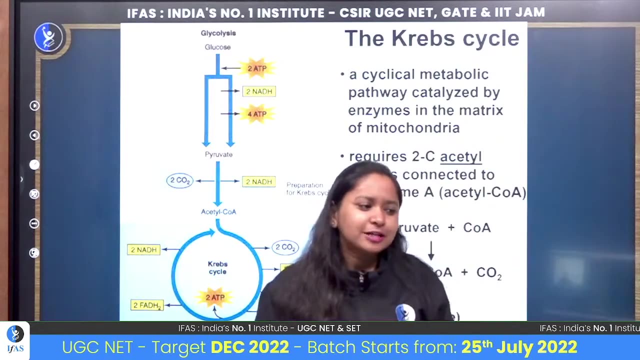 out a lot. okay In that. yes, I have seen that. By the way, it has broken in pieces. Lactic acid formation molecule is made only in physical workout or excessive mental work and stress, not It will not be made in excessive anxiety when you are physically working out a lot in that case. 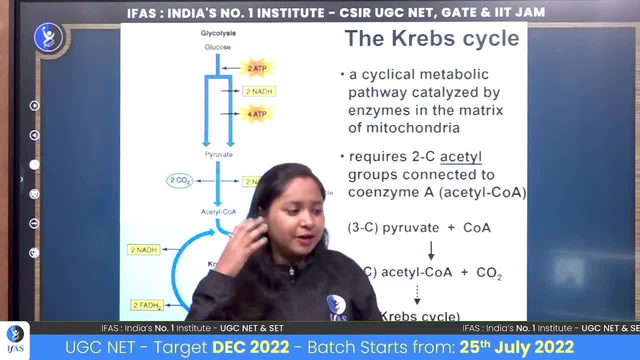 it will be formed, Because if you are physically working out, if you are like mentally stressed or something, then what happens is in that case your muscles do not work so much right. Oxygen demand in the body does not increase at all When the oxygen demand increases when you are. 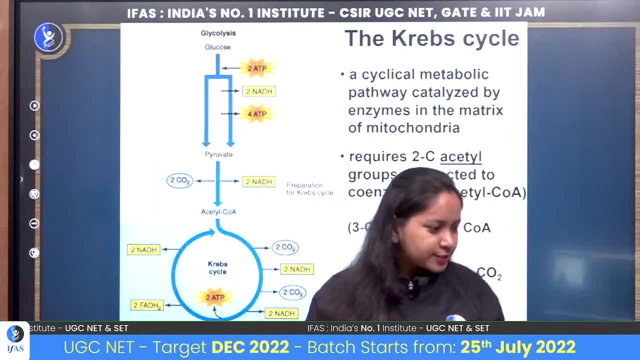 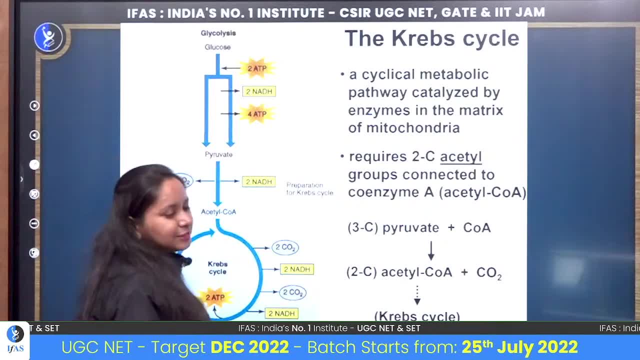 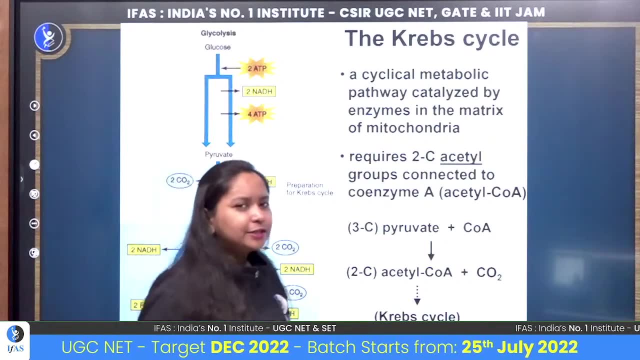 Okay, Okay, Okay, Okay, Okay. So, yes, what happens? where does your TC cycle run? first of all, it runs in the matrix of your mitochondria. Okay, tell me, where does your ETC run, in us. 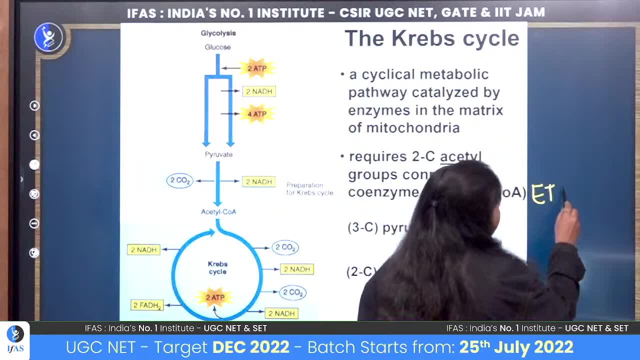 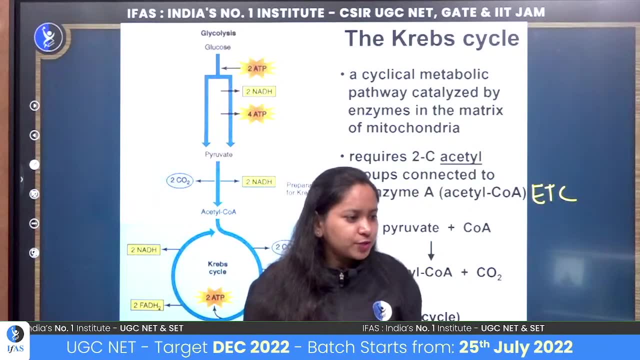 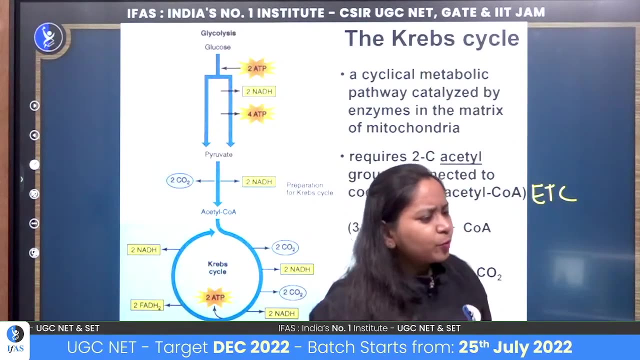 Where does the electron transport chain run in the case of humans? Where does the electron transport chain run in us? In that condition, you may have normal shortness of breath. In that case, there can be normal shortness of breath. See, when you are stressed, do you get cramps? 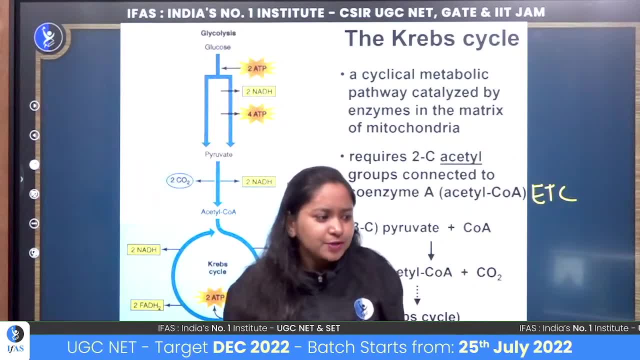 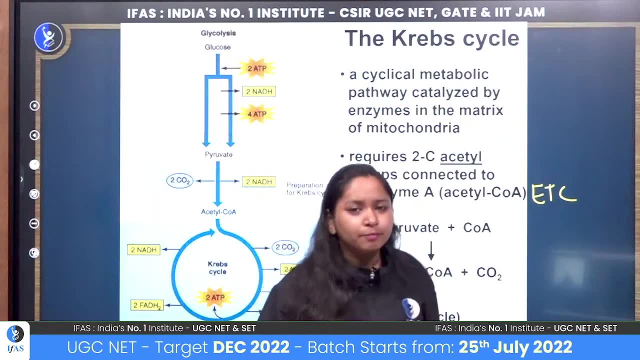 We never get cramps right. What does it mean that you are getting cramps? It means that there is a lot of physical exertion in your body. You have pain. you have pain in your knees. our muscles start paining. there is pain in the thigh muscles. 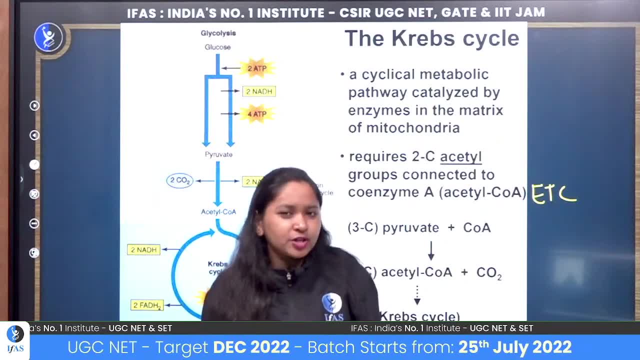 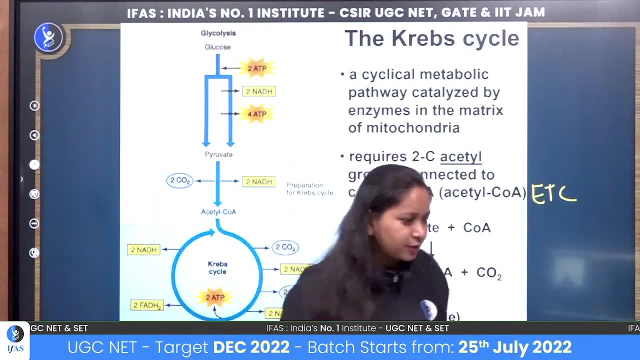 Okay. so if you are stressed, if you are worried, you may have shortness of breath for some time, But in the case of lactic acid, there is no shortness of breath. Okay, that will come later when there is a lot of it. 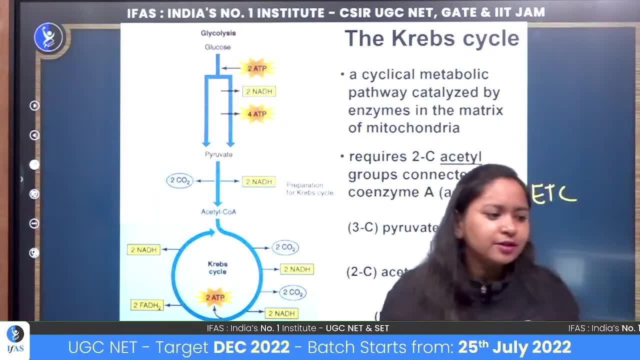 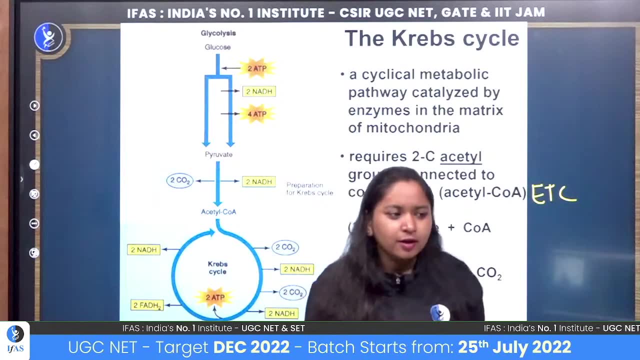 Yeah, we can say Yes, it takes place in the inner mitochondrial membrane. Okay, good, If we talk about bacteria, then where does it happen in them? In case of bacteria, what is the site for electron transport chain? Very good everyone, good answers. 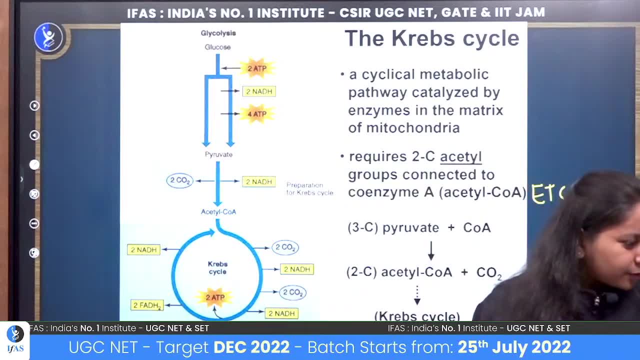 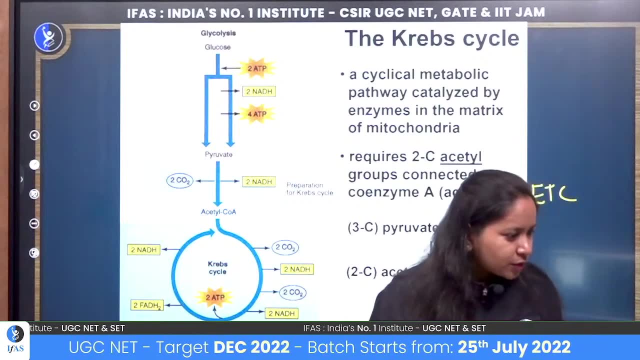 Everyone gave me the correct answer here: Janhvi Samad, Amit Rishi, Pradiksha Vagdevi, Karishma Veeru, Sonal Anamika. Sonal Anamika. 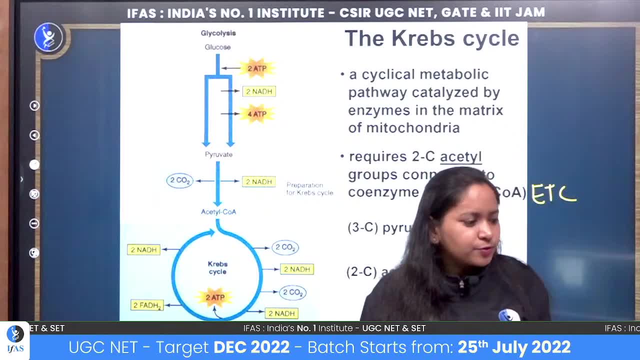 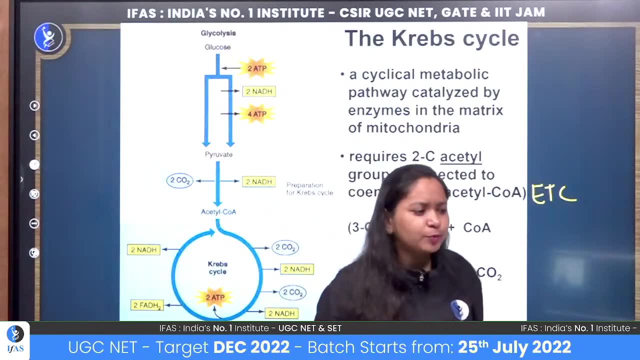 Yes, yes, yes, Rishi, In case of prokaryotes, in case of bacteria, it takes place in their plasma membrane. Okay, in their plasma membrane, all the metabolism. when there is an electron transport chain, it runs in that particular region. 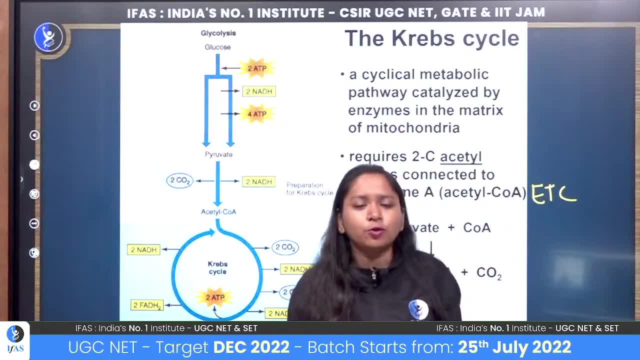 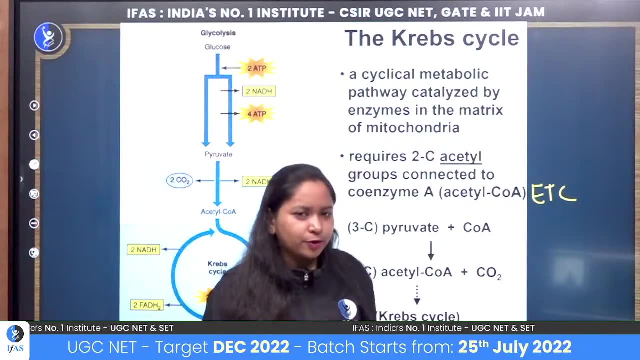 Okay, Because we know that prokaryotes, they do not have proper, well-defined organelles. they do not have them. So when their membrane is there, their electron transport chain runs there. In case of plants, where does it happen? 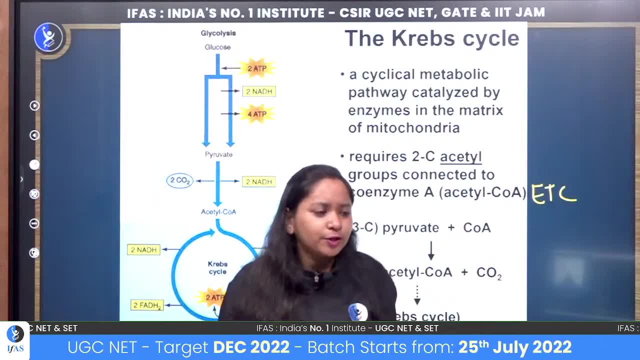 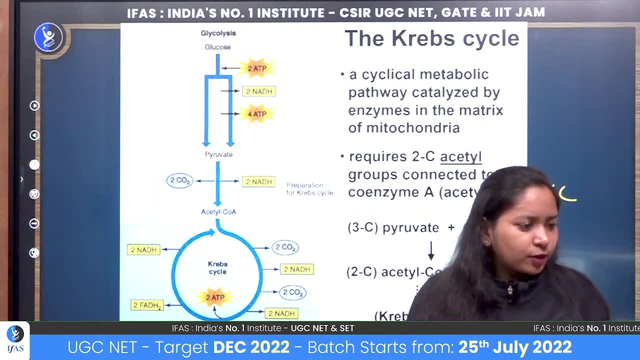 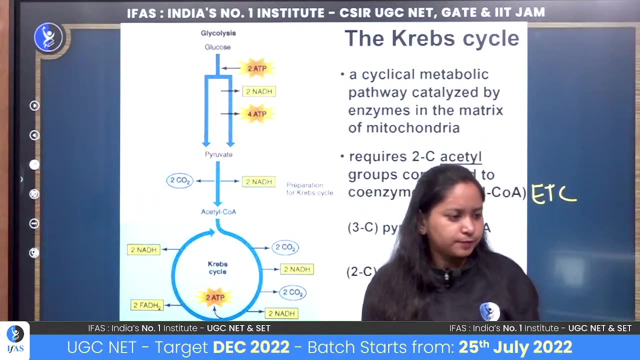 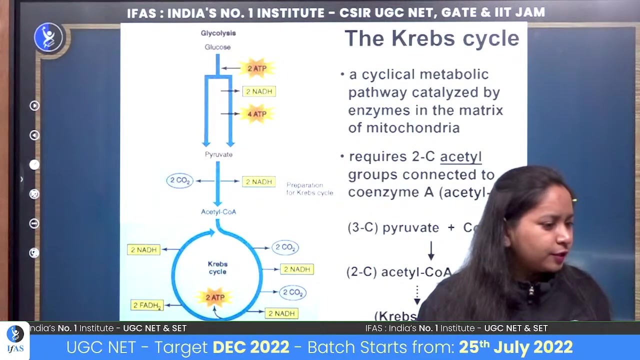 In case of plants. what is the site for electron transport chain In case of plants? where does their electron transport chain take place? Chloroplast- Okay, where does chloroplast take place exactly? In case of? where does chloroplast take place? 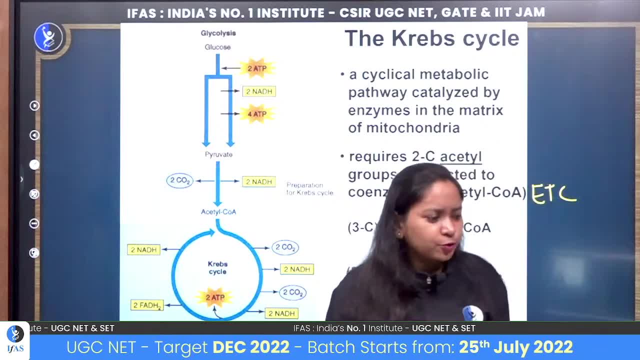 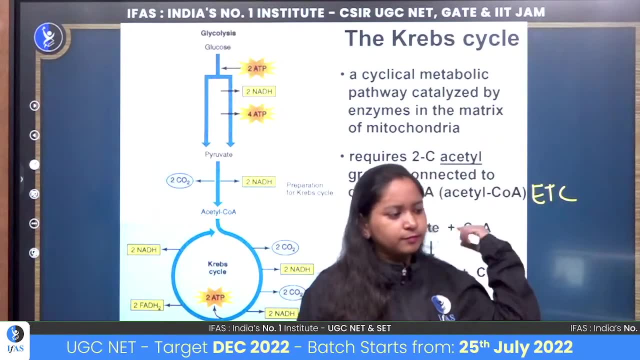 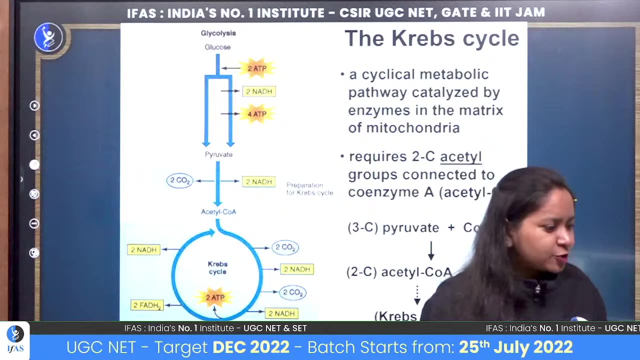 In the mitochondrial membrane of plants. Chloroplast takes place in the mitochondrial membrane of plants. Some are saying chloroplast, some are saying mitochondria In plants. on thylakoid, some are saying on thylakoid, Karishma is saying thylakoid. 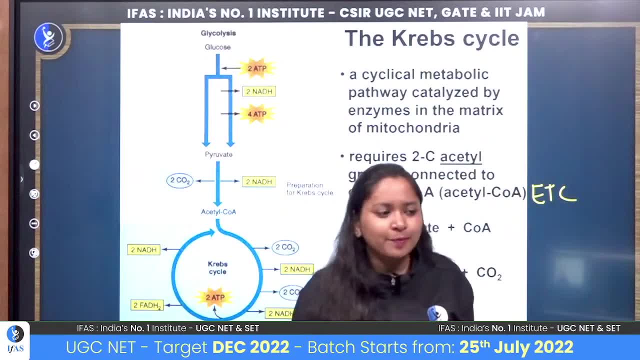 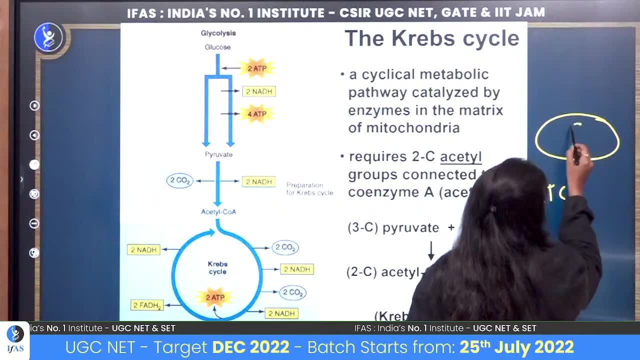 Yes, yes, yes. So see, in plants mitochondria does not take place. Okay, if we talk about plants, they have this chloroplast. Chloroplasts have thylakoid in them. they are called grana. 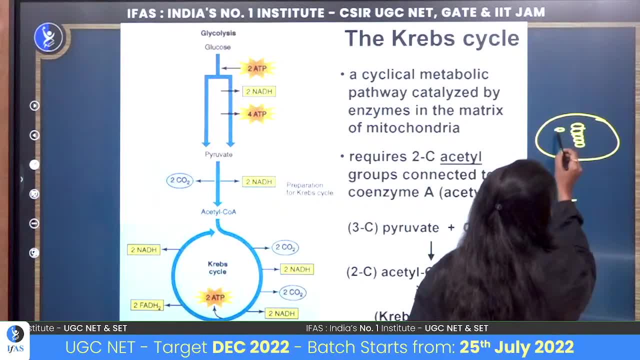 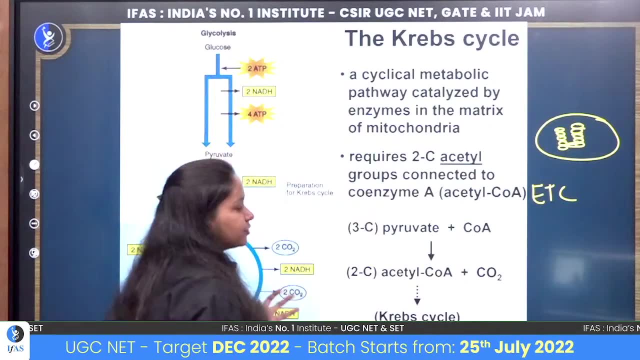 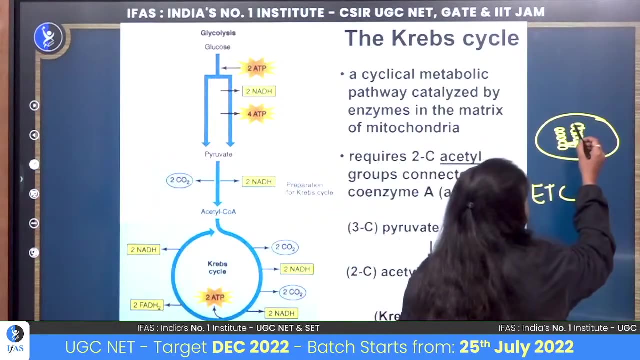 You call it grana- Which are connected to each other in this way, Right Later in the rest of the region. their stroma is present there. So when they have grana, when they have thylakoid, it runs in their membrane. 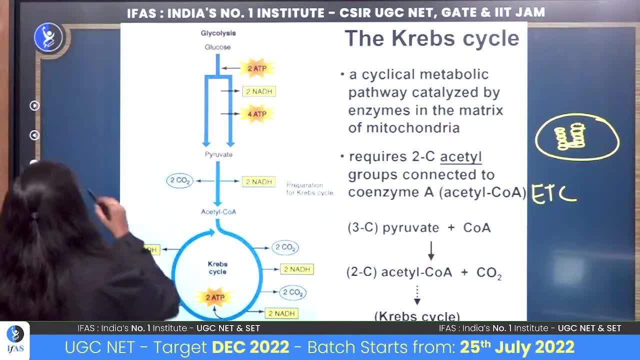 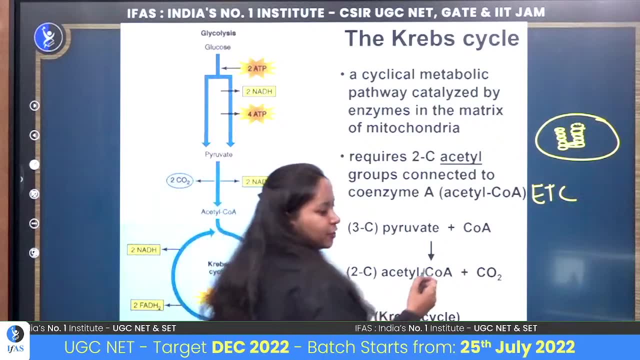 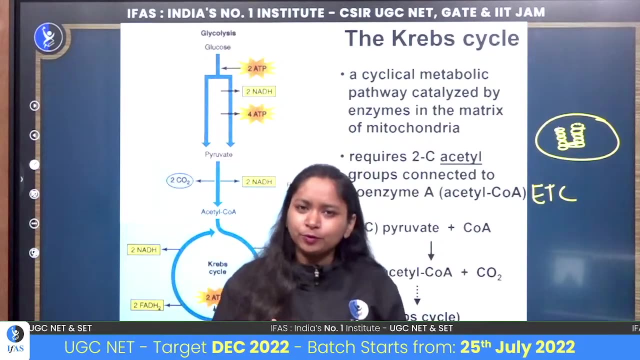 Okay, In the membrane of thylakoid electron transport chain runs in the plants. Okay, In their thylakoid membrane. it runs there, Their electron transport chain. So it will not take place in the mitochondria. In case of animals, mitochondria is present in the inner membrane, etc. 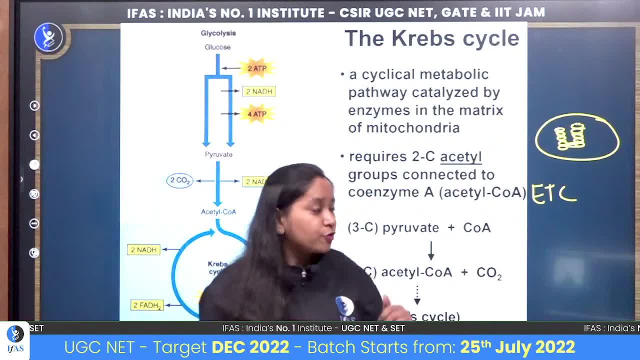 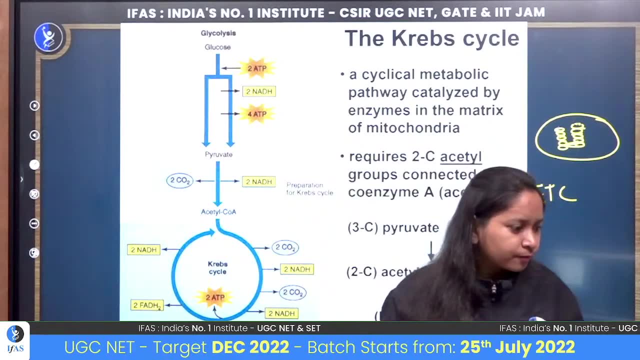 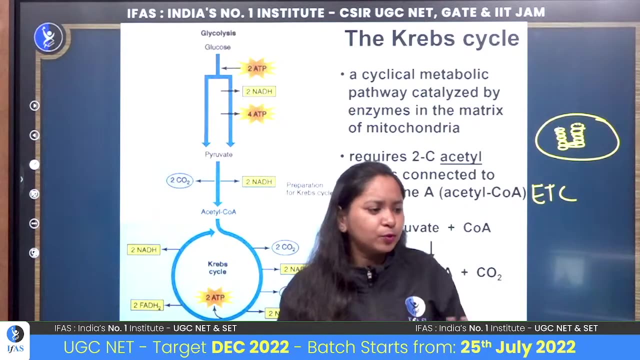 In case of bacteria, it is the plasma membrane And in case of your plants, it is the thylakoid membrane which is present in their chloroplasts. It could be dangerous. But, yeah, if you are stressed, if, like you, are sitting, in that case there will be no formation. 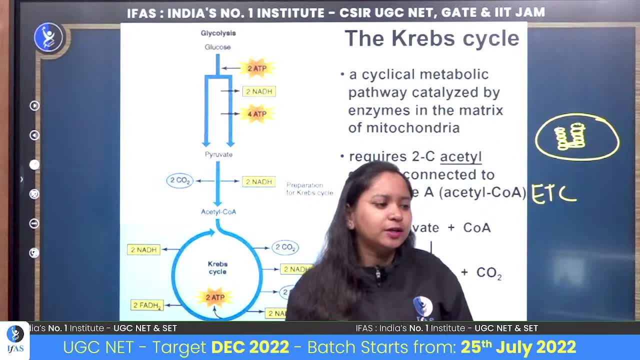 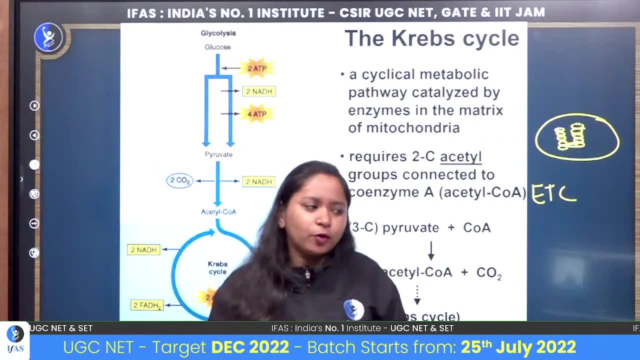 Okay, If you are not working out physically. see when will lactic acid be formed? When there will be deficiency of oxygen in your muscles. Okay, When there will be deficiency of oxygen in your body, in the muscles, then lactic acid is formed. 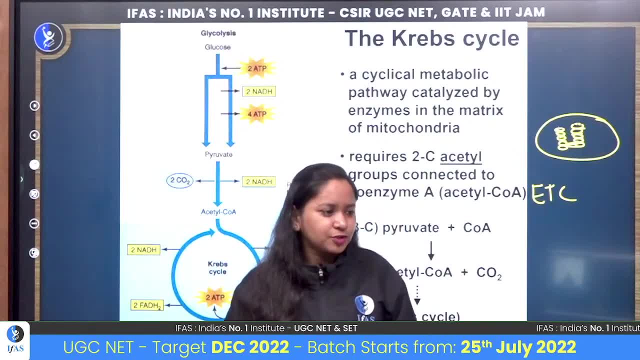 If it is not formed in the stress condition you are not working out that much. Deficiency is not there. Maybe you are very worried. you get a sudden breath. we get stress. heartbeats become fast. That is a different thing. 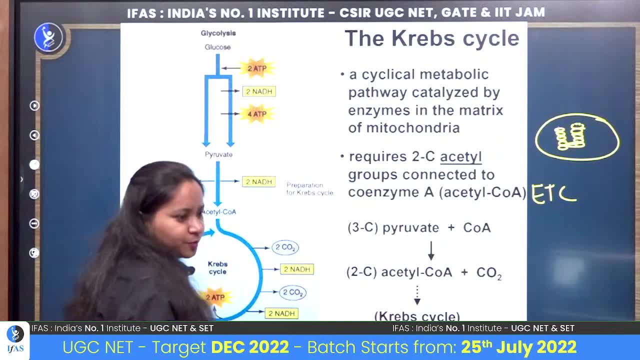 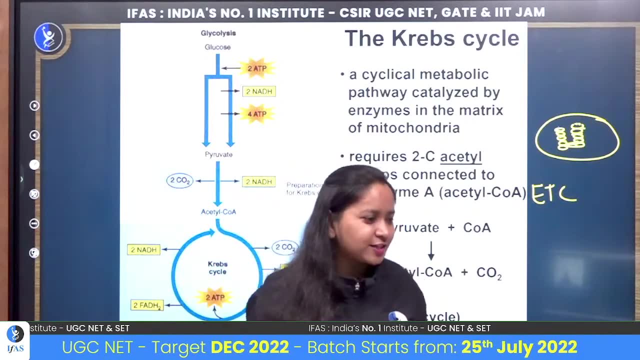 Okay, Okay, So let's have a session in which we will discuss animal sciences. Okay, I think some of my students are here, So they will know that we have discussed all this in the sessions. Okay, Let's go. 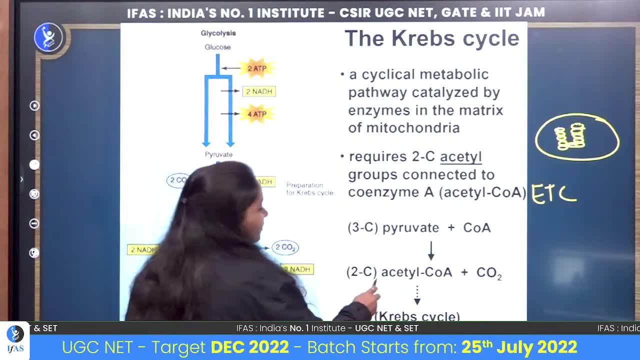 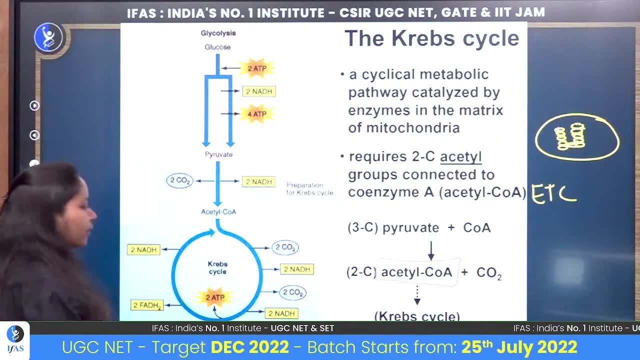 So, yes, what is happening here? Acetyl Coenzyme A is forming. This is entering in your TCA cycle. It is getting added with your oxaloacetic will come here And then your Krebs cycle will be formed. This will start. 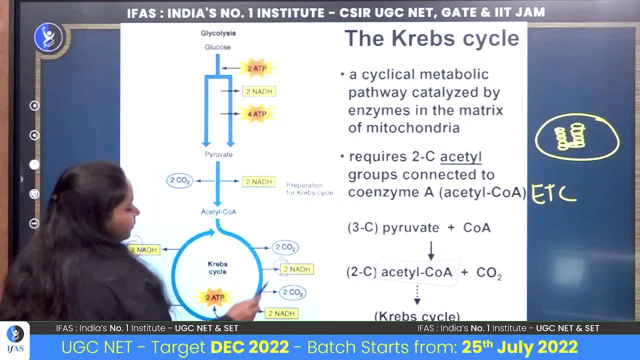 We have seen that your NADH is forming here. Okay, 6 NADH and 2 FADH2 are forming here, And they will now enter the Krebs cycle. So this is 2, 3,, 4,, 5,, 6,, 7,, 8 and this is 9, 10.. 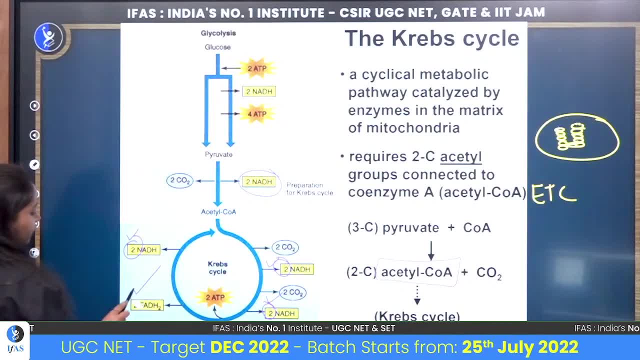 Okay, This is a FADH2.. This is FADH2.. I am counting NADH from this. So, yes, NADH2.. What is happening with all these? So, all these are making your NADH. 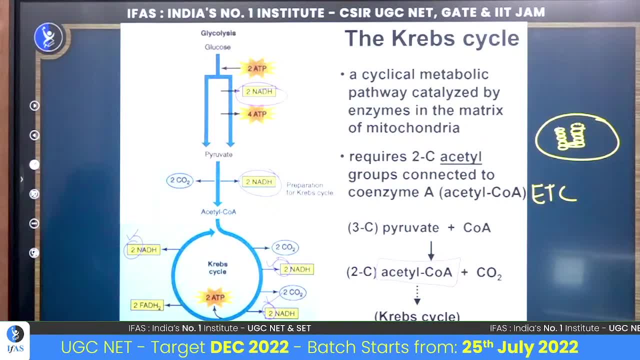 So our NADH is being made here, So we also get 2 FADH2.. So this is 2 FADH2.. So this is 2 FADH2.. So this is 2 FADH2.. 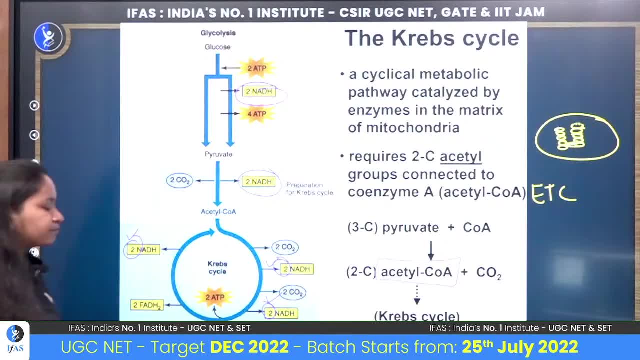 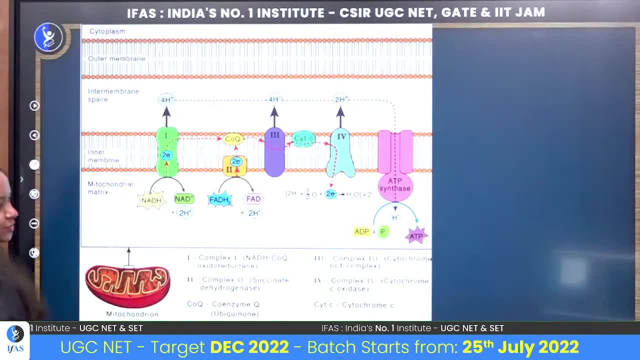 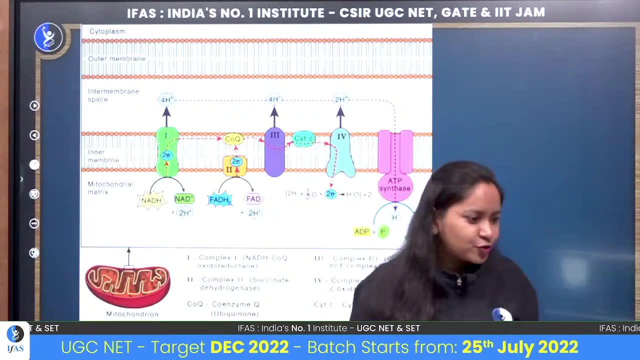 Okay, This makes your 2 FADH2.. What did you do which is not going in your comment? Now we will talk about the most important part, that is, electron transport chain. Okay, What will happen in electron transport chain? So membrane: 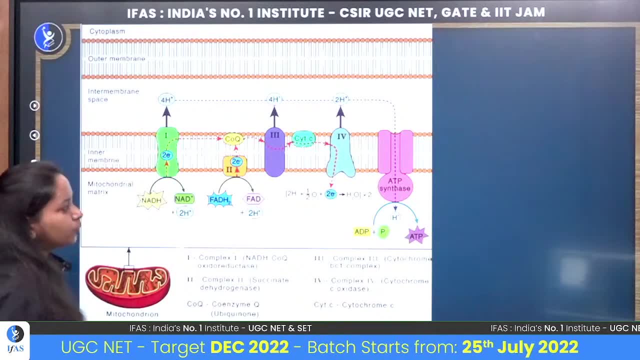 All your proteins are present on membrane Complex. 1,, 2,, 3,, 4 are present. At the end there is ATP, which is present in the synthesis, And that is why you can't destroy it. First complex breakdown is there. 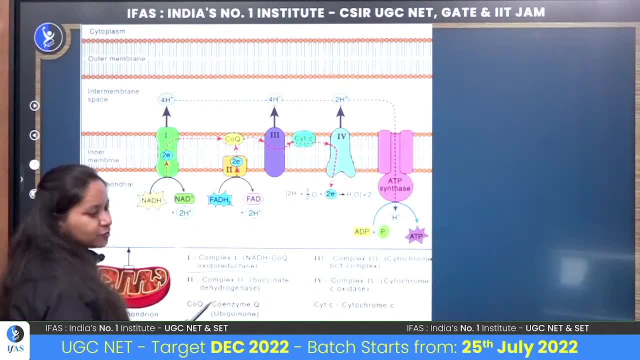 What happens? NADH oxidative reductase or NADH dehydrogenase. second is succinate dehydrogenase, third is your complex, that is, cytochrome BC1 complex, and fourth is cytochrome C oxidase. answer me one question. 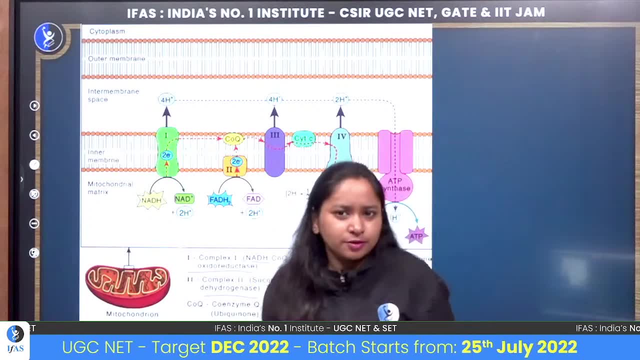 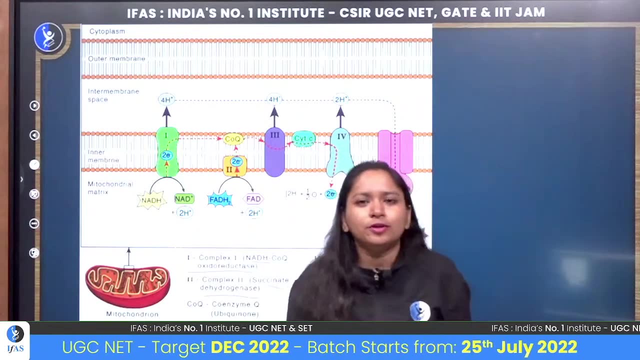 which is the only enzyme present commonly between the TCA cycle and the electron transport chain. ok, which is the common enzyme used in ETC as well as in TCA, which is that one enzyme used in both. you have to read about enzyme inhibitors. ok, actually, Veeru, I have not added that slide, but yeah, we can study that as well. 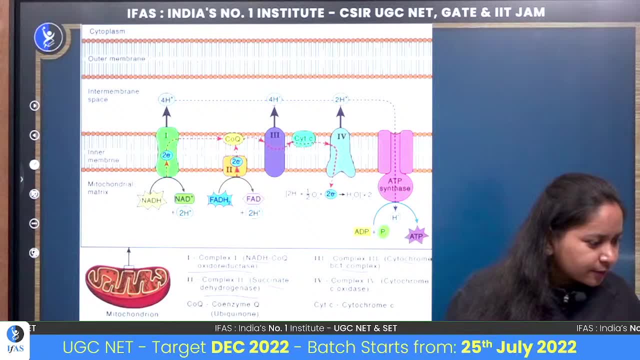 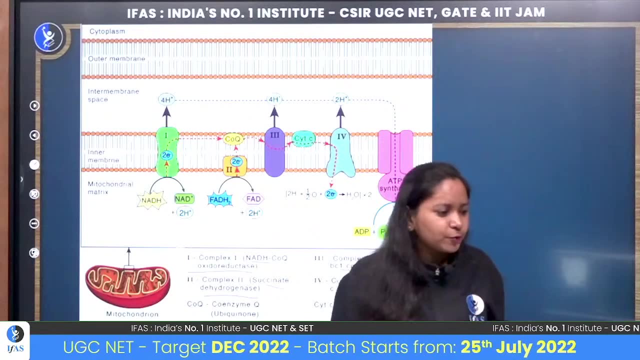 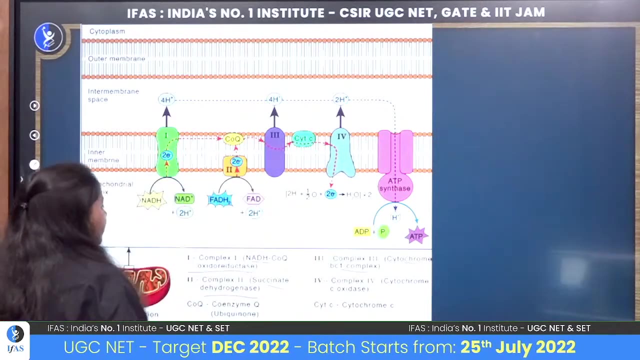 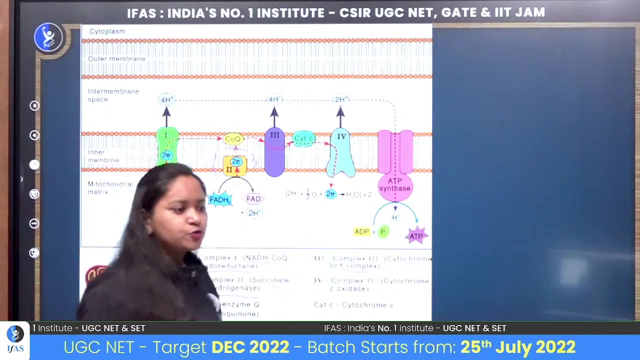 actually today we have to read about metabolism, so I have not added that slide. ok, Veeru is saying succinate dehydrogenase. ok, so yes, your enzyme which is succinate dehydrogenase complex 2. this is the only enzyme which is common between your electron transport chain and the TCA cycle. 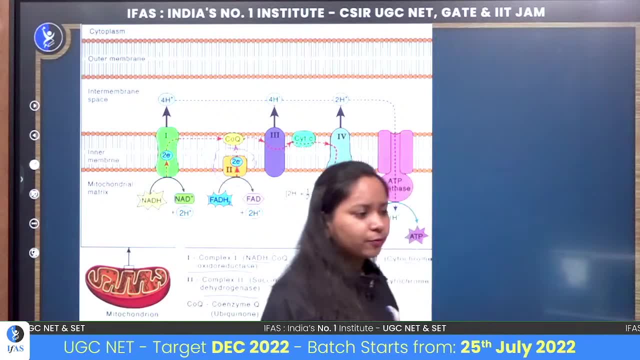 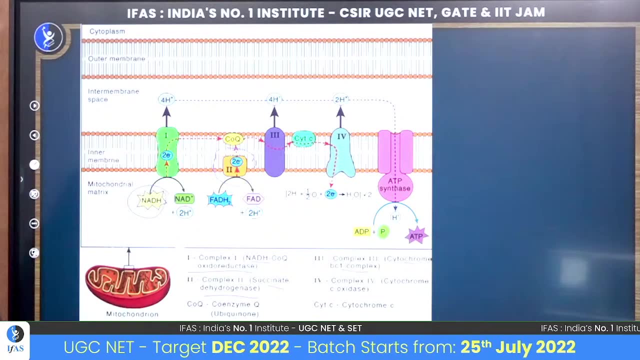 ok, this is common between the electron transport chain and the TCA cycle. see what happens here: NADH is used. when NADH is used, then the electrons start moving from here. when electrons start moving, then it will go to the pole, it will go to the coenzyme Q. 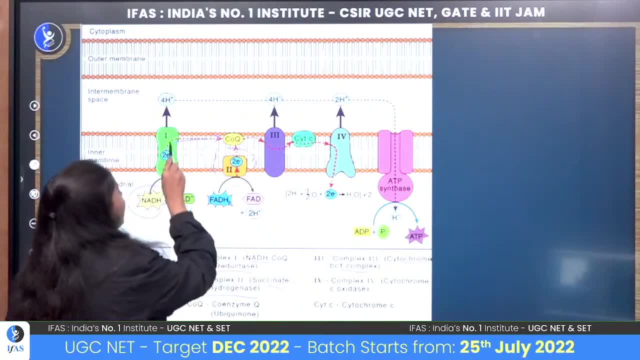 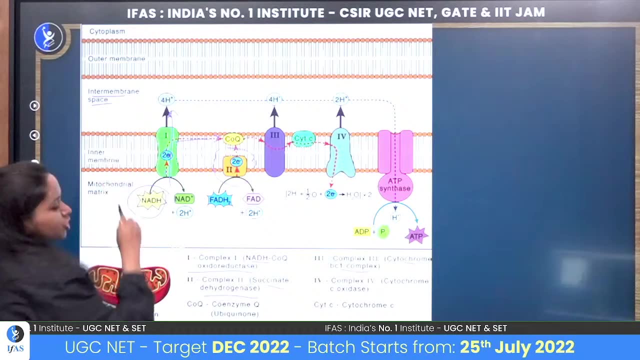 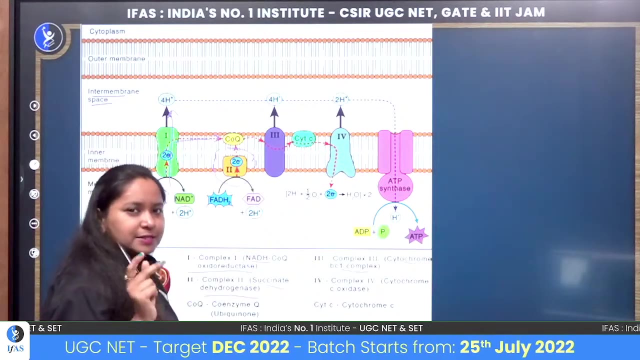 when electrons start moving, then the 4 protons go from here to the inter membrane space. in case of in the inter membrane space, your protons 4 go that direction. the second complex is the place where the protons are not transfered. when the second complex is not transfered, then the electrons can move forward. 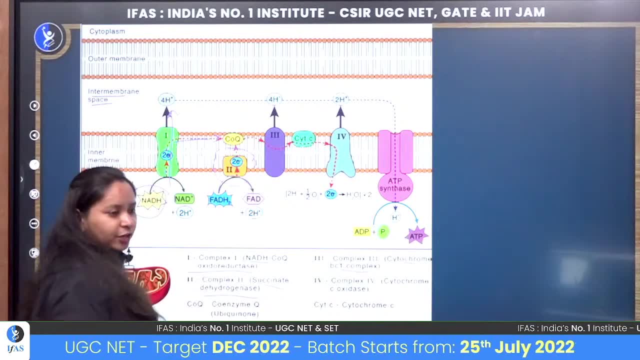 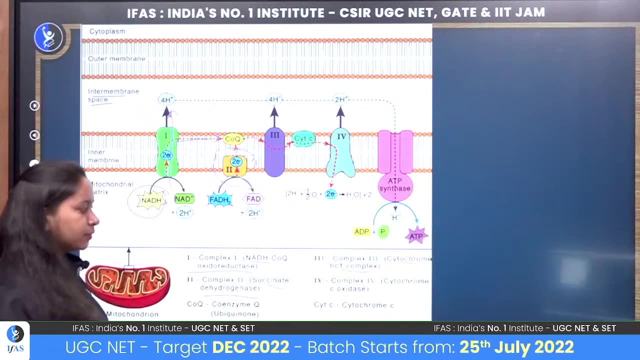 and here is FADH2. FADH2 is used here and electrons are transported to the coenzyme Q. electrons are transported to the protein which is known as coenzyme Q. we call it coenzyme Q. it works like a ferry boat. it keeps rotating on the membrane. 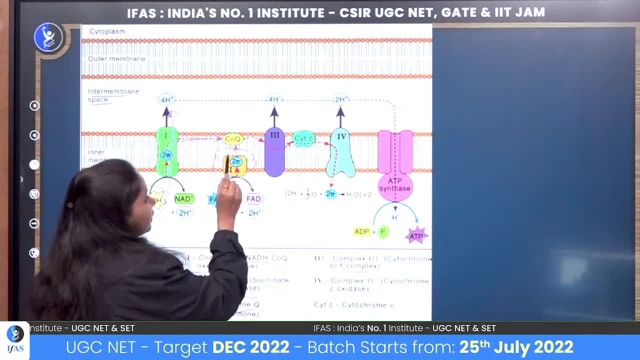 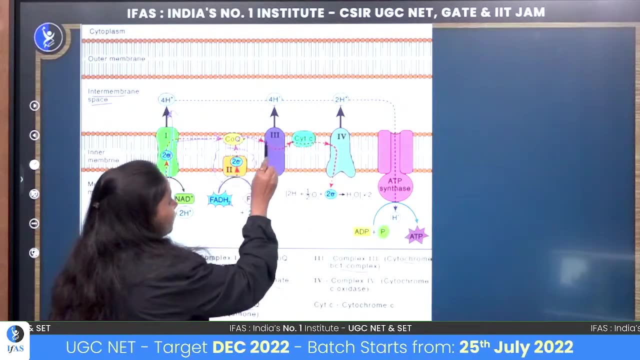 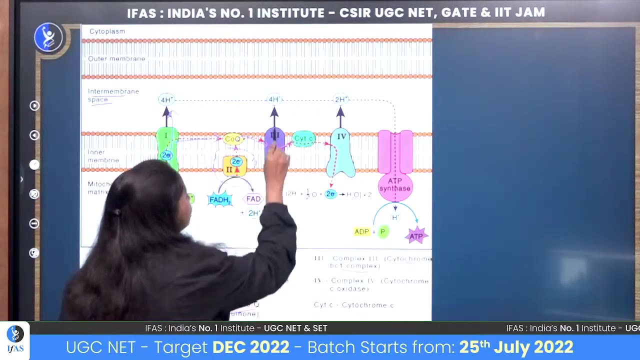 its work is to take electrons from first and second complex towards third complex. this is the work of coenzyme Q. it takes electrons to third complex. and what will happen in third complex when electrons pass to the cytochrome C? again 4 protons pass from here. 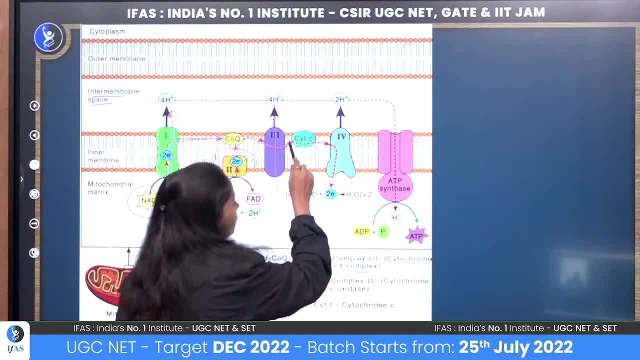 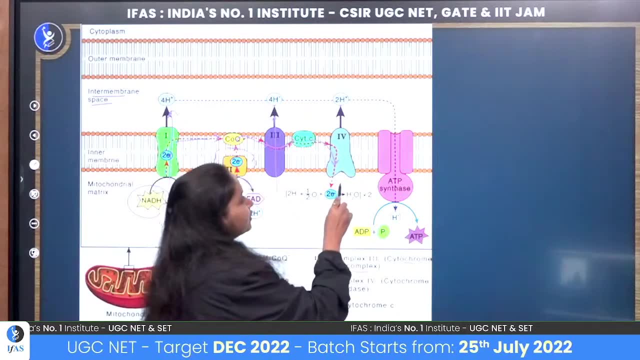 then what will happen? electrons are now given to the cytochrome C. electrons pass from cytochrome C to the complex 4, and when it goes to the complex 4 then also 2 protons pass from here in the intermembrane space. ok, 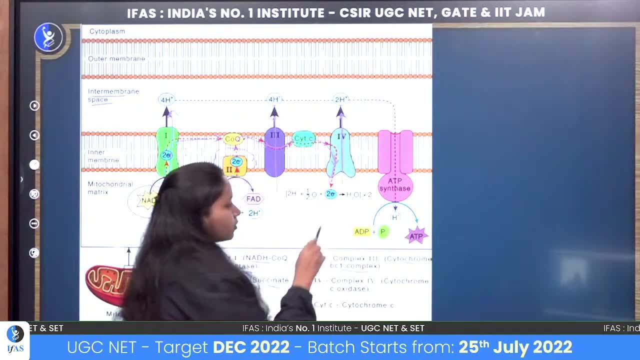 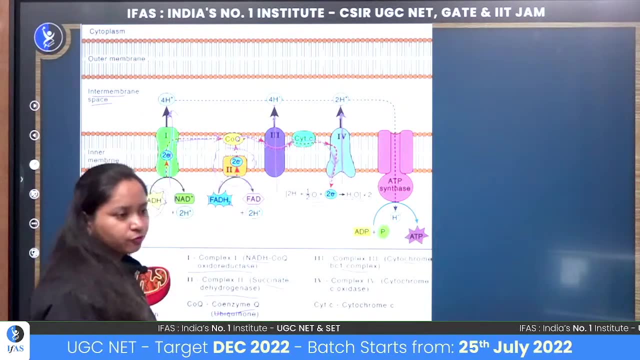 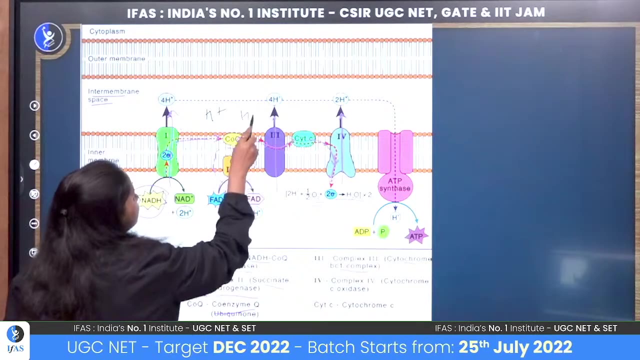 then the electron which is accepting at the end is oxygen. oxygen accepts electrons at the end in the form of H2O. then the end product is formed like this. so what is happening in this pathway? one thing is happening in this pathway: that the proton is accumulating in this region. 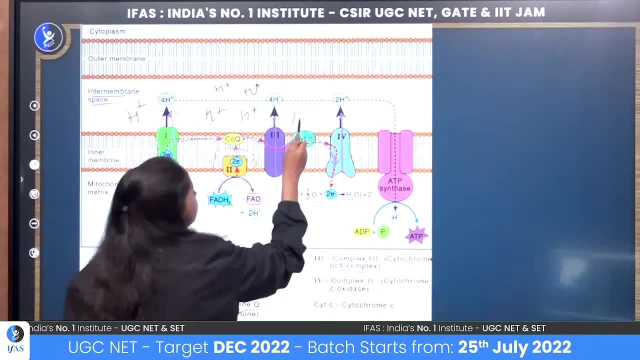 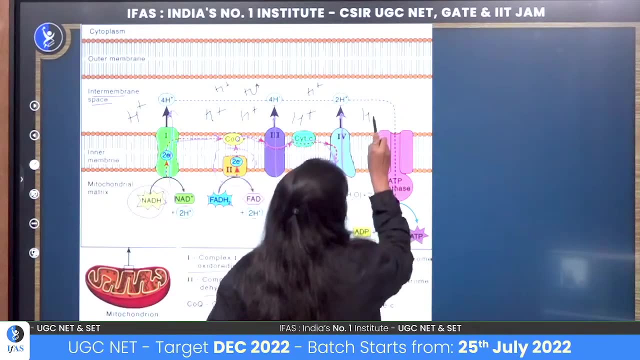 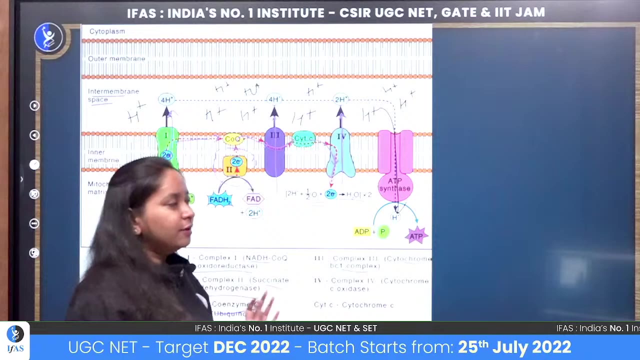 proton is getting accumulated in the intermembrane space. and when the proton enters, when this proton enters in the cytoplasm region, then what will happen? then your ATP synthesis will take place. so when the proton enters from here to the inside, then ATP synthesis takes place. so tell me one thing: how many protons are required to make one ATP? how many protons are required to make one ATP? how many protons are required to make one ATP? 4? Amit is saying 4. ok, Viru is saying 8. brother, we have to make one ATP. 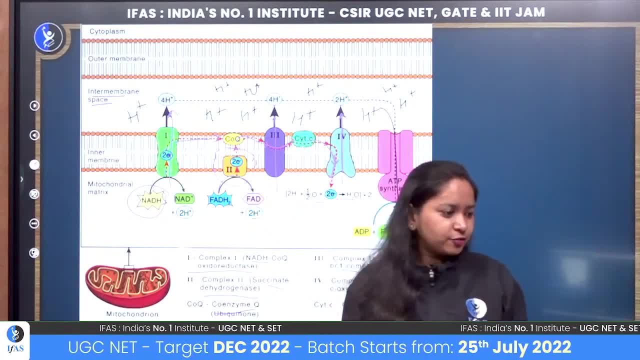 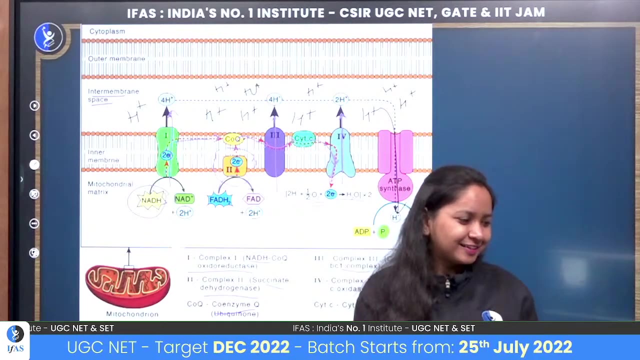 Viru is saying 2 maximum. people are saying 4. ok, ok, tell me how many protons are required to spin the ATP synthesis. Rishi is asking me. ok, son, you will ask me just kidding. yes, ok, yes, Rishi, it is 4 only. so tell me. 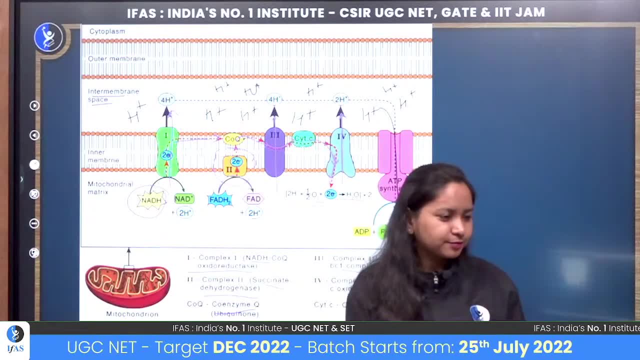 to spin the ATP Synthase. to spin the ATP Synthase, 3 protons. so what is 1 proton doing? why did you write 4? so the ATP Synthase is moving away from those 3 protons. why we are requiring that one extra proton. 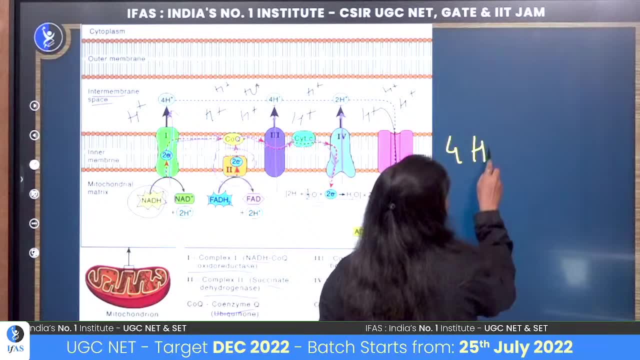 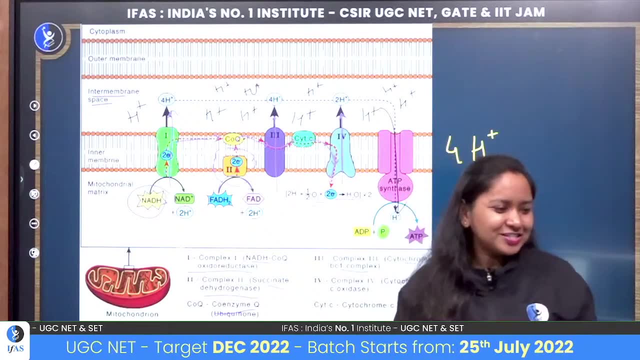 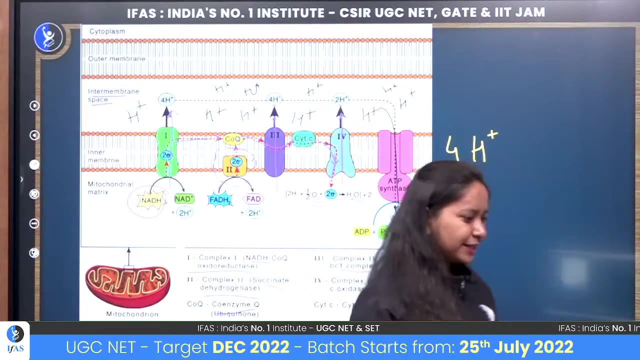 why we are requiring that one extra proton: 4 protons seems to be. you all told us exactly the same. it is ok, Rishi, I am just kidding. you are right, 4 protons are required to make. yes, yes, yes, jagori. I'm so sorry if I'm mispronouncing. 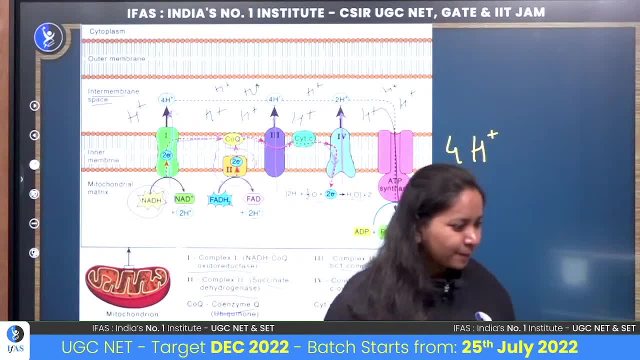 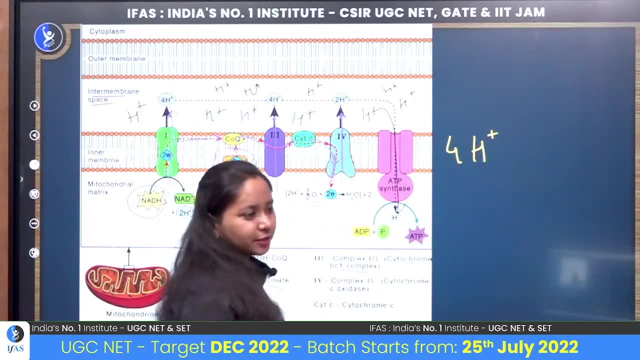 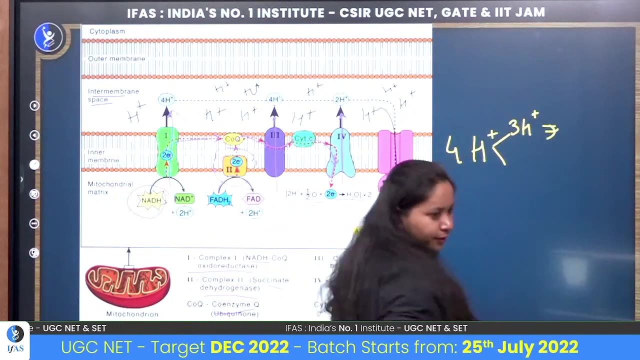 your name. okay, I think it's jagori balance maintenance. no, balance is not maintained. yes, it is required to bring one inorganic phosphate inside. okay, see what happens. 4 protons are required. 3 protons are required to spin the pump. it is required to spin the pump to pump. 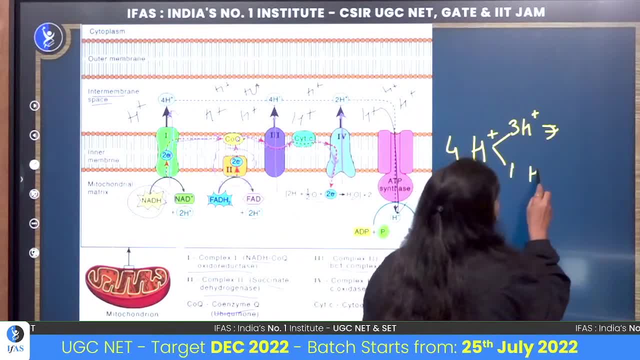 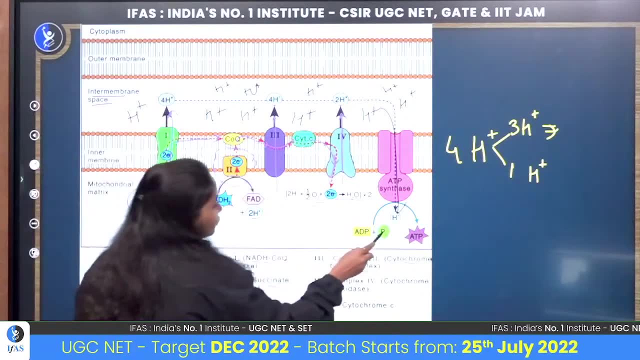 the other one, it is required to pump the s dungeons, but when you think of one proton, it takes us to bring the inorganic phosphate inside. okay, so in your reaction, where it is used, how this inorganic phosphate is coming here. so there is another pump present in the 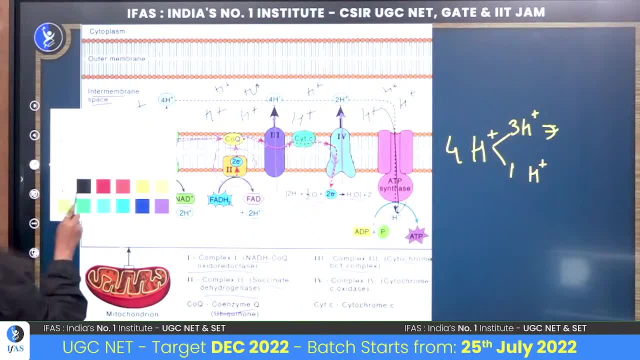 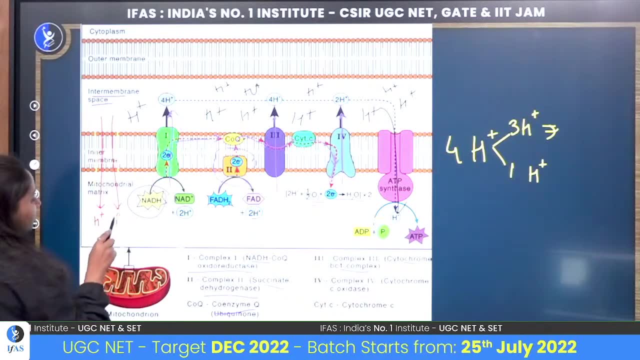 membrane. there is one more pump present in the membrane, and what happens here? so here, when a proton comes in, with that, your one inorganic phosphate also comes in right. so yes, if we talk about totality, you are looking at one proton, so that the one proton comes. 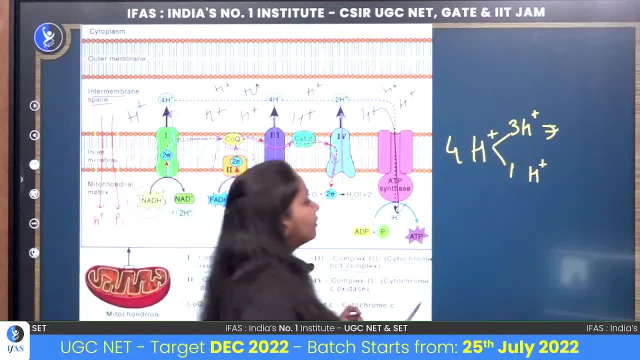 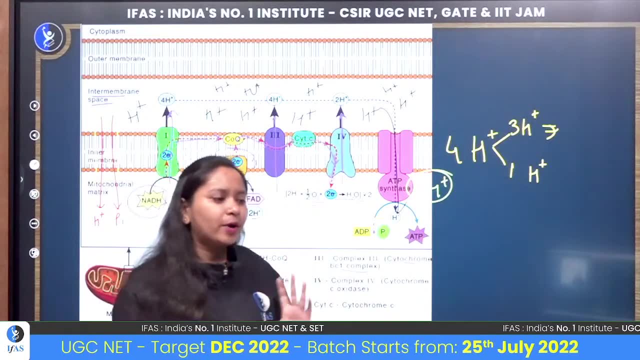 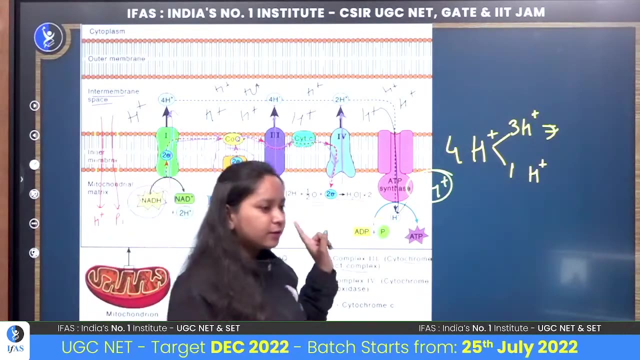 in here. so it is a very important thing to understand that it comes in and you are not to bring inorganic phosphate and three protons are required to spin the ATP synthase. that's why we say that four protons are required to basically perform this ATP synthesis. okay, now tell me from one NADH molecule. 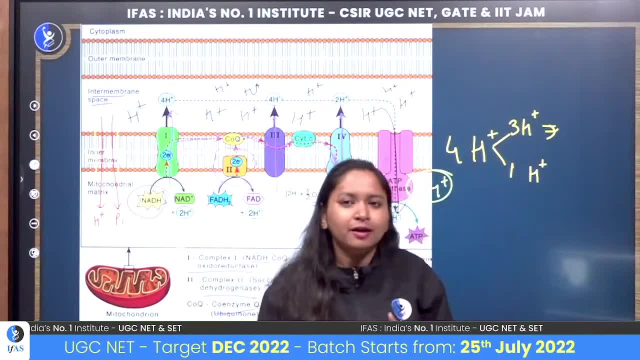 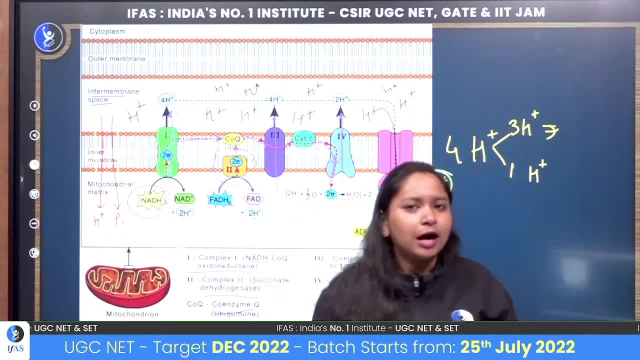 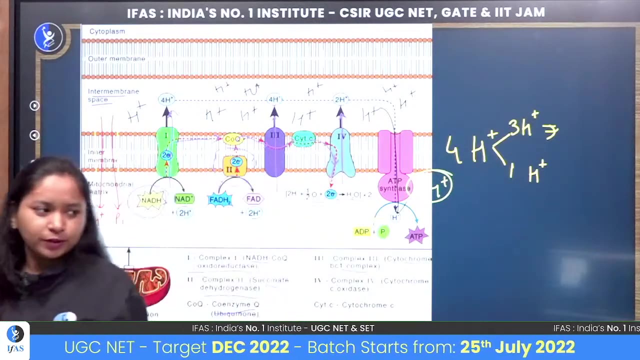 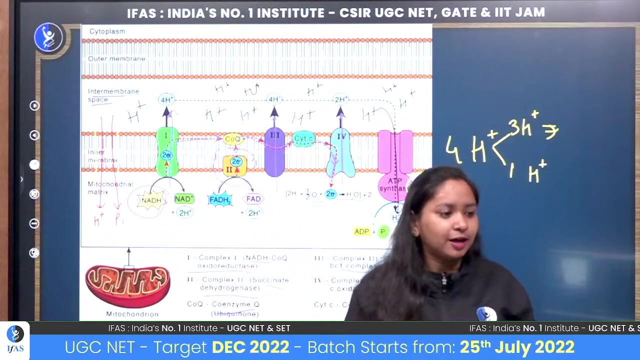 okay, not NADH. let me tell you this first: see, our cycle runs completely once. if our entire electron transport chain is running once, how many ATP can be made, how many ATP can be synthesized by this one electron transport chain- transport, say, or just one pathway? how many? no, no, no, no, we are not talking about glycolysis. I am only asking you. 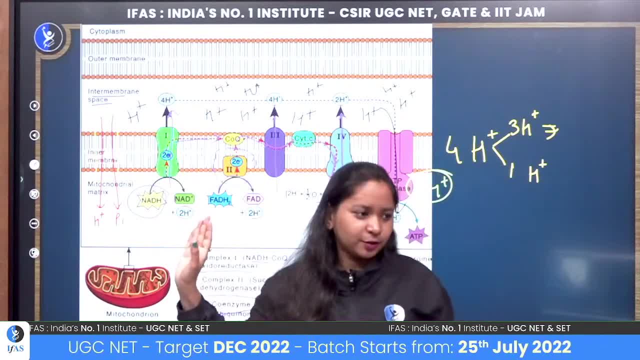 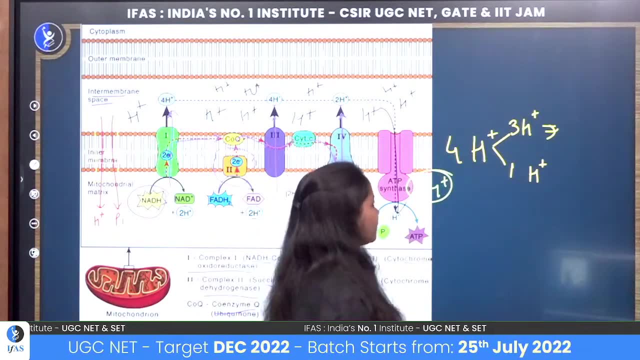 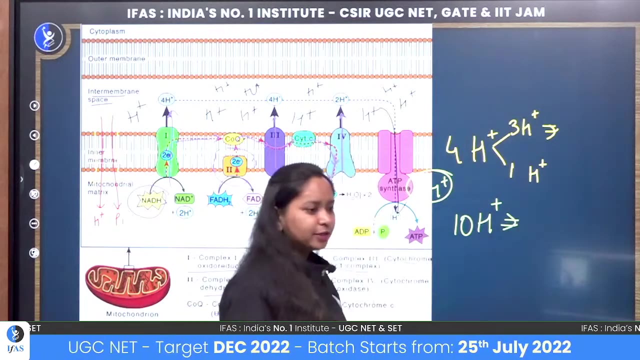 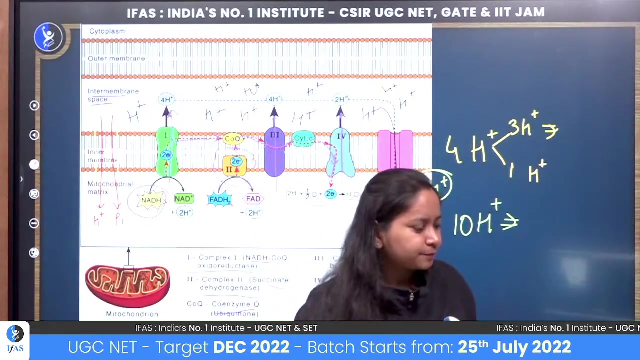 that, even if it runs across this entire pathway, I am just talking about it. we are not talking about your NADH. oh, no, no, no, you are going too far. wait for a while, be patient. 10 percents from here. protons are coming from it. How many ATP will be formed from it? How many ATP will be formed from your 10 protons? 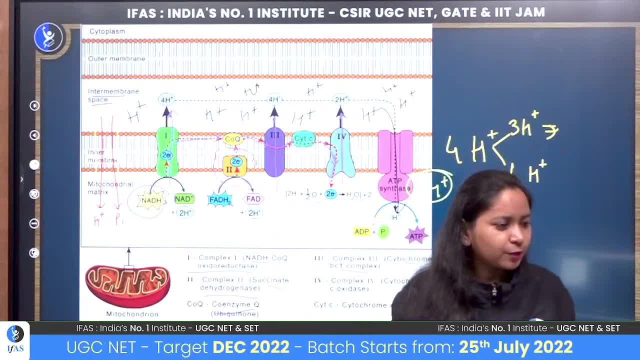 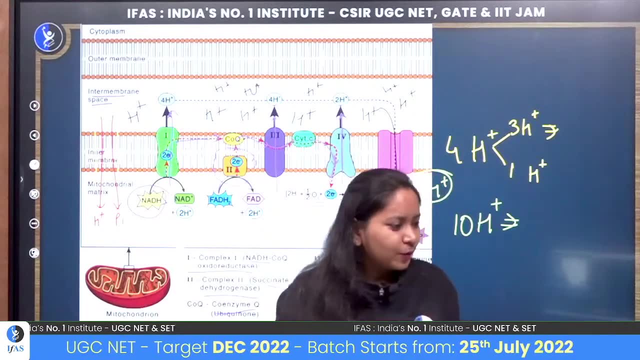 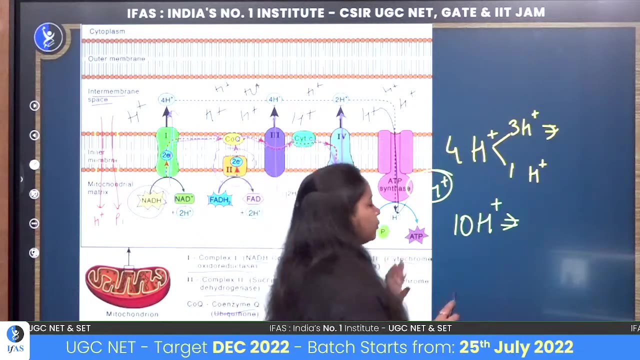 Yajur is saying 2.5.. Tano is saying 2.5.. Yes, I think Yajur is also new to the session. Jagur is also new to the session. Welcome to the session, kid. Okay, 2.5, 2.5, yes, yes, yes, you all are right here, Because if your ATP is formed from 4 protons, its 1 ATP will be formed from 10 protons, so 2.5 ATP will be formed. 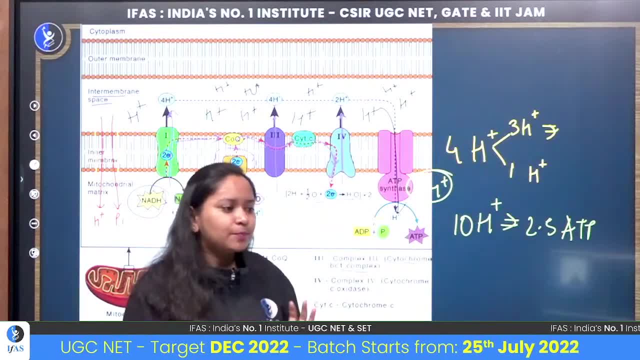 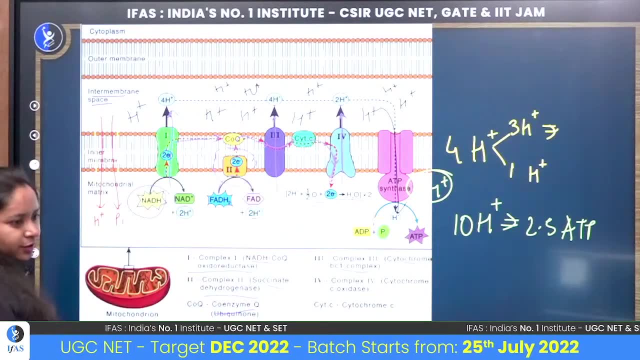 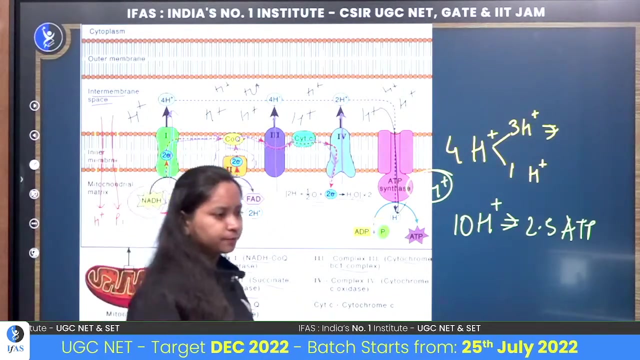 Okay, Now tell me one thing. Suppose there is an inhibitor. It is an inhibitor which have come and inhibited our COS complex. There is one inhibitor which have inhibited our COS complex, So will it make any difference for ATP Synthesis? Will there be any difference in ATP Synthesis if the complex 1 is inhibited? 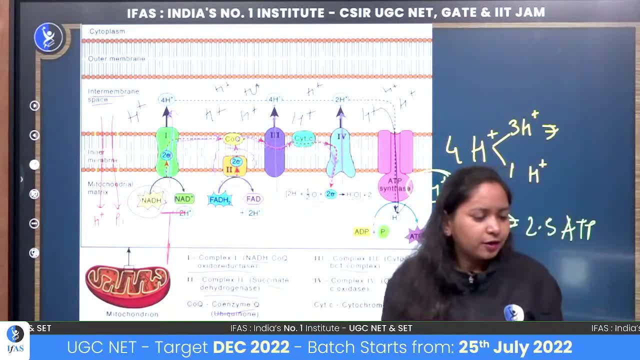 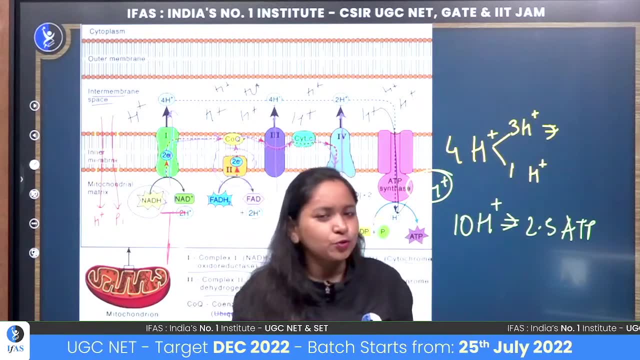 A warm welcome to everyone who is joining the session for the first time And children, those who have not seen the previous session. I request you all to go and watch that session. once We have studied bacteria, virus pathogenic organisms, we have also discussed Microgenetics. 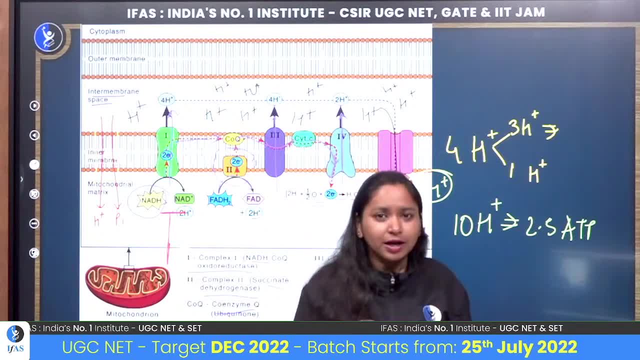 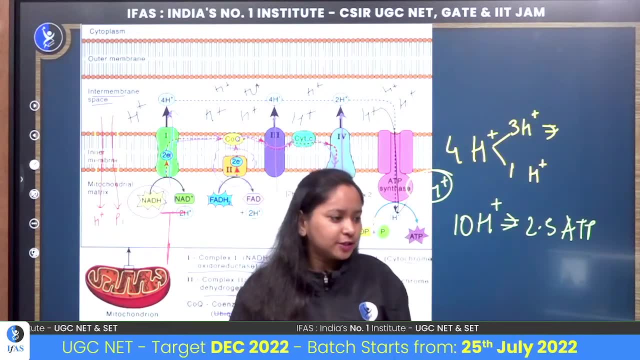 Yesterday we also studied very important techniques and we also practiced questions which you are asked directly in the exam. They ask you very simple questions through detecting and it gives you a lot to understand. You just have to do this much that you can go and play the sessions in fast forward, but at least you have to watch the session once. 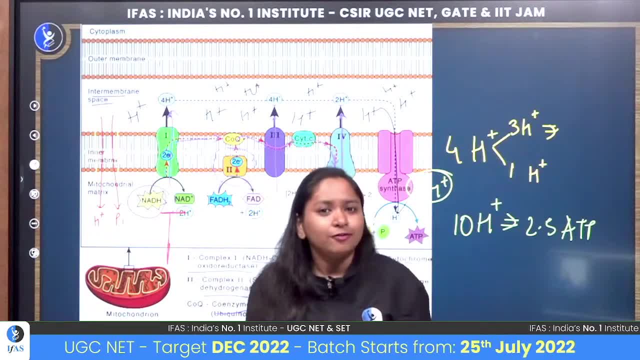 Just watch all the sessions in which we have studied in great detail In virus. we ask you questions like: in which class does the virus belong? In the last lesson I gave you a list properly that you have to study: which disease is there? what disease is happening? 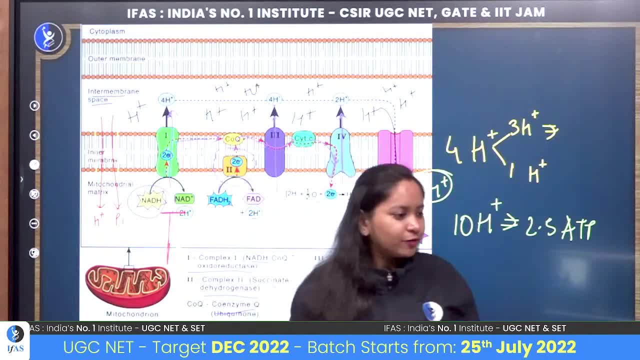 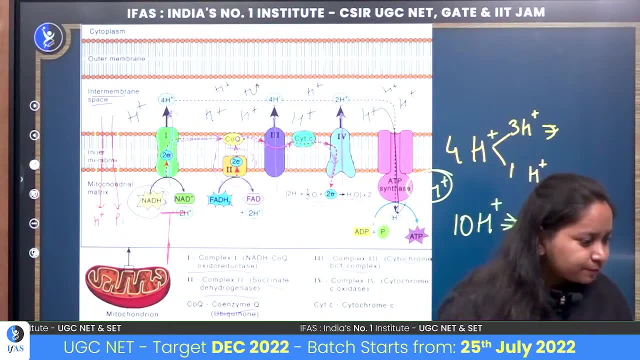 symptoms are there and so on. We can ask the same question from there. So I request you all to just watch that session once. Okay. so Viru is saying 0 ATP. Vagdevi is saying will not continue further. Samadhi is saying 4 protons will not be available. 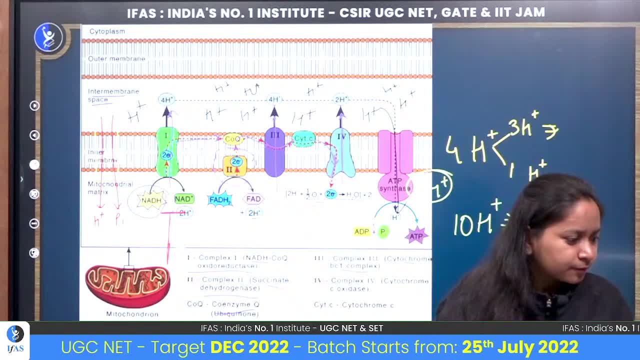 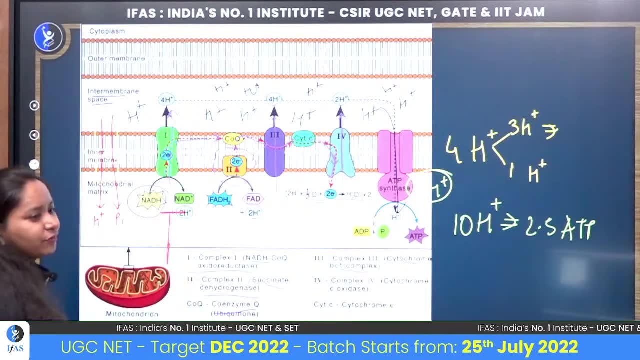 1.5 ATP will be made. Okay, let's go. So, yes, the people who are saying 1.5, Yes, you are right. See, complex one is inhibited. If complex one is getting inhibited, What will happen? FADH will remain present in the cell. 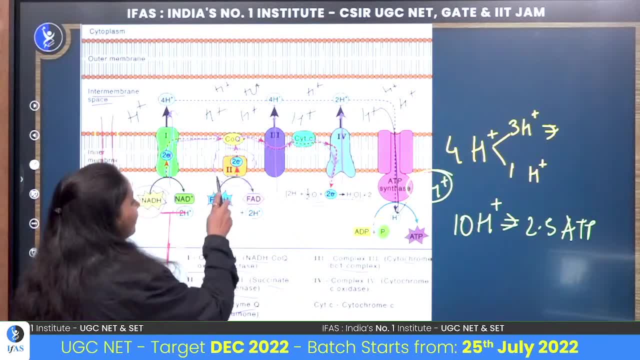 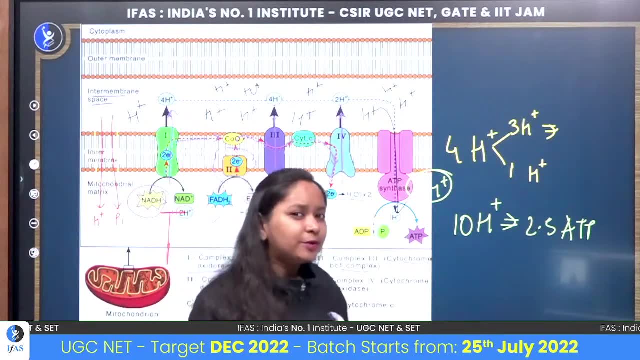 FADH is also present. Your second complex is also present. So what was the problem in not sending electrons further? Right? If complex one is getting inhibited, what will happen? Complex two is present there. Complex two can start. Yes, Samad, you said that. 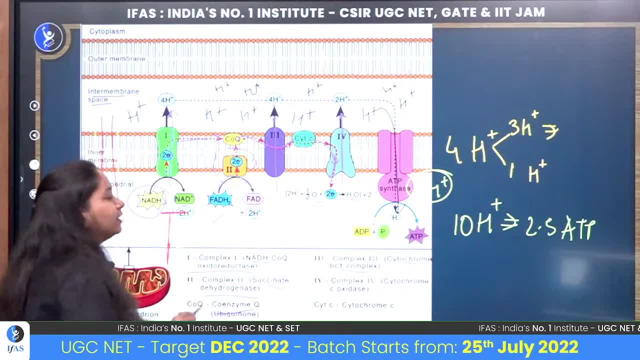 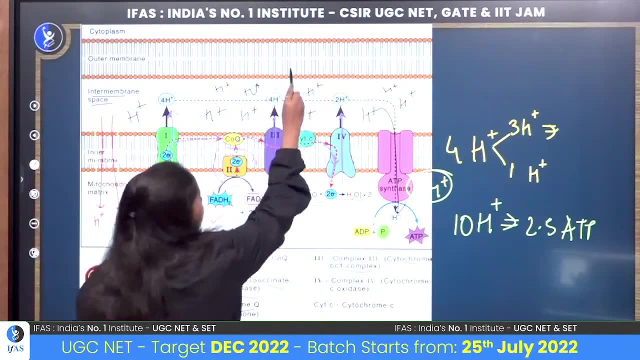 Complex two is present. So what can complex two do? It can start the electron transport chain And, yes, electrons will remain And will continue to be transported. And your only 4 protons, 2 protons, We will only make 6 protons. 6 protons will basically move. 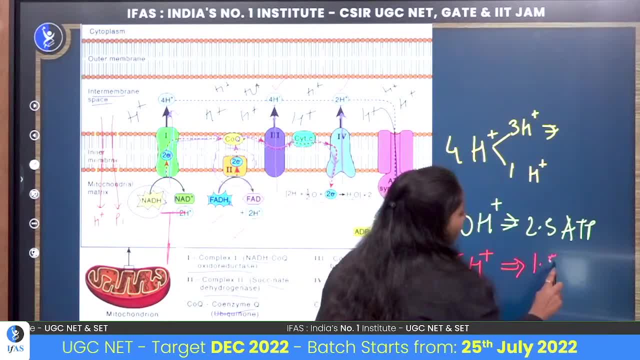 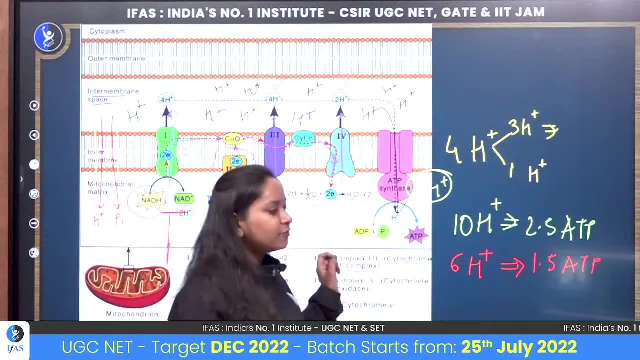 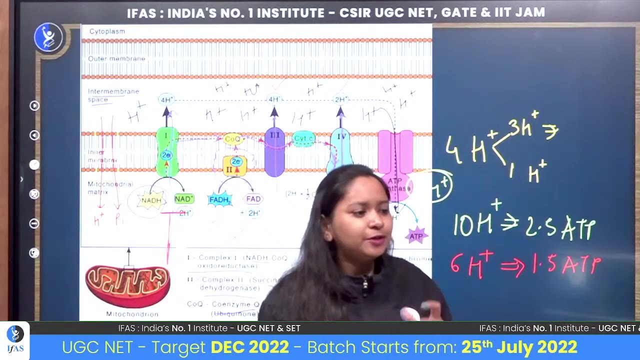 And if 6 protons are moving, Then we will make only 1.5 ATP. Okay, so in case if the complex one is inhibited, What will happen? Only 1.5 ATP will be made. Okay, is it clear to everyone? So there are many inhibitors. 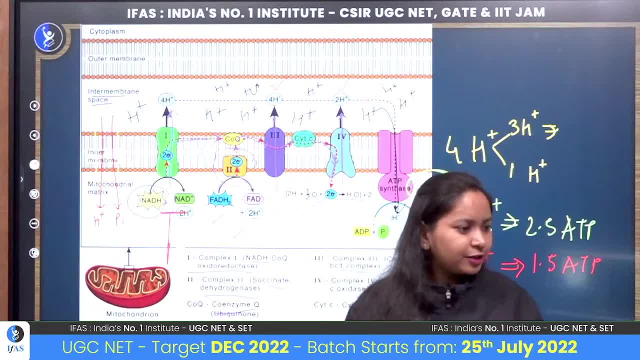 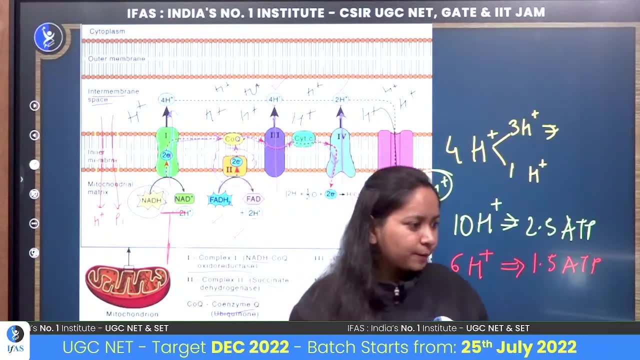 Which can inhibit your different complexes. They will inhibit the complexes By which our ATP formation happens. Pathways never stop, But some things can happen here and there. Okay, So this is the electron transport chain. Everyone understands the mechanism. What is happening? Protons are going that way. 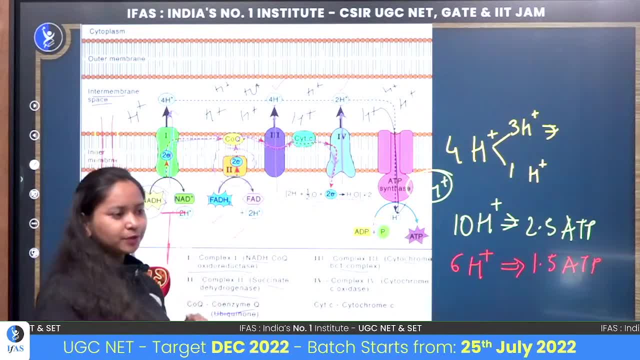 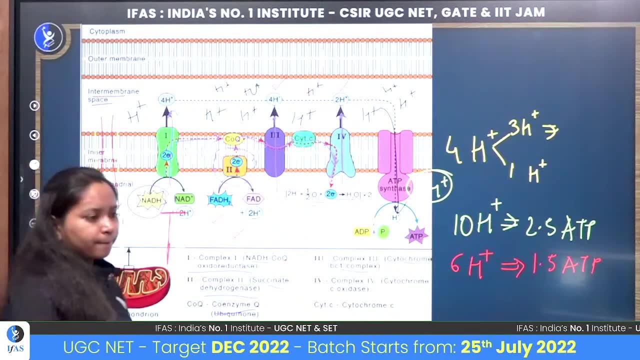 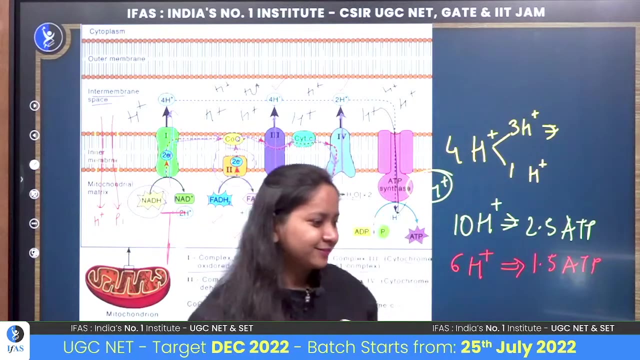 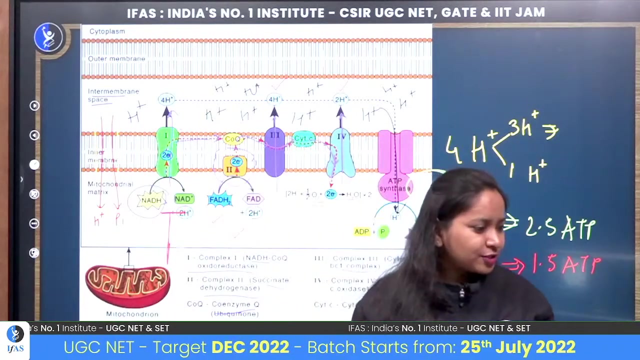 Gradient is being formed When they come inside. So here is the synthesis of ATP. Is it clear to everyone? You have understood the electron transport chain. I, I captain. What is that? Amit? Okay, so, Veeru, In the end of the session, I will just 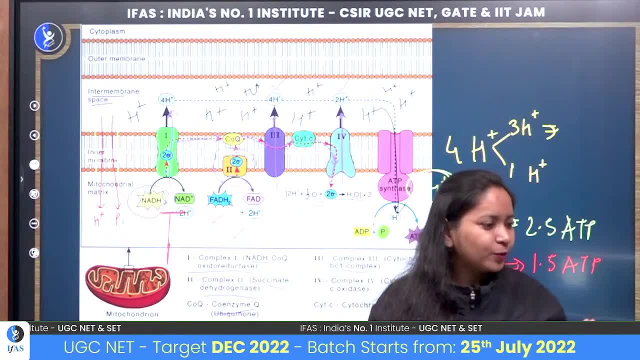 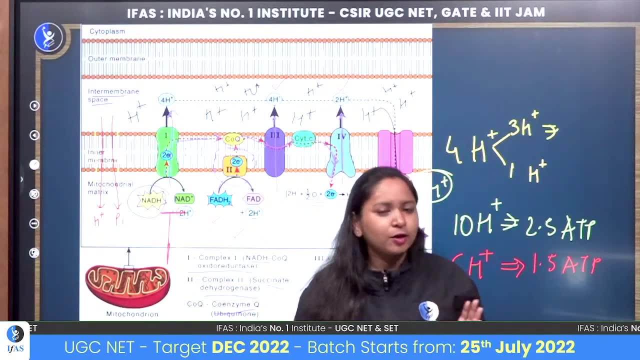 Actually I don't have a proper list. I have a proper list. You can search the list as well. You will get in many books as well. There are many inhibitors. actually There is oligomycin. There are many inhibitors Which can inhibit your every complex. There are inhibitors for ATP synthase. 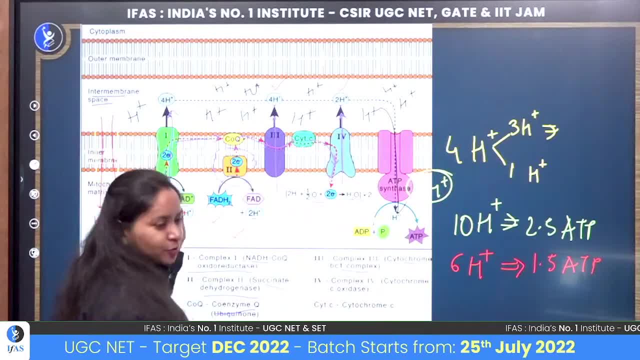 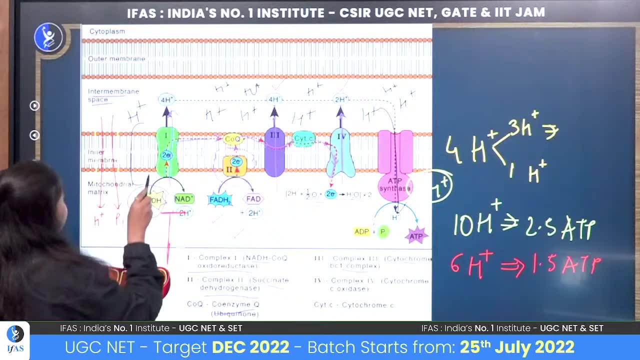 Some inhibitors can be inhibited. Complex inhibitors are also present. There are some uncouplers as well. Do you know? there are some uncouplers. What do uncouplers do? They bring the protons here like this: There are some uncouplers present And what they do? 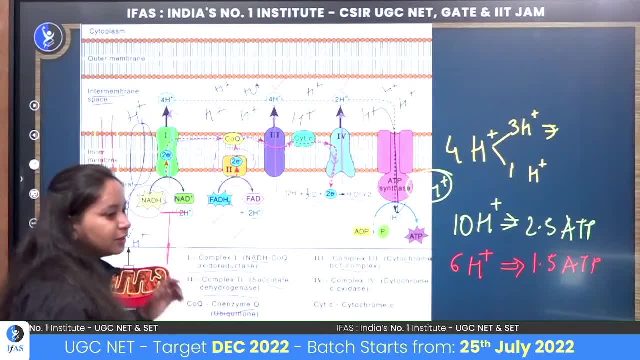 They will bring the proton in the matrix Or in the cytoplasm only. What will happen with this? If the protons start coming like this, What will happen Here? the gradient will not be maintained. And if the gradient is not maintained, What happens with that? 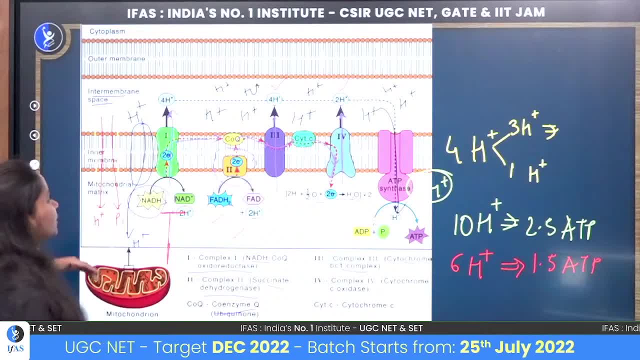 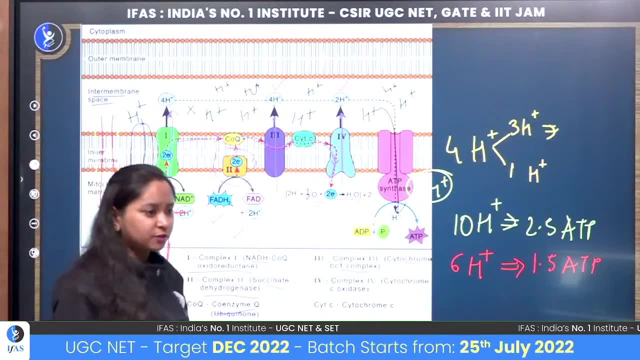 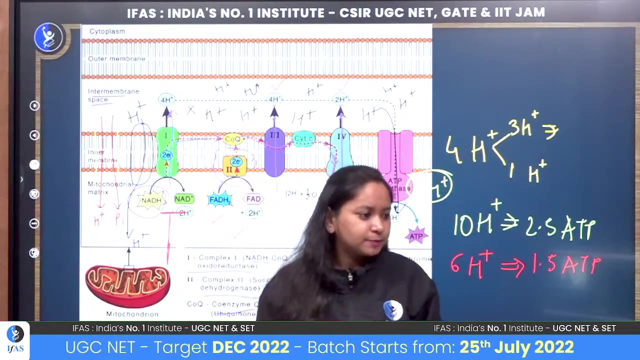 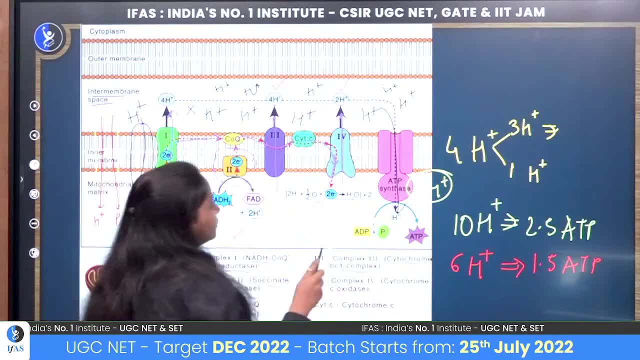 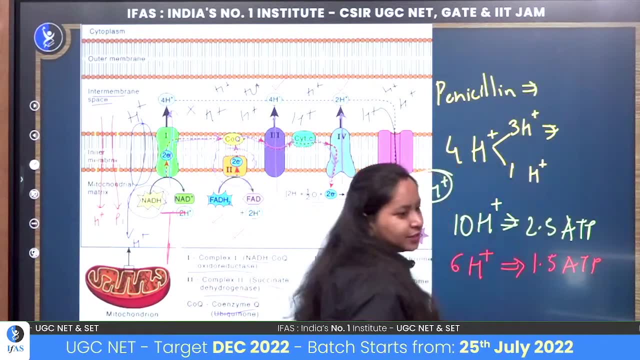 In this case? Ok, This is penicillin inhibitor, But it is not inhibitor. Oligomycin is there? Yes, Penicillin inhibits the transplant peptide. Penicillin at your When the penis Abbott Exist? Okay, Penicillin inhibits Whom has the name which is transpeptide. 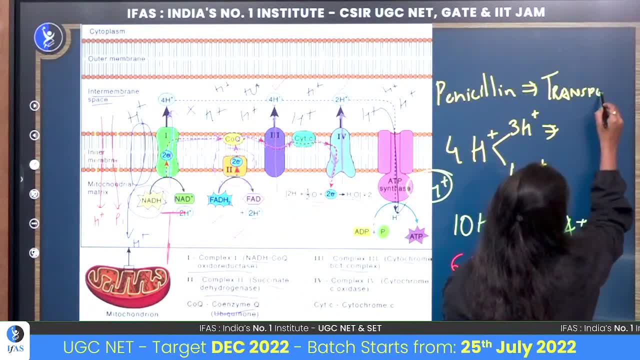 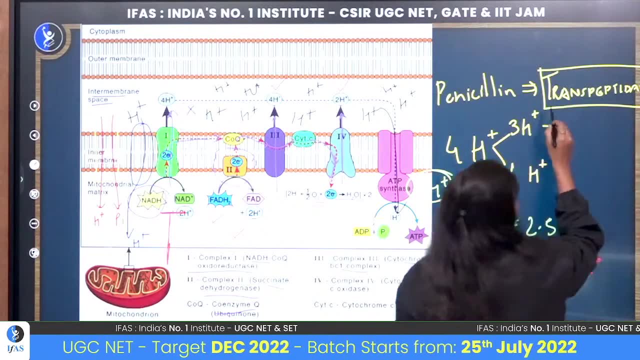 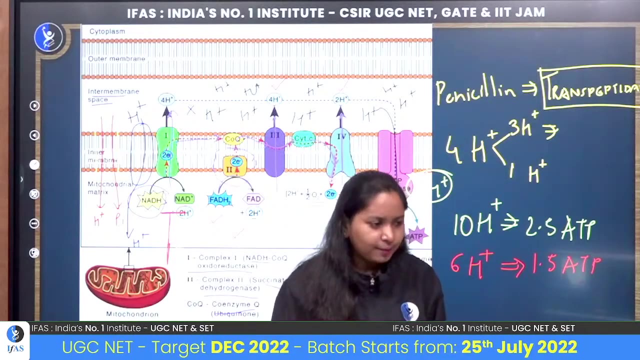 What is the function of transpeptide? Who will tell you No, 9, 9 And when it is inhibited? Now you also know No penicillin, What? I took a session in which I told you what is transpeptides. We took a session. you can search the session. 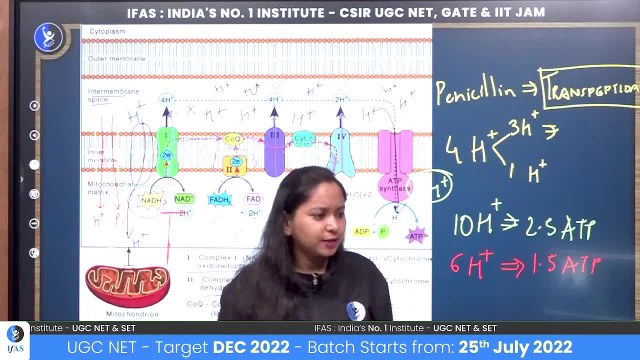 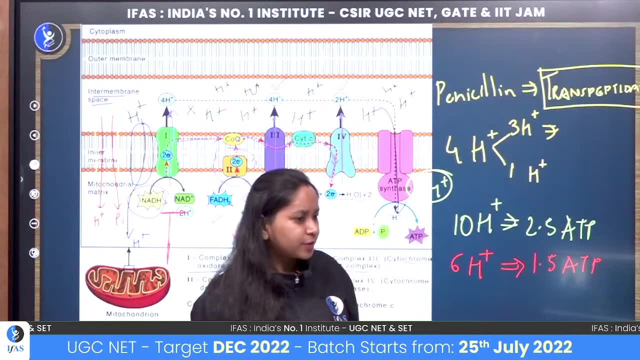 I think the session was taken last week. this is my session In which we discussed that we had read all your antimicrobial drugs, So you can see in the session what penicillin does. It is an antibiotic. it inhibits the enzyme transpeptides. 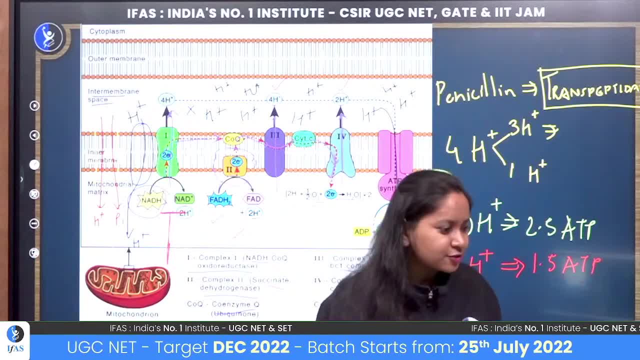 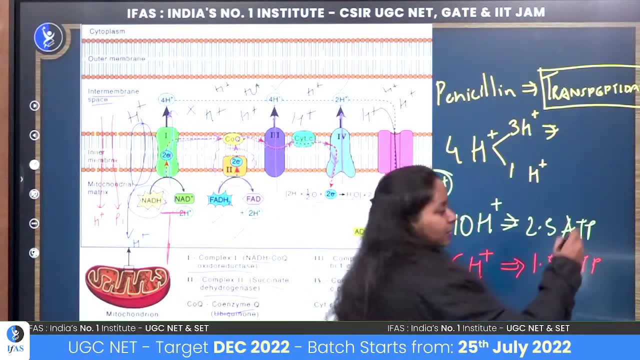 Yes, yes, yes, yes. so see the kids who are consistent in the sessions: Samad Rishi Atanu. yes, because you have attended the session, you know that very well. So the work of transpeptides is to cross-link. 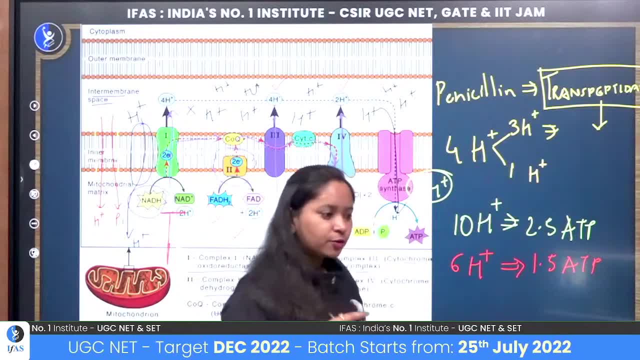 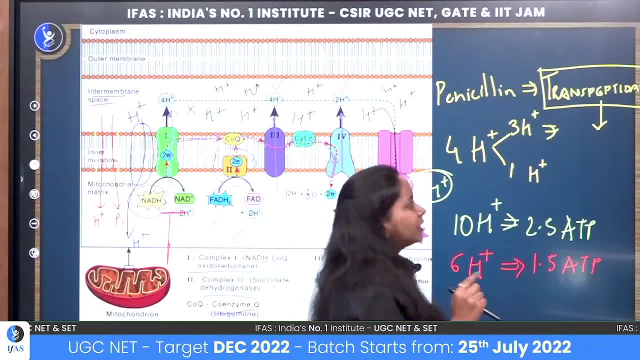 Its work is to cross-link your bacterial cell wall properly. And if cross-linking is not possible, then what will happen? If penicillin comes, inhibits transpeptides, then there is no cross-linking. If there is no cross-linking, then what will happen? 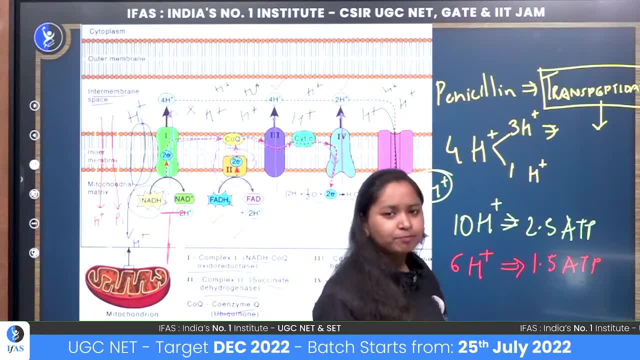 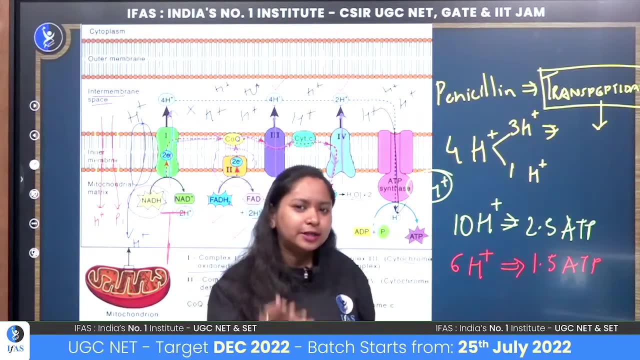 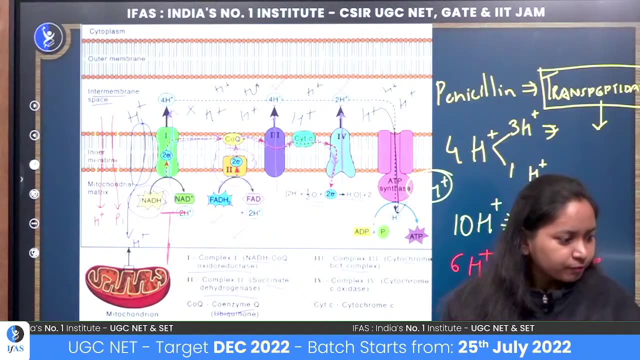 There will be a very weak cell wall in it. its cell wall will not be very rigid. If there is no rigid cell wall, then there is an osmotic imbalance And bacteria ultimately die because there your cell wall will be lysis, Cell wall will degrade. there is osmotic burst. yes, we can say that as well. 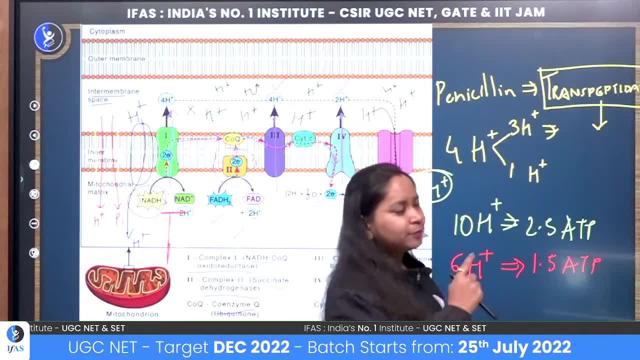 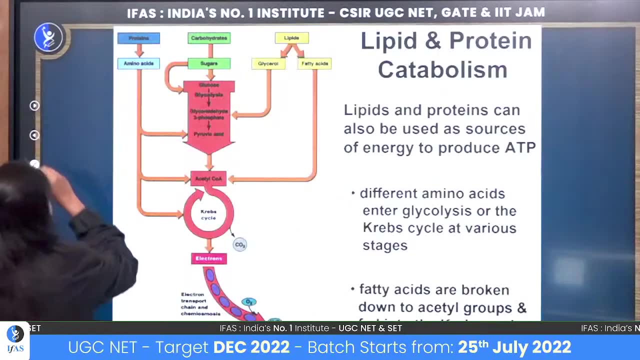 So whatever penicillin you have, it is an inhibitor, but it is not its inhibitor. It inhibits that bacteria stops the formation of cell wall. This is going on in the membrane. So this is an electron transport chain. Now where can we take energy from? 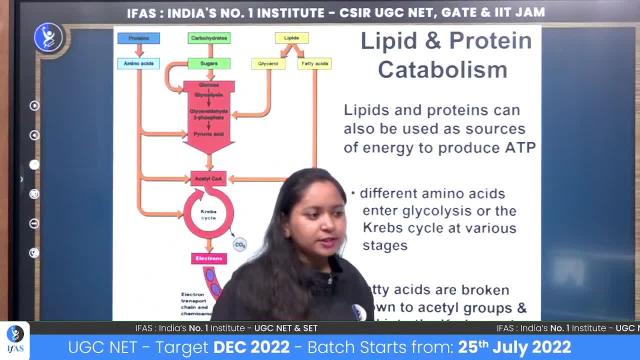 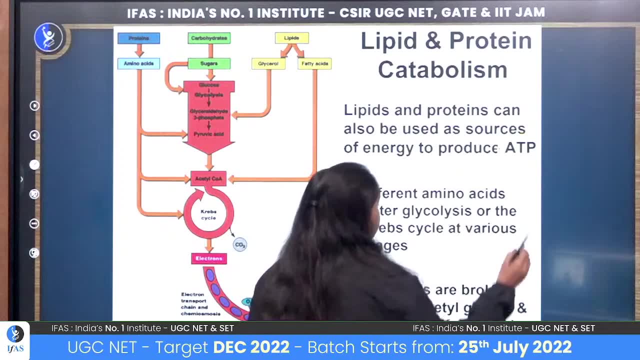 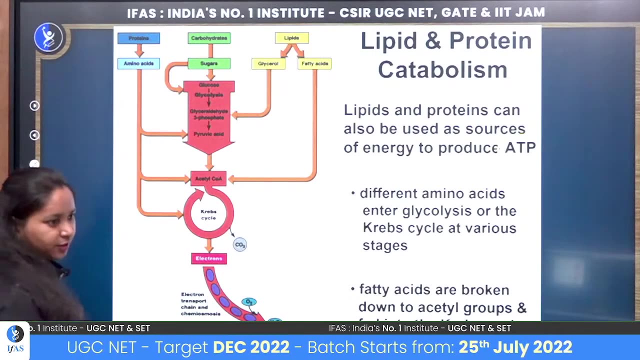 So lipids, proteins, are taken from there. We can catabolize it, we can break it From where. we can get ATP. We can use some amino acids. We can use some amino acids, We can use fatty acids. Whatever happens, whatever energy they can get. 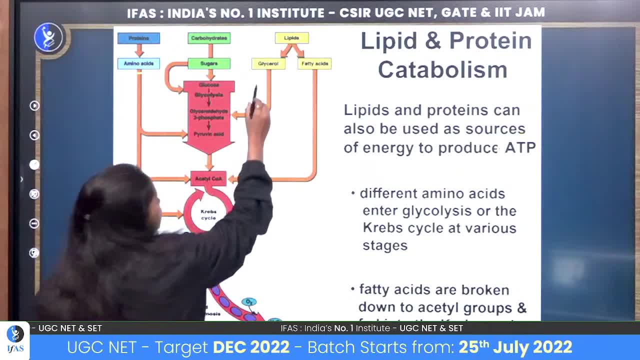 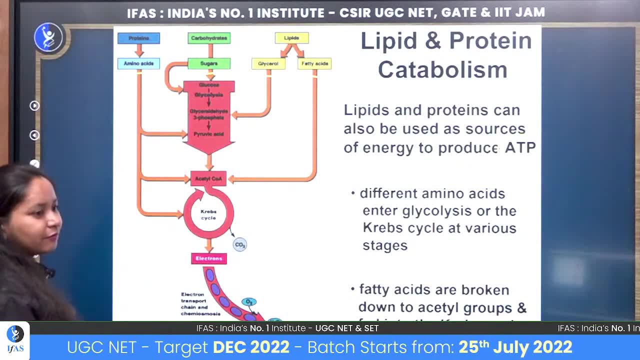 So we get amino acids from proteins. We get glycerol, fatty acids from lipids. We talked about sugars, glycolysis. So what happens to everyone? We can take energy from everyone And every energy can be converted. lastly, to the acetyl coenzyme A. 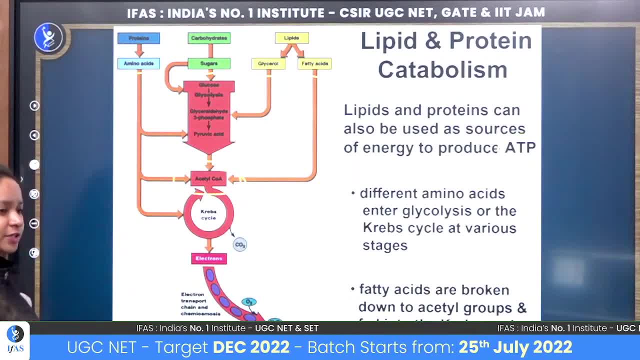 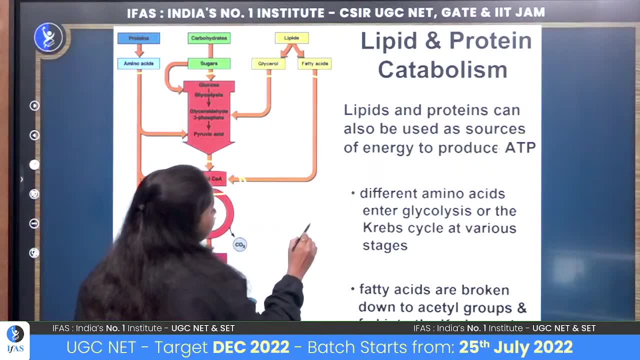 Which will ultimately enter your TCA, From where we will get a lot of NADH And you will get a lot of FADH. It means that we get 2 FADH and 10 NADH, So it will enter into the electron transport chain. 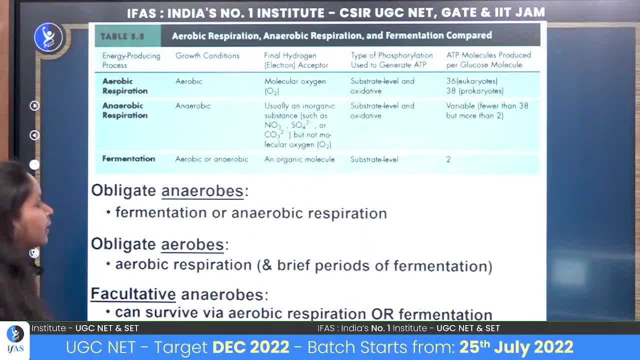 And yes, we will synthesize ATP. Okay Then, yes, lastly, I have this list. If we talk about aerobic respiration, So here the final acceptor of electron is molecular oxygen, Which is your aerobic respiration In aerobic condition. If we talk about your aerobic condition, 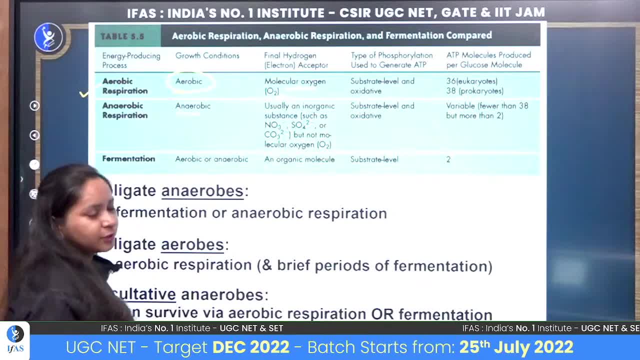 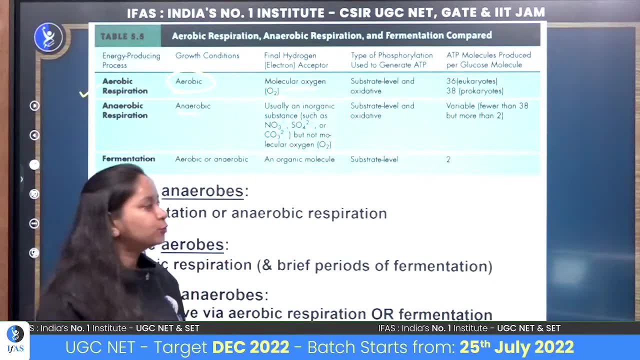 So what happens here? Here different pathways used to run, Here different pathways used to run, Lactic acid used to be formed. Sometimes ethanol used to be formed. So what happens in that case? Whatever ATP generation you have, It decreases a lot. Okay, After that, if we talk about 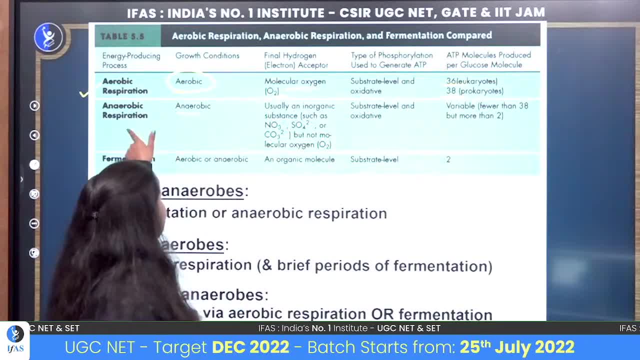 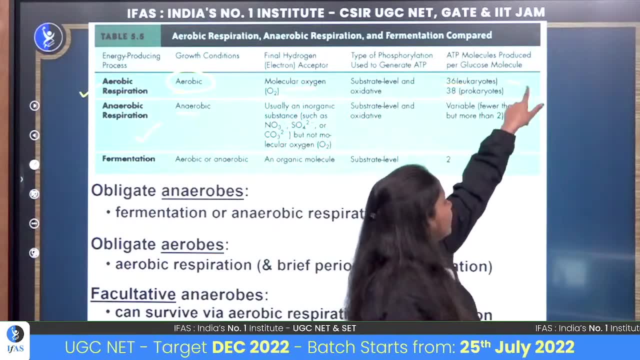 How much ATP is being formed at the end. So in case of your anaerobic, it is variable. Species to species it can vary. But if we talk about our eukaryotes, Your eukaryotes are formed here. Your 36 ATP is formed in prokaryotes. 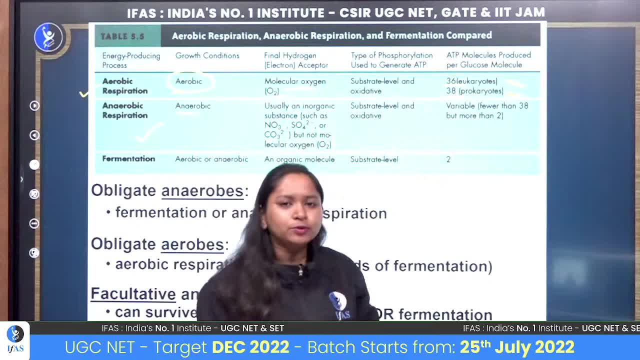 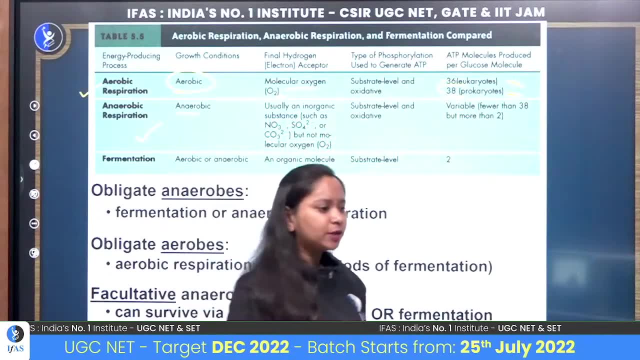 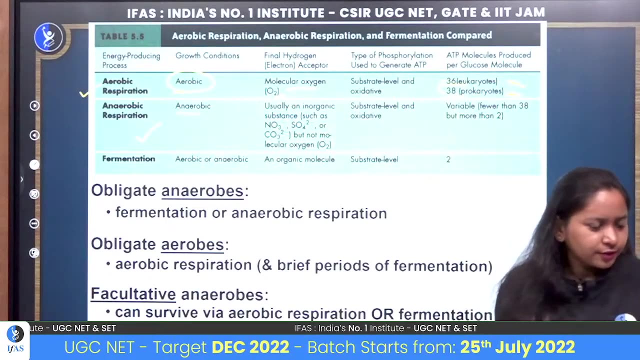 Your only 38 ATP is formed. Why does this happen in prokaryotes and eukaryotes? What can be the reason? Eukaryotes are producing less ATP. 2 ATP is less. Why does it happen like this? Okay, Okay, Janhvi. No, no. I am asking you that, Whatever your eukaryotes are, Only 36 ATP is being formed there. Okay, Eukaryotes have 36 ATP, Prokaryotes have 38 ATP. So what is the reason Why 2 ATP is decreasing? 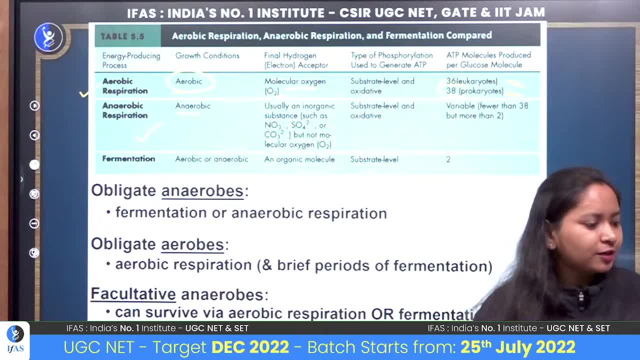 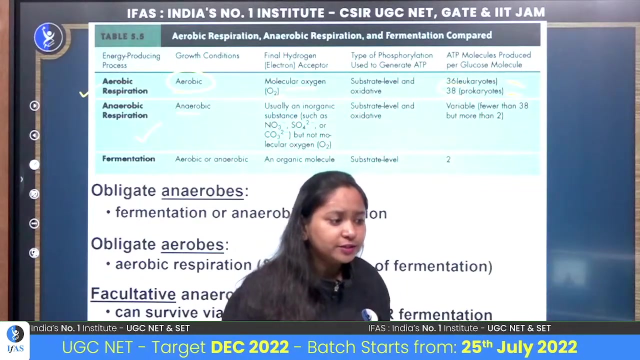 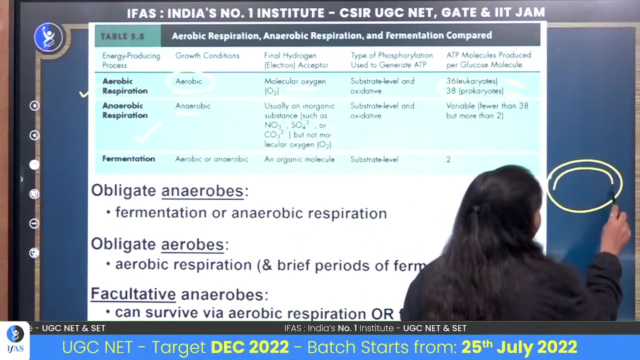 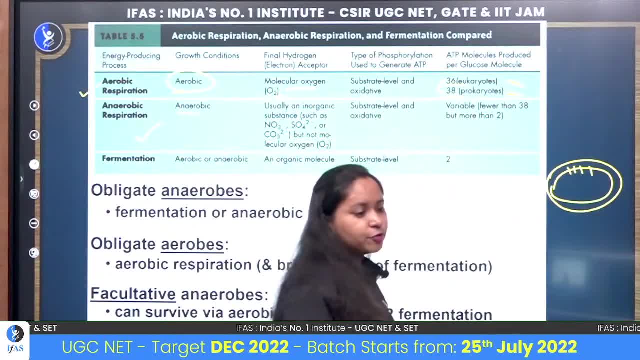 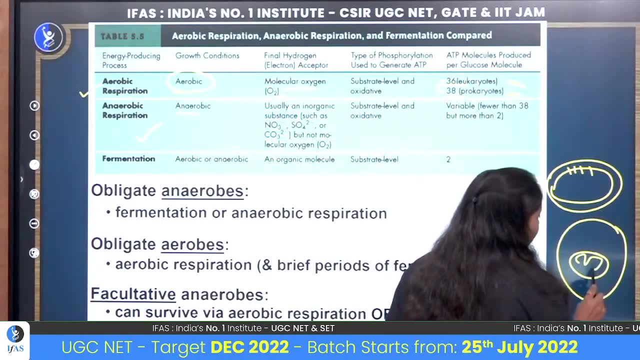 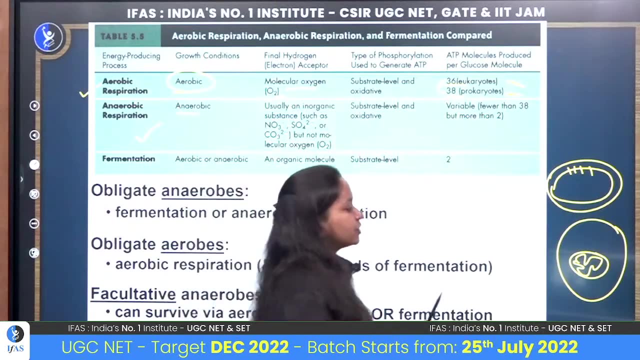 The electron transport chain runs here, If we talk about the animal cells. So what happens in us is that our cell is there, mitochondria is there and our electron transport is going on there right. So what happens in us is that we have to bring some things in from outside, we have to do things inside and out. so there we get 2 ATP extra. We require 2 extra ATP to bring substances in the mitochondria. that's why we minus it there, because we have 2 ATP less in us. So, yes, we make 36 ATP in total, and if we talk about your prokaryotes, so they make 38 ATP, right? 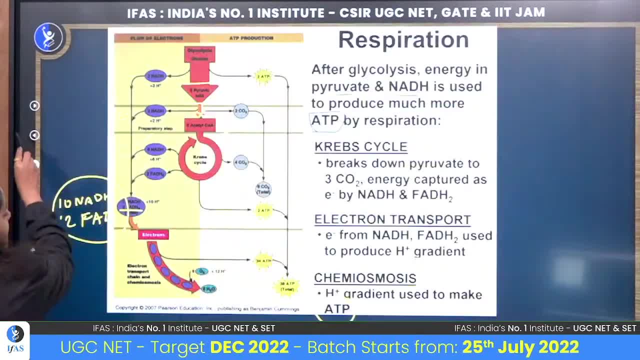 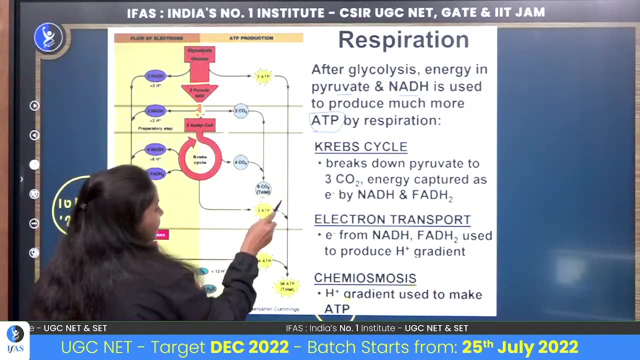 One more thing: where are your 2 ATP made? They are made in your Krebs cycle, right? Look carefully: 2 ATP are made in our Krebs cycle, 34 ATP are made in our Krebs cycle From the CTC pathway- I am talking about 1- glucose- and 2 ATP are made from your glycolysis pathway. 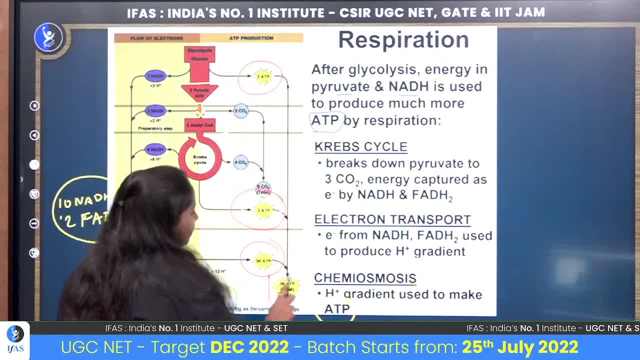 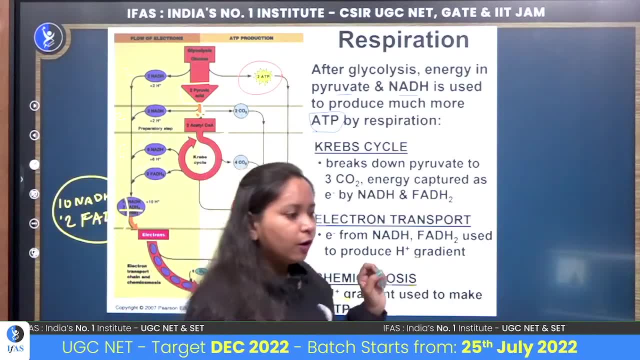 So we are making a total of 38 ATP, right? What are we doing? We are making 34 plus 2 plus 2, we are making a total of 38 ATP. So my question to you is this: how many ATP are made in mitochondria? 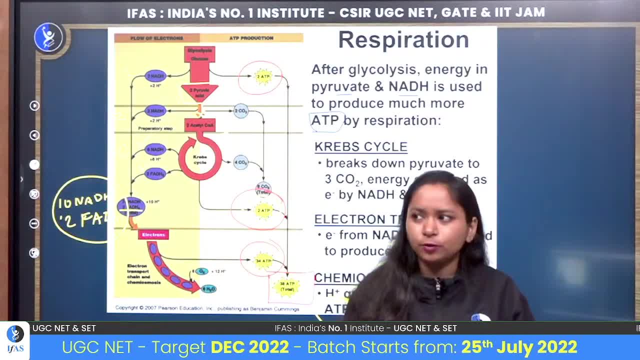 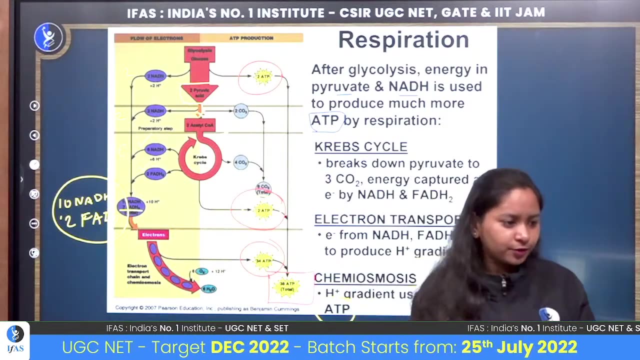 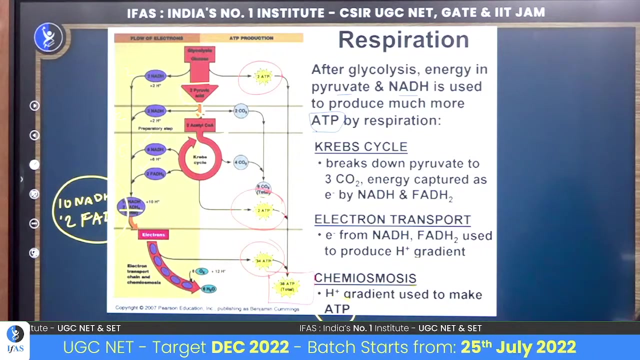 How many ATP are made in mitochondria in case of one pathway, How many ATP are made in mitochondria? How many ATP are made in mitochondria? The question is 36,, 36,, 36,, 34,? okay, 34, 36.. 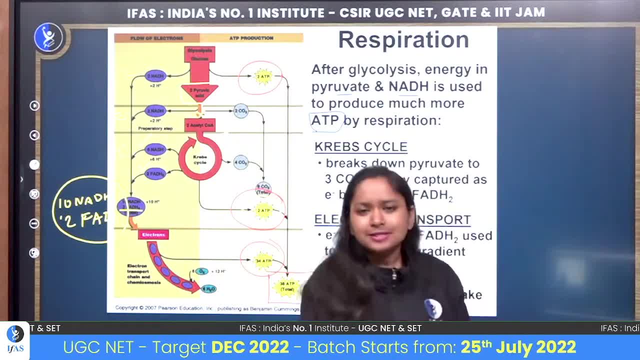 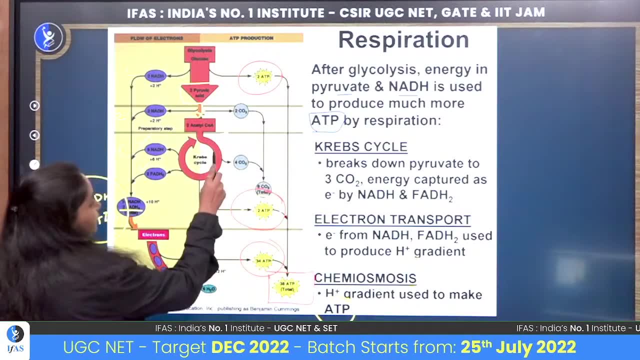 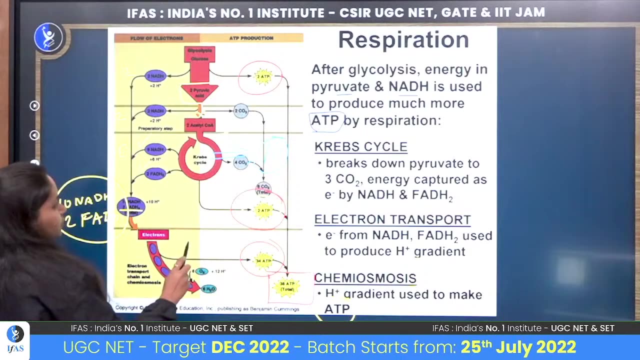 So yes, kids, look where does your TCA cycle run? It also happens in the mitochondria, only, right? Whatever Krebs cycle is running, this cycle runs in the mitochondria. only This cycle is taking place in the mitochondria, and ETC is also taking place in the mitochondria. 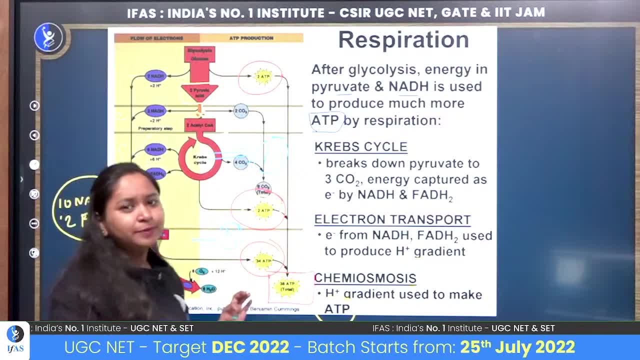 So 34 plus 2 makes a total of 36 ATP in our mitochondria and glycolysis runs in the cytoplasm. Glycolysis takes place in the cytoplasm. Glycolysis takes place in the cytoplasm. 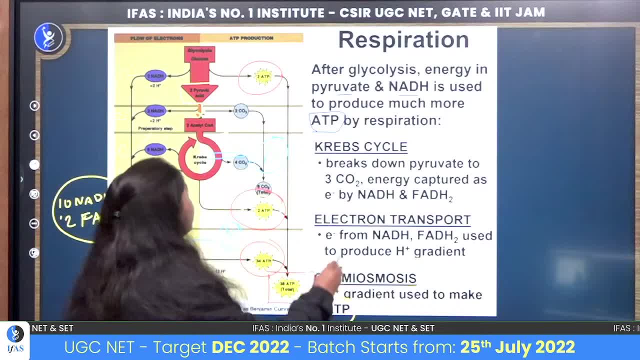 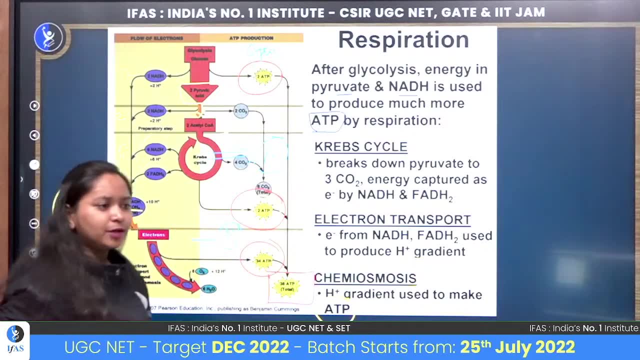 Glycolysis takes place in the cytoplasm. That is why the two ATP that are being made above you are being made in your cytoplasm, And whatever 36 is being made, they are made in your mitochondria. Okay, so what is the question being asked to you? 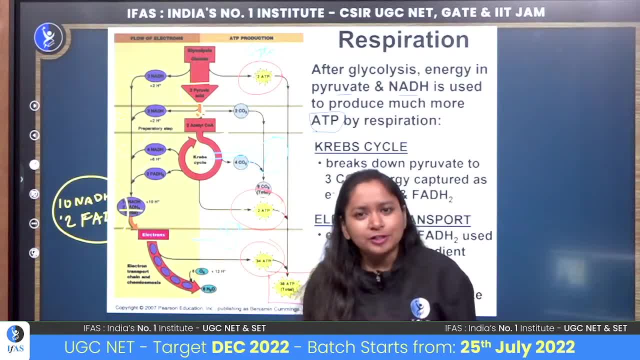 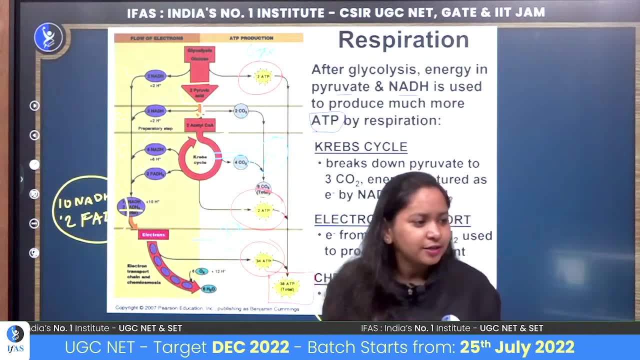 How many ATP are being made. 2 is being made in the cytoplasm, the rest whatever, 36 is being made in your mitochondria, then you should also know these things a little bit. Okay, have you understood what we have read now? 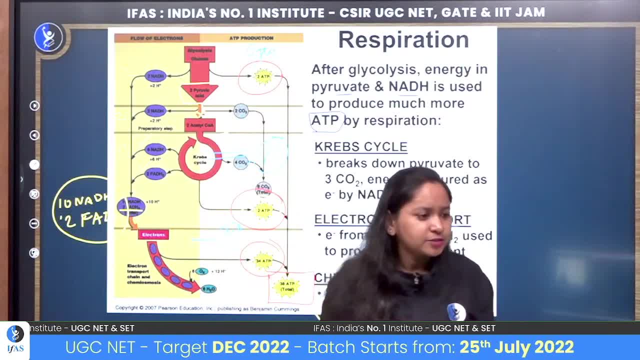 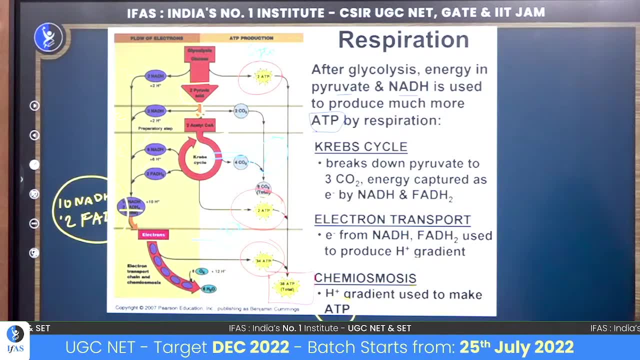 What is 36,, what is 38,? what is 2?? Is it clear to everyone? Please confirm, Can we understand trinus in холодing the compound? Yes, it is clear, And may we include this in our 我的? 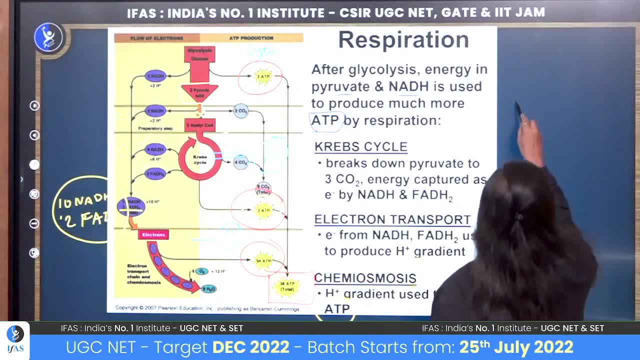 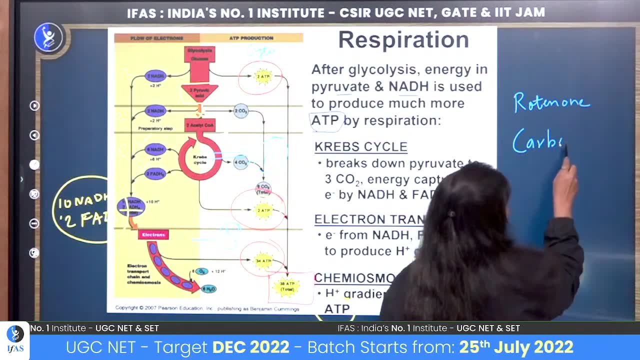 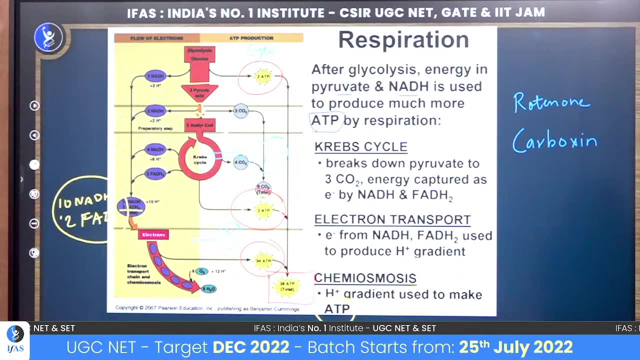 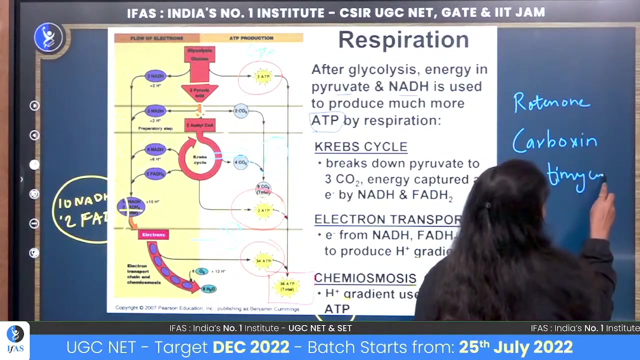 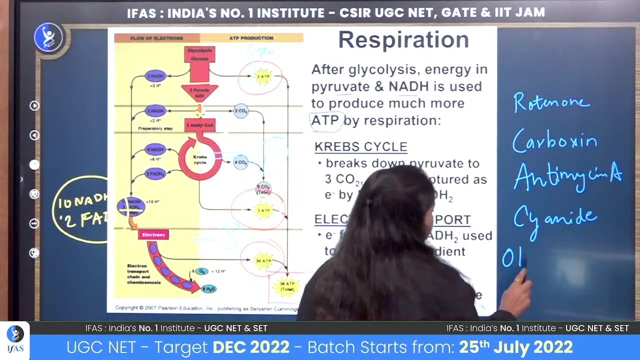 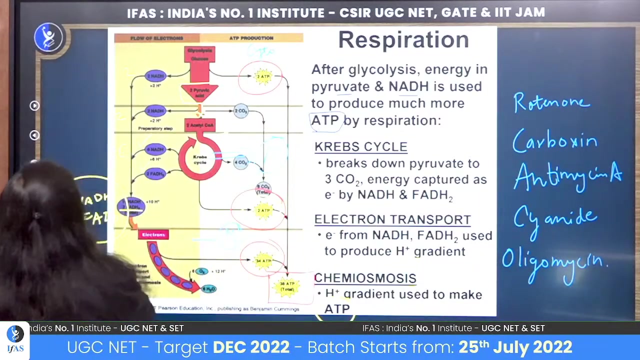 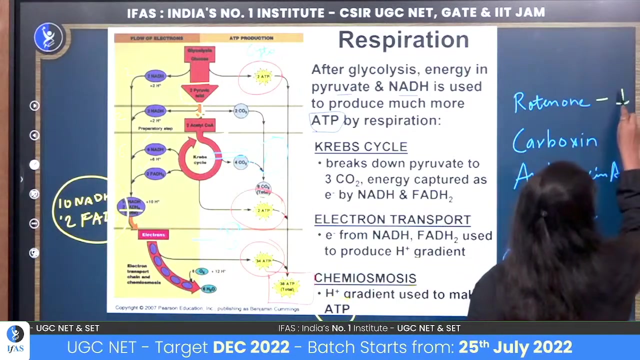 Father, sister, Peru, Brazil, America. Is it blue colour visible to everyone? Okay, These are the inhibitors of ETC. You guys asked me about inhibitors, So you guys can note somewhere Rotinon inhibits complex 1. We are talking about electron transport chain. 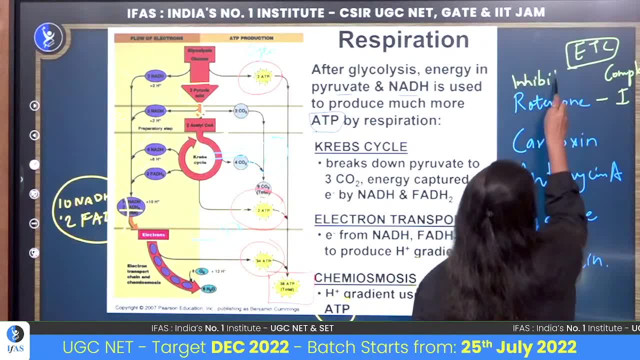 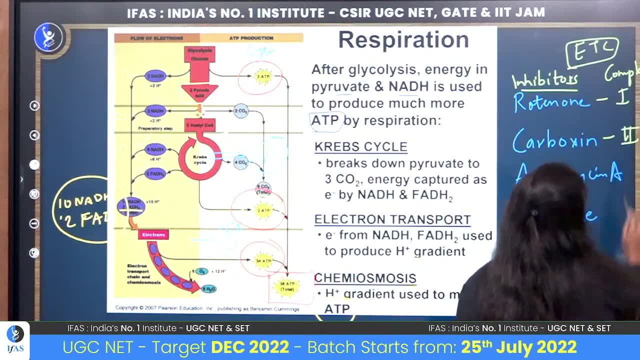 And these are the inhibitors. These are the inhibitors. Okay, Carboxyne inhibits complex. 2. Antimycin A inhibits complex. 3. Sinal inhibits complex 4.. Also, Helicobacillus inhibits ATP synthase 4.. 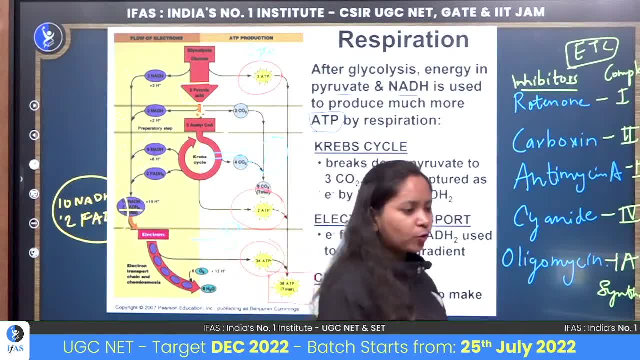 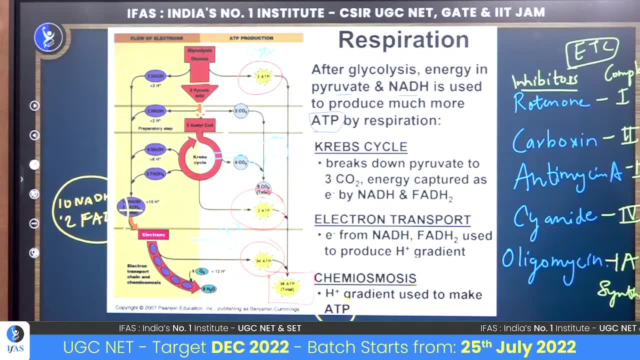 Okay, There are many more inhibitors. I have written the common ones. You can just note it down in your copy or something. Yes, Yes, Azine. Azine also inhibits complex 4.. You can mention that, But you will also see that. 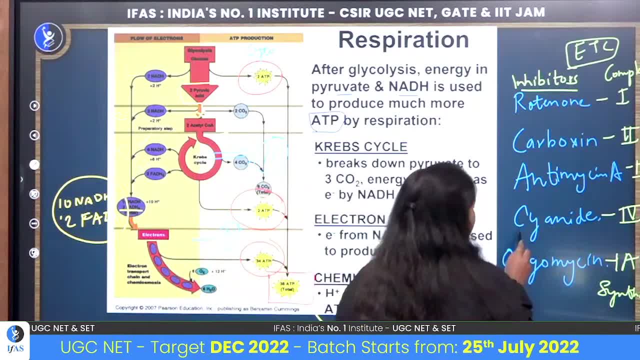 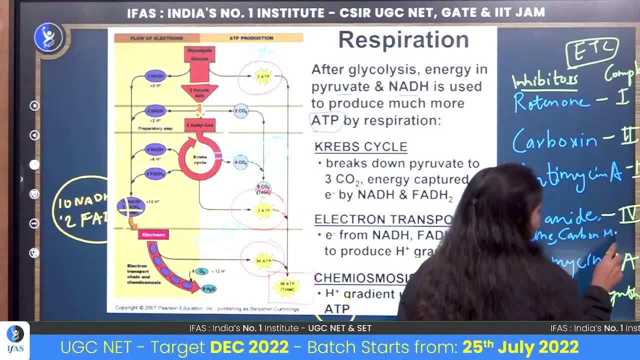 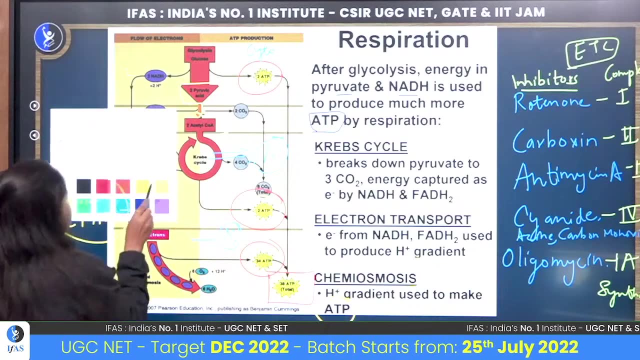 There are many names If we are going to write all of them. So here, Azine will also come. Carbon Monoxide will also come, Then Carbon Monoxide also inhibits complex 4.. Okay, So you guys can remember just one name. 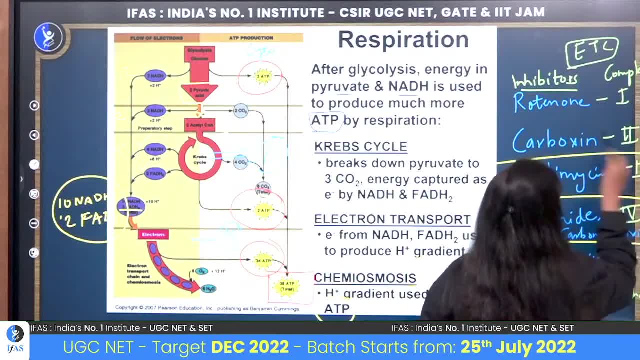 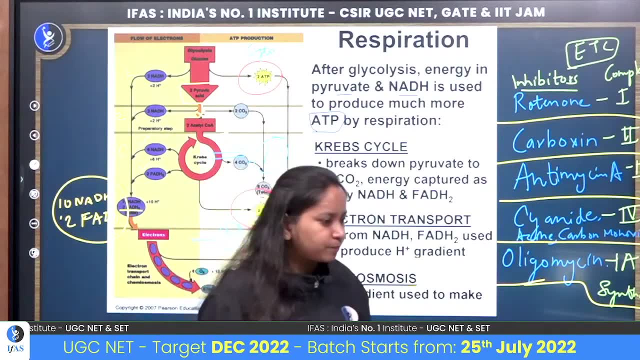 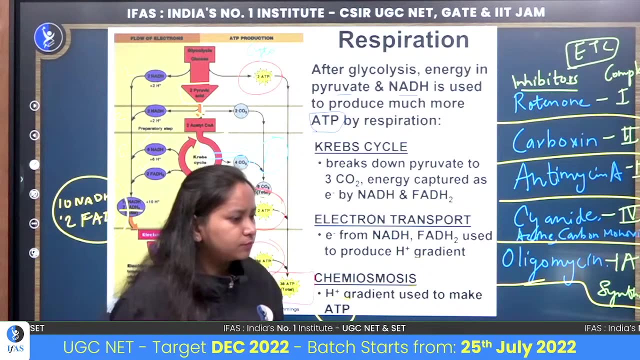 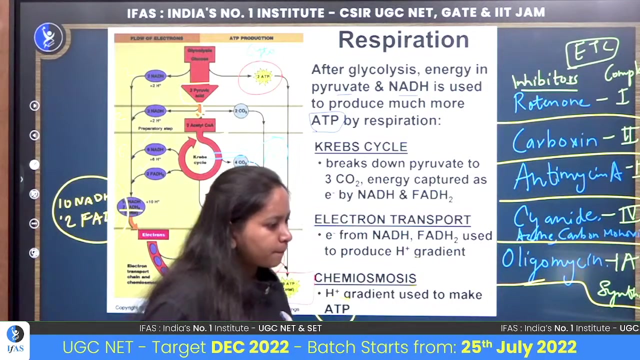 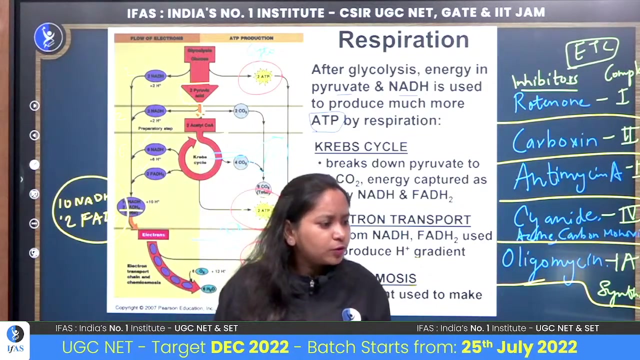 Rest, you can check in our books. You can check in our books, You can check in our books. Okay, So these are the inhibitors of your electron transport chain. okay, is it clear? now please confirm. is it clear to everyone what? no, what happened, child? what is the problem? 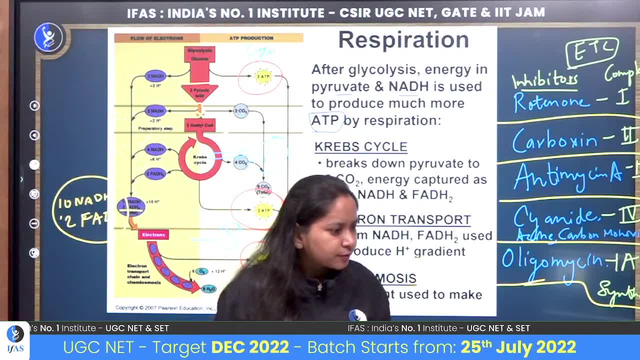 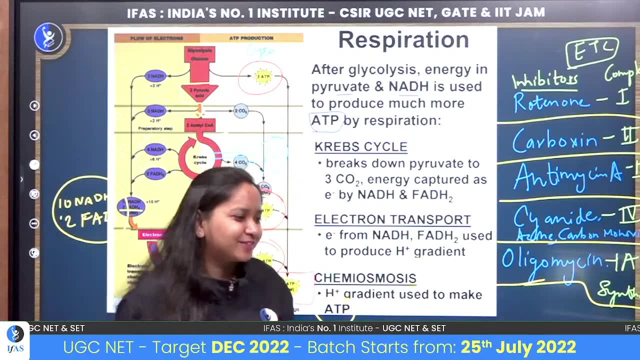 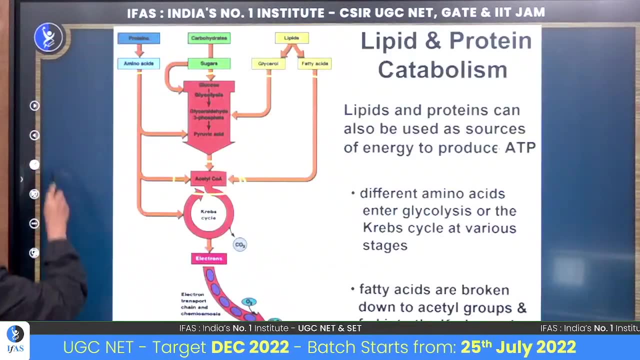 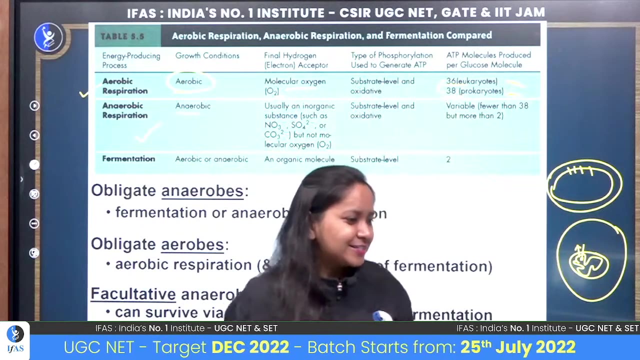 is it saying: yes, what is I? I captain, I am running a ship. if I run a ship, then everyone will drown. I don't know how to swim. you have to save your captain, okay? so yes, if we talk about anaerobes, so they perform this fermentation. 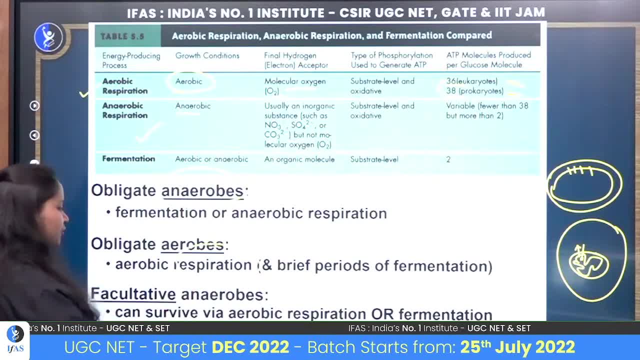 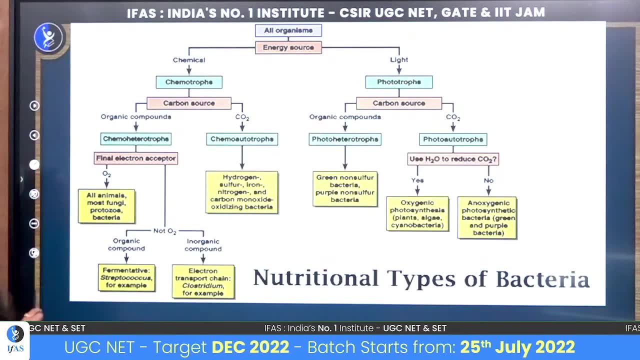 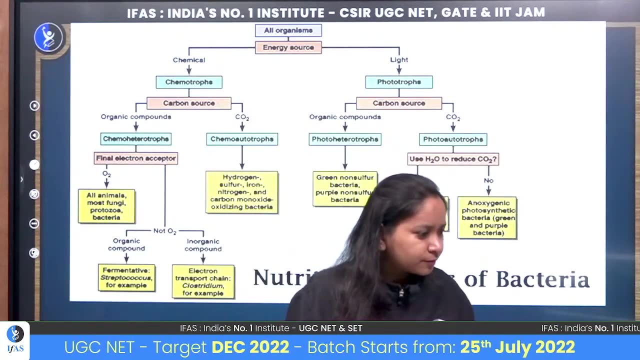 aerobes perform. your respiration facultative can perform both aerobic as well as anaerobic depends, and these are some examples that perform different metabolic. these are the nutritional types of the bacteria. okay, nitrous oxide. I thought you are telling ma'am. I didn't understand because I asked. 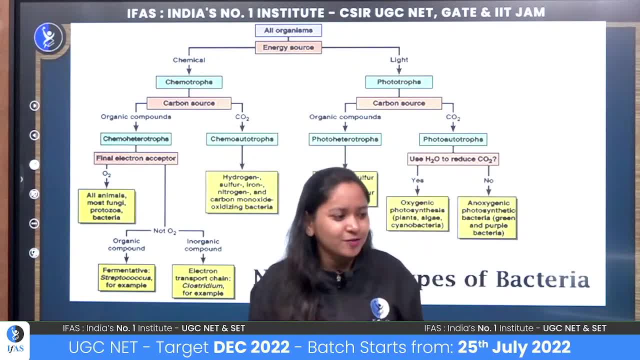 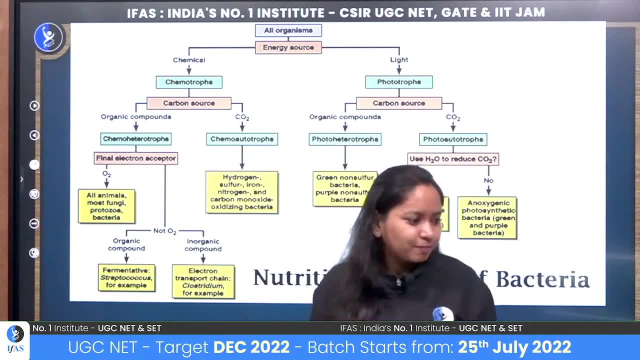 that. did you get it? and you said no, okay, okay, yeah, yeah, nitrous oxide is also an inhibitor of complexes. so see, there are a lot of inhibitors. actually, we had to study metabolism so I didn't add any inhibitor chart. okay, so you can get many inhibitors. you can search. you will get a list of a lot of inhibitors in the net. 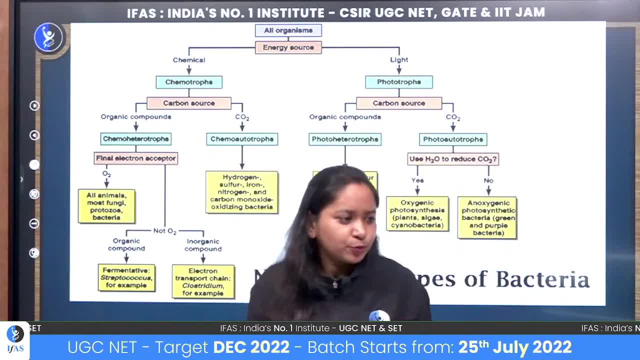 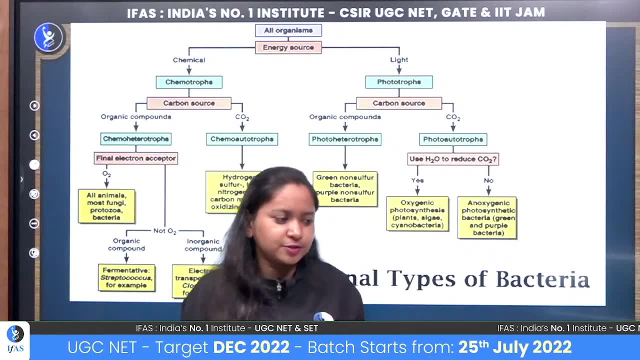 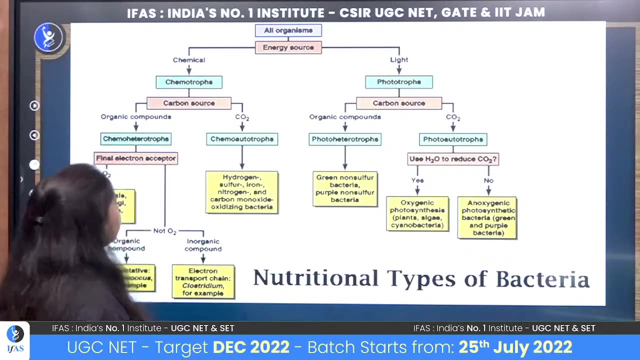 okay, so now the questions will start. now we will have some good questions. come on, call all your friends as well, like and share the session quickly. you all have to practice the questions now. we are very busy, so the question is sorry, not the question. this is your list. we use chemically. 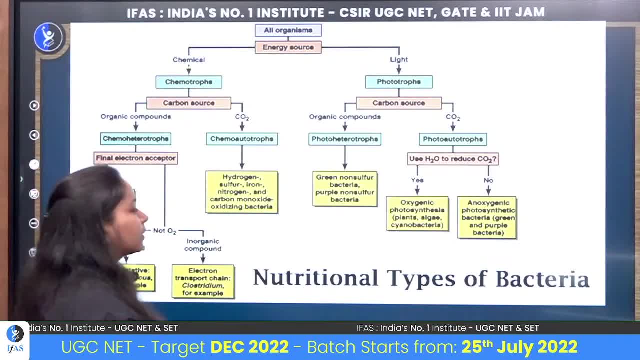 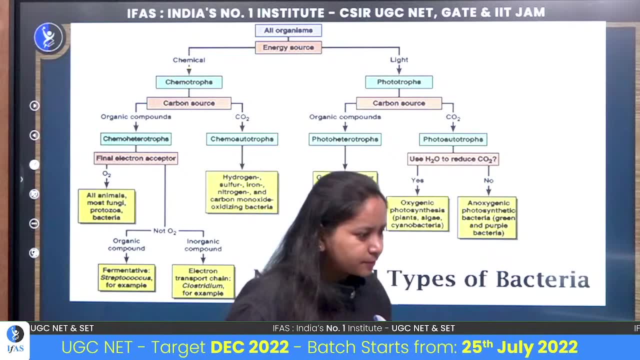 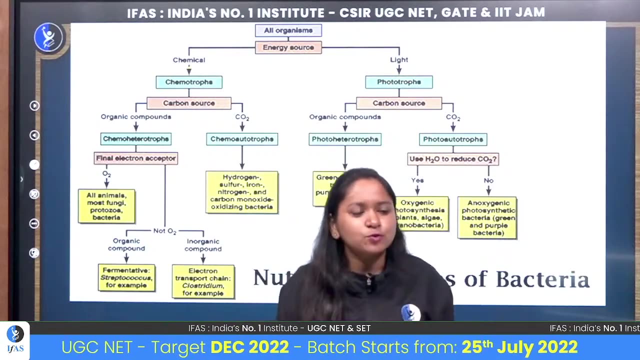 something happens. so if you are going to use light, then remember your list. what is your sulfur bacteria, what is non-sulfur? how does it perform? so you can easily read the chart once: yes, samad, yes. so that's why I am saying that we have so many inhibitors. we have so many inhibitors. I 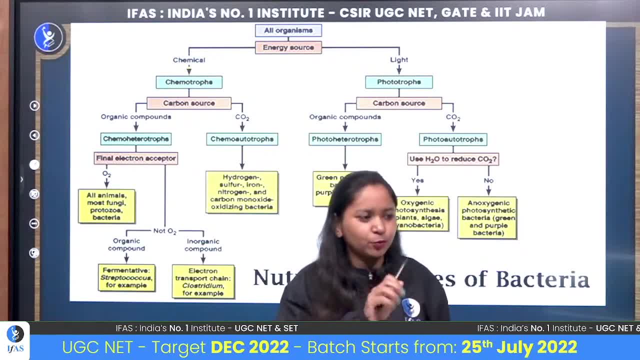 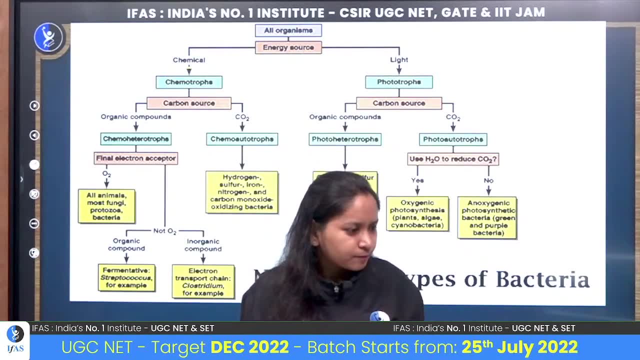 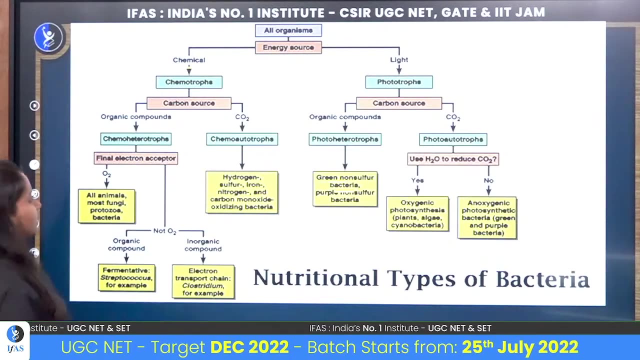 have just given you one name for each. that's it for today. I just give you one name for each. I have not brought a list for you today, so that's why I didn't prepare this. they care now ready for the questions everyone. I think this is the question only. 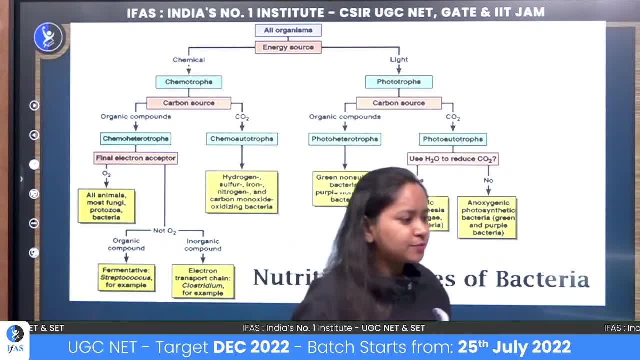 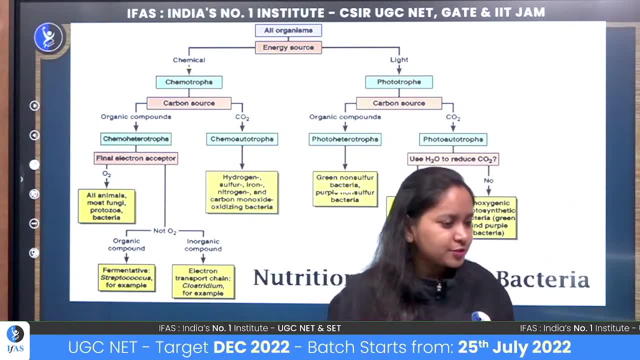 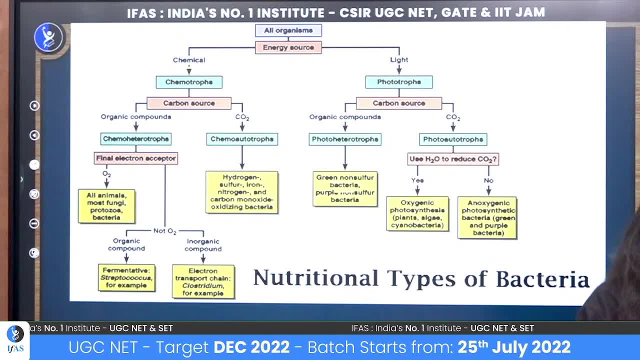 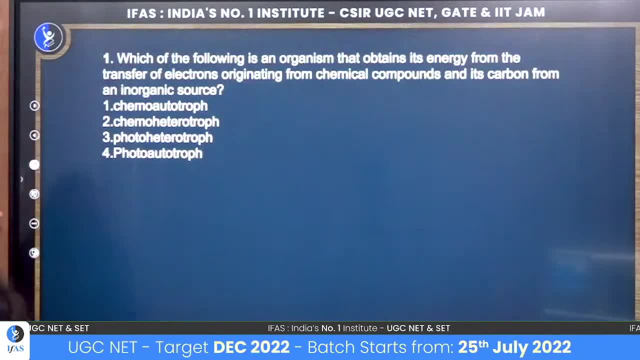 So first question for everyone: give it a try, read it carefully. I am completely away from the screen. Yes, see, Veeru. we got to know the names of all the inhibitors in the chat. these are not all there. so where are the inhibitors? we have so many inhibitors. 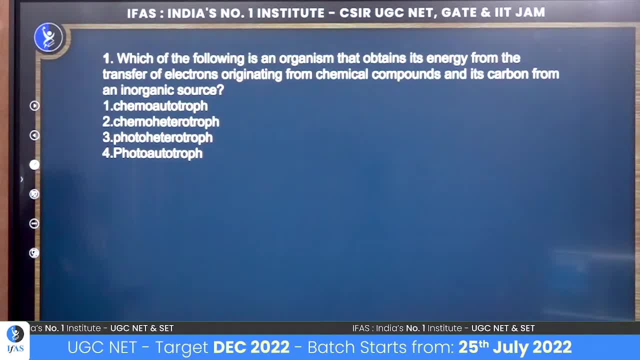 So there are two types of inhibitors: one is non-inhibitor, the other is inhibitor. So the inhibitor is the type of inhibitor that is used to get rid of the inhibitor. So in order to get rid of the inhibitor, we need to get rid of the inhibitor. 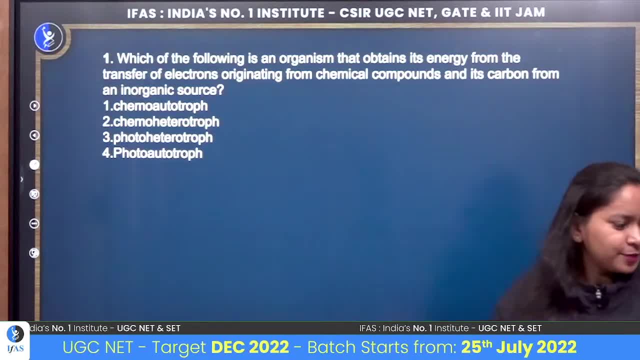 Okay, call all your friends quickly, easy peasy. yes, 1 1, 1, 1 a, a, a, yes, yes, yes, you all are right here. chemo autotroph: yes, what has been asked, the question has been asked, that what is such an organism which will take energy from where it will take? it will transfer, transfer of electrons. 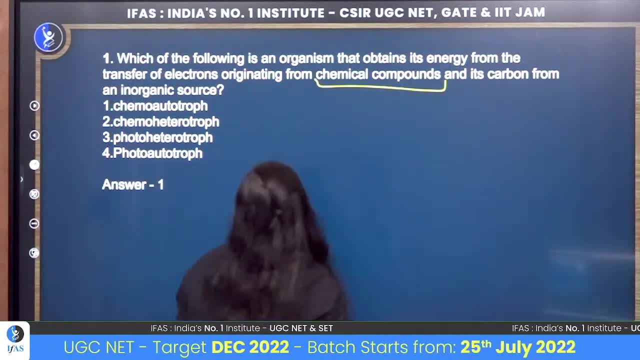 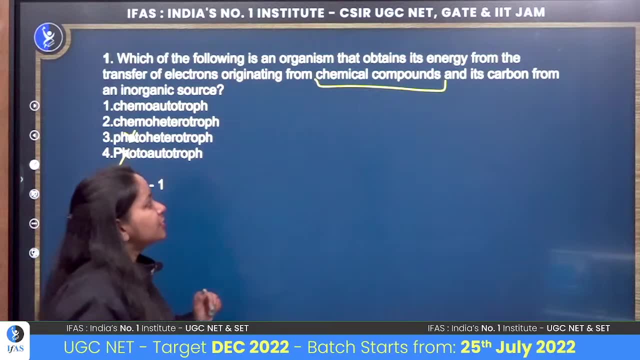 from the chemical compound. chemical compound means what is the photo can't be. our answer can be chemo. only can be using chemical carbon source. it's carbon from an inorganic source. okay, inorganic source means what is? it is a autotroph. if there is any other source, then we call it heterotroph, but it is using utilizing directly inorganic, so that is, co2 will use it. so your answer will be option number 1. option number 2 means when it does not take co2, it takes some other carbon source, like acetic acid, methane, if it takes something. 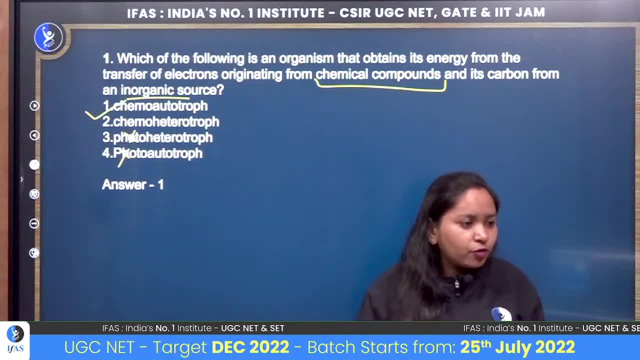 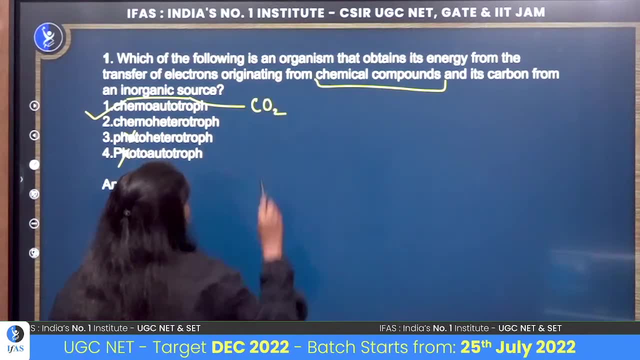 like that, then we can say that, okay, there is something else. in this case, that is will be a heterotroph, but since they are asking us about the inorganic source, that is, co2, so your answer will be option number 1. we started the session with this, by studying. 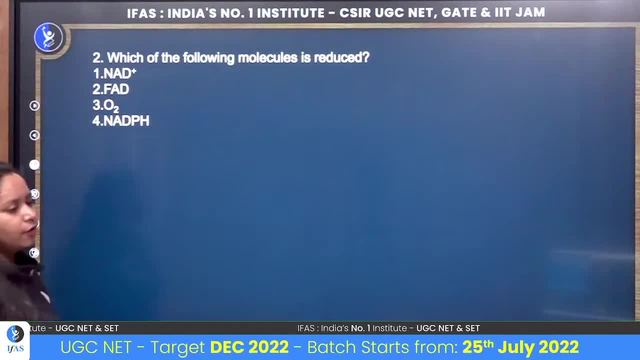 chemo autotroph. next question for everyone: which of the following molecules is reduced? okay, many are saying 4, some is going with 2. I am very confused here. everyone, give it a try, then i will tell you the answer. oh gosh, I am getting three answers from one person. 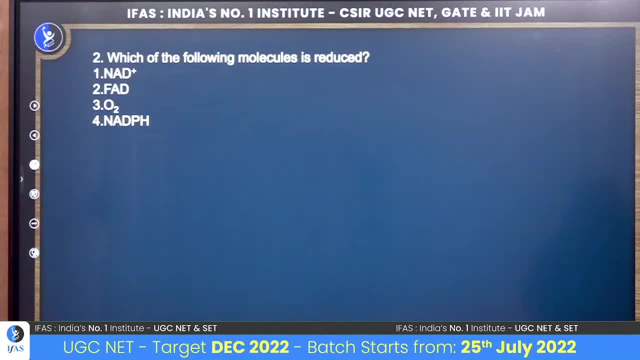 to reduce means now what is to happen? you can reduce it from this form: cheers. sorry sir, please listen to me. are you having a hard time? you are not understanding me. What does reduce mean? The one which accepts electrons. We say that they have reduced. 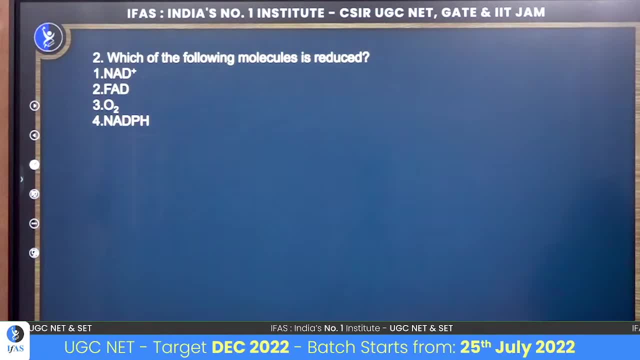 Okay, What are you trying to tell? You can tell One of the above. Okay, Okay, Okay, Yes, The one which accepts electrons. Hmm, The one which accepts electrons, we say that those molecules can be reduced, Okay. 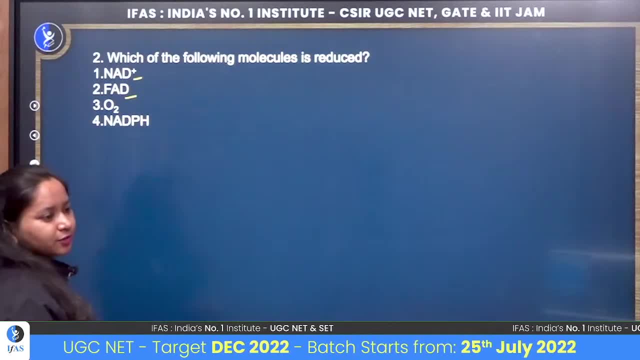 Now, this and this are already reduced. Your NADH- only this is capable of accepting electrons. This form, which is present here, is capable to accept more electrons and can now get reduced. We can also not do oxygen. Your FAD and NADH. 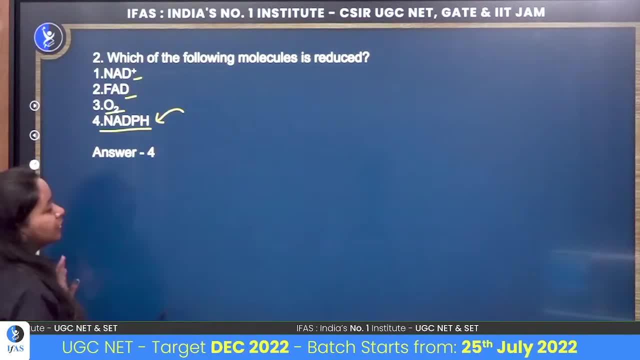 are already reduced molecules. Your NADH can only be reduced. here. The correct answer is option number 4.. Those who have also said 4, bang on. Yes, you all are right, And those who were a little confused. now I think you all are clear. 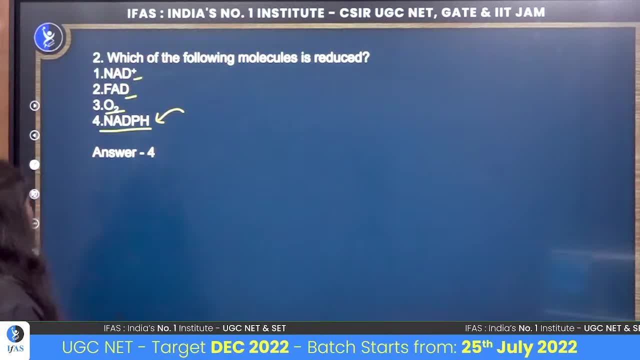 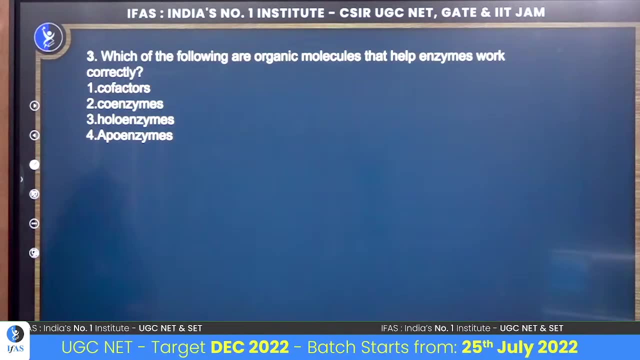 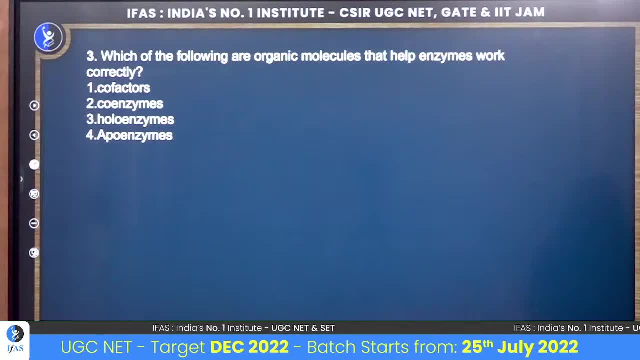 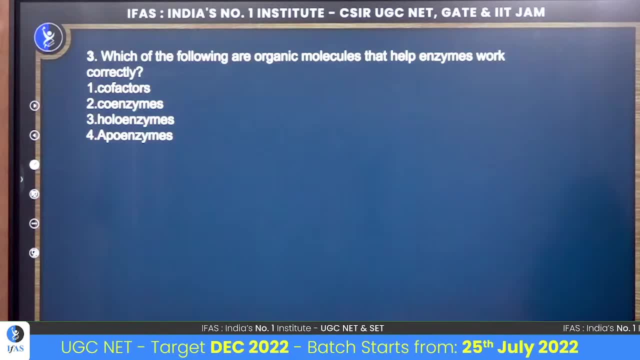 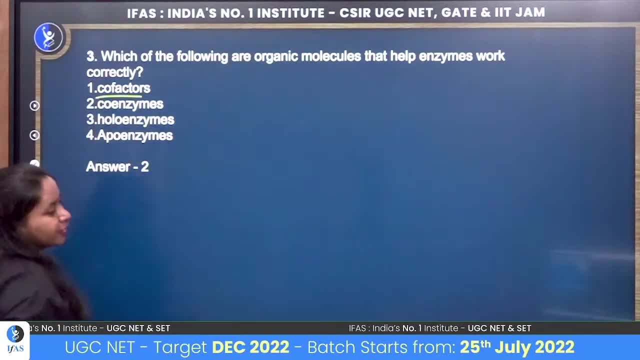 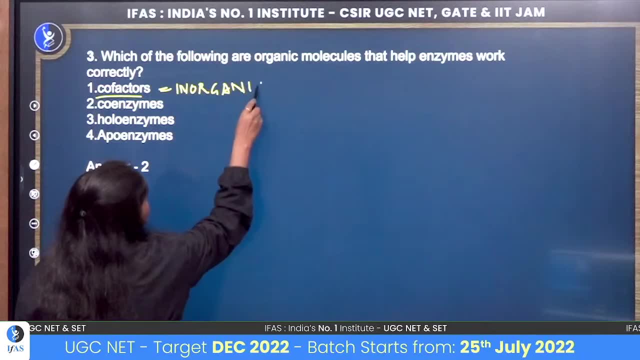 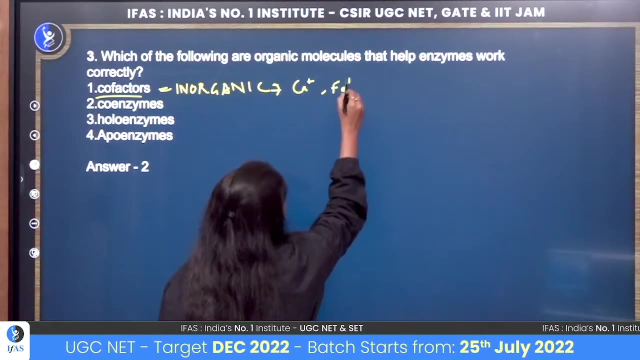 So, yes, they are coenzymes. These are your inorganic molecules. These are the inorganic molecules, Just like your metal ions are there. they come in this. It can be like calcium, iron. Your metal ions are there in the category of your cofactors. In the question, organic molecules were asked, So they come in your coenzymes. Then your enzymes- NADH, NADPH, FADH- are all your coenzymes. These are all the organic molecules which help your enzymes to work correctly. 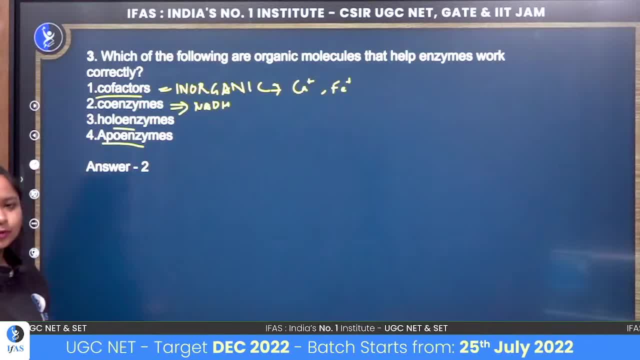 Okay, Rest. these are the forms of your enzymes. Apoenzyme means the inactive form, that is, apoenzyme, And the active form of enzyme is your hollow enzyme. Basically, when all your enzymes are combined, it makes a hollow enzyme, which will make your functioning. 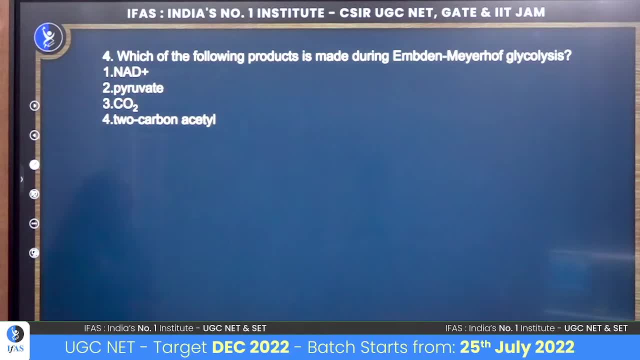 Next question: Which of the following products is made during EM? that is, Emden-Meerhoff glycolysis. What happens? What happens? I am not sure, I am not sure, I am not sure. Okay, So yes, Emden-Meerhoff-Paras. this is how the EMP pathway is called in glycolysis. And yes, you all are right here: Pyruvate is made at the end of your glycolysis. Okay, Next question: During the catabolism of glucose, which of the following is produced only in the Krebs cycle? 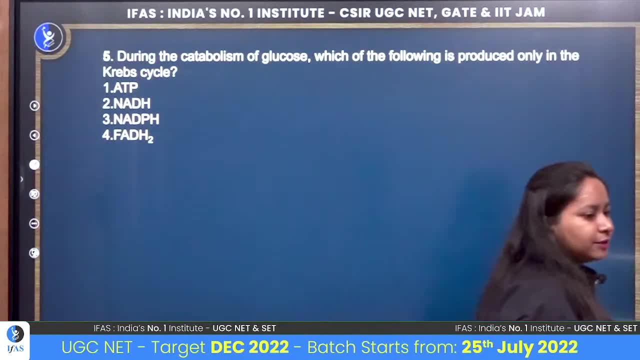 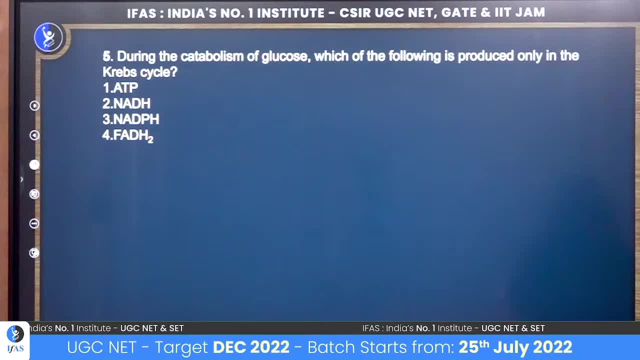 At least, if they are not watching live, let them like. tell them to watch it later on as well, But ask them all to watch 以兼 Discussion. please watch this session as well. Please tell them to watch this session as well. 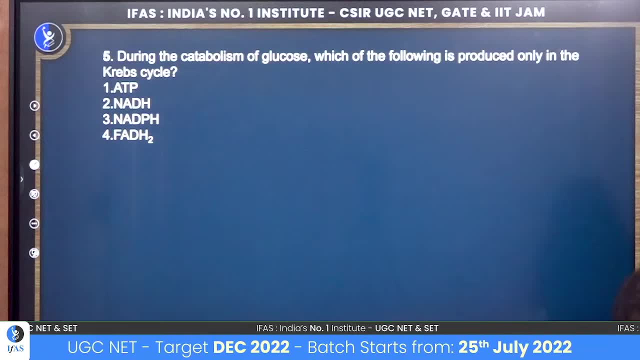 But ask them to watch this session as well, Because Mer Esto ko ingestir titre. thank you V. Mediterranean blood surgery wollen το urhiyar Joanna Banu ulang moralistisch appellate polikiloga. forgot Translate it. Press the subscribe button and share the video. 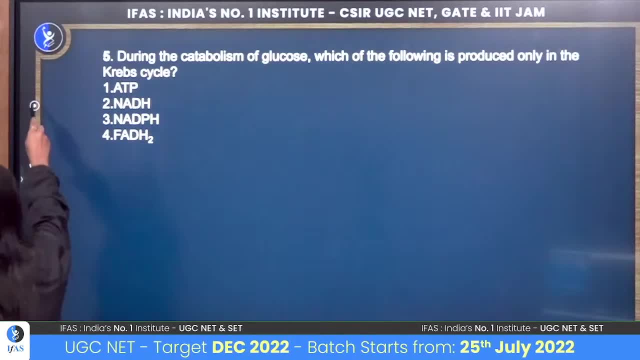 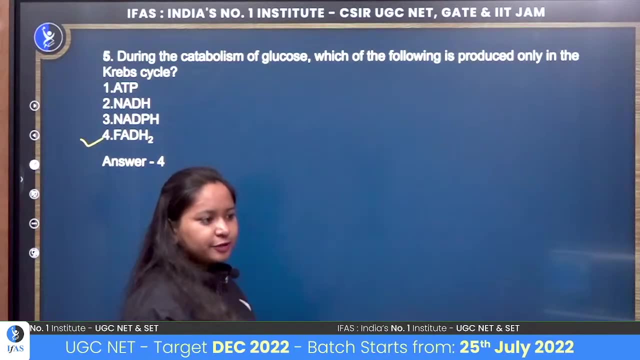 Thike hai, Tell them to watch this session, Thike hai. Okay, Yes, Your FADH2 was there. Rest of the steps were also being done In glycolysis- your NADH, NADPH, ATP- But your FADH2 is specifically done. 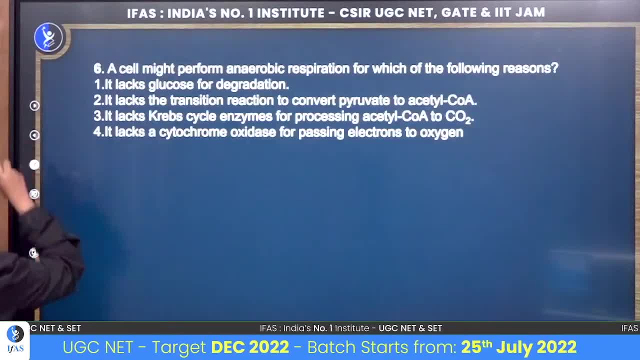 Only in your PC cycle. Next question: A cell might perform Anaerobic respiration for which of the following reasons: Why does a cell perform Anaerobic respiration? What is the reason? Why does a cell perform Anaerobic respiration? Pay attention, read: 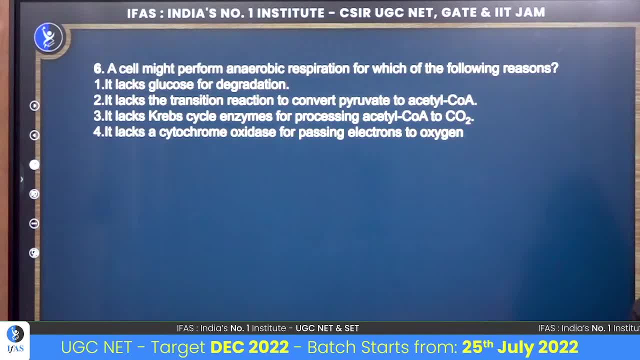 Anaerobic respiration. What is the reason? Why does a cell perform Anaerobic respiration? What is the reason? You are thinking in the wrong direction a little bit. Does endorphic respiration perform? Why does endorphic respiration perform? 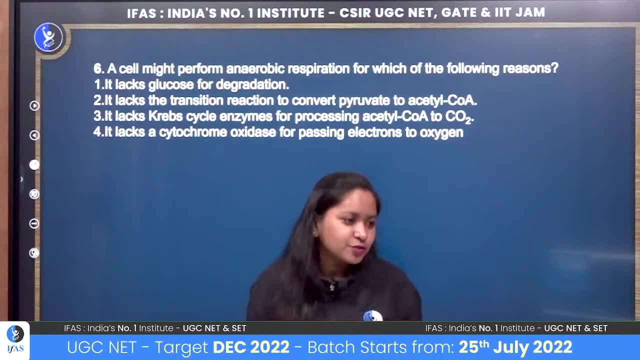 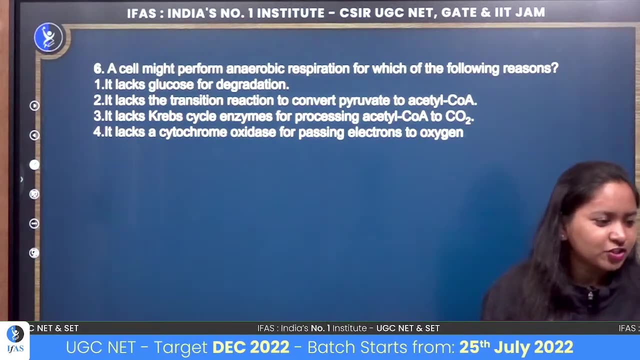 Answer is very simple: Anaerobic respiration. Read the question again carefully. You can change your answers. still, Many people can change their answers. I will not say who wants to change. Yes, yes, yes, So the answer is actually option number 4.. 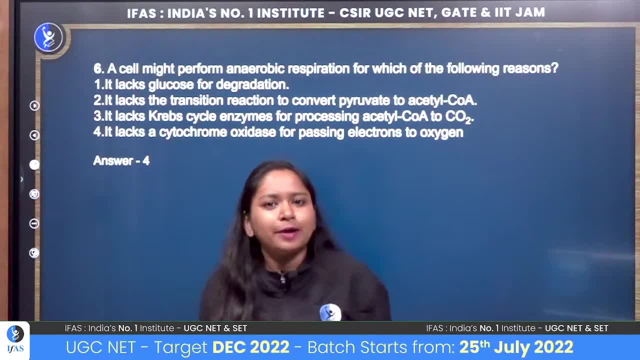 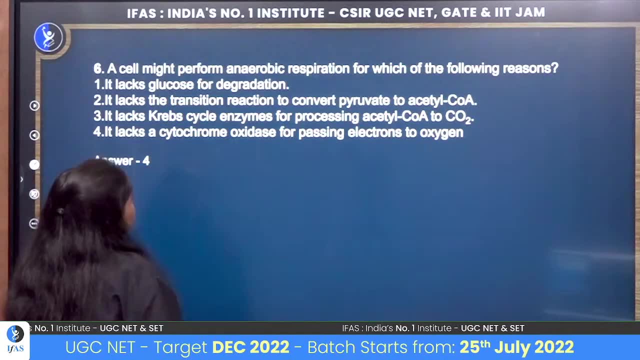 Look what has been said in the question. A cell might perform anaerobic respiration for which of the following reasons Isn't it? Now, it is not like that. What is the first option? Lacks glucose or degradation. Everyone has glucose. What is the second step? It lacks the transition reaction to convert pyruvate to acetyl coenzyme, A Brother anaerobes also perform reactions Even if you make less energy. you do fermentation, you make ethanol, you make something. So it is not like that. 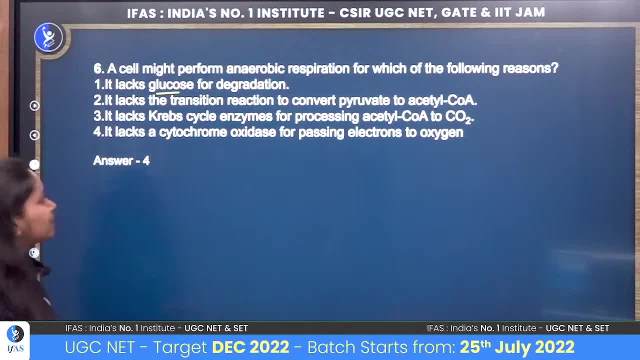 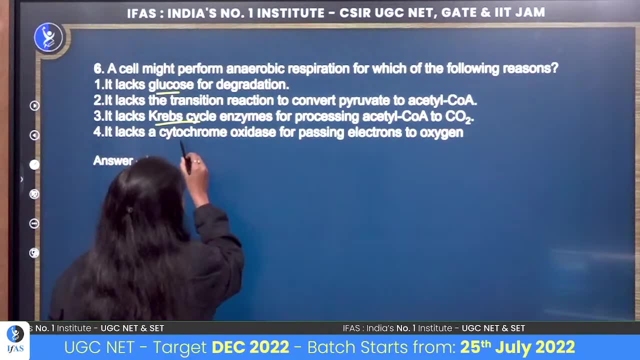 They can't do it. What is the third one Lacks Krebs cycle enzymes. No, they do it, They have Krebs cycle enzymes. What is the fourth one? It lacks silicon oxidase for passing electrons to oxygen. So this is the correct answer. Because they will perform TCA. They will perform transition reactions, Although they will make less ATP, But they will do the reactions. That's why option number 1, 2 and 3 are wrong, Because anaerobes can perform those reactions. 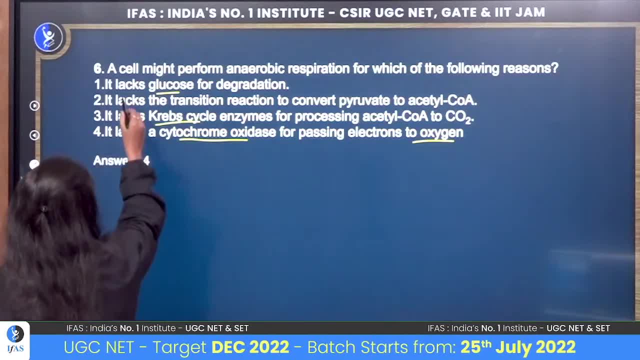 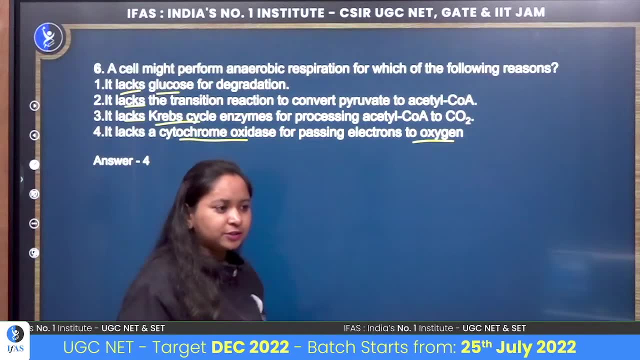 They can do that. What did Bola say in the question? They lack, lack, lack. No, they will not lack. They possess everything. But the difference is that they do not have that cytochrome oxidase enzyme present there, which passes their electrons. 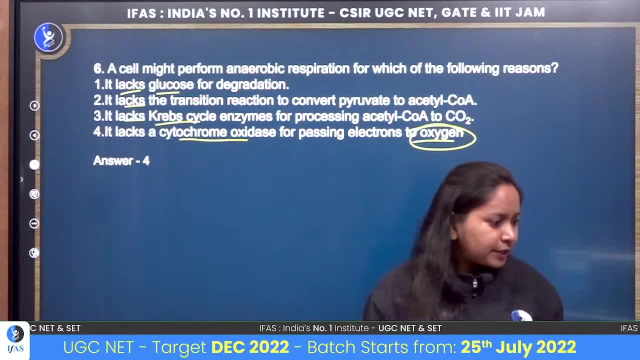 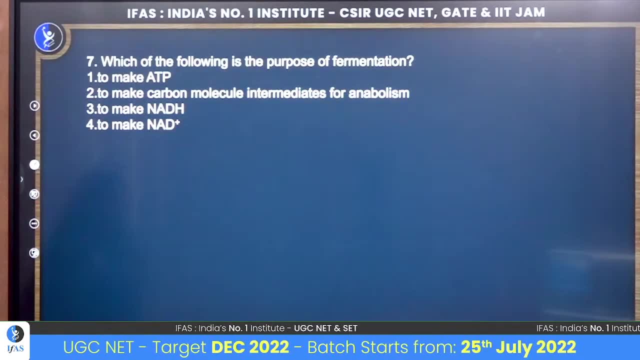 Where did the oxidase come from? It doesn't stay with them. Okay, It's okay. Next question: Which of the following is the purpose of fermentation? I have read that. what is the purpose of fermentation? What is the purpose of fermentation? 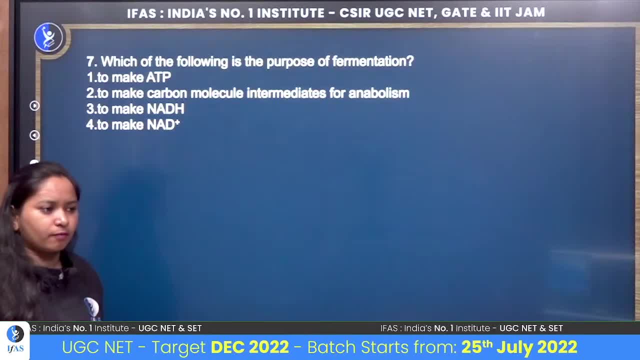 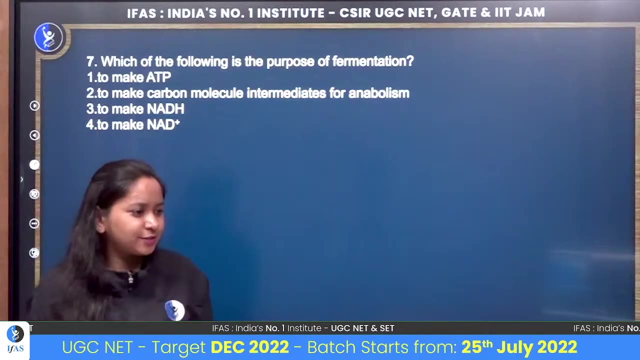 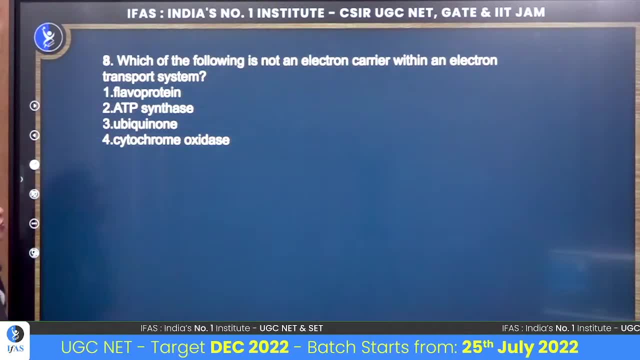 next question, last question: which of the following is not an electron carrier within an electron transport system? not an electron carrier. Rishis, write that they don't cheat. they don't ask me to copy. if they cheat, then it will be like this: which of the following is not an electron carrier within an electron transport chain? 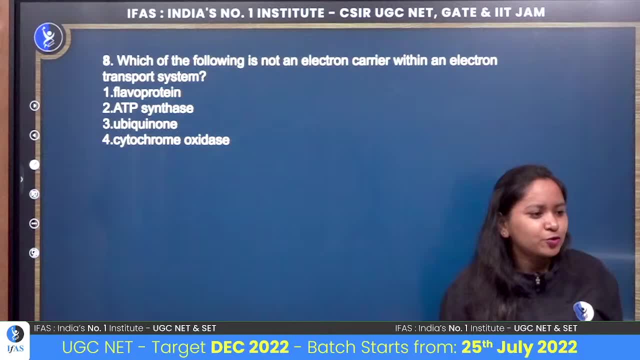 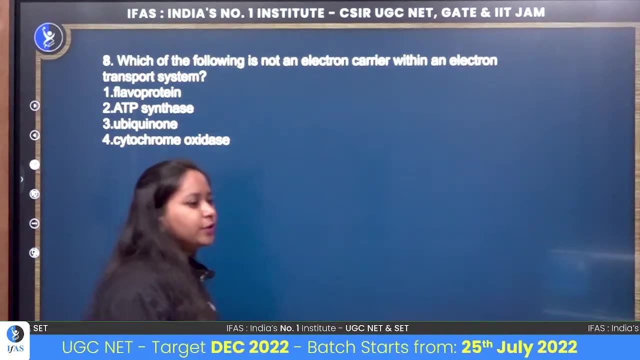 which of the following is not an electron carrier within an electron transport chain? so yes, yes, yes, most of you are right. the option number 2 is the correct answer here. what does this do? it doesn't carry electrons. actually, when electrons flow, a proton gradient is formed which makes the synthesis of ATP. 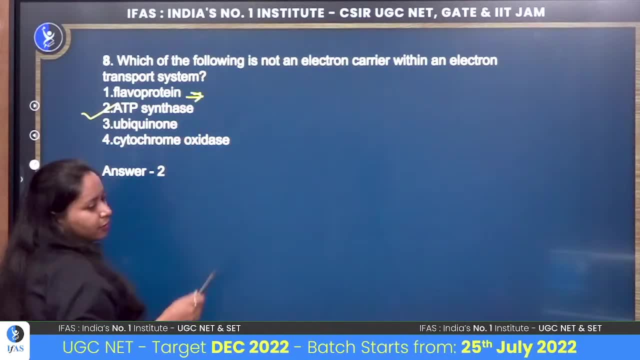 ok, flavoprotein is used in the plant electron transport chain. we don't have it, but it is used in plants. what is flavoprotein? this is in us. ubiquinone and cytokine oxidase is in us, but this is not in us, but in plants. 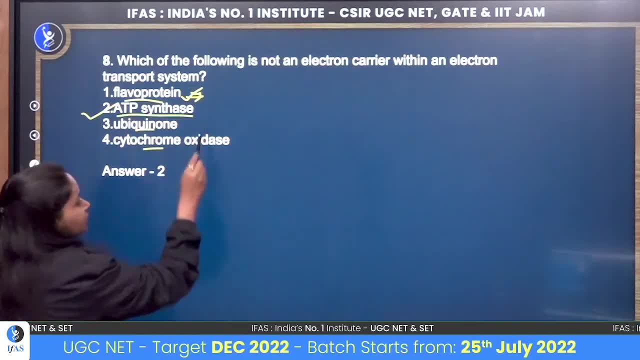 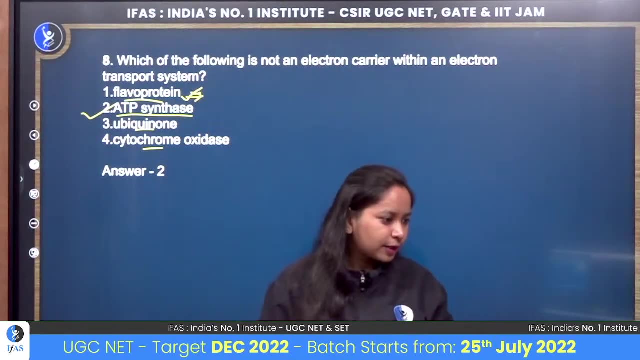 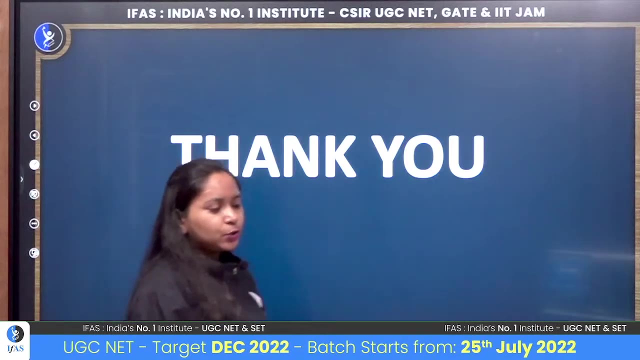 flavoprotein is present there, but the ATP synthesis that never carries electrons, only passes protons and pumps them out, and it does the generation of ATP ok, so that's the correct answer, option number 2, and not any other option. so, yes, thank you everyone for joining the session. 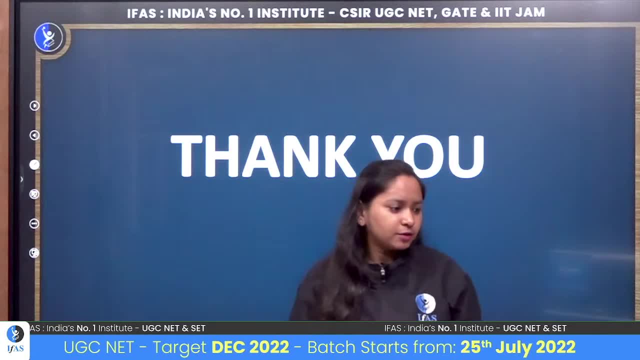 stay with me for the whole week. we have done a lot of studies. oh so ok, so we have got a good quote. yes, the person who fails the most has a lot of good stories. Janhvi, all the sessions, kids, you will get on the channel only. 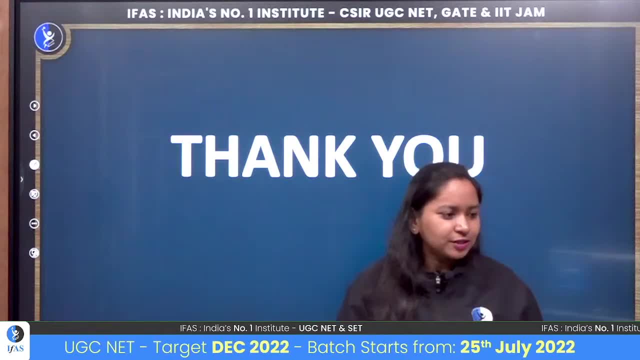 you go to the channel IIT GADBI, which is the official channel of IFS. in that session you will get all the sessions. all my sessions are there from the line lecture 1,, 2,, 3,, 4,, 5. this is the 5th session. 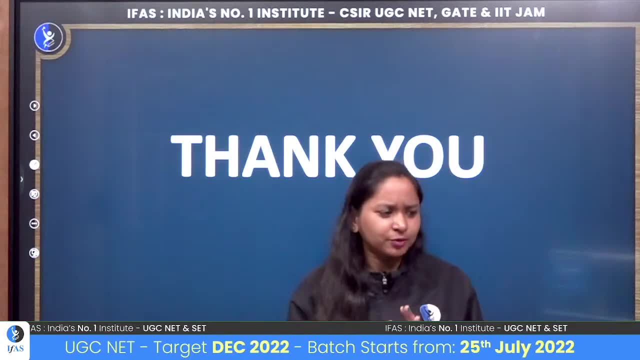 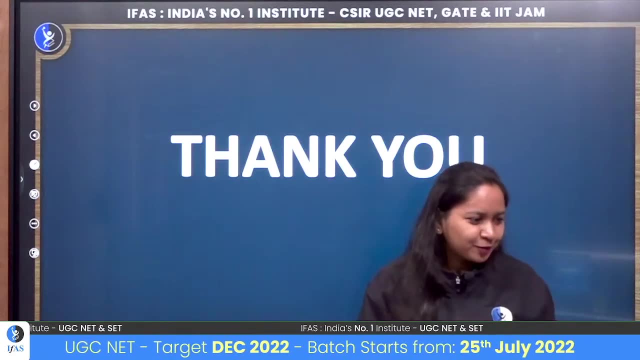 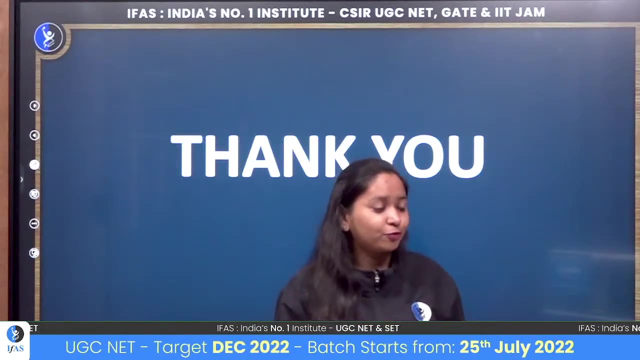 you can get this session later, but you will get this session by the evening. but you will get all the 4 sessions here, absolutely sure. I also had a lot of fun with you guys. we had like good time, we had daily like good sessions, and for all your love and support. 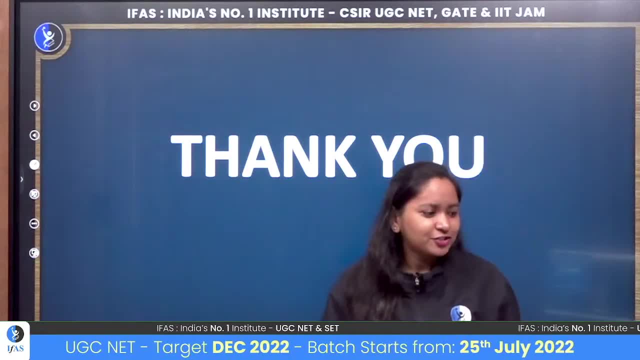 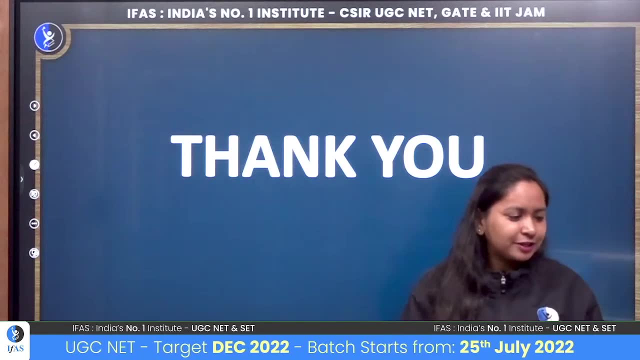 because you all responded so well. that made me more energetic for the session. yes, it's lunch time. Virgi is hungry. ok, you can go and have your lunch. no, no, no, these are not permanent. actually, from next week your second talk will start. ok, some other teachers will conduct sessions for you. 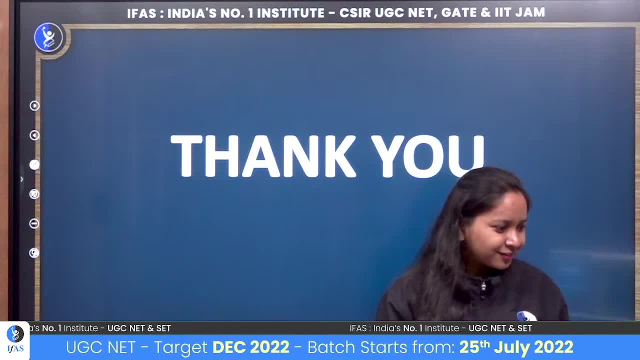 my session was about microbiology. it was till here. oh, in the next session I forgot that we had to do something like this. ok, I just remembered that thing, no problem. ok, we have to take a lot of sessions on YouTube, ok. so I hope you all enjoyed the session. 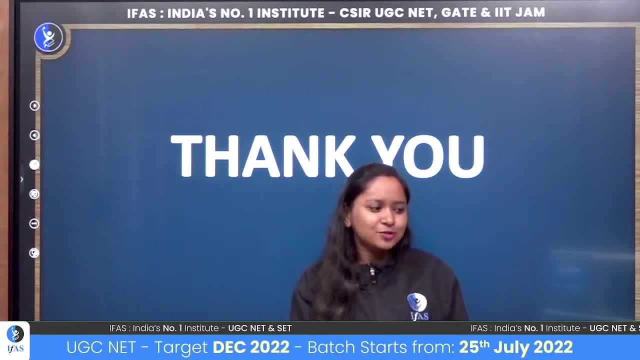 you had a good time. we learnt a lot microbiology today and please- yes, those who haven't watched the sessions, the old ones- please go and watch the sessions once again. you will get a good information about all this, all the lectures of microbiology. ok, you will get the questions from here. 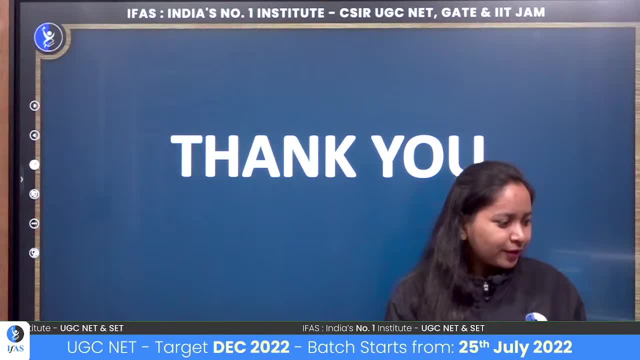 you will be able to attempt all of them. that I can tell. ok, yes, yes, definitely, I will be back soon. we will conduct more sessions in which we will bring a new series for some other topic. if you want any specific sessions, you can just post in the chat box. 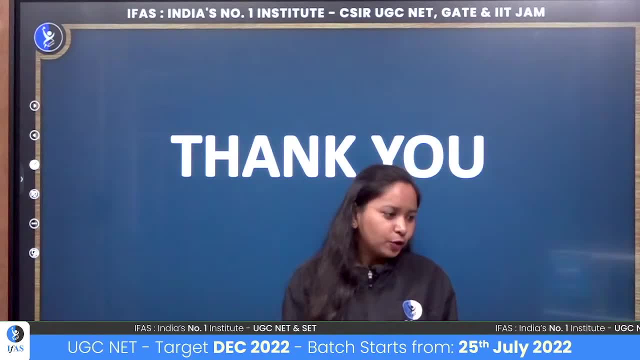 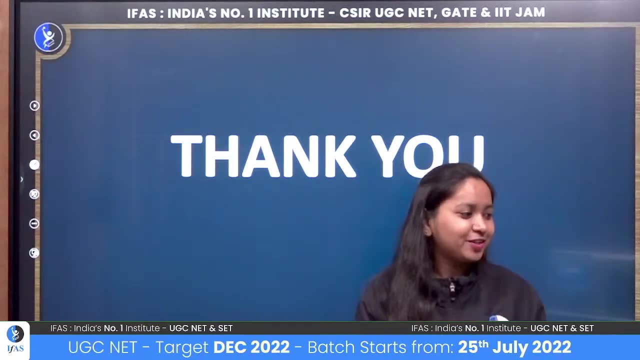 you can write in the chat box which sessions you want to do. you have to do revision, then we will conduct such sessions for you. stop it now. you will run away. all of them will go away in the next series, for sure. I am so sorry I don't do like this. 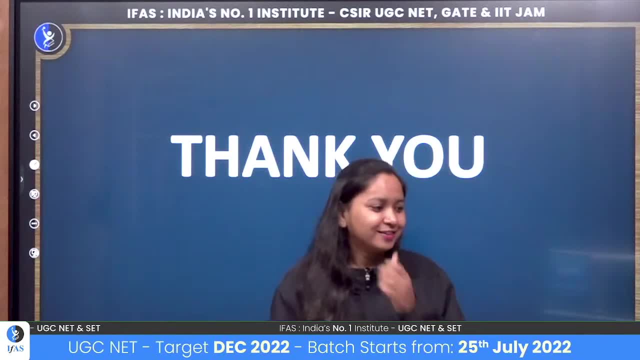 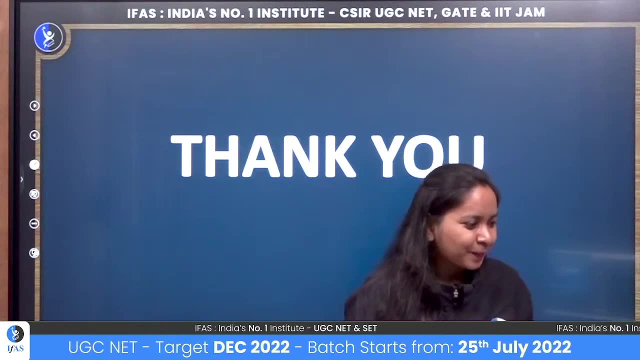 that, I don't want to say it, but I forgot. I can tell you a story, but I don't remember anything. but, ok, you want immunology? ok, no, no, no, so, ok. so, whatever your requests are, you can post them at the end of the session, after the session ends.